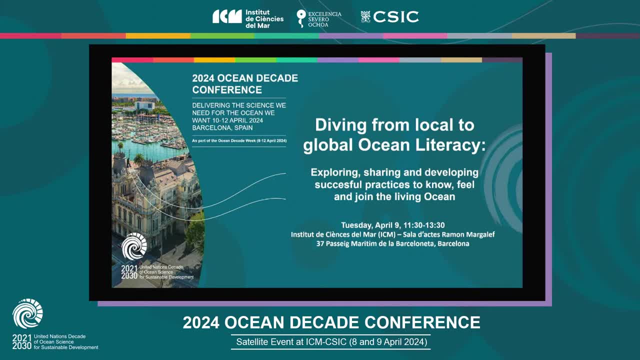 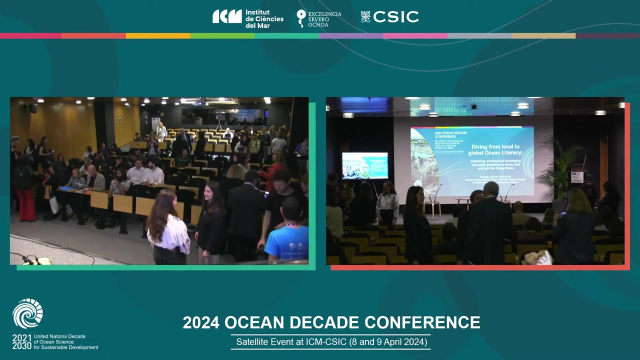 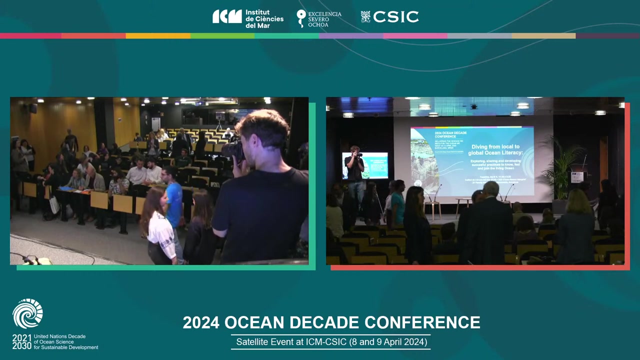 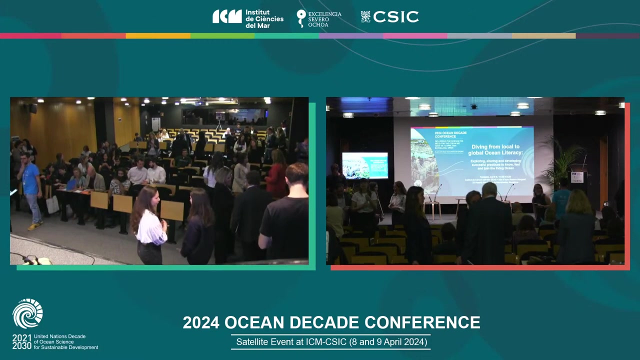 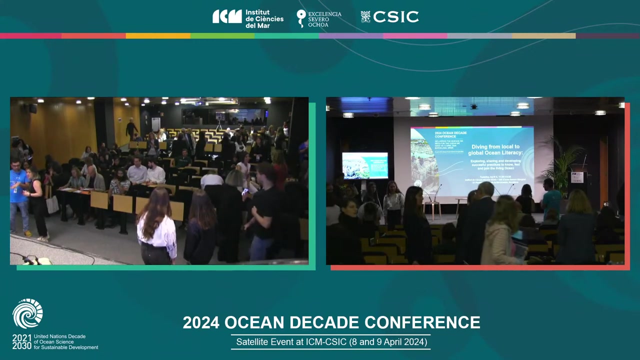 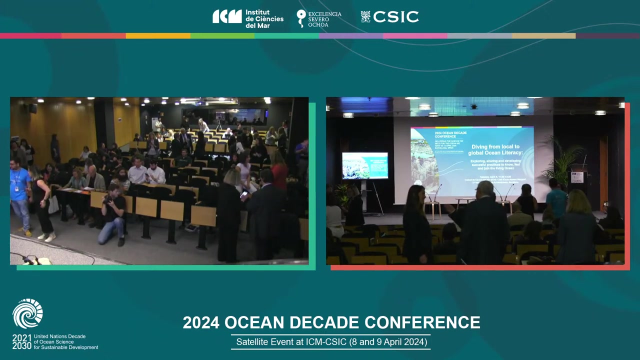 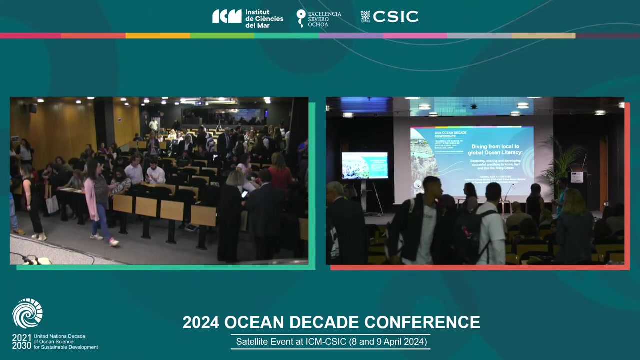 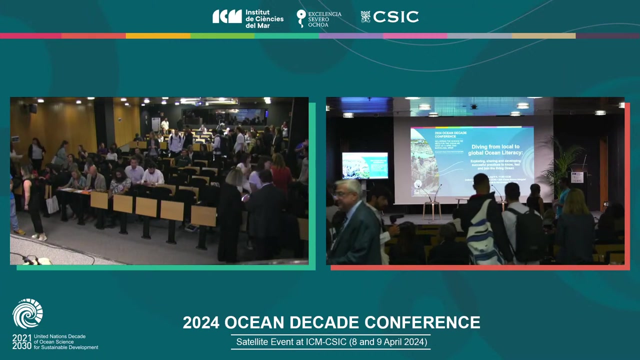 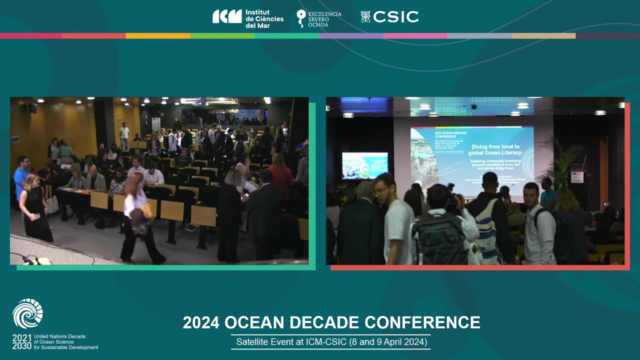 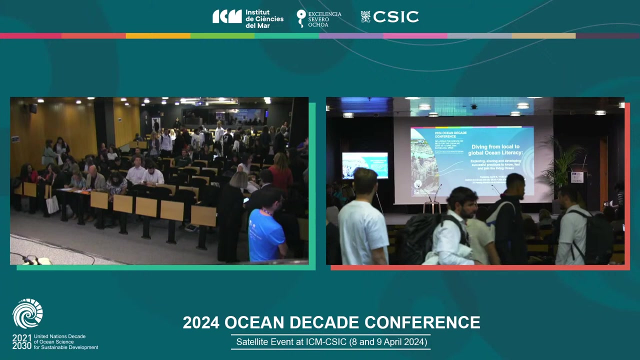 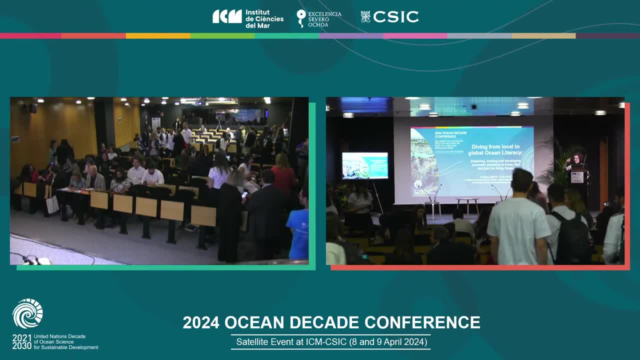 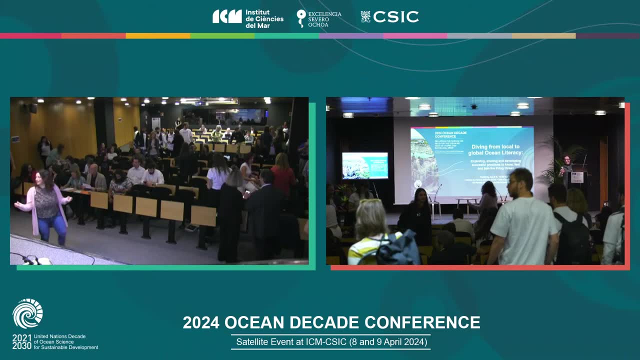 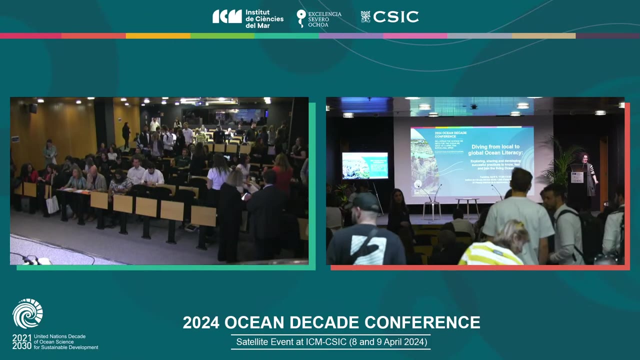 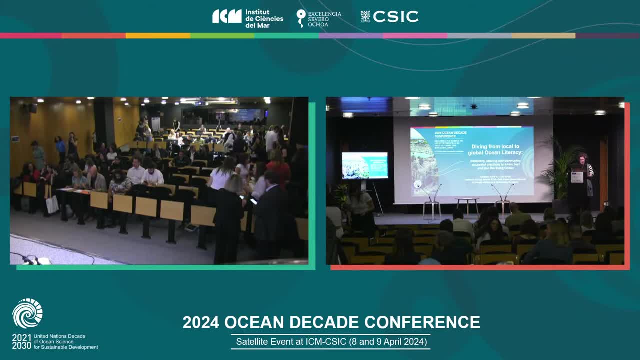 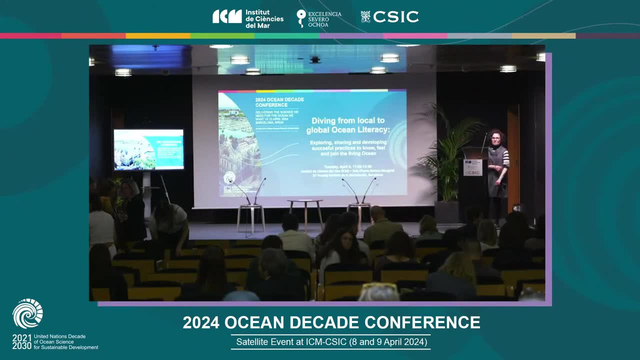 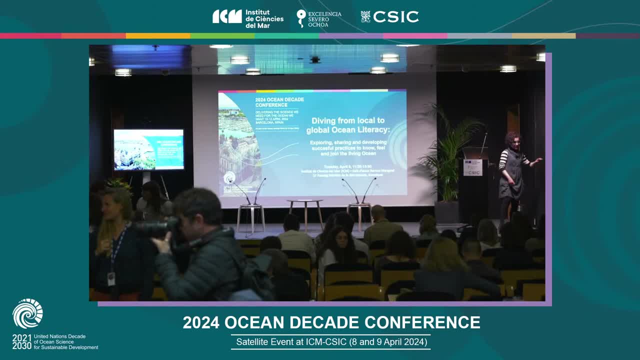 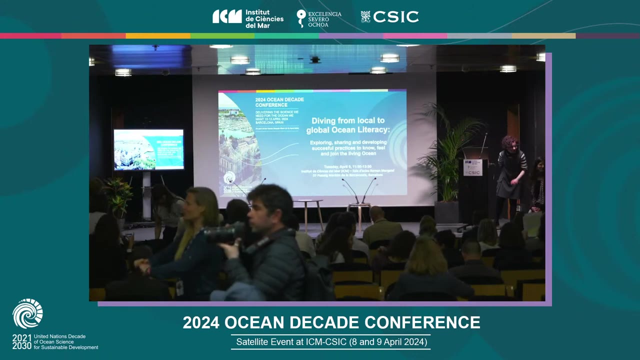 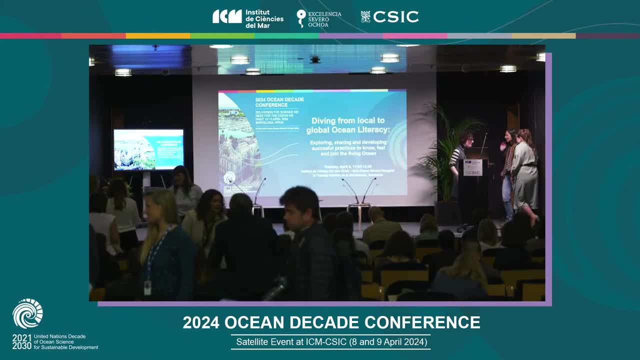 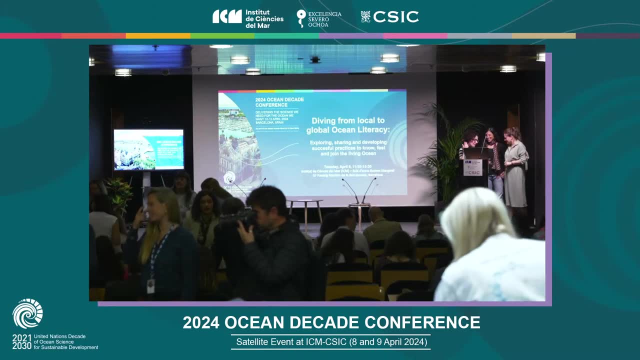 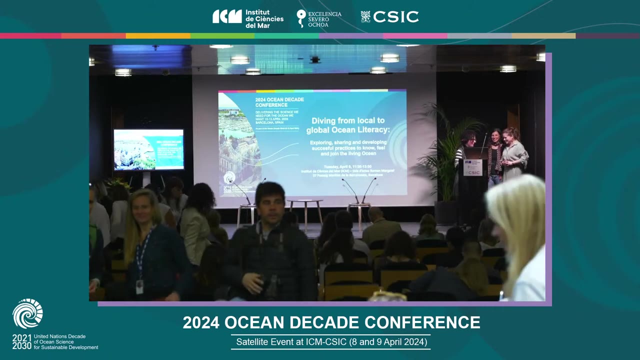 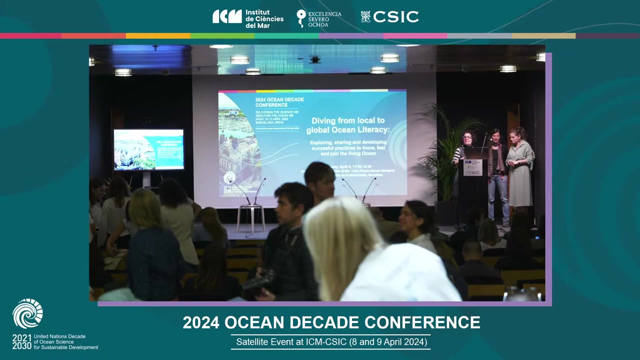 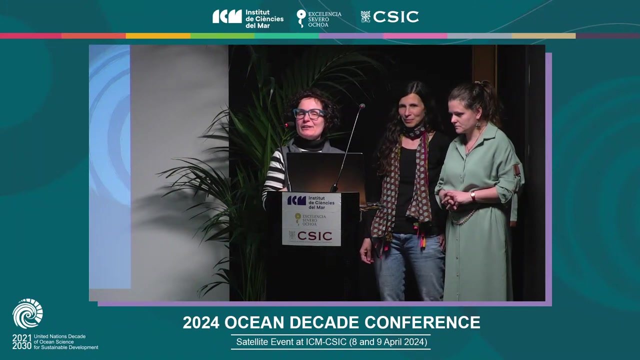 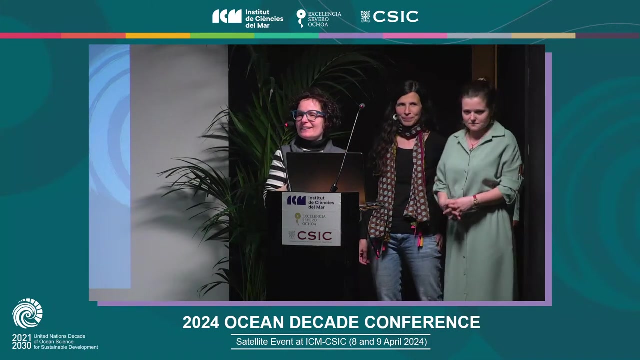 Thank you for watching. Thank you for watching. Thank you for watching. Okay, Hi all, It's great to have you here. We are delighted for you to be here, So we are going here together. sorry, what's the matter? 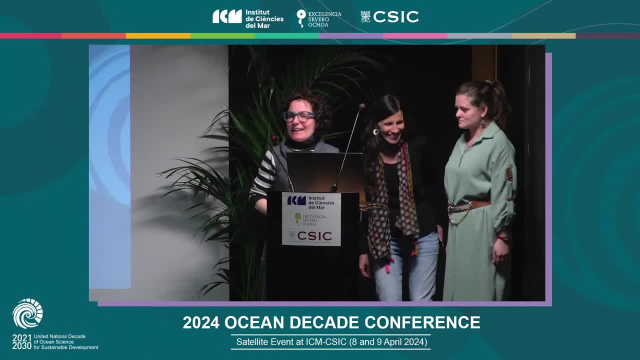 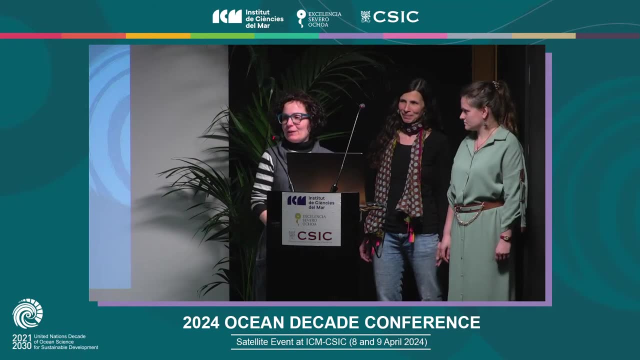 Thank you very much. Okay, so I hope you enjoyed yesterday, the first day of the Ocean Day Week. So, as you all know, I'm sure, one of the challenges of the Ocean Day is to change the relationship between humanity and the ocean. 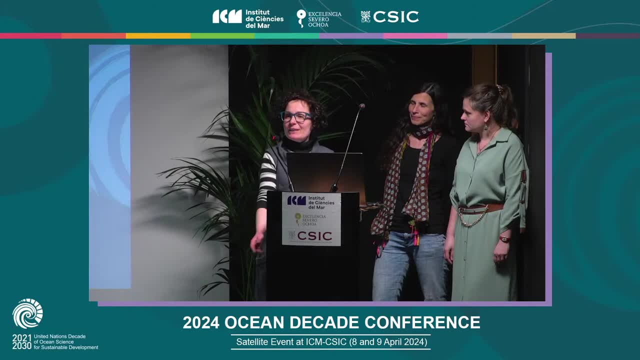 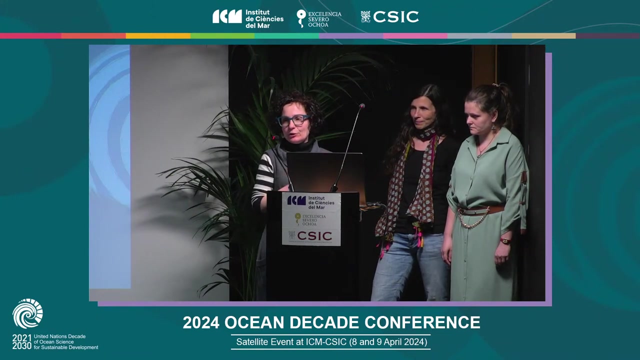 And one of the problems, one of the major methodologies to do that, is the ocean literacy. And ocean literacy has changed a lot over the years. It's moved from being purely science and knowledge-based and limited to the school environment, And it's now deployed, I would say, in all many possible contexts to try to fill this gap between us and the ocean. 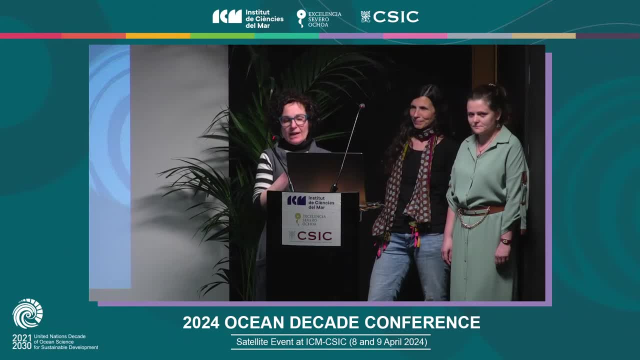 So today, with our event that is called diving- you can see there diving- from local to global ocean literacy, exploring, sharing, developing successful practice to know, feel and join the living ocean. we want to share with you through four very engaging panels. 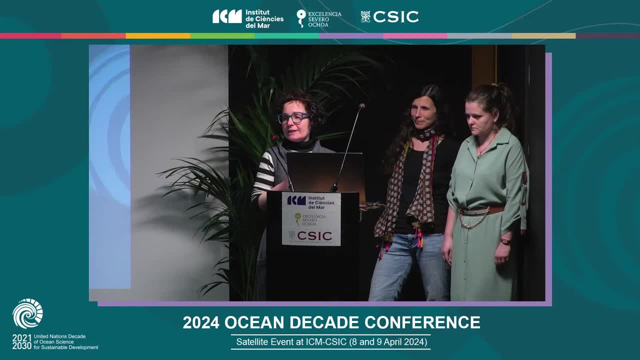 some successful stories of how ocean literacy has been used worldwide to create impact to deal with at local level with the global challenges of our times. So this is going to be a hopefully very inspiring event for all of you, but I must say from my side it's the result of the work of a fantastic group of people. 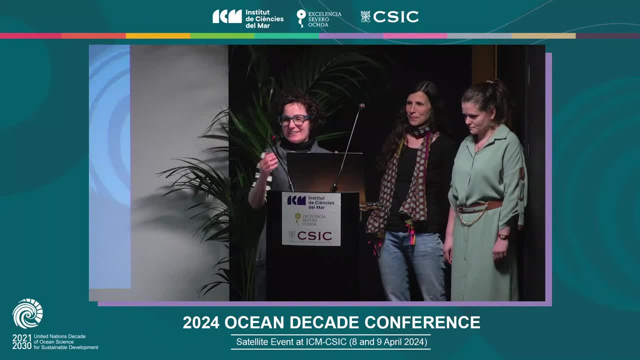 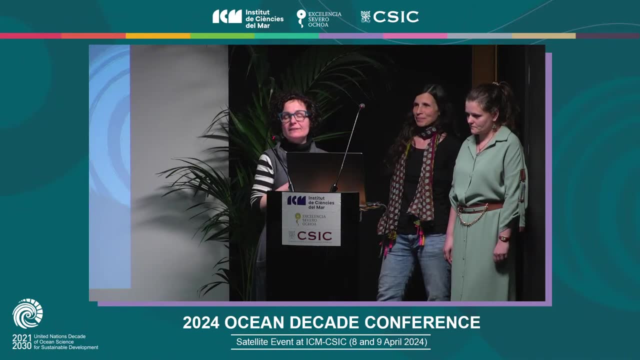 And we, the three of us here, just represent the three original proposals that were merged to create this event. So I introduce myself. I am Maria Victoria Marra. I work at Galway Land Aquaria and for the Irish Ocean Literacy Network in Ireland. 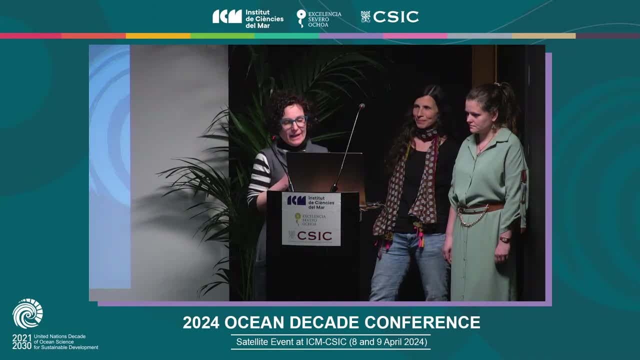 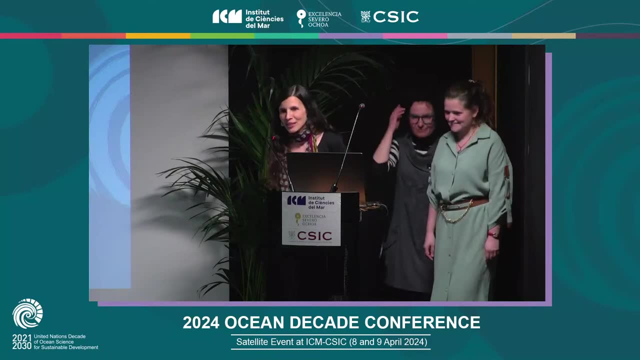 And I'll be the general moderator for today And I'll pass the word to Begoña. Thank you, I'm Bego. I'm a teacher and I work at the University of Barcelona, and I was a former PhD researcher here in this house. 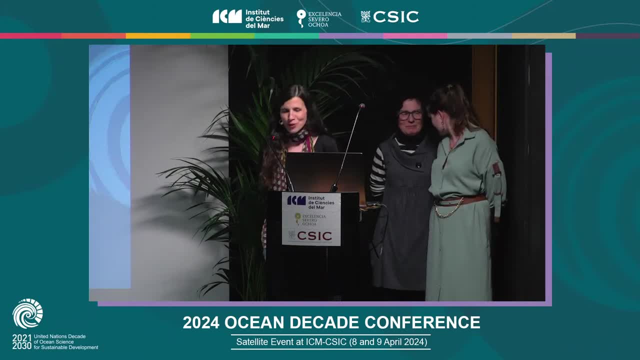 And now I'm conducting the PhD on ocean literacy, of course, But I just wanted to remind you that we have a small but very nice poster exhibit. It's up here and you just go up the stairs and it's in one of the terraces. 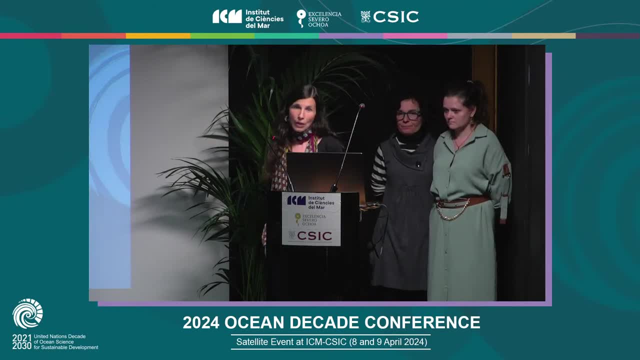 And there are very nice posters on local initiatives and some which are not so local, And the authors are here in this room. so after the event you are invited to go there and visit the poster exhibit. We have also left some post-its and some pencils. 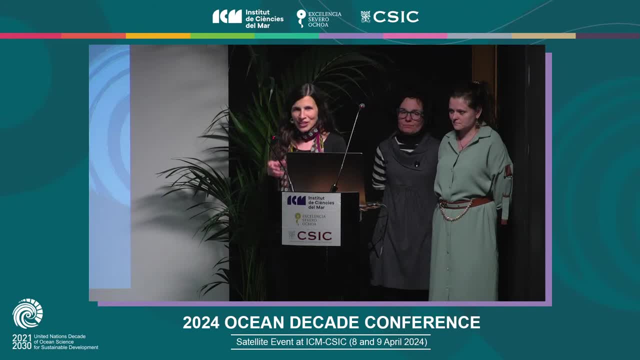 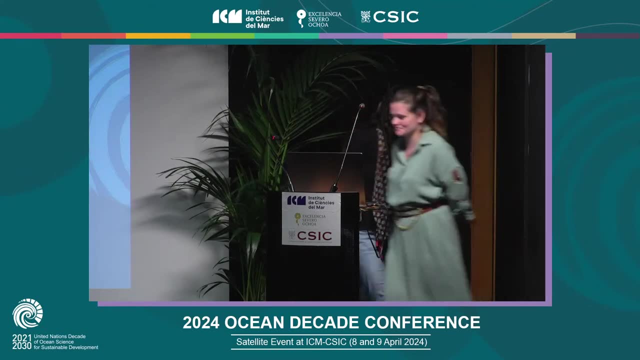 so if you want to write comments or questions or leave your contact on the posters, you can also do that, So we encourage you to visit them. Hello everyone, My name is Eugenia Castanei. I represent the third proposal. 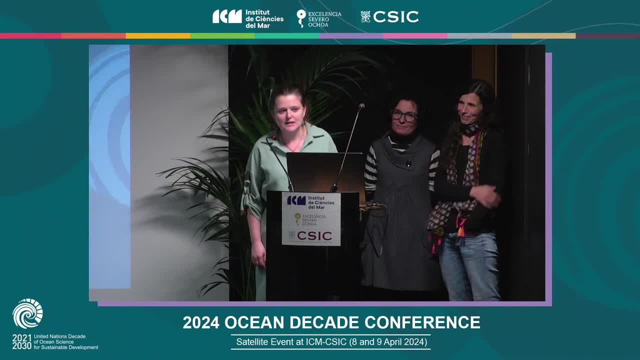 I'm the global coordinator of the ECOPE programme, which stands for the programme, the Euron Ocean Decade Endorsed Programme for Early Career Ocean Professionals. So two months ago, the ECOPE, the ECOPE Programme, Ocean Literacy Task Team. 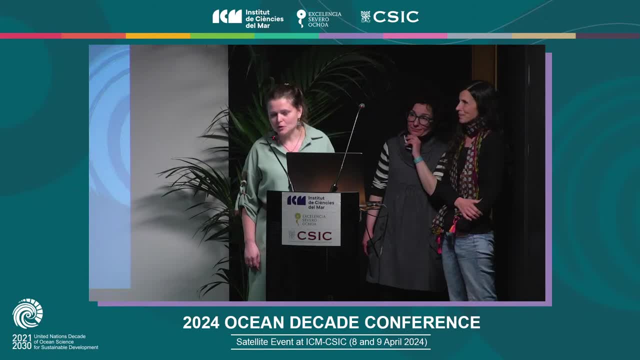 and the ECOPE Programme, Ocean Literacy Asia Hub launched a big worldwide campaign to collect materials on ocean literacy activities. We were looking for successful stories, innovative approaches that people were doing in their ocean literacy work across the globe. We especially were encouraging applications and submissions. 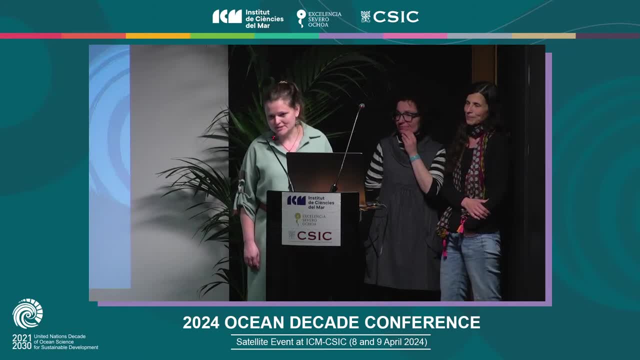 from the regions and countries that are normally underrepresented and such discussions around ocean literacy. So, in the context of our initiative, ocean literacy would encompass both formal and informal education and we were really looking for some innovative approaches. So we received really a great number of amazing submissions. 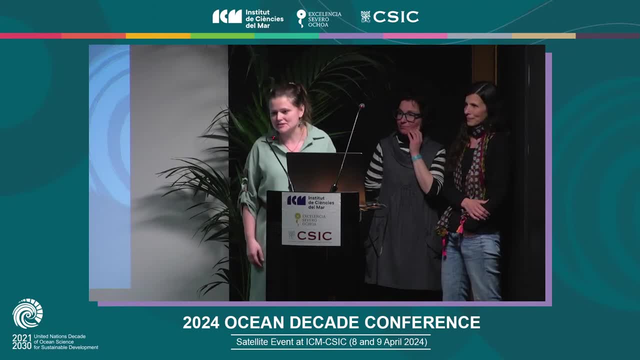 We learned a lot, and some of the people who submitted they are here in this room. they will talk about their work, And so the results of these findings will be presented right now. today and at some other events. It will be shared on our social media. 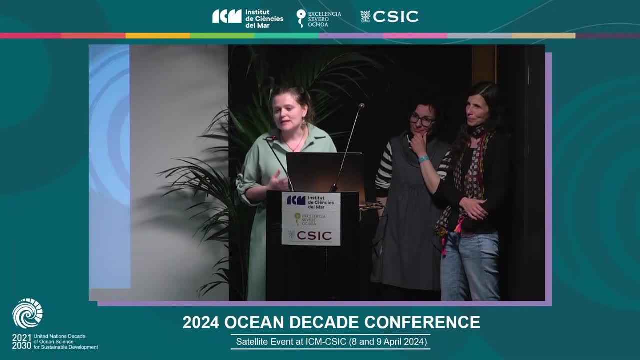 on the social media channels of the ECOPE Programme and at the next big conference, which is the second Euron Ocean Decade Regional Conference, in conjunction with the Westpac International Marine Science Conference, which will happen just in two weeks in Bangkok, Thailand. 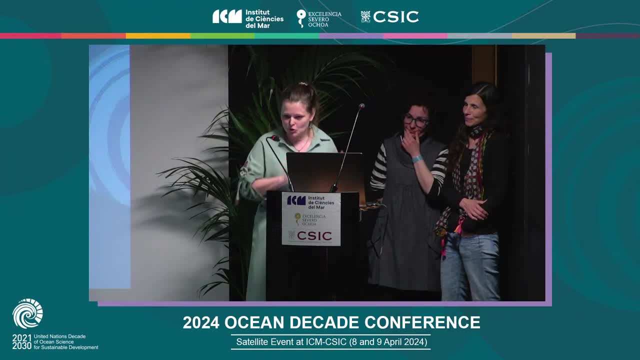 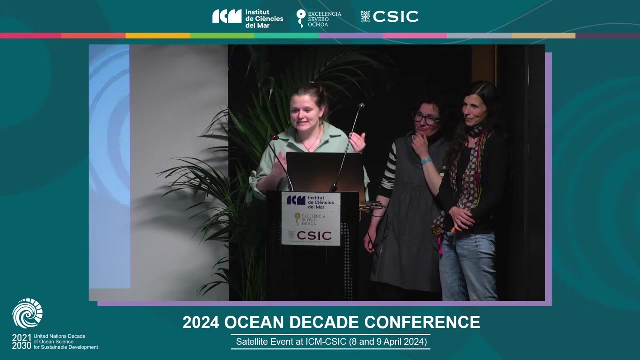 So we hope that this online space and this in-person space will inspire people to connect, to learn from each other and really to create some more greater ocean literacy approaches and initiatives. So I would like to share now the teaser video that we've created on all these amazing initiatives. 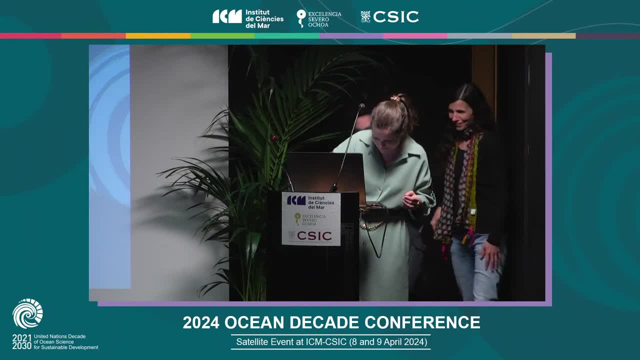 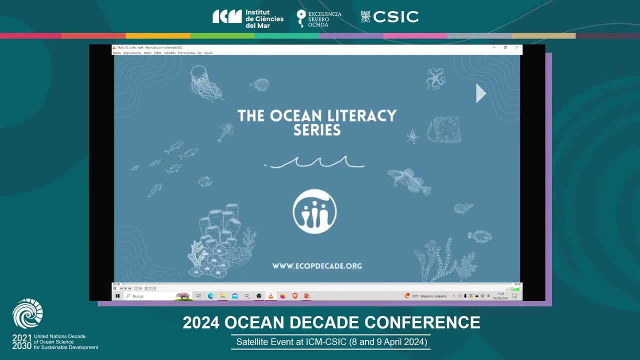 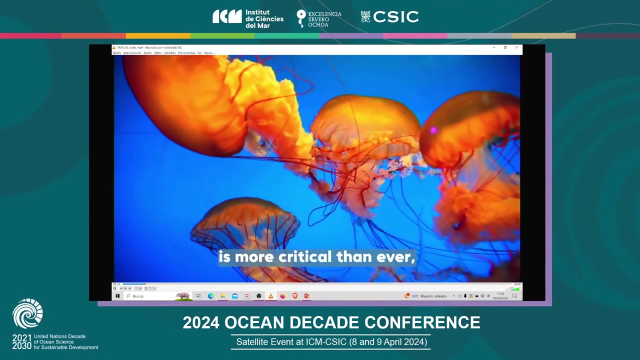 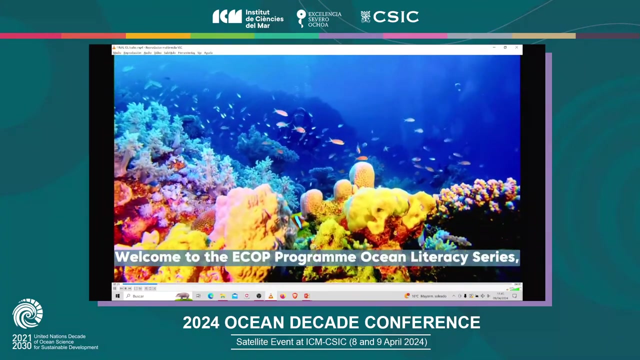 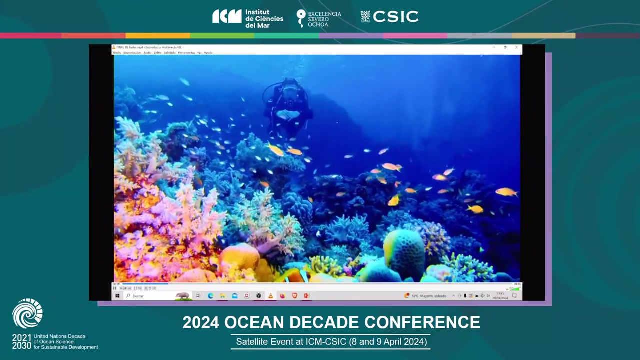 So let's watch it together. In a world where the ocean itself is more critical than ever, a global movement is underway. Welcome to the ECOPE Programme Ocean Literacy Series, an initiative dedicated to inspire change in humanity's relationship with the ocean. 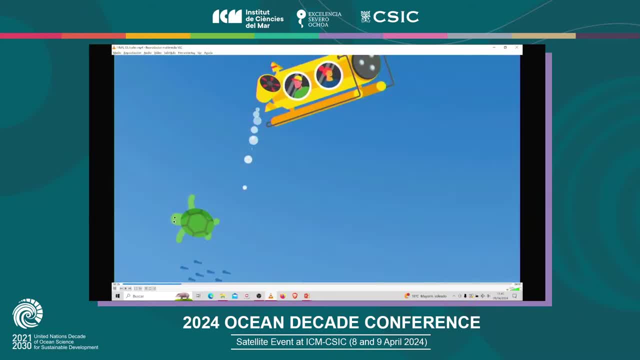 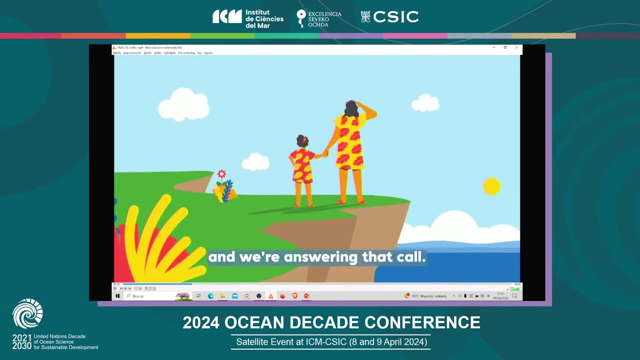 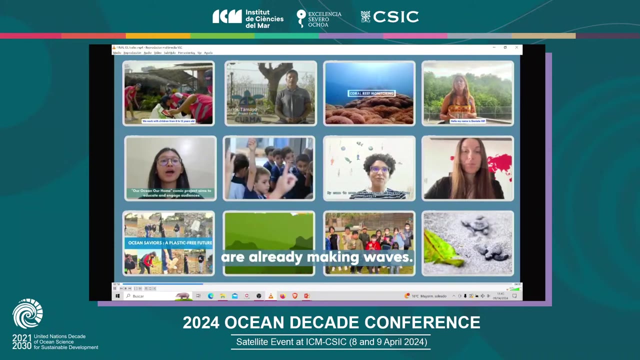 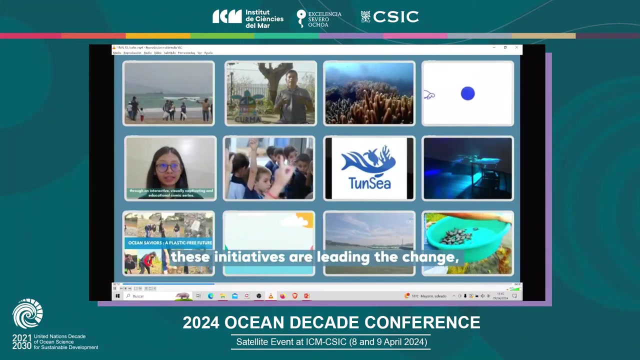 Challenge 10 of the UN Ocean Decade calls for transformative action And we are answering that call. Across the globe, innovative projects are already making waves. From teaching programmes to community engagement. these initiatives are leading the change, showcasing the power of knowledge in action. 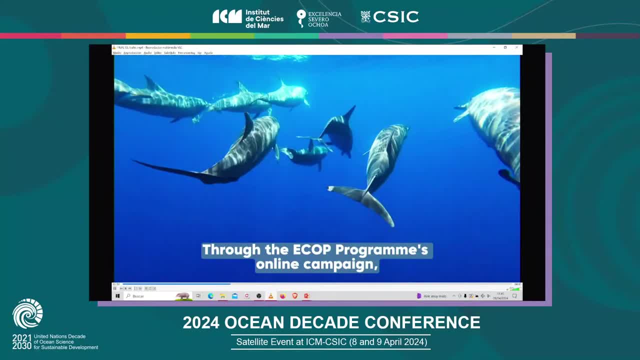 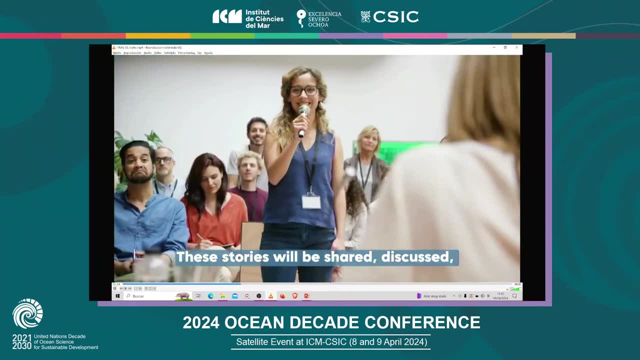 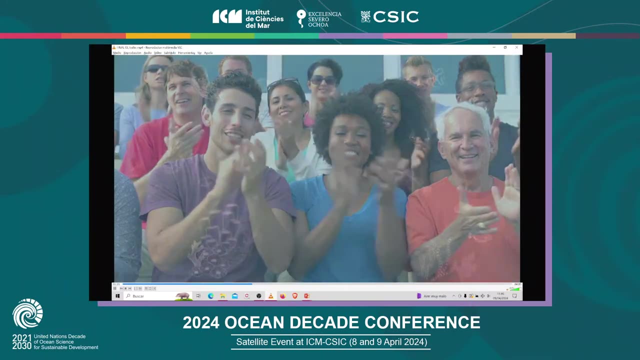 Through the ECOPE Programme's online campaign, we are gathering stories from every corner of the Earth. These stories will be shared, discussed and celebrated at our interactive panel event. Here are just a few of our favourite projects that are part of the series. 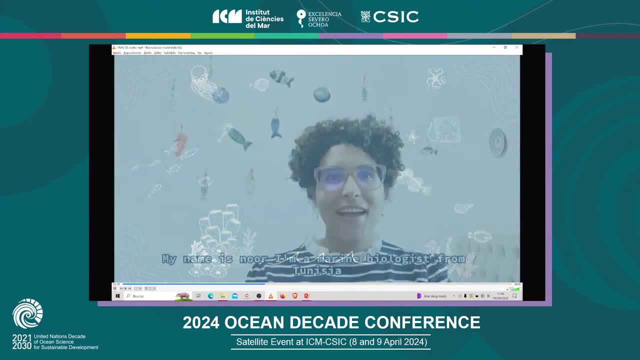 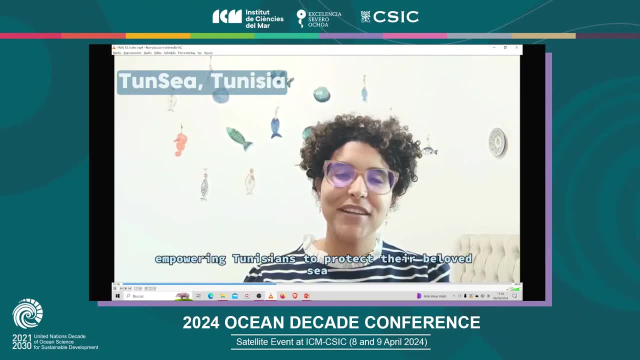 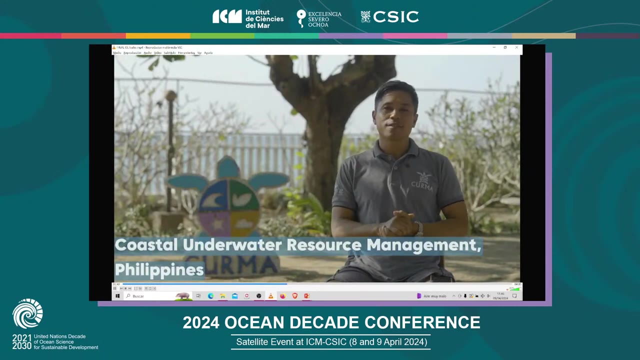 highlighted for their outstanding innovation. I'm a marine biologist from Tunisia and I am the co-founder of TuneSea, a citizen science platform empowering Tunisians to protect their beloved sea. We managed to turn former poachers into the protectors of sea turtles. 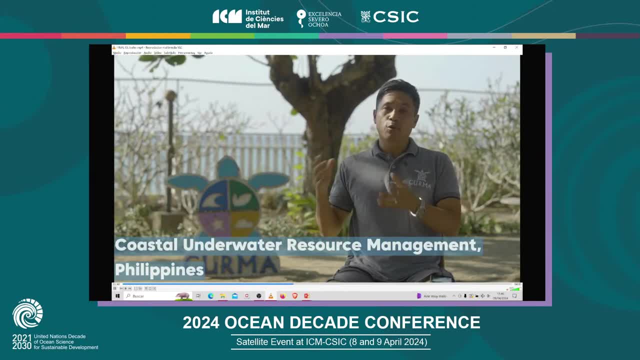 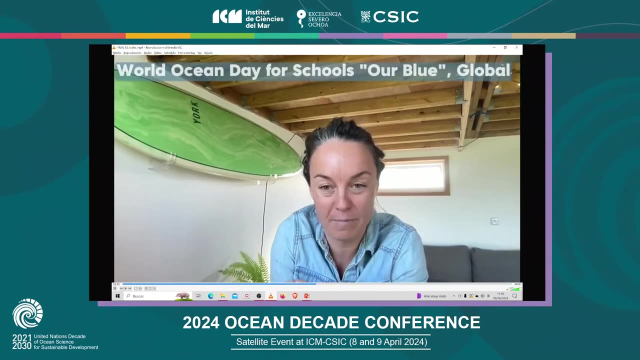 So through educating them and showing them the importance of sea turtles, especially to their livelihood, and also providing livelihood support for them. So nowadays, 98% of the sea turtle patrollers are former poachers. So we ended up with these beautiful memory maps. 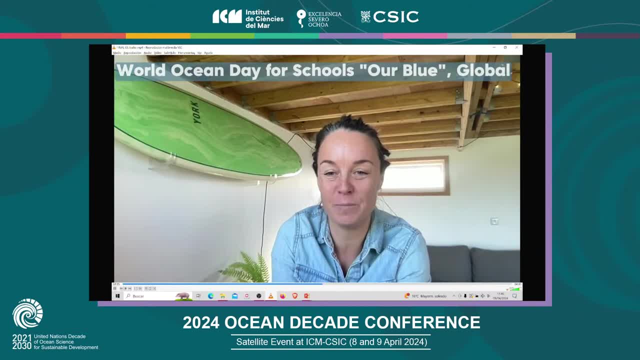 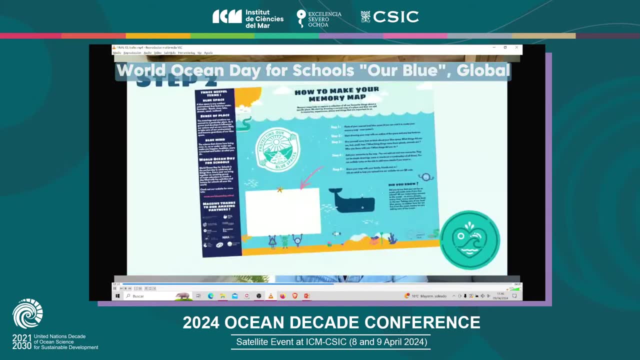 from kids all around the world, showcasing their connection to their local blue space, And I think it's vital because research shows that increased sense of place positively influences environmental behaviour and collective action, And that's what we really want in kids to start doing. 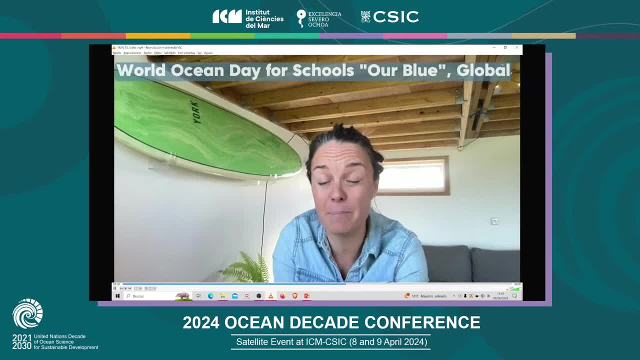 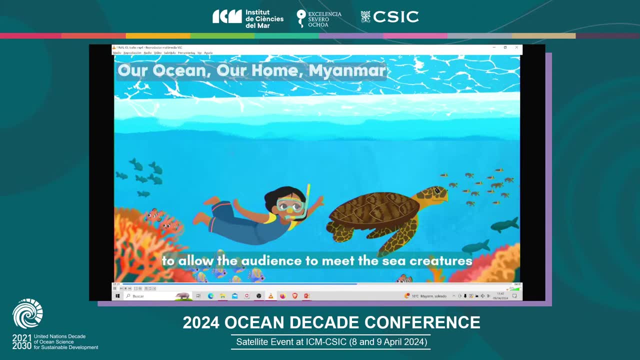 is going back to their blue spaces again and again and recognising that that's their personal connection to the ocean. Our aim for this comic series has been to allow the audience to meet the sea creatures through the zen a child's eyes and learn of fun facts and threats. 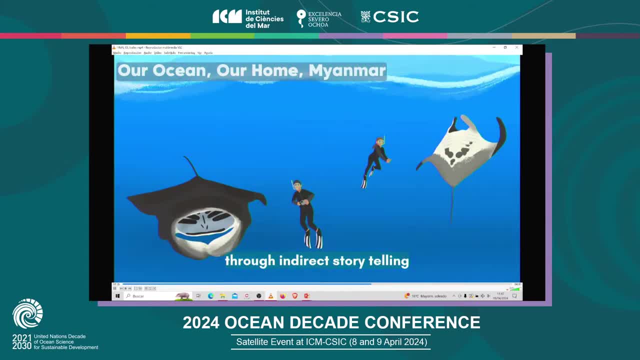 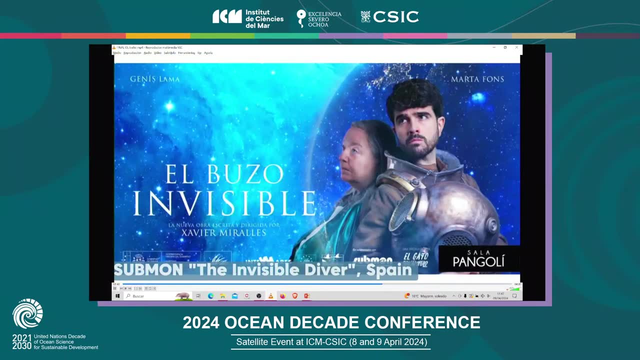 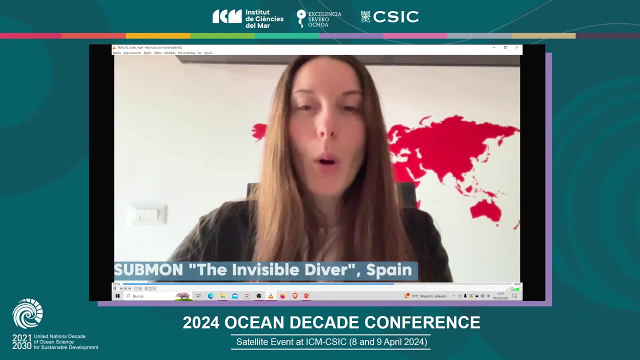 the animals face through indirect storytelling from the animal's point of view. Our ocean literacy initiative is a theatre play, and it's called Invisible Diver. So the integration of scientific information in a captivating way was probably the most relevant challenge, which was overcome thanks to the strong collaboration. 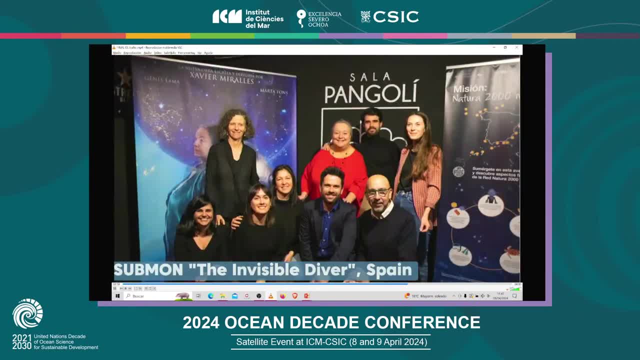 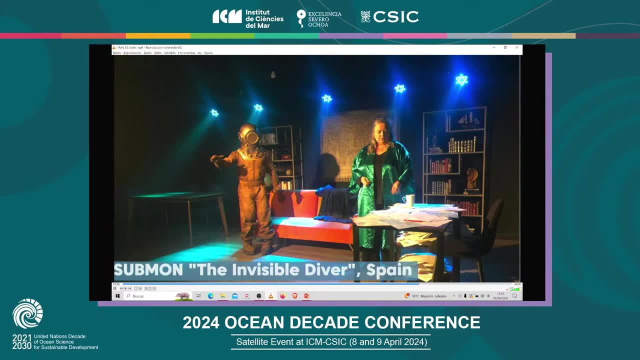 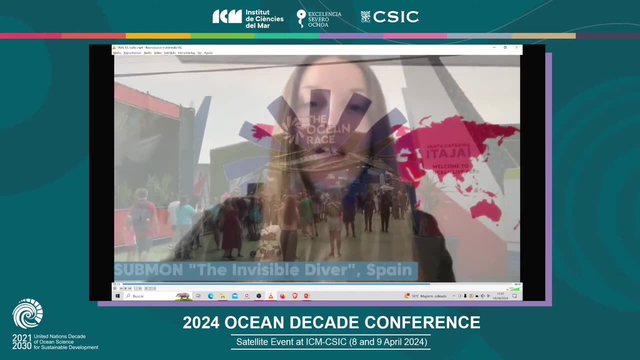 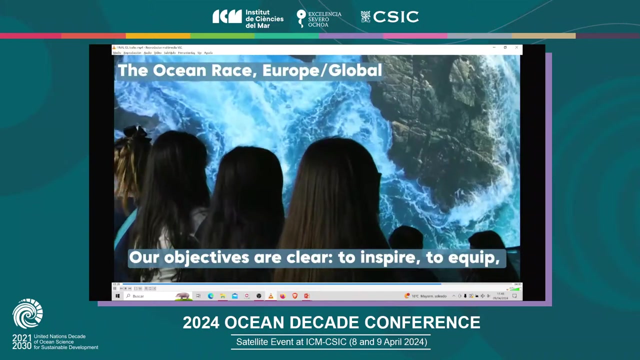 between the director and scriptwriter, Xavier Miralles, and the team of scientists at Submon, And the results proved to be effective, with science meeting art to raise awareness while leveraging on emotion. Our objectives are clear: to inspire, to equip, to connect and to advance. 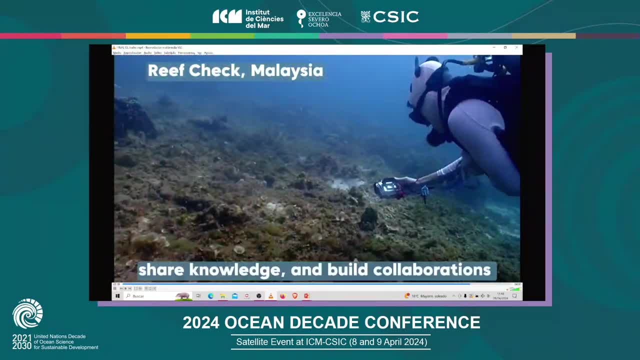 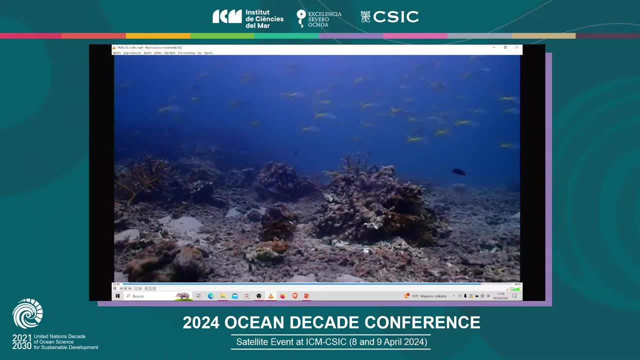 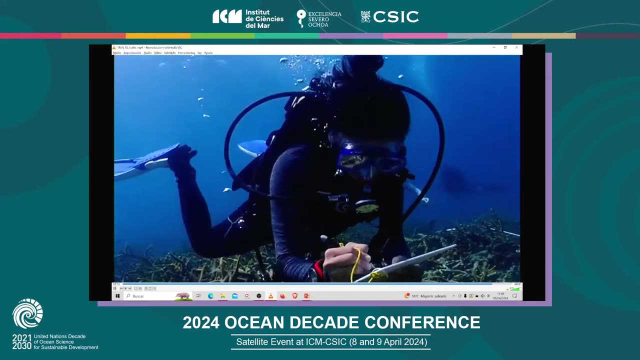 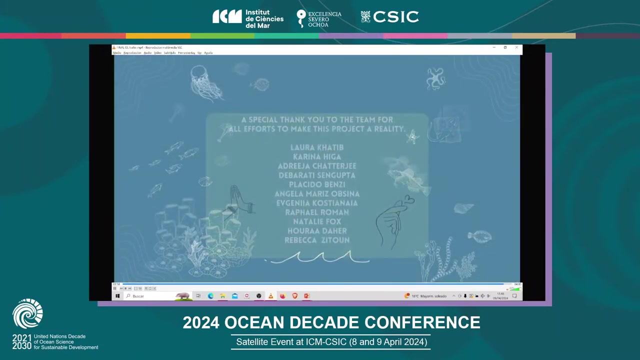 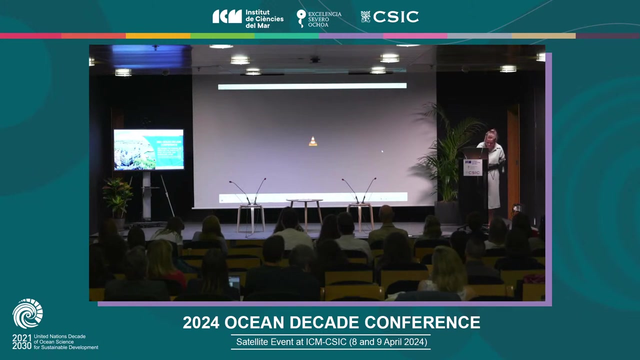 Together, we'll explore new methods, share knowledge and build collaboration that will shape the future of ocean literacy. Join us on this journey to create a more sustainable ocean. Together, we can make a difference. Thank you all. Maria Vittoria, over to you. 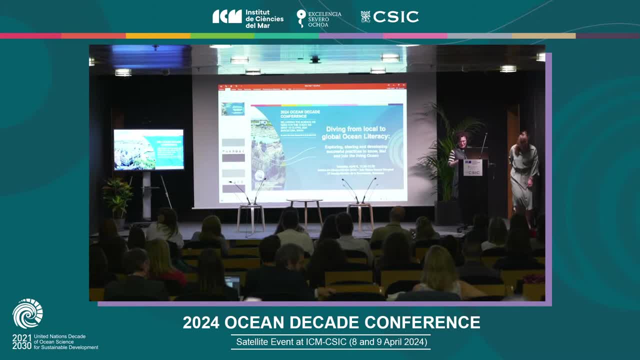 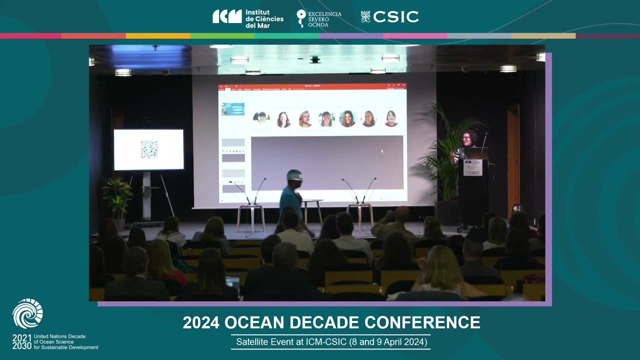 Thank you very much, Evgenia. So now we will start with the first panel. Sorry, If you, please thank you. So it's The first panel, is It will be about It's removing barriers in addressing ocean literacy globally. 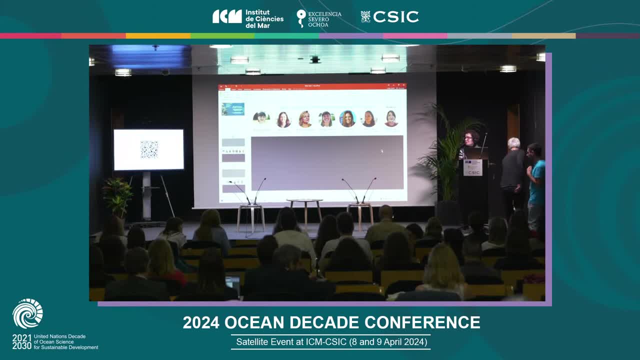 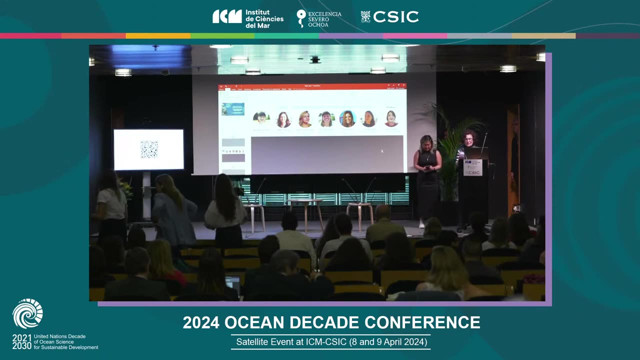 The moderator is Carina Higa, from the ECO program, And we have six wonderful panelists for this panel: Alicia Perez Porro from the- Forgive my pronunciation- Centro de Investigacion Ecologica y Aplicaciones Forestales. Patricia Puig from Oceanogami. 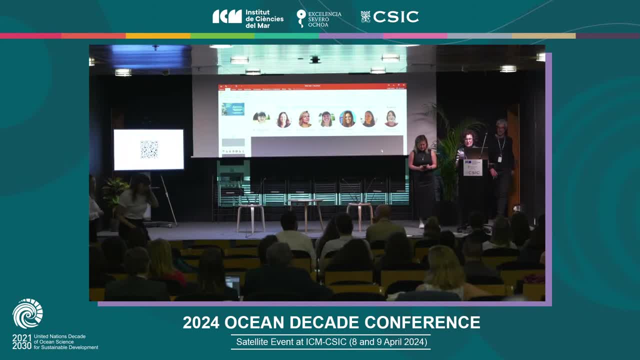 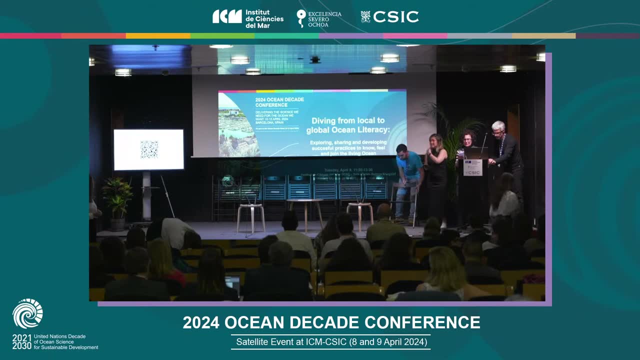 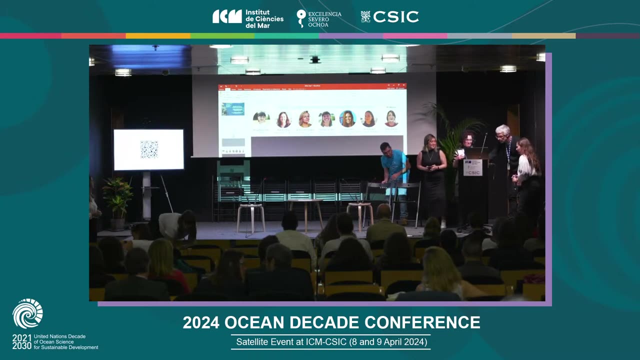 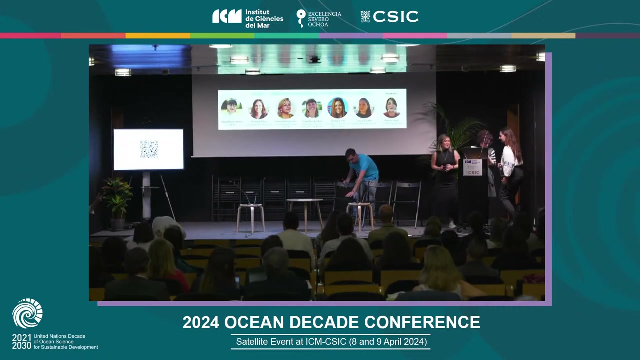 Antonella Vassallo from the International Ocean Institute, Yolanda Sanchez from Relato and Ocean Grants Program, Daniela Hill from the Fundacion Amiguitos del Oceano And Laura Katip from Guardians of the Blue. So welcome everyone. 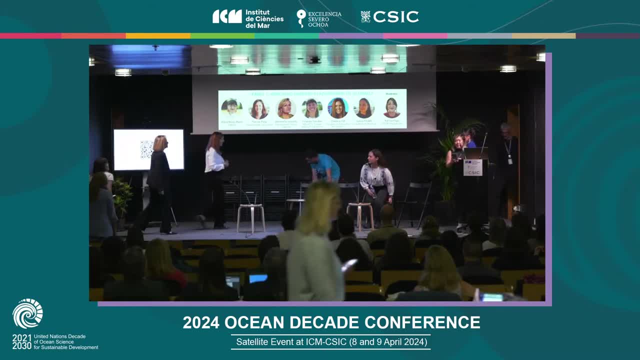 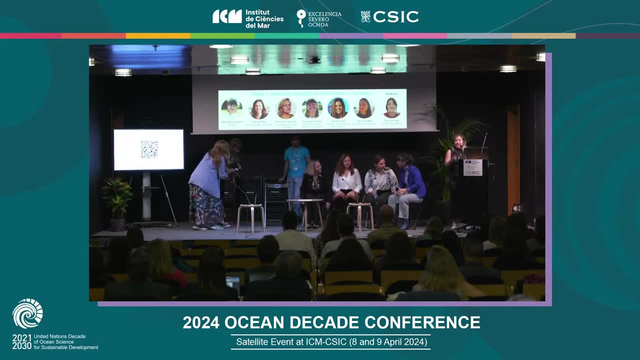 to our panel discussion on removing barriers for addressing ocean literacy globally And the unique approach taken by various initiatives to address challenges in this field. Today, we have a diverse group of panelists who will share their insights and experience on how innovative approaches, such as citizen-side projects, 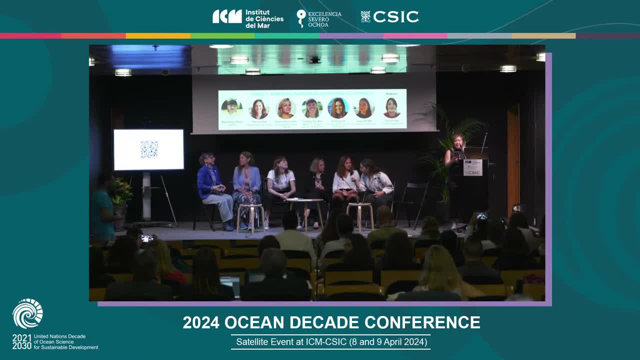 and local community engagement efforts can bridge gaps in knowledge and empower individuals to actively participate in ocean conservation. Thank you, So today let's kick off our discussion, where each panelist will answer a specific question about their project. So we have a limited time, but each one is going to answer one question. 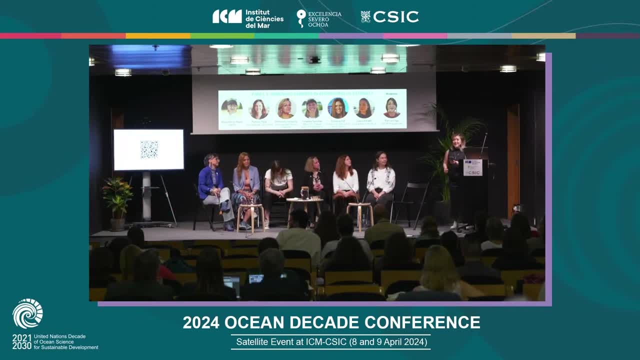 and then I will open questions for the audience, Because I guess you guys will have so many questions. To start off, I would like to ask Yolanda: Yolanda, Could you please share about the Ocean Grants Program, how they address and they support? 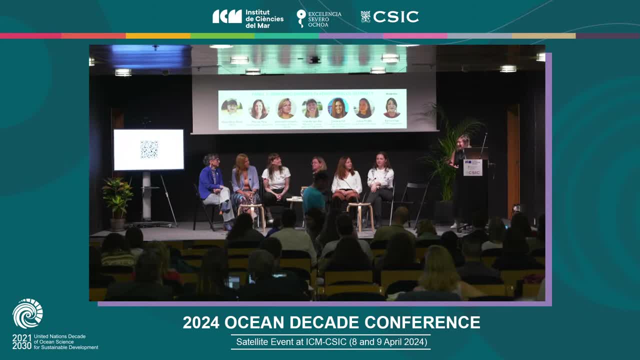 Relatos network: okay, to fund challenges commonly faced by marine education initiatives ensuring sustainability and longevity in the efforts to improve ocean literacy. Okay, Thank you so much. This is a. we just have three minutes, so it's quite a lot. 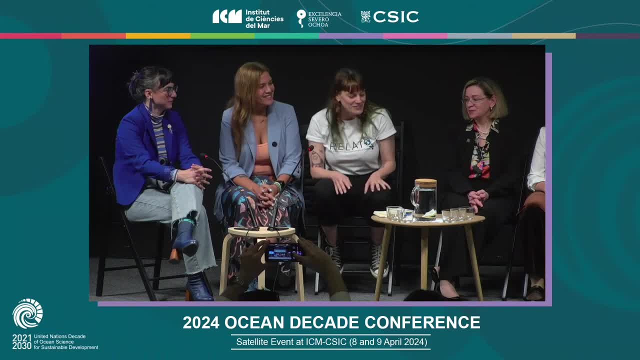 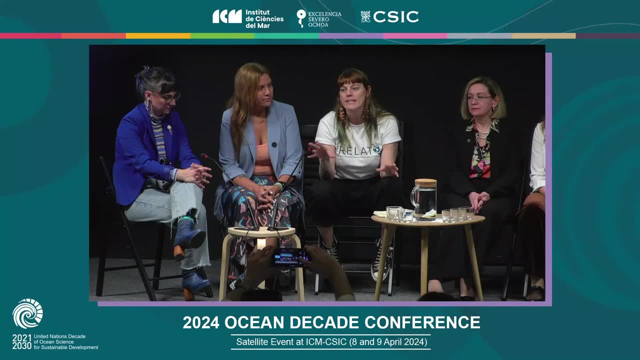 Thank you. Quite of an elevator pitch thing that I don't like at all. But let's try to first of all starting to doing the difference between what is the Ocean Grants Program and what is Relatos. So Relatos is the Latin American Marine Educators Network. 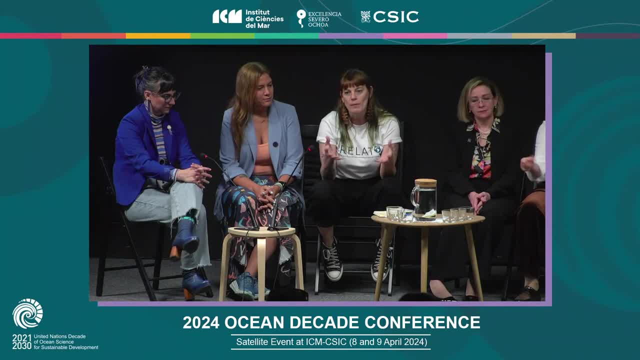 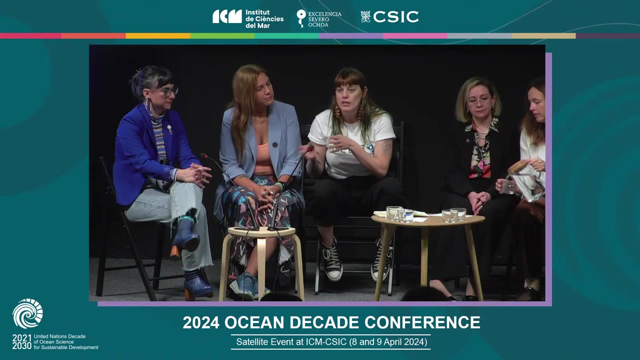 That it was created. thinking about how to empower communities who is doing ocean literacy in Latin America to support them in make more visible the results that they have doing ocean literacy. So thinking about the and the Ocean Grants Program is a UK government program to fund communities in the developing countries. 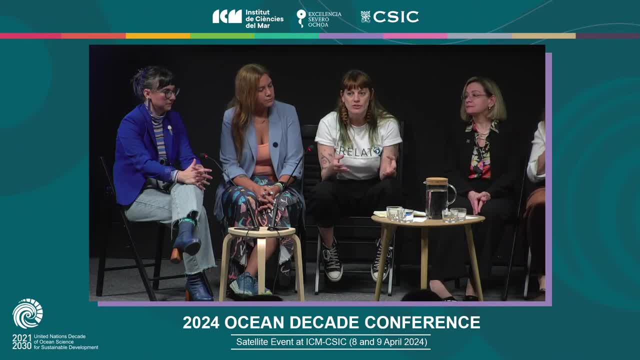 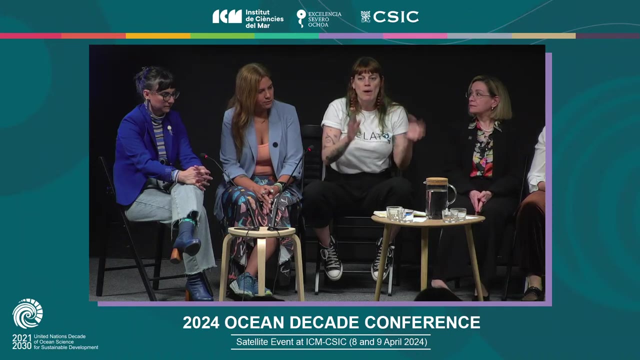 to implement projects in conservation and poverty reduction. So thinking about how to cross the barrier, about funding, I have this very amazing two points of view about. Firstly, let's think about Relatos. So let's think about how to empower the community, trying to connect them. 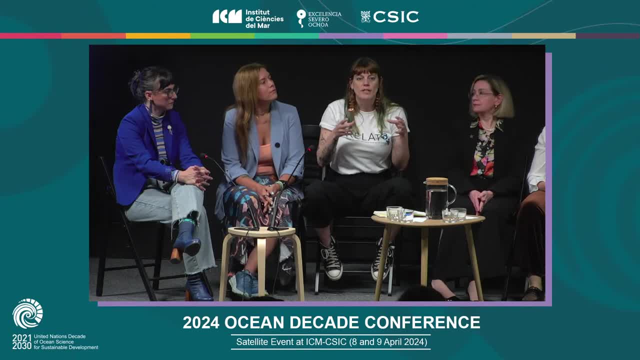 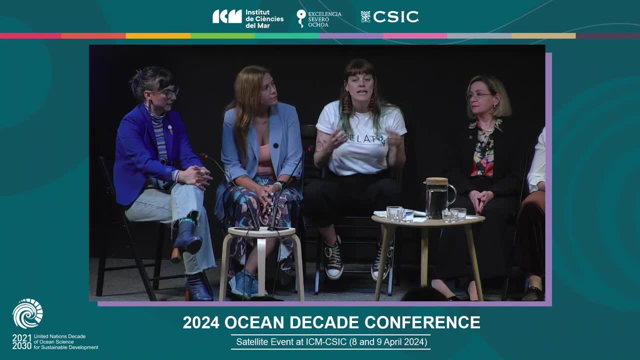 what Relatos does: connect them, trying to understand what barriers they have, what kind of challenge they face, what kind of support they can give each other, And that kind of thing is sharing all together. We have 1,000 members in the Relatos network now. 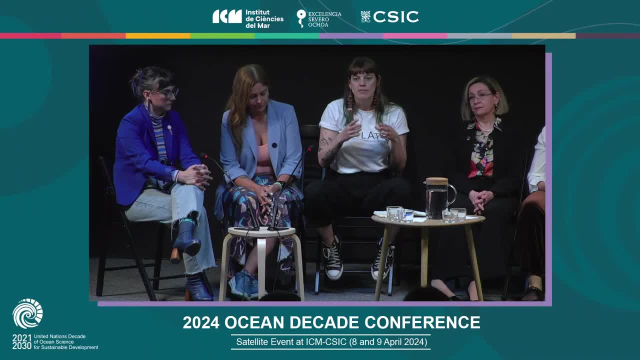 So having this time for sharing is a time for empower ourselves, because we realize that we have already a lot of experience to improve. how are we doing ocean literacy in Latin America? So that is so important: to convince funders about why we have to fund. 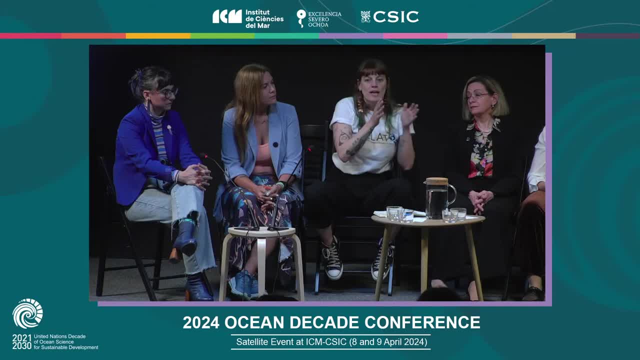 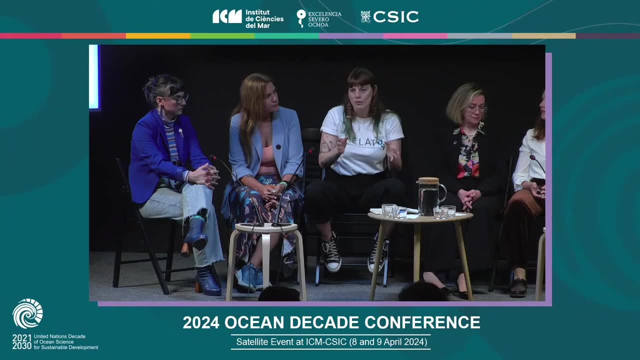 not only just give a talk on the community, but how to analyze the context we are going to work with, how to analyze the program we want to design, how to test it, how to implement, how to evaluate and how much time is it? 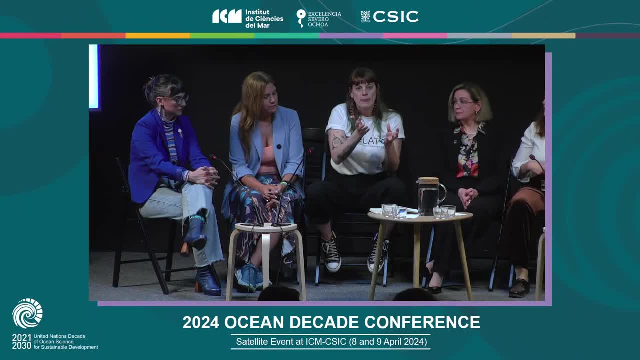 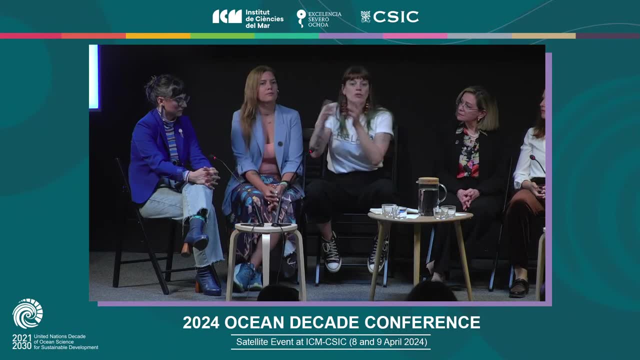 and how much money is it? So, having all this idea and power inside the community, inside the ocean literacy community, you can go to the grants opportunity as the ocean grants opportunity. So, going to the other side, I think that this new program in ocean grants 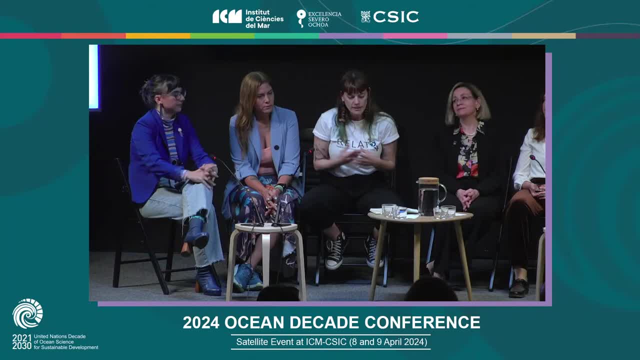 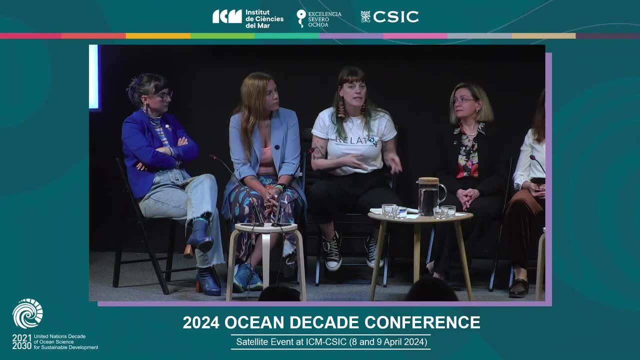 and conservation funding. it's very thinking about how to support communities to get fund for that kind of project. So it's not focused only in ocean literacy but it's focused on how to empower communities. So absolutely understanding how much ocean literacy is important on that. 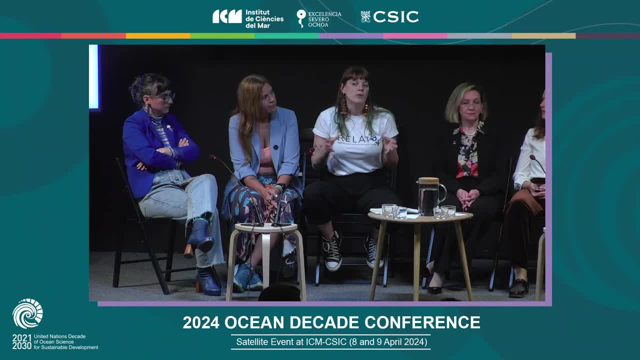 I think that some of the most important ideas that the ocean grant program has is like we are developing a lot of strategies to support communities to apply for the grant- like having webinars, help desk or all those ideas- but also thinking about how to set the rules to make the things easier. 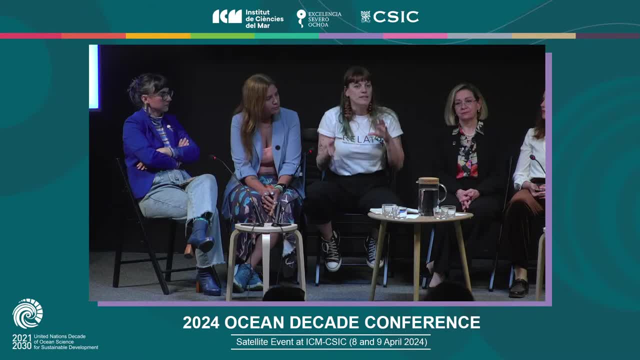 for the people who want to apply for that kind of grants. So I think that just having both points of view, we can understand a little bit better how to try to face these barriers in getting funding. It's not easy. It's the topic that everybody will talk in all the sessions. 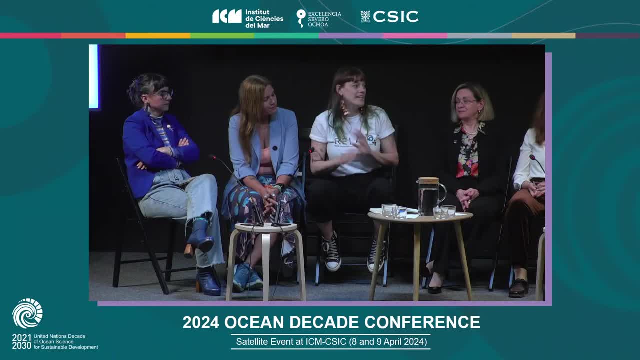 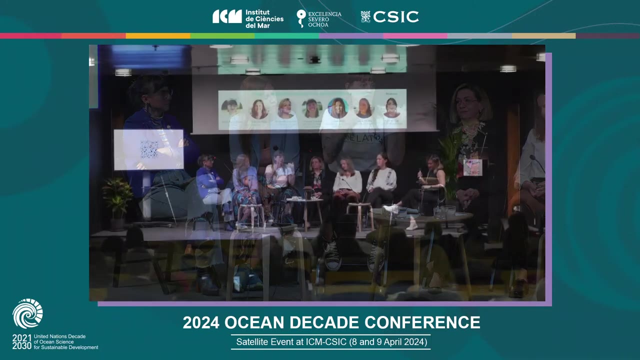 that we still have the problem of funding everywhere in all the topics. But let's try to understand how to strengthen organizations so they can be more powerful asking for the money, and how the organizations can also try to have and share the vision from the communities. to understand how to make easier. 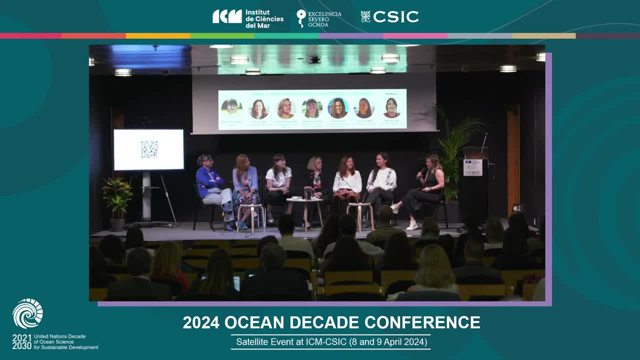 these applications in funding. Thank you, Thank you very much. So can you see the QR code over there? So we prepared for each panelist. we prepared like a story, So you can access each story of each project through the QR code. 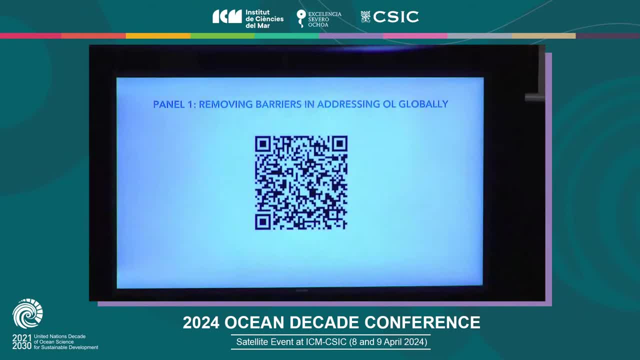 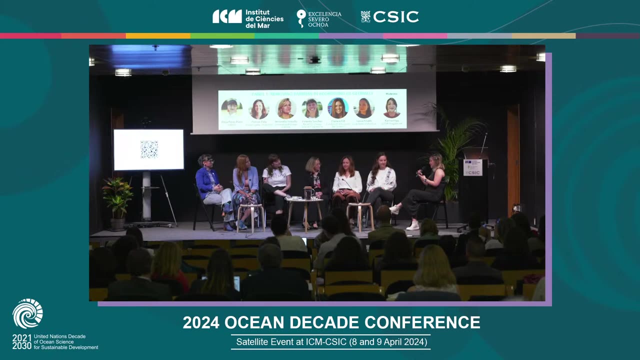 So yeah, if you're curious about each project, so yeah, please check it out. So for the next panelist, I would like to ask: Lara, Guardians of the Blue has been doing remarkable work in Lebanon in addressing ocean literacy challenges. Can you share how your organizations tackle? 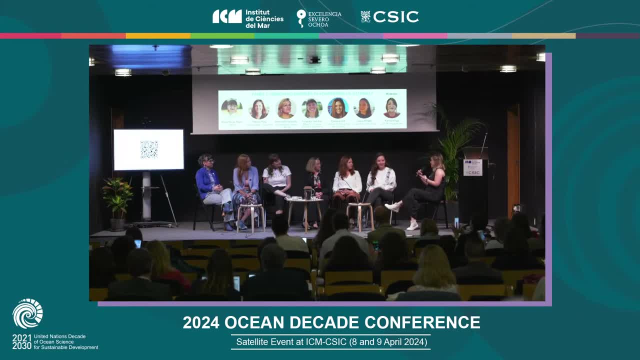 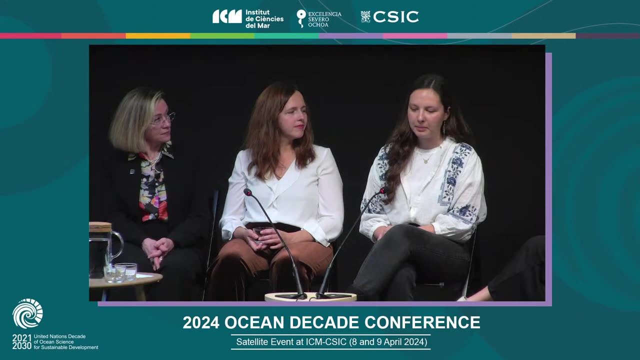 the low ocean literacy rates. Thank you, So yeah, we're facing a lot of barriers in addressing ocean literacy in Lebanon. Obviously, the current political-economical crisis, the constant instability and the lack of public governance and infrastructures are all having an impact on the country's capacities. 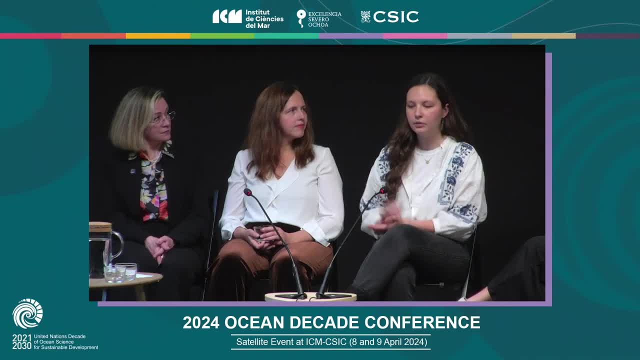 in terms of marine research and marine education, formal and non-formal. So when we created Guardians of the Blue, it was out of passion and out of necessity And since the beginning- it's been three years and a half now- we've been partnering with Xiphias Diving. 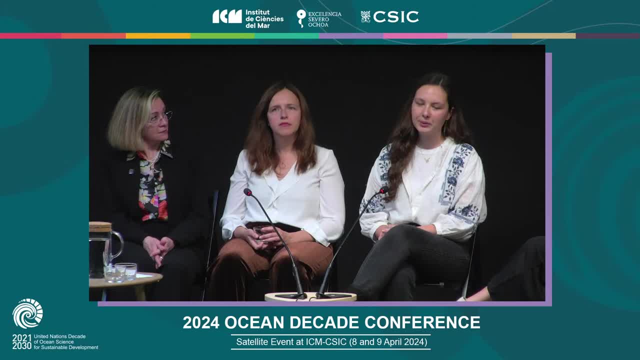 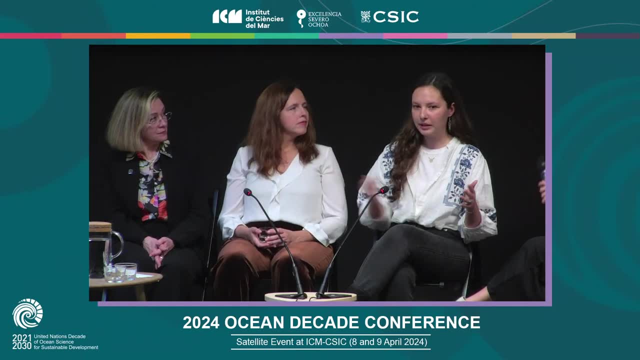 the only scuba diving club in Byblos, And so we started with what we had, which was 10 years of underwater footage taken by the club around the coast of Byblos, And this was really valuable because it allowed us to create a kind of baseline. 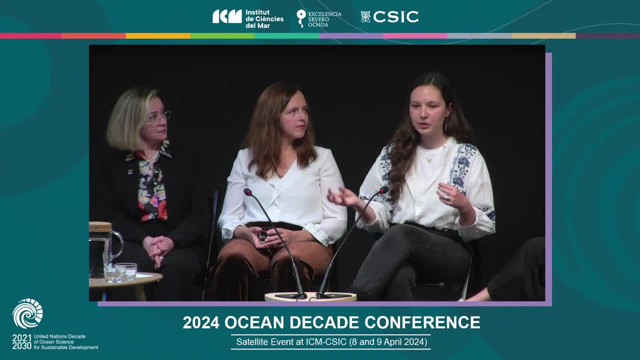 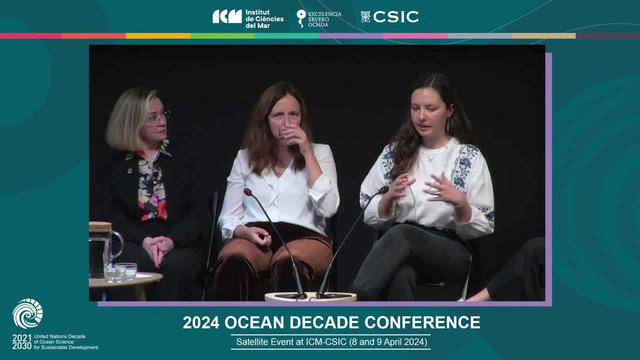 to know what is in our coast, which species, and to see how it changed over the past 10 years. So we compiled this information with the scientific research that has been done in the rest of the country, and that's how we started. 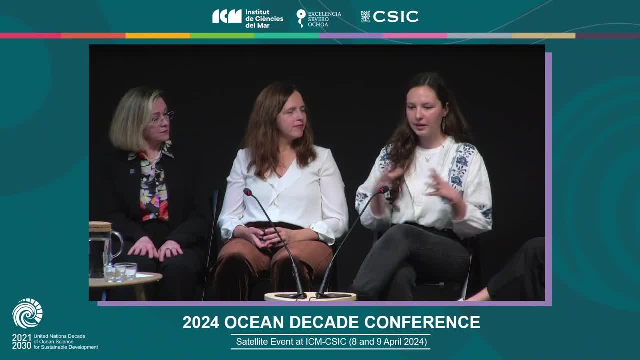 So we created educational posters and a big marine species poster for the club to educate and train divers about their sea so they can become kind of ambassadors and they raise awareness among their peers. And we're also using all of that data and footage to create posts on social media and on our website. 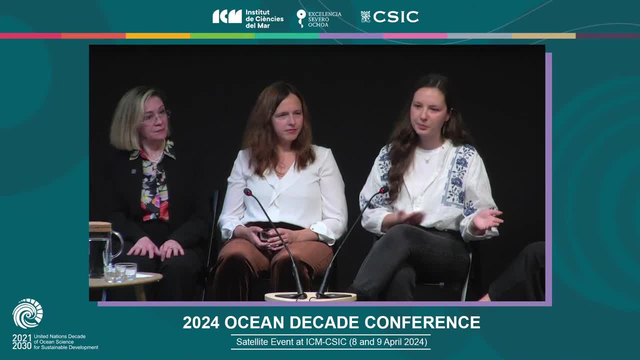 So we're sharing information on the different marine species we have in Lebanon and we're also making awareness campaigns about certain topics- So last summer it was about sharks- And we're also sharing information about general marine science. So all of our content is available in English and Arabic. 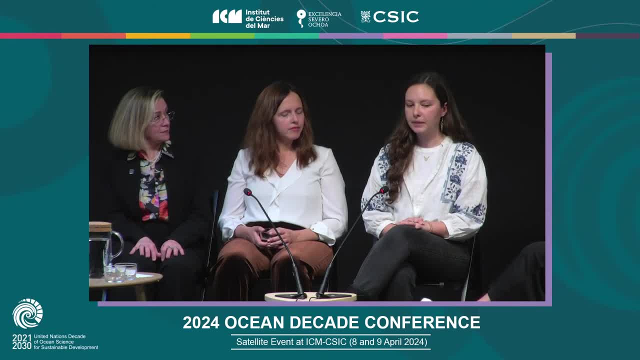 and sometimes also in French, And so far we reached around 20,000 people And we always get very positive feedback, because it's quite rare to get underwater footage of the Lebanese coast, And so there's so many people in Lebanon that think that the coast is empty and dead. 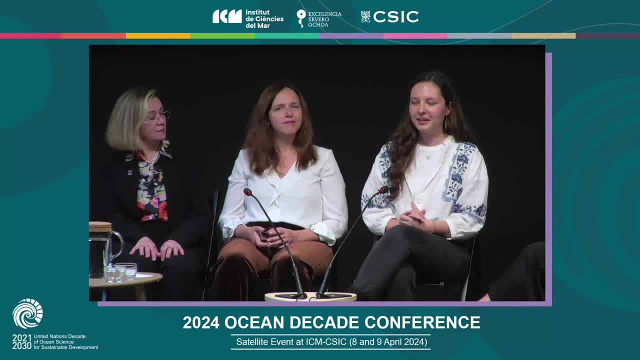 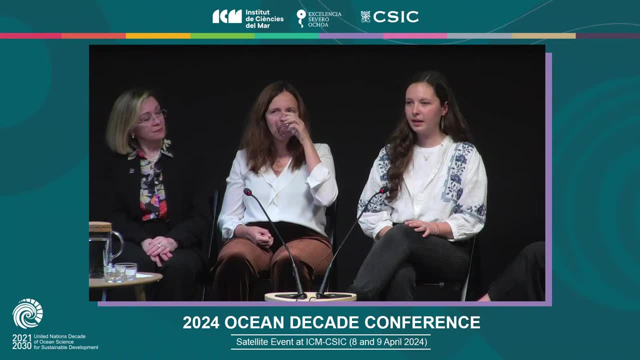 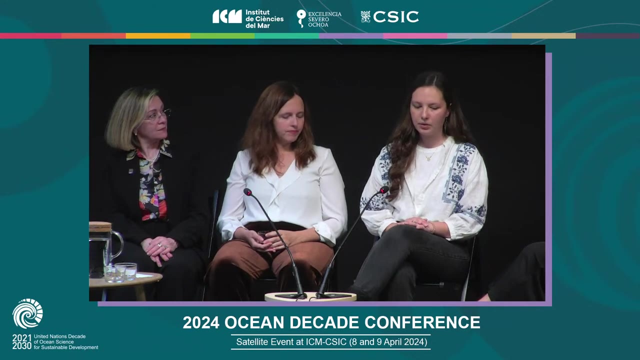 because they never see what we see when we dive. So this is kind of our way of removing this visual barrier, together with the knowledge barrier, And we also work with divers and the local community of fishermen to organize underwater cleanups, And so we use these times to talk about 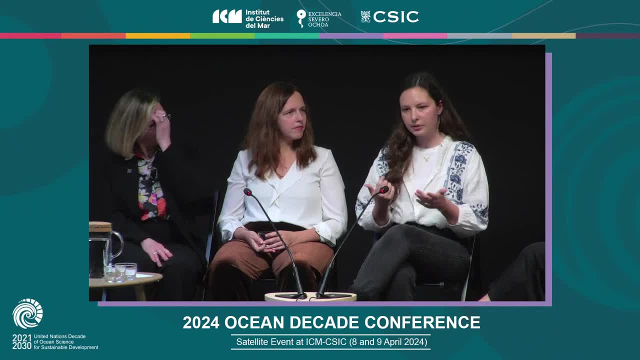 the impacts of marine pollution and the importance of keeping the sea clean, And we're also working on raising awareness about the lionfish invasion. So we're trying to democratize the consumption of lionfish and its hunting, and we're also making lionfish jewelry. 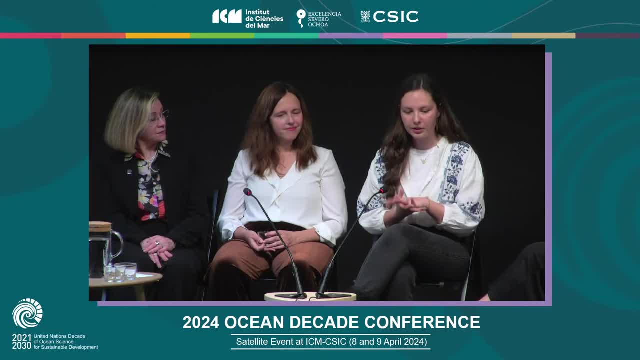 And so, finally, one of our most recent projects is working with the municipality of Byblos, in collaboration with the municipality of Saint-Jean-Cap-Ferrat, In the south of France, And so we're going to organize workshops both in the sea and in the classroom. 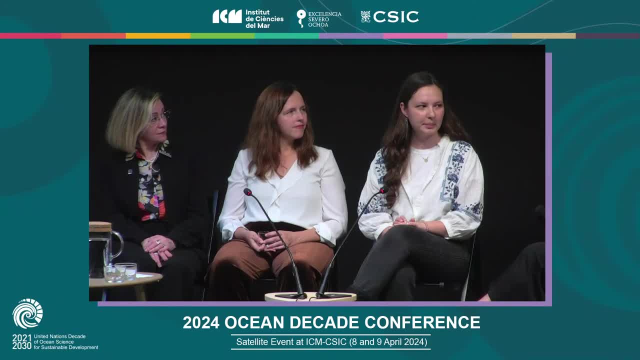 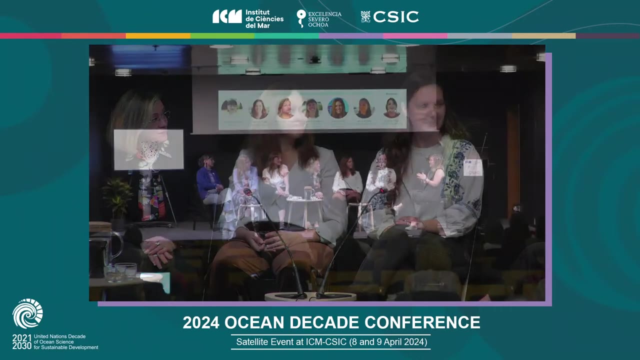 with the use of both cities, And our long-term goal is kind of to get funding to create a sea school in Byblos and also for the future marine protected area of Byblos, and to produce a marine documentary series about the sea in Lebanon. 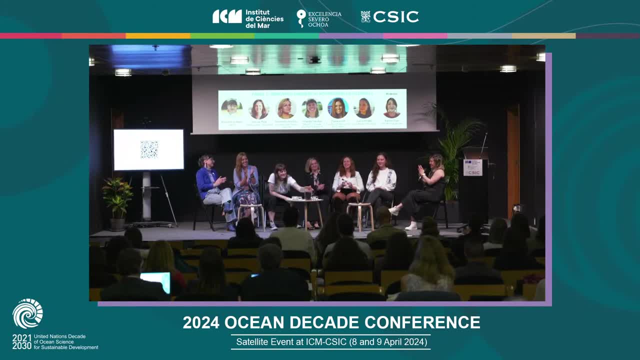 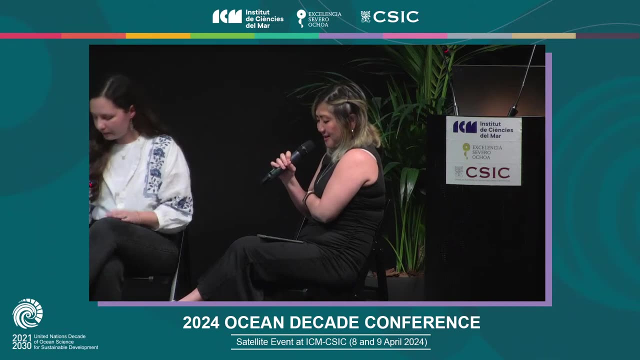 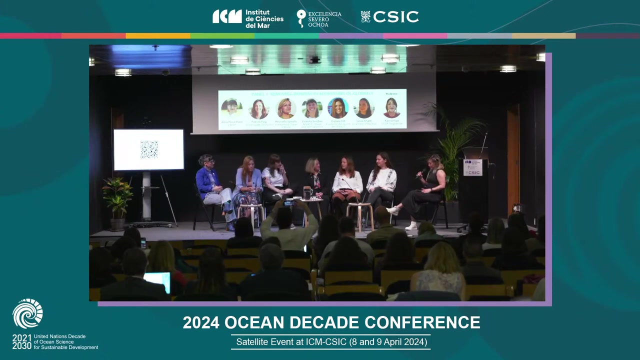 Thank you. Thank you for sharing your story with us. Now I would like to move on to Antonella. Can you explain more about how the IOI Ocean Academy emphasized on ocean knowledge that, related to local culture, helps people in neglected communities feel more connected with the ocean. 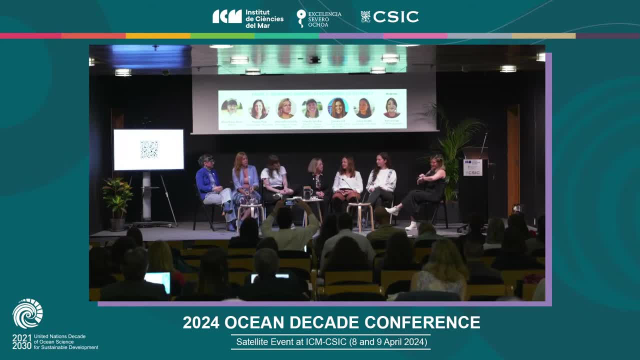 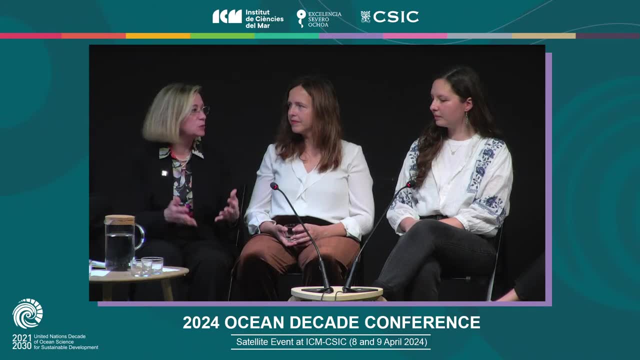 Thank you very much. So I'm from the International Ocean Institute And, as well as capacity development and training for ECOPS, We recently devised an ocean literacy level, if you wish, program called the IOI Ocean Academy, And this idea came up as first of all. 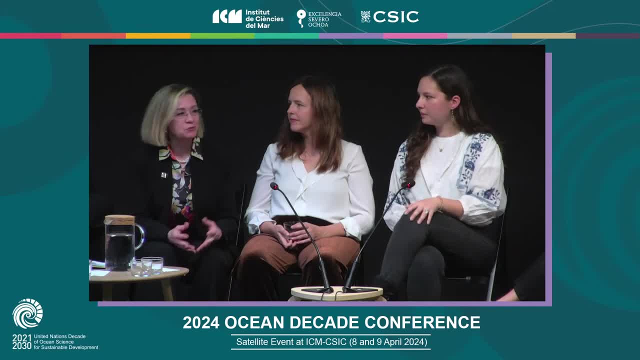 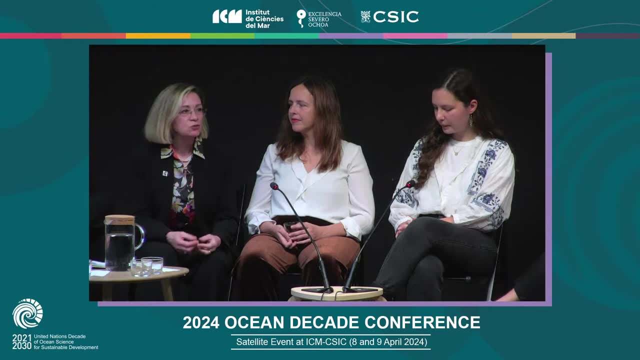 it was a 50th anniversary program of the IOI. So in order to celebrate and emphasize how far we had gotten and to continue working with those people who had graduated from the IOI training over the previous five decades, the IOI Ocean Academy was created as a way to 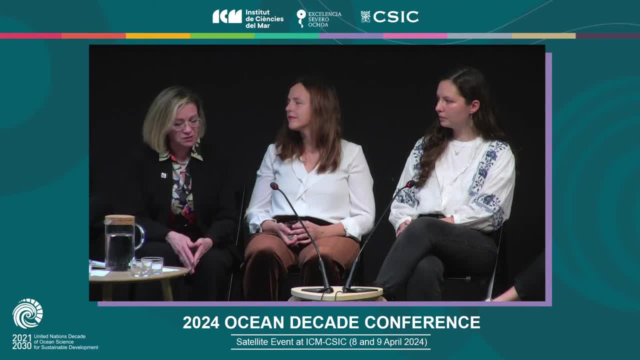 for even the alumni of the IOI to give back to their communities. And one thing we noticed is that very often- and it's a barrier that Laura mentioned- that there is material out there, It's not necessarily available in those languages which the local communities 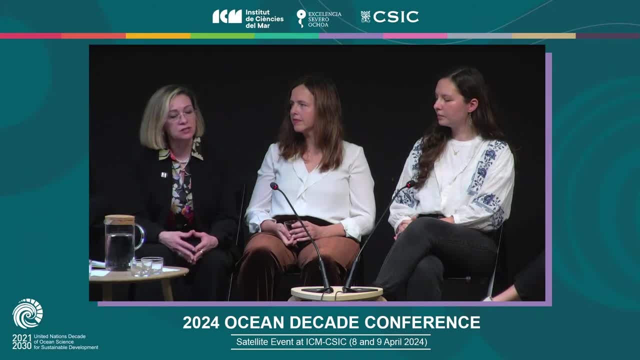 maybe some of them in vulnerable environments which are at the forefront of climate and ocean threats. There is no material out there which people in these communities can access, So we created the academy which removes barriers to ocean knowledge, which are created by funding. 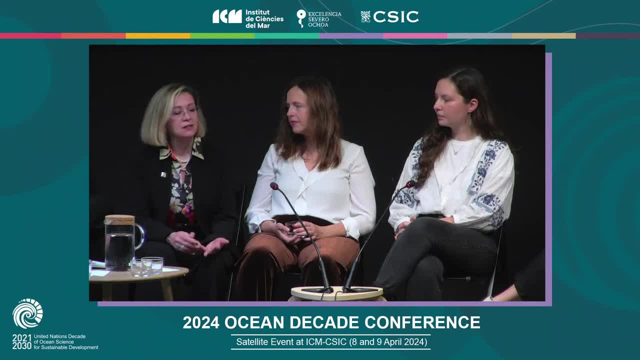 So it's free for all our audience to attend. It's free by language, So the Ocean Academy is offered in, I believe, 17 different languages and growing. So, in fact, shout out to our Ocean Academy director from Morocco, who's here. 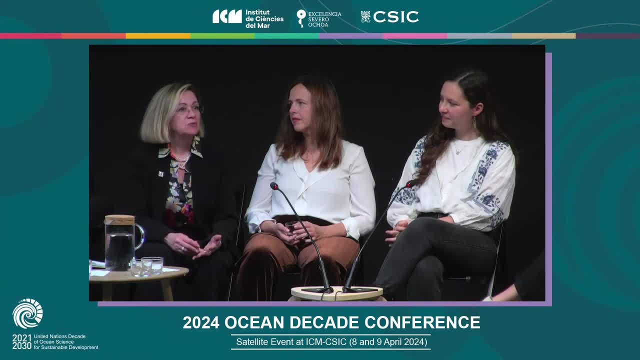 And they will be offering, for example, locally targeted 20-hour online modules for people from Francophone African countries at an ocean literacy level, which I think we like to say that it doesn't discriminate for or against anyone in the generational age range. 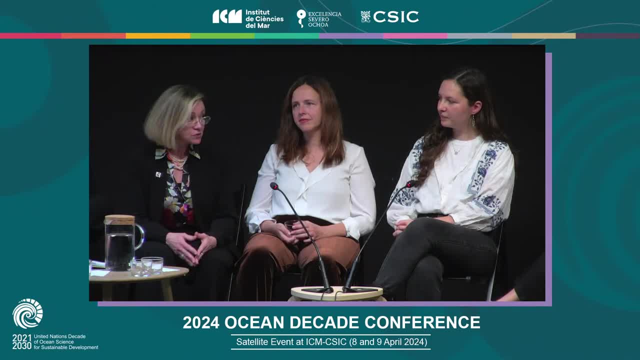 And literally we always say: if you're interested and you have a smartphone and you have a Wi-Fi connection, you can join, You can join and you can learn. I think one of the things we really like about these Ocean Academy modules. 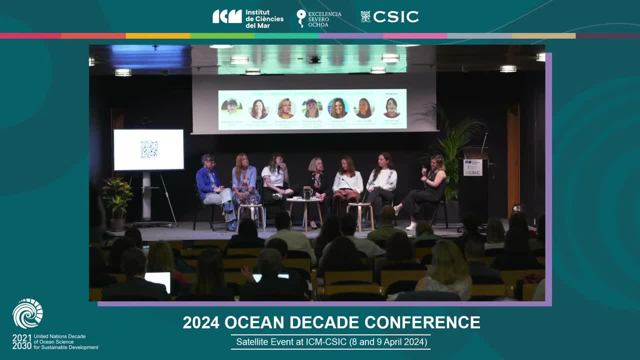 which are offered, you know, in. I think we'll have about 40 this year, this year alone, in many different countries all over the world. what we like about that is that they are a forum not only for learning to proceed from local experts. 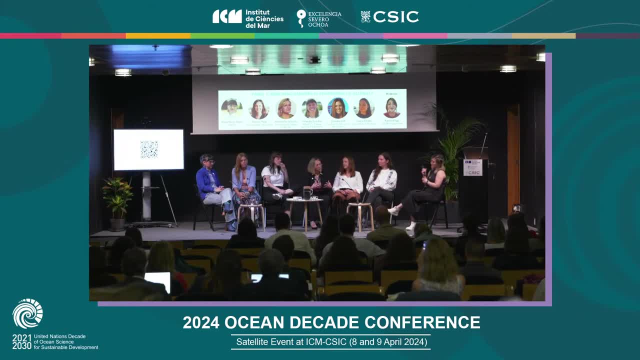 about local situations, but it's also a forum where they can, where people can ask their questions. It's 10 seconds, People can ask their questions and we notice as well that these questions, this involvement, empowers them to go and be really proactive about. 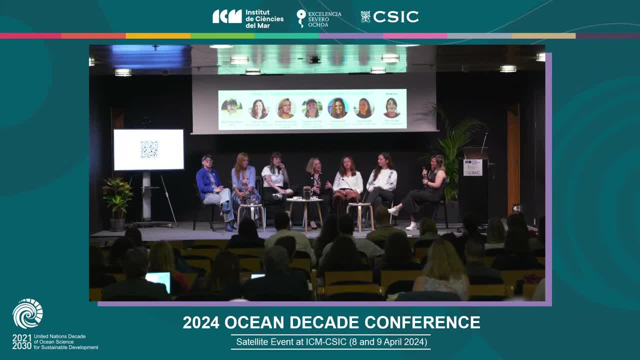 and bring positive change to their community. So I think it's a project which really goes deep into the heart of local communities, with issues that interest them and that they can be empowered to do something about. Okay, amazing, yeah, Yeah, we need to have this access. 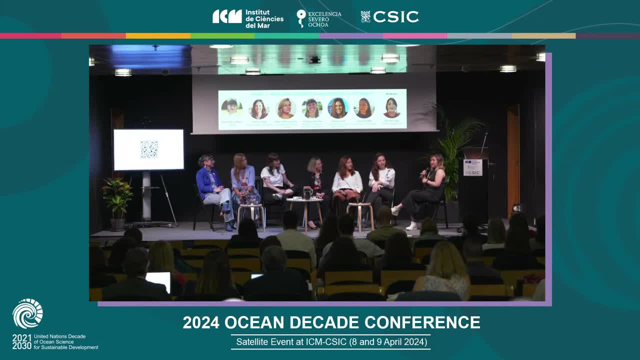 to different languages, but also not in different idioms, but different languages to talk with, for example, private sector. So yeah, and I would like to ask to Patricia about her project with private sector, For example Oceanogami. 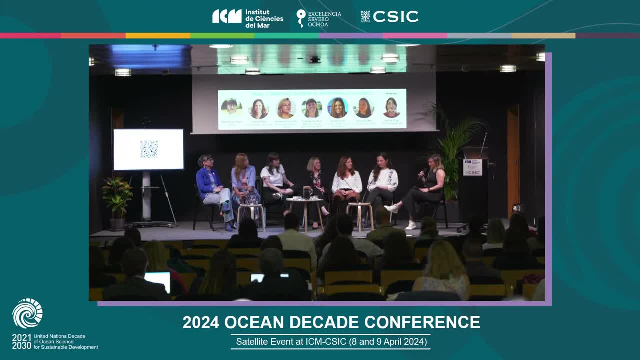 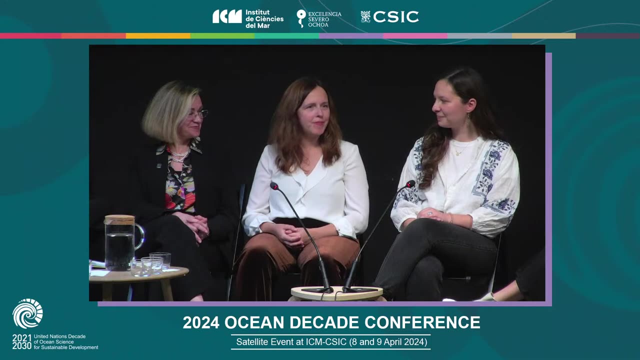 how does Oceanogami approach of conducting team building workshops contribute to overcome the challenges of engaged private sector in marine conservation efforts? Okay, thank you very much for the invitation and it is great to share our experience engaging the different stakeholders for ocean literacy. 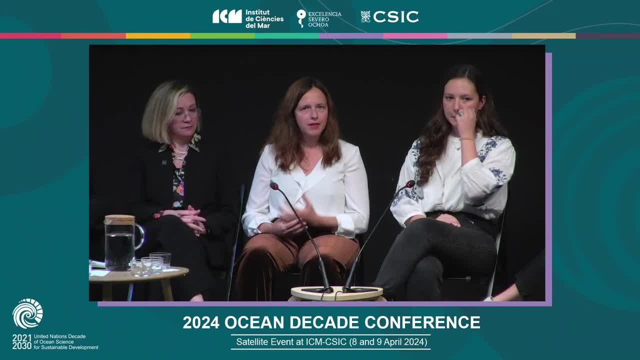 So I'm the founder of Oceanogami and the idea of Oceanogami actually started when I was working in Galapagos. I saw that there was a lot of connection of the people with the ocean and there was a lot of respect. 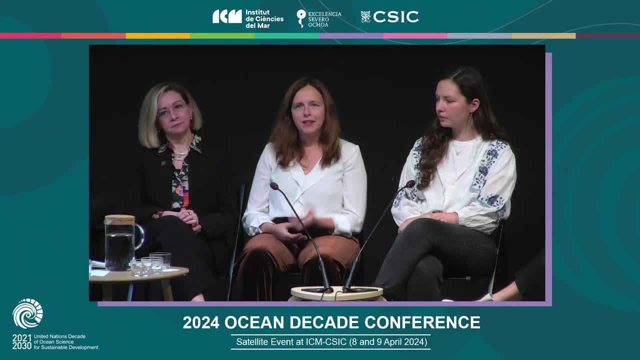 for the nature there. And then I came back to Barcelona and I realized that we were, at the moment we were still living in the- we say in Spanish, the espaldas al mar, in the back to the sea, So we were not really looking at the sea. 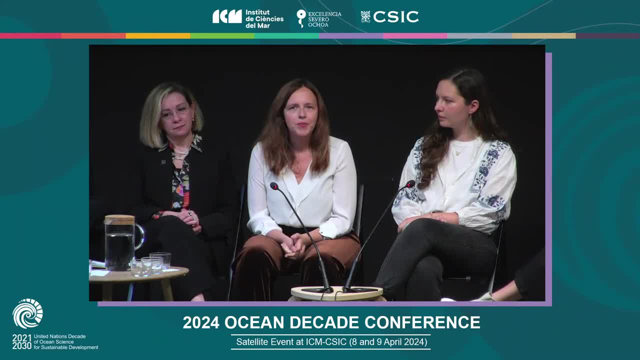 and what we have here actually. And I wanted to ask you- okay, we are quite biased audience because we are here, because we care about the sea, but how many of you have been doing snorkeling, have done snorkeling in Barcelona? 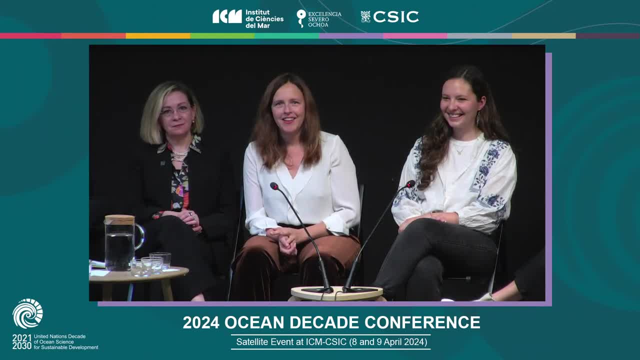 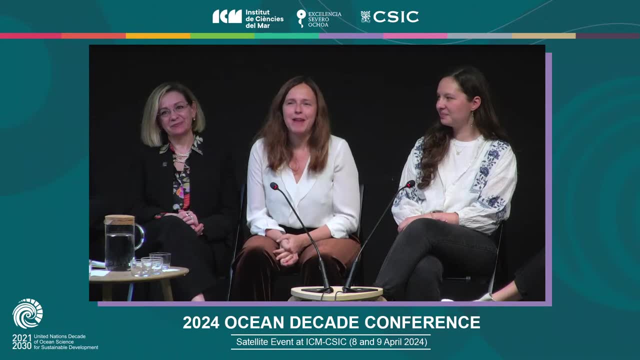 Can you raise the hand, Okay, well, okay, I was thinking it was going to be more actually. so, yeah, this raises my point. no, There is still. I know some people. they come from abroad, so they didn't have the chance. 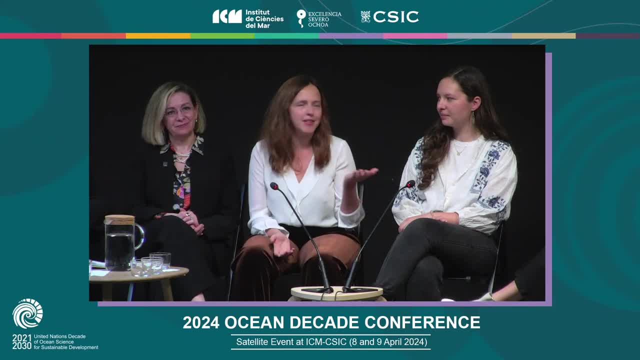 but if you have the chance these days, I encourage you- it's amazing weather at the moment- to do a snorkeling in Barcelona. I can recommend you where to go and with who to go. So, then, that's why I founded Oceanogami. 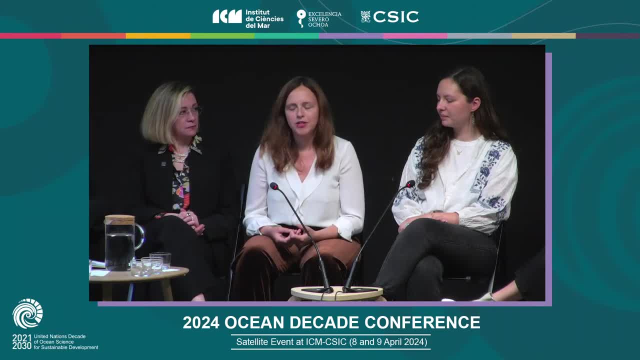 to engage the different stakeholders for the marine conservation And particularly, I found that there was a need in the private sector. The private sector, even if the company doesn't have any relationship to the marine environment, they have to do, the employees can do something. 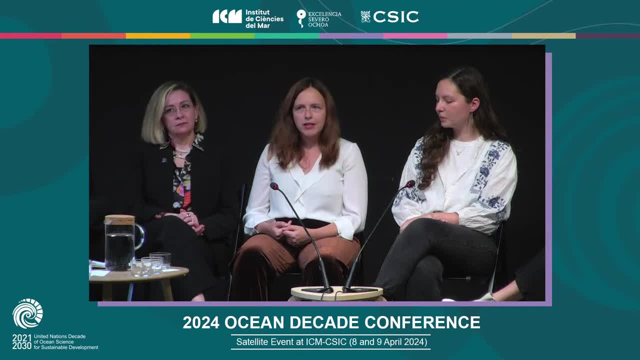 to protect the ocean. So we work with actually any company you know that wants to do something to protect the ocean, and we work with the employees. So we do also other things, but one of these projects with the companies is that we go actually here in Barcelona. 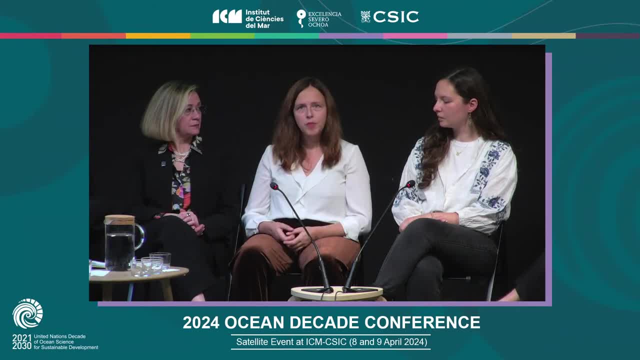 and also in different places in Europe, but particularly we focus a lot in Barcelona and with the collaboration of the Marine Science Institute of Barcelona as well. We go to see the impact that we are causing. So we think this is a thing that activities. 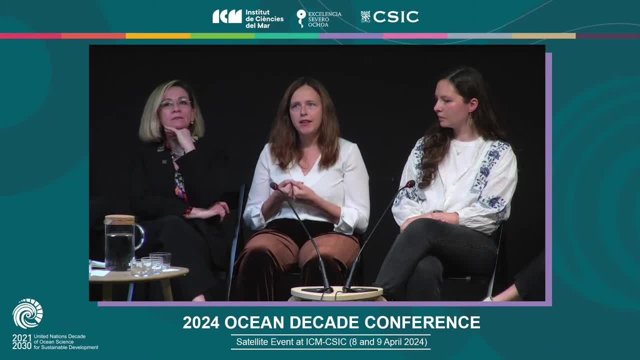 that you were mentioning. So this is the way that the employees they see the impact that we are causing. For example, the single-use plastics that there are still a lot in the coast. We collect it with citizen science approach, So we share this. 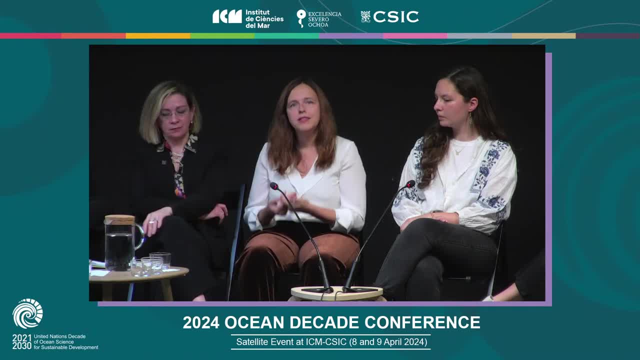 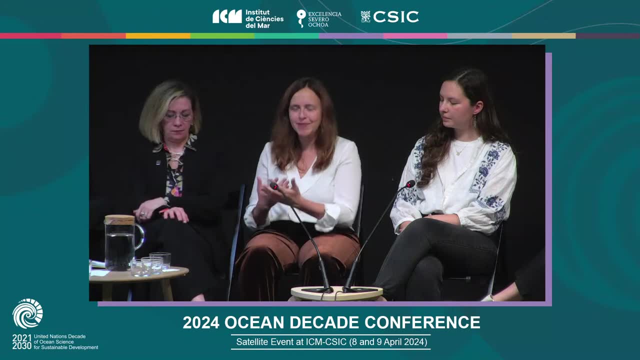 with the scientists And then, if they see for the first hand, they see the impact and they also go snorkeling to see the marine biodiversity. that is in Barcelona. It's quite amazing. I recommend you. So this is a way to engage. 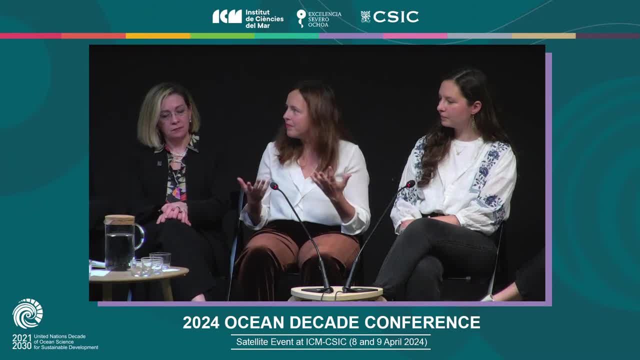 And I think for any sector, for any person, people in general, it's important to see, to really care to protect it. So this is the message that we want to give. So if you see it, you see why it's important. 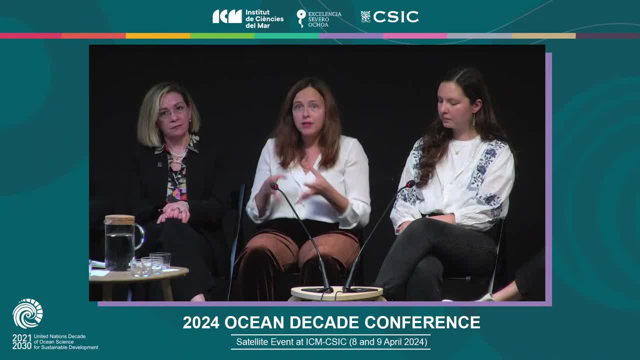 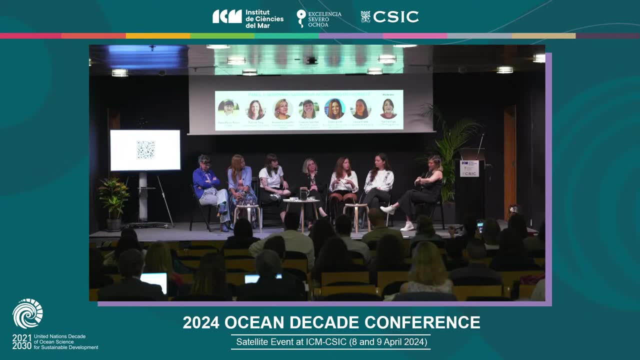 to protect, then you see the impact that we are causing and then you see you have to think about, okay, what I can do to protect. So then we can, for example- just giving a short example, and I finish- So, if you find us, 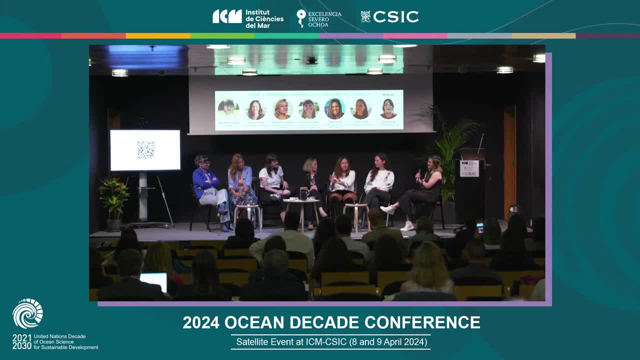 ear bat in the beach, for example. you have to think, okay, how this came? So this came because somebody throw it in the toilet and went to the river and then went to the sea. So just an example, just to think. 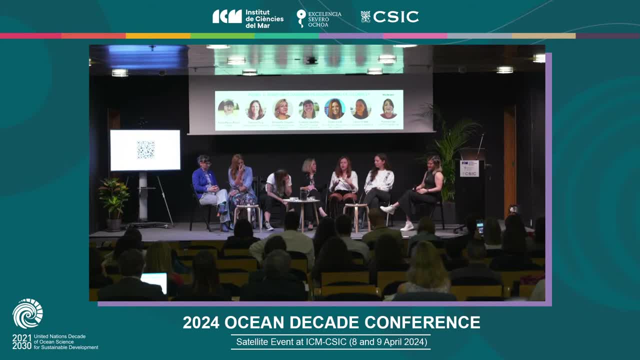 okay, maybe we can avoid it somehow. So this is a way that every one of us- and of course, this has to be from all the sectors, not only the citizens, but this is a way to think- okay, how we can do something. 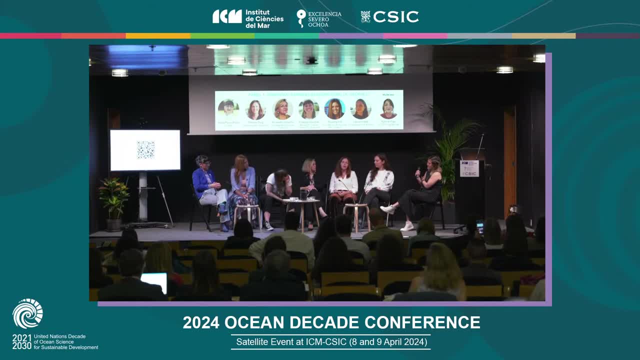 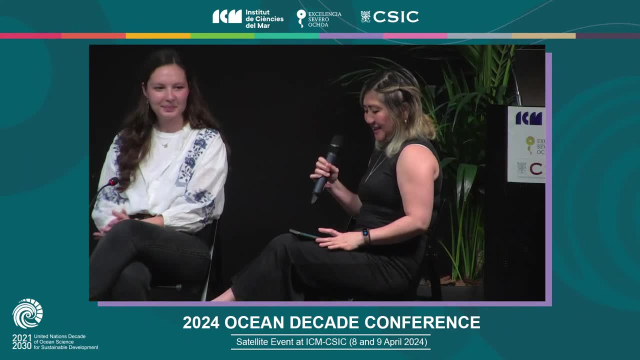 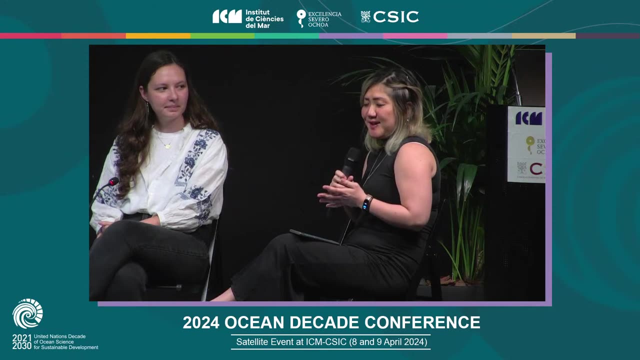 even if it's little. So this is what we do with the companies. Okay, thank you. Thank you for sharing your experience with us. So we are talking about the relationship with humanity and the ocean. So, but how we measure the behavior change? 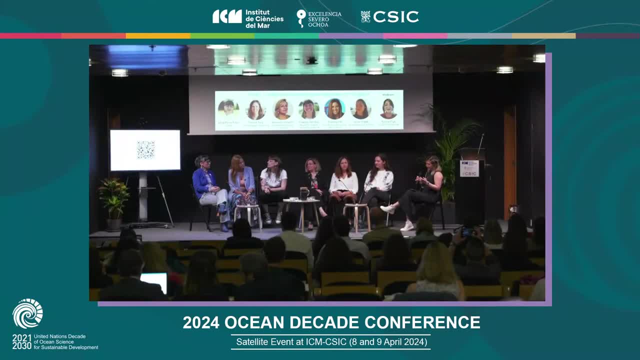 So I would like to ask Daniela: can you elaborate on how the ESRA methodology effectively measures the internalization of ocean literacy concepts within coastal communities and evaluate the short-term change in habits and actions towards marine conservation in your community? Okay, thank you. 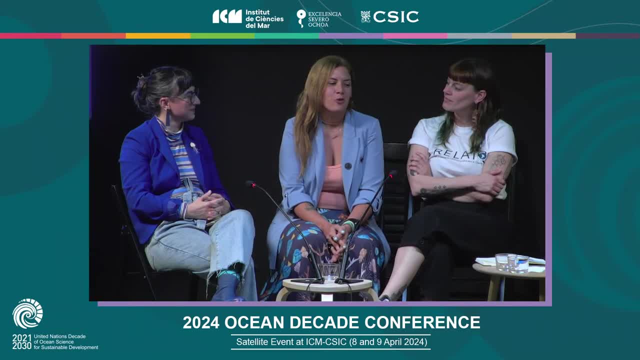 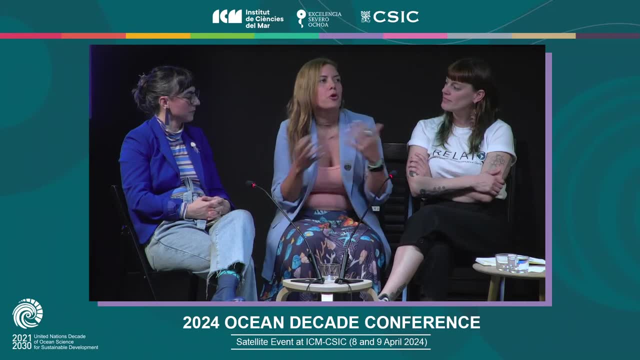 for the invitation. I'm from Ecuador and we're very excited to be here. So first of all, we I need to talk about like before COVID, we had another program and we had another methodology which had three steps. It was awareness. 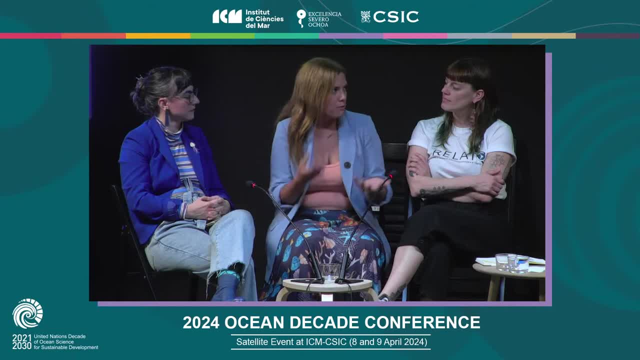 hands-on, which we used to go to the beach, you know, for picking up the garbage and a final stage of art art session. So, and in two years that we were doing this methodology, we were able to reach more than 10,000 kids. 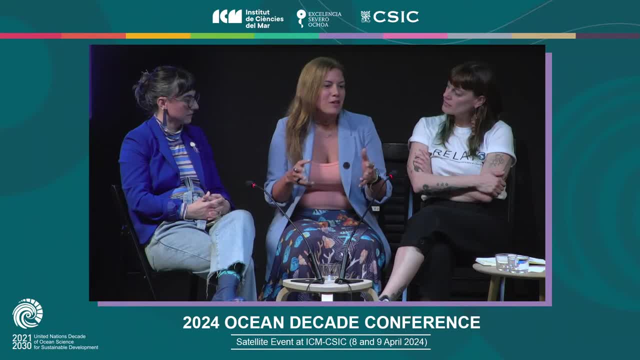 But then, during COVID and during those years, we were thinking about: okay, you know, we are missing something. We want to know what happened with these kids, that they were part of the project. So we were, you know, asking ourselves and we did like: 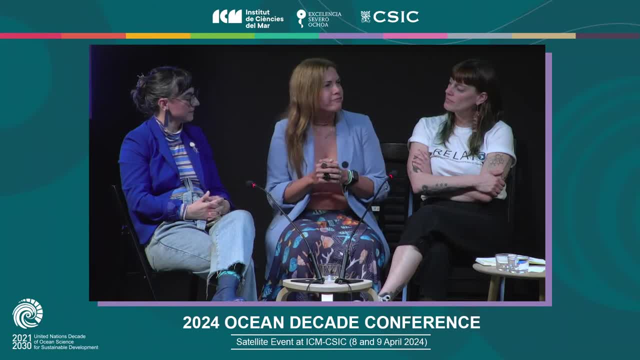 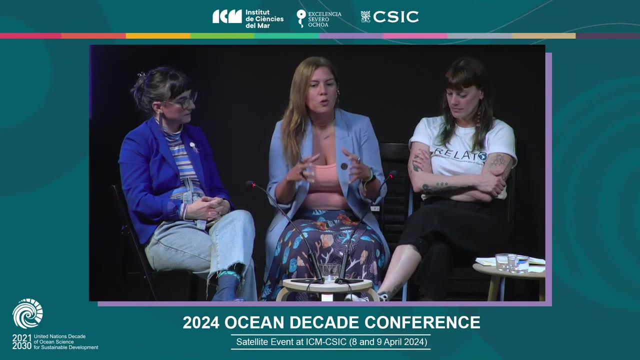 a team building initiative and we were like talking about: how can we know what happened with these? you know people that we are working with. What's the change? For us, it wasn't not enough to have this total number. total number of the beneficiaries. 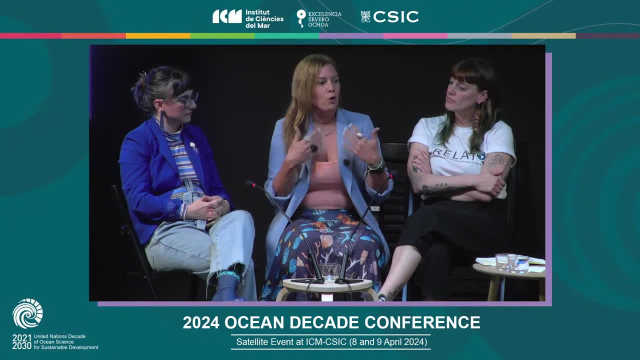 that we are reaching, But you know, we wanted to go beyond. So then, with this new vision, we started to create or updating these old methodology into ESRA. ESRA in Spanish means Explora, Siente Reconecta. 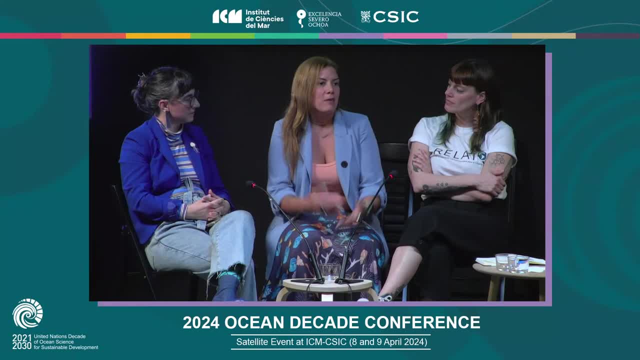 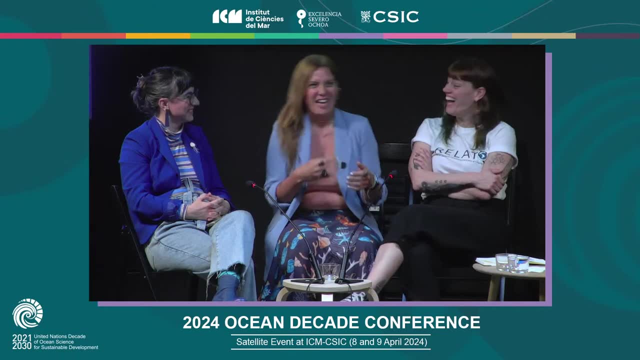 Actúa, which is explore and explore, aims for exploring the ocean literacy principles. Okay, Don't scare me To explore the principles. Feel it's like you know it's a ESRA, brings you to inter like it's an introspective analysis. 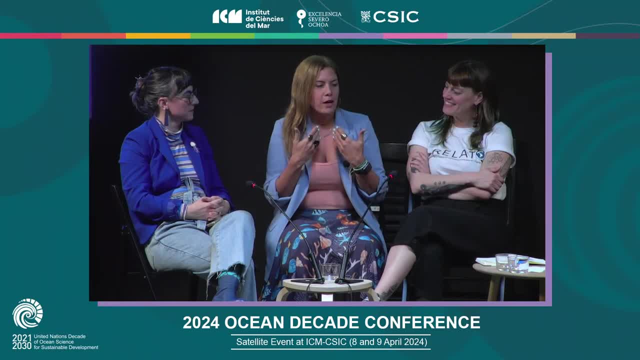 a personal introspective analysis of what is happening with these kids. So it's like you know, ESRA brings you to like it's an introspective analysis, so it calls you to do action, not just to wait for you know. 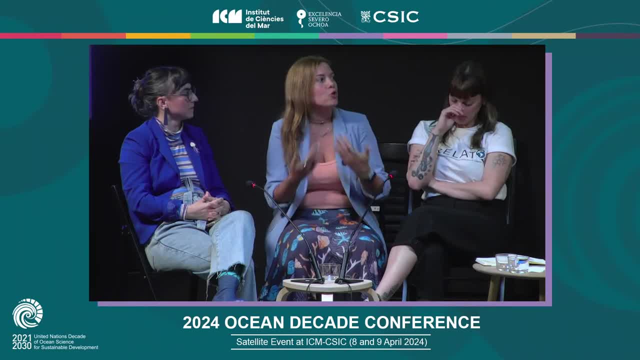 governments, other institutions, NGOs to act, but you know you do it for yourself. So these different phases from ESRA feel is like: okay, let's, it's about a lot of emotions and you know where are your thoughts. 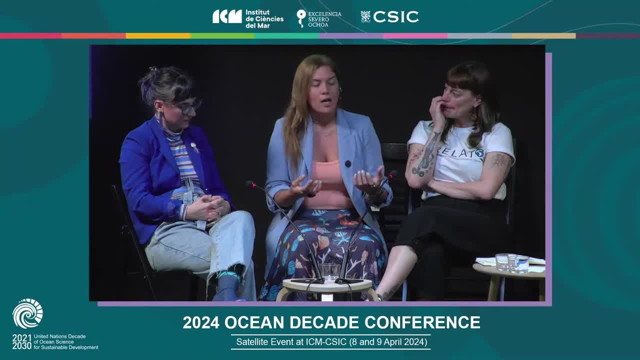 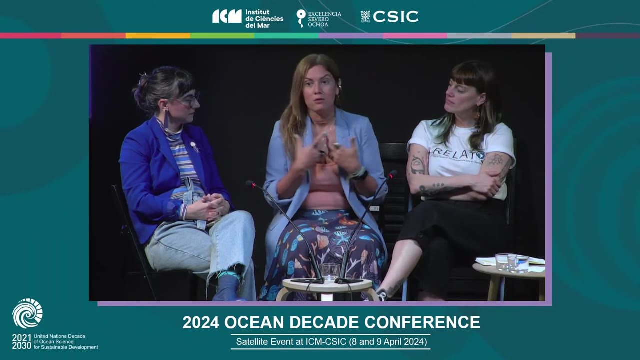 We bring together these emotions and construct this connectivity with water that we all have. sometimes that we forget, And you know it's about reconnection and it it goes like putting in presence our ancestrality and our culture that we have. 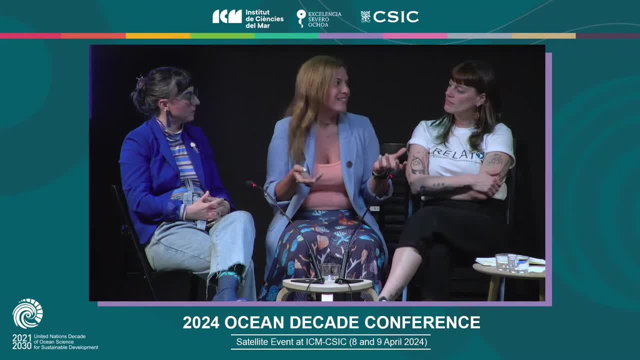 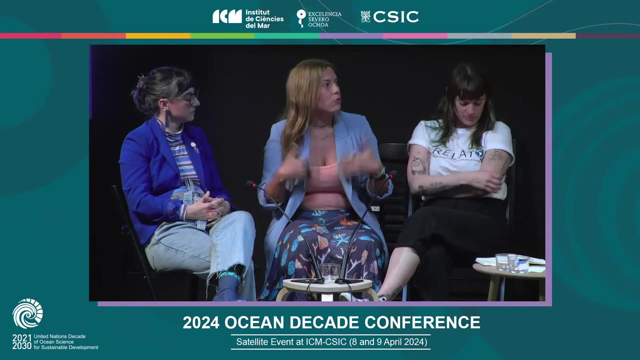 in a lot of places lost maybe because of colonization, And okay, and and act. It's, like you know, the call to action, how these, these kids who are in this 11-month process, are reaching outreach in their community. 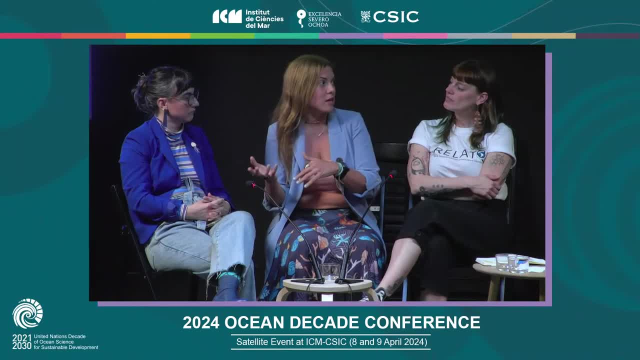 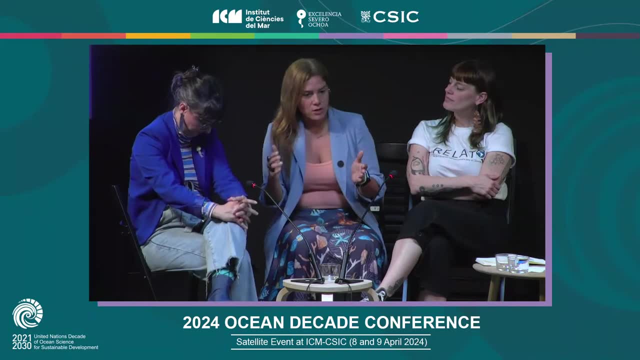 through their projects that they ourselves, they create. So at the beginning we are doing this survey, So we have this baseline and during this process of ESRA and this 11-month process of ocean literacy that we are building together, 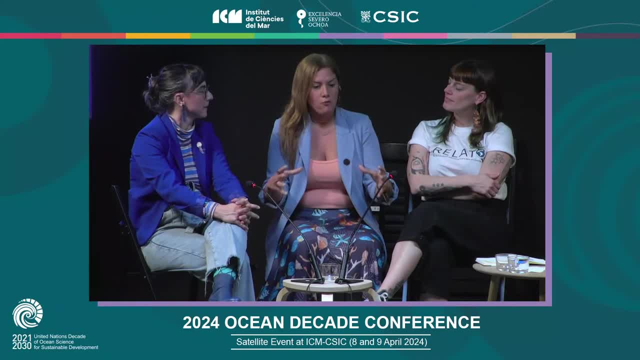 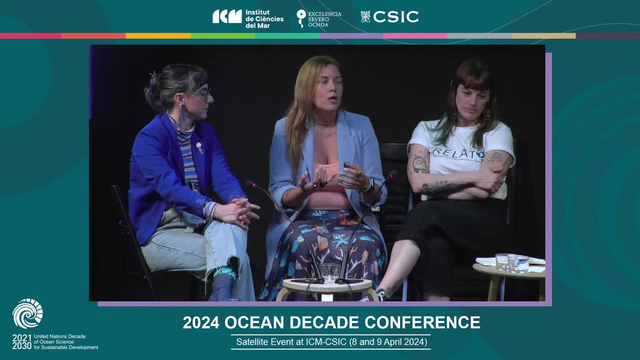 you know, we all bring perspectives and emotions and thinking for constructing these concepts that are very new. So we have this, for example, the percentage of people who are think to the ocean, about ocean literacy, knowledge, the, the changing behavior. 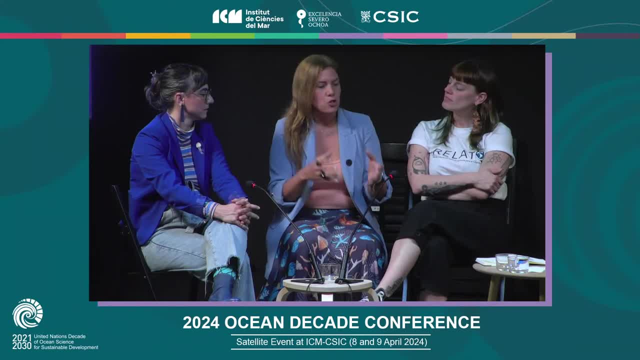 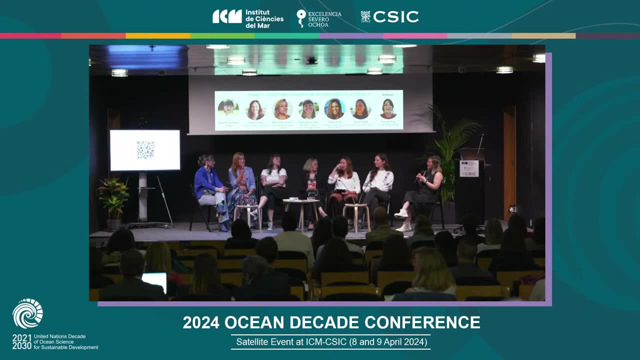 what? what are they doing? So we have observations, evaluations and other surveys so we can manage the information like a before and after Right, Like try to summarize Awesome. Yeah, I think we have a lot of to talk with Daniela. 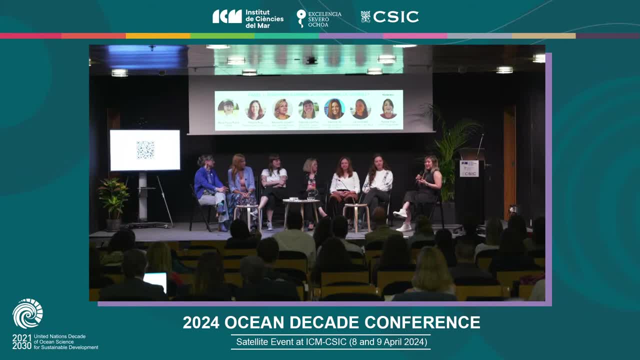 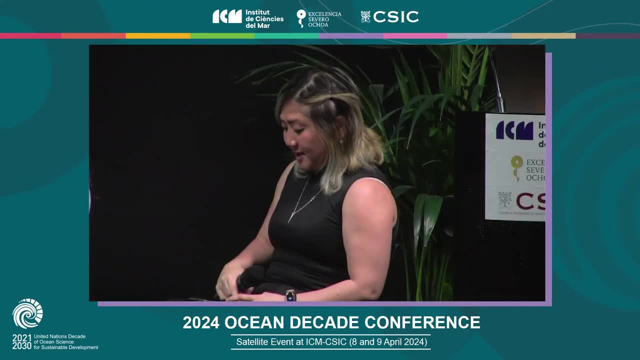 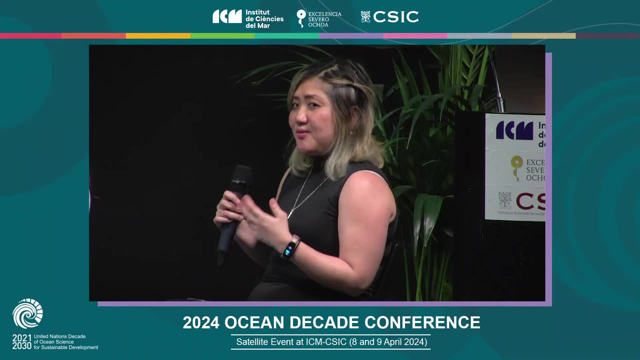 because it's very inspiring that this methodology, this metrics that we can use for many projects based on behavior change. But move on to the next panelists. We, we work. ocean literacy needs to reach different actors and stakeholders, And I would like 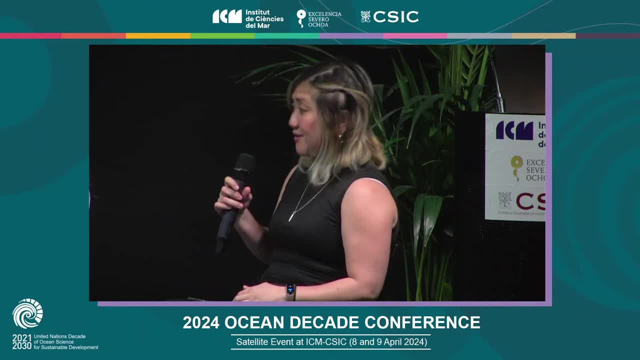 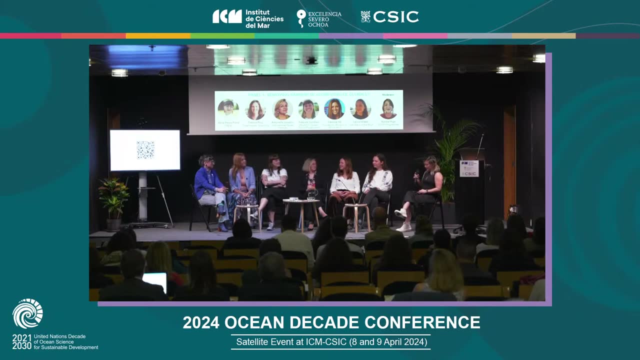 to ask Alicia. Alicia has a very different research field And she works with different stakeholders, So I would like to ask you: how does promoting your project helps research, researchers, policy makers and decision makers understand better how land and ocean ecosystems 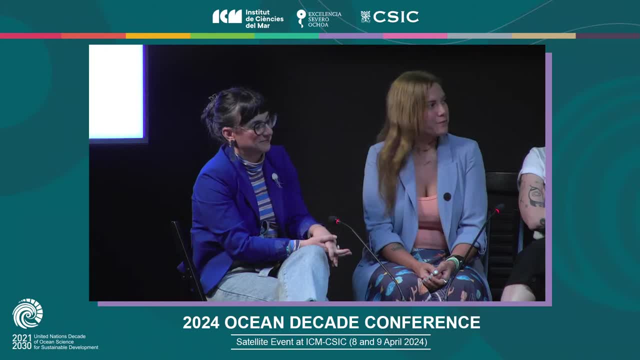 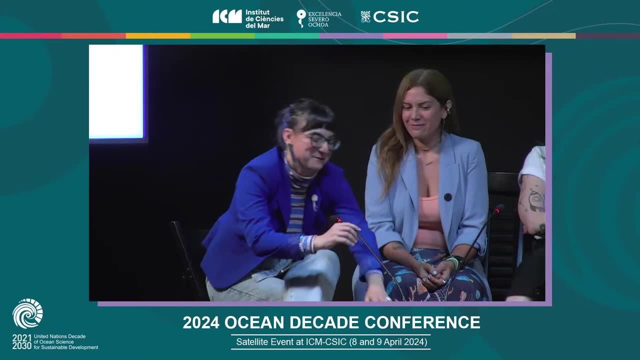 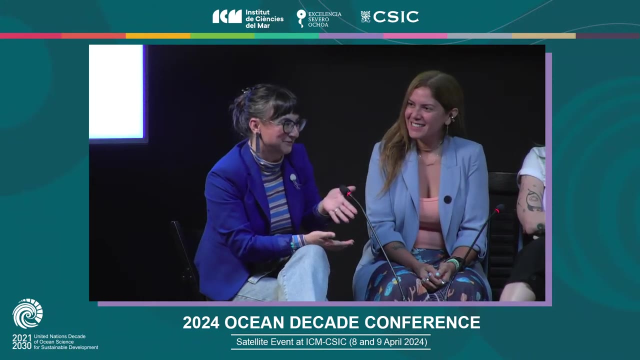 are connected. This understanding can improve oceanology and encourage better ways to manage the environment. Can you explain a little bit? I will try. I will do my best In three minutes, In three minutes. So thank you very much for the invitation. 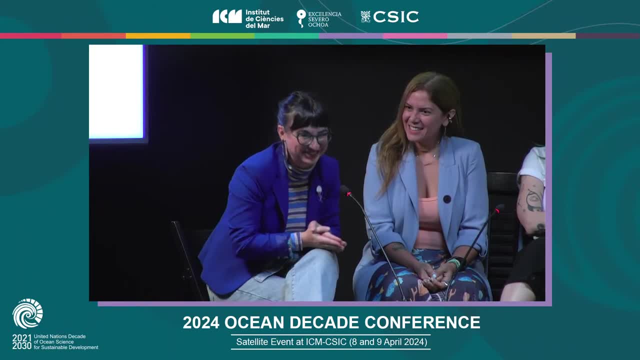 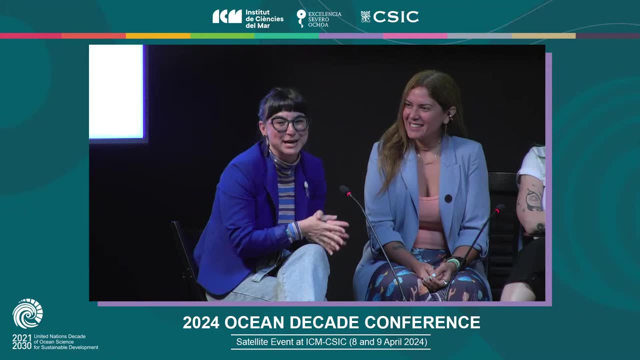 and for being bold enough to invite me to this panel. So I'm the exotic element of this panel. So, for those that are living in Barcelona, I am the scientific coordinator of CREAF, which is a research center in terrestrial ecology that mainly 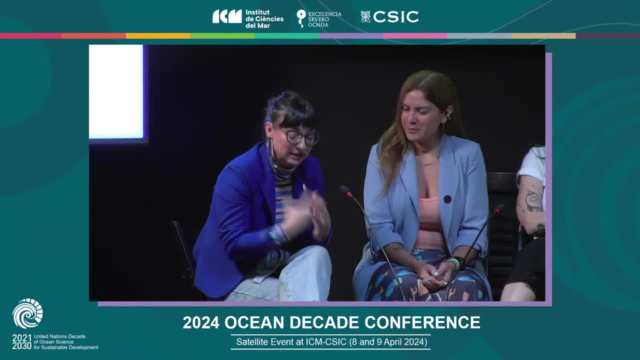 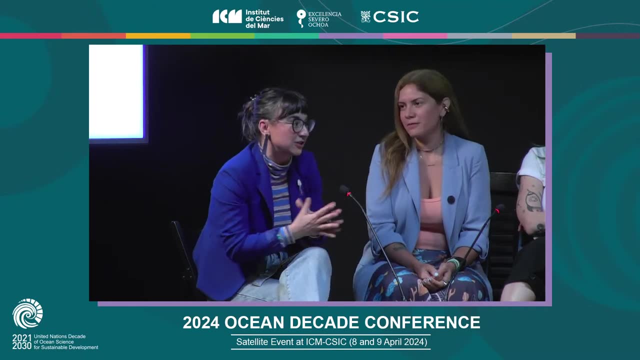 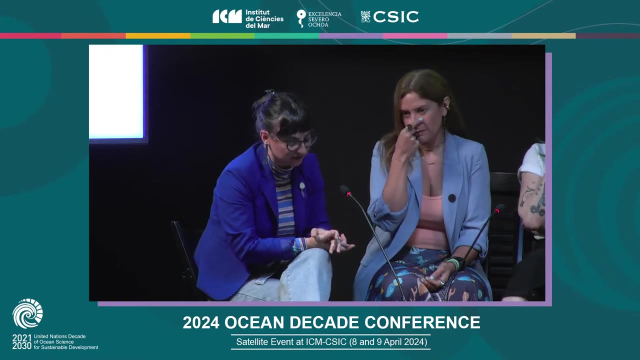 focuses on forestry. So by training, I'm a marine biologist And we are going to talk about why even researchers sometimes were giving our backs to the ocean And we started talking about something that, I have to say, I didn't create. 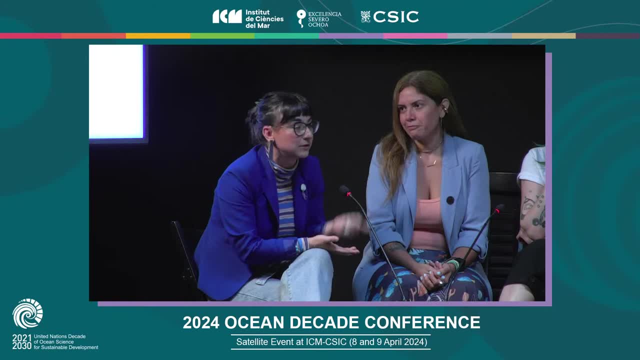 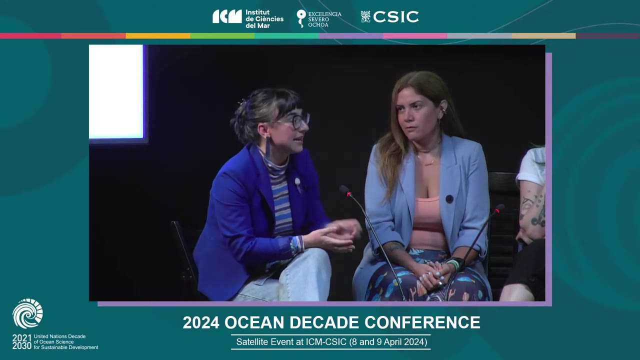 this name, but we started talking about turquoise ecology. And we started talking a couple of years ago when it was COP25 that was supposed to be in Chile and that ended being in Madrid. And we started talking about turquoise ecology because Chile has a lot. 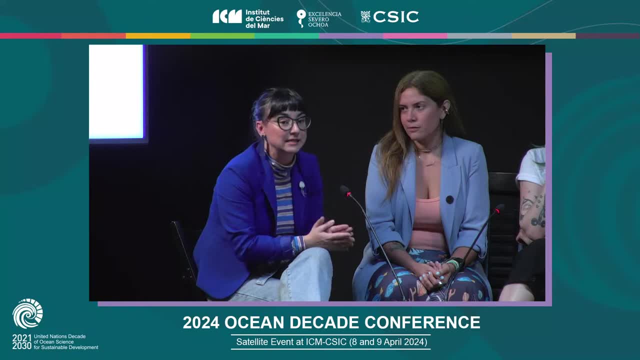 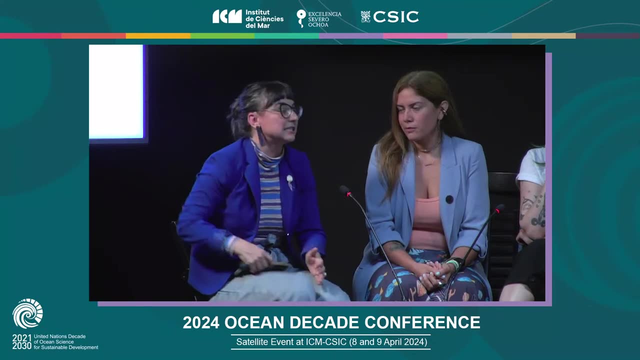 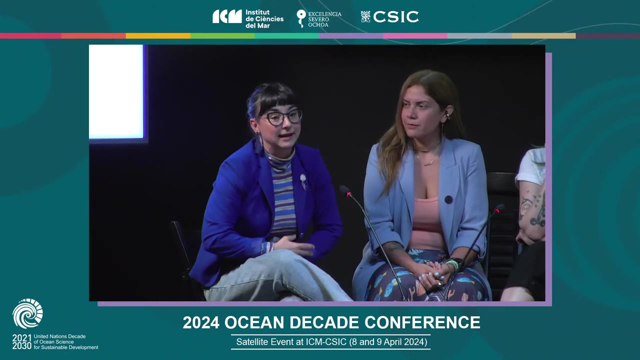 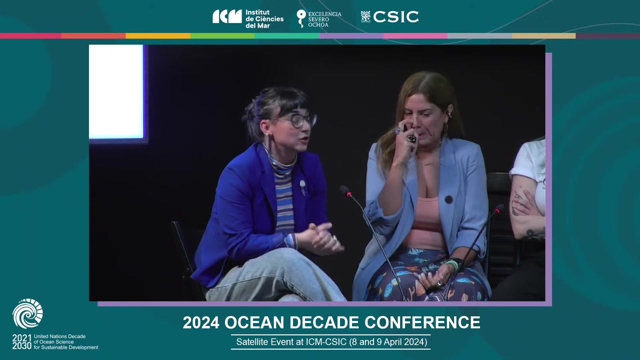 of coasts and also has a lot of mountains and land. So they created this turquoise diplomacy that now is transformed into turquoise foreign affairs strategy And, inspired by that, we started creating our turquoise ecology narrative. so we said, well, no blue. 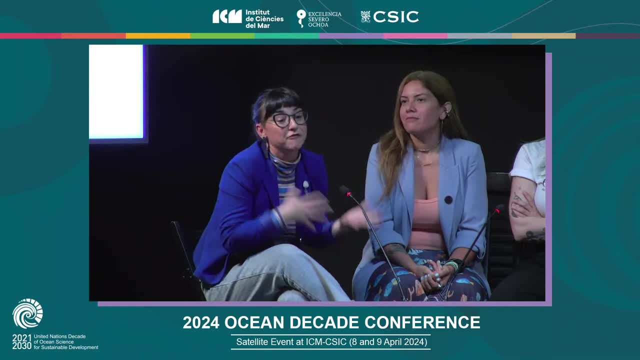 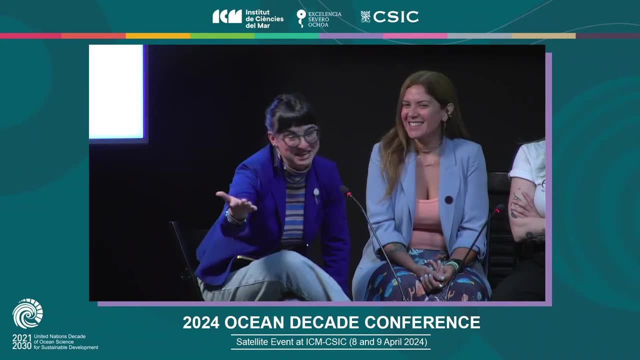 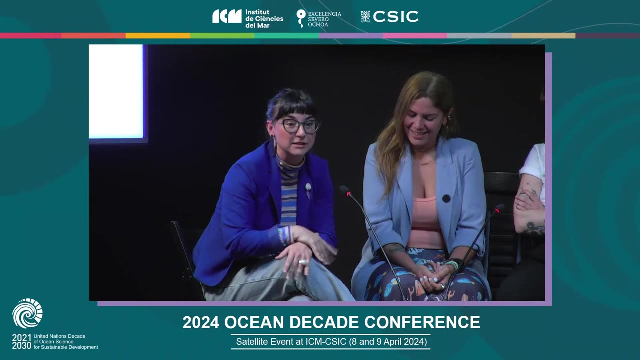 no green, and what happens in the green doesn't stay in the green, affects the blue, Hence the blue plus the green turquoise. So in case you needed the explanation, So we started creating this narrative of like well. 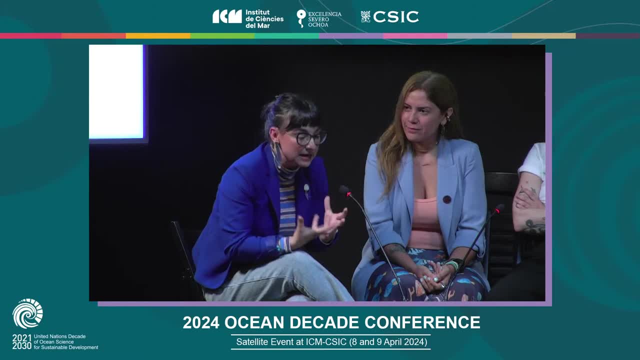 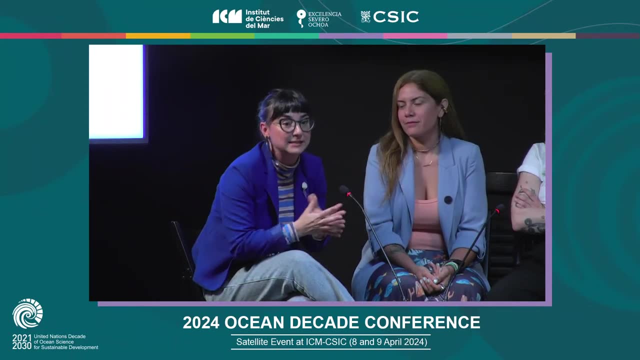 there's a couple of researchers at CREAF that they are like studying things in the ocean. So let's start putting a name of this, and because what I basically what I do is that I do science for policy and science diplomacy. So 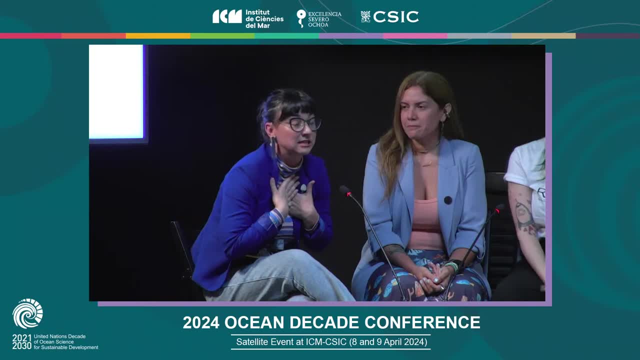 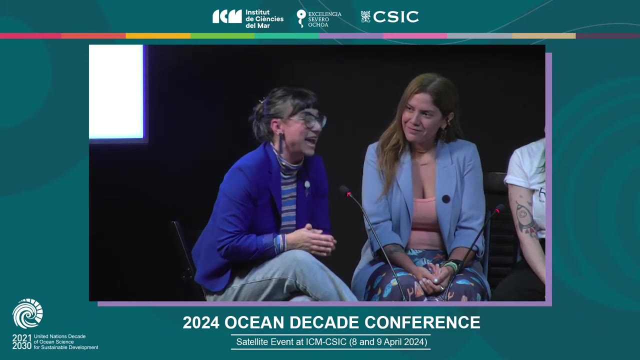 I talk to a lot of decision makers and policy makers and I started informally talking to those people to see how they were creating their policies and legislation and I saw not. I'm not going to say that everything was completely separated right, And 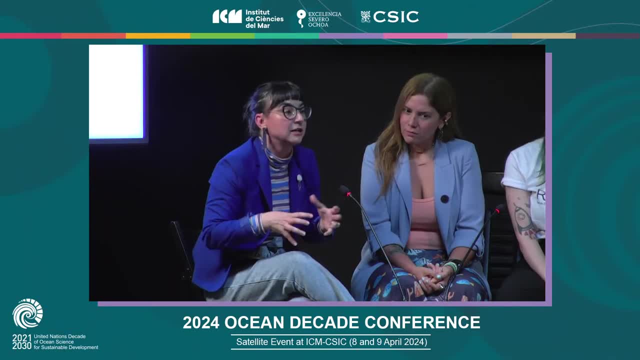 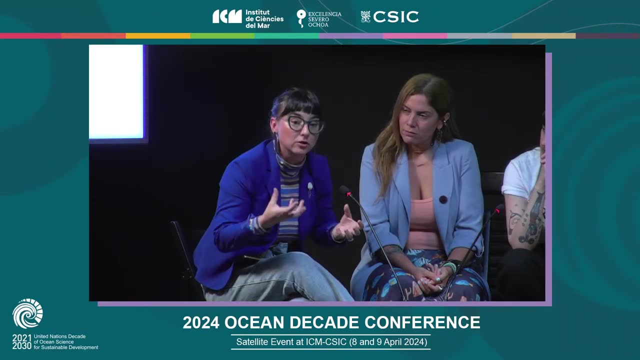 internationally. we are always talking about breaking the silos. We are talking always in silos. So what we are looking for with this turquoise ecology that right now, more than a project, is a narrative that is permeating in our strategy and we are 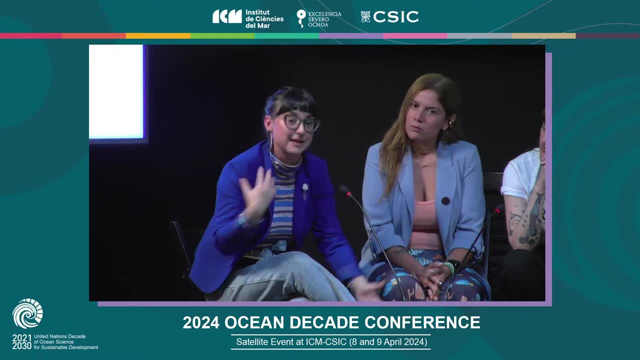 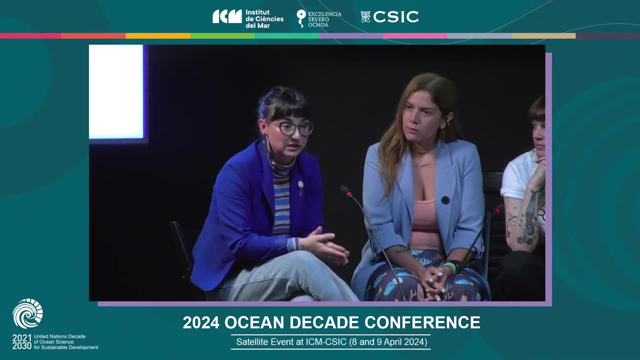 start like we started talking to other people and we joined forces and when we talked to legislators and decision makers and policy makers, so they consider this as a whole as a turquoise, not as a different silos for green, for blue, for climate change. 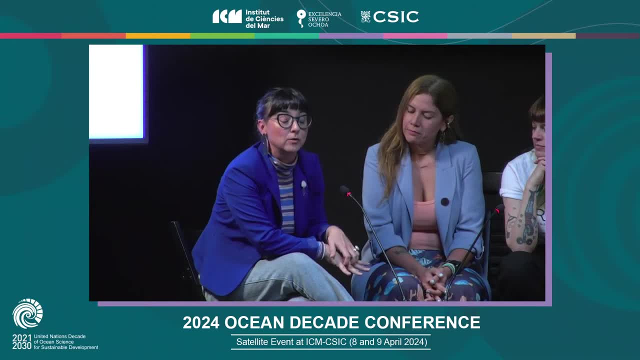 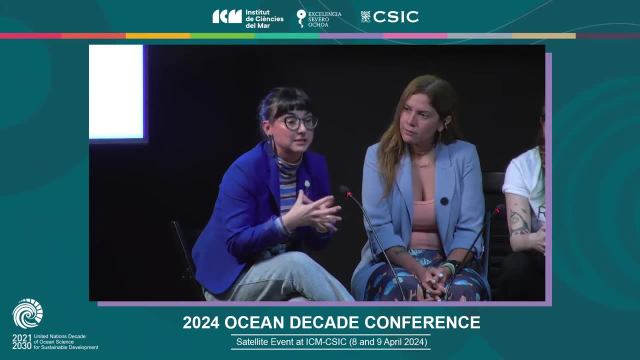 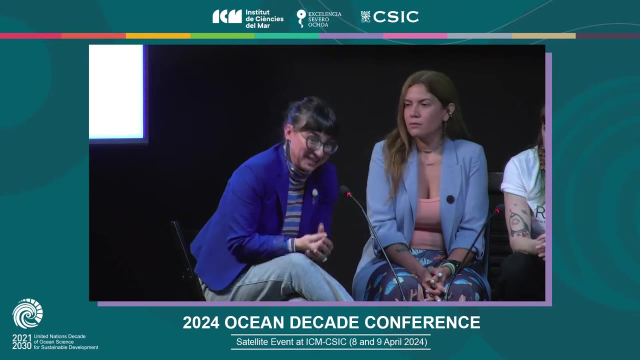 for biodiversity. So, and and the idea is to like, do our little thing on breaking this silos and construct a turquoise narrative that is going to, yeah, make them understand basically that what happens in the green doesn't stay in the green. 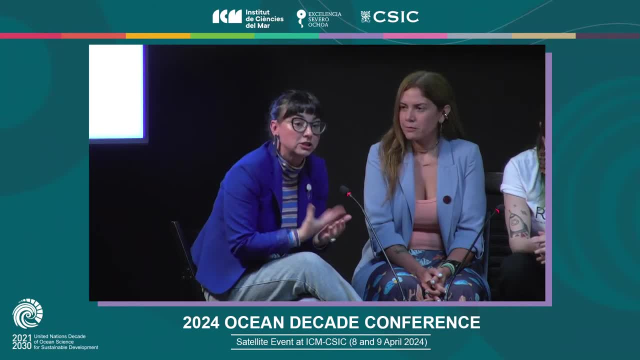 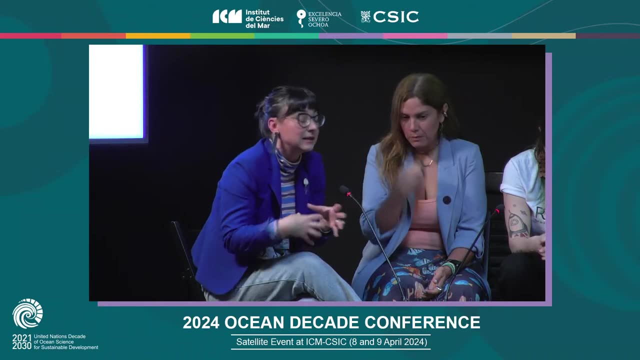 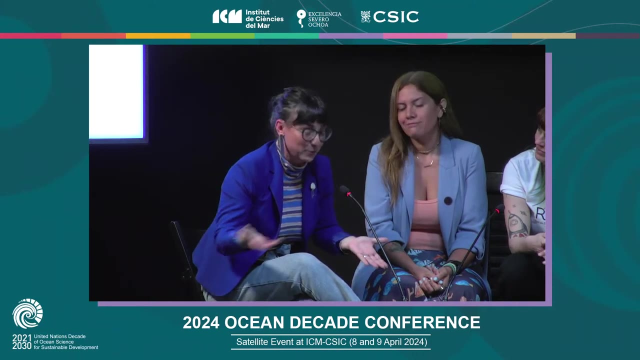 and when you create certain policies, you need to take into consideration not only the effects in the green, but also the effects in the blue, and it's very much a work in progress. It's very challenging, as you probably know, but hence here we are, so wish us luck. 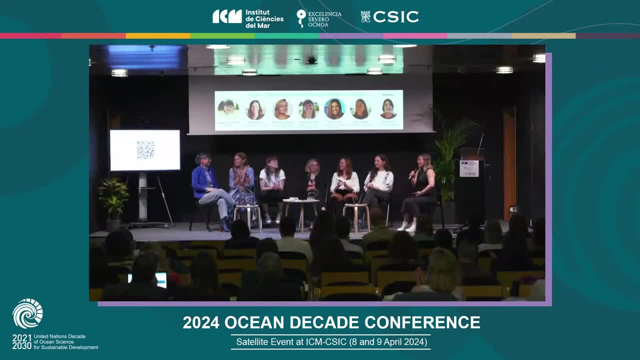 and join us if you're interested, Thank you. Thank you for sharing. So now I guess the audience is very curious about the all these amazing projects we present today, so I will open a few minutes for the audience to ask some questions. So we have two microphones. 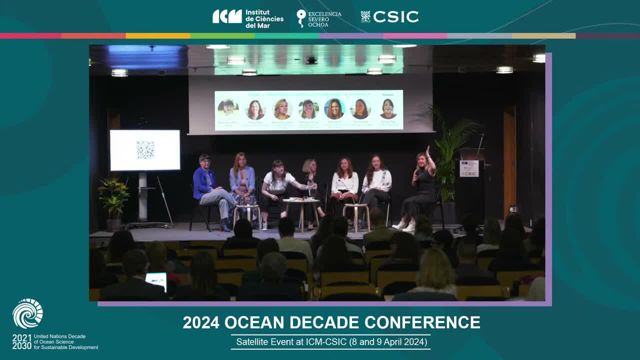 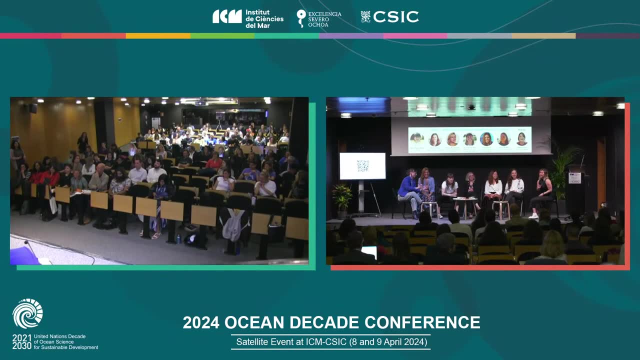 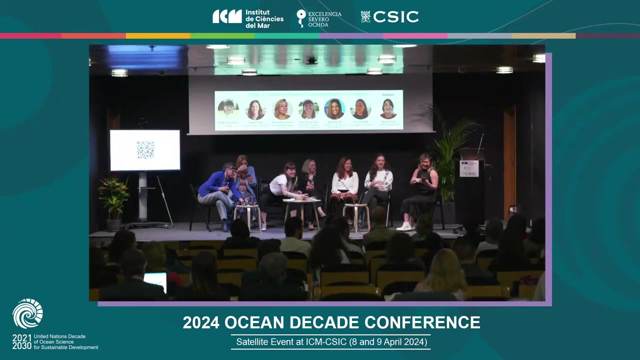 around here. so just put your hands up and yeah and ask No, No questions, Really. So you guys understood everything. huh, They explained very well. yeah, I will give you the last chance. Last chance, Okay, Thank you all. 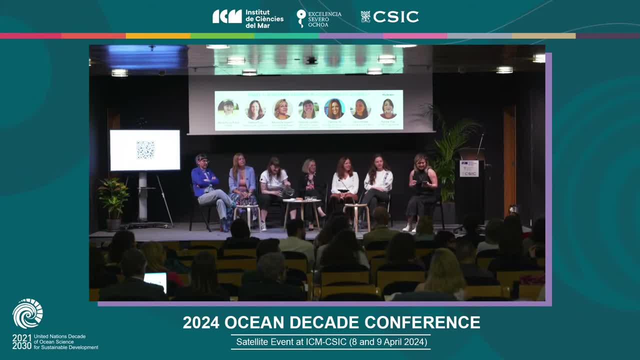 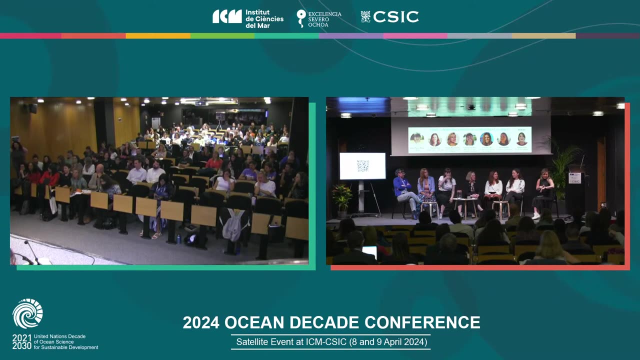 Really interesting. All were really interesting, but I have a question to Antonella about her tool: if she can explain a little bit more how it works, where it is accessible for projects, for example. and so thank you. Okay, Thanks for your question and your interest. 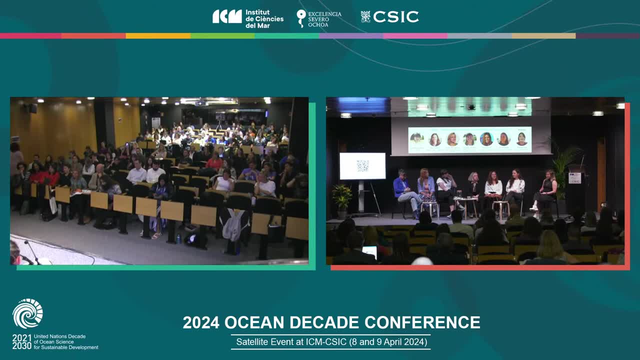 I'll try and make this short. The Ocean Academy started because we had a lot of people graduating ECOPS from our capacity development programs. They came back to us, they indicated that, you know, while the program was very interesting, interdisciplinary- something they also got. 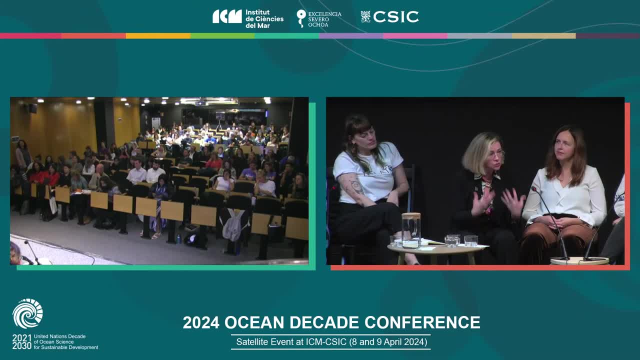 from the program was the awareness of needing to give back to their communities. The alumni come from all over the world, and thus the Ocean Academy, which is the Ocean Literacy level project, reflects that. So what we did was we created a program to work with our alumni. 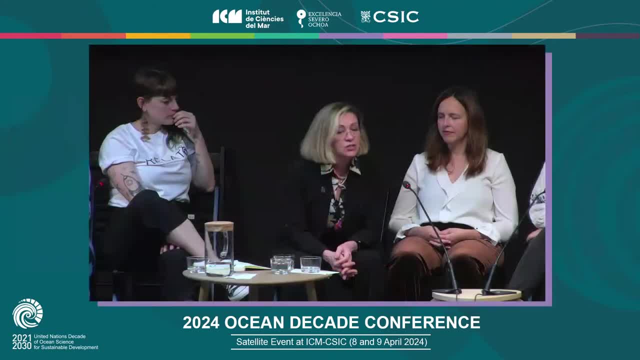 We, you know, we started the Ocean Academy and we started the Ocean Literacy level project in 2009.. We trust the alumni that they, who themselves are experts, professionals in their own field, will be able to take knowledge back into their communities. translated. 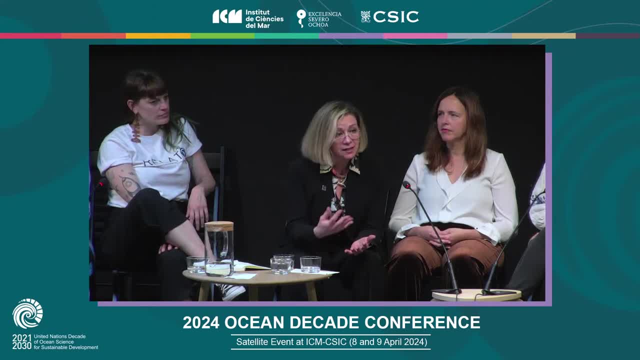 into the local idiom, the local languages. and just to give you an idea, for example, in Sri Lanka they work in the local languages. In the Maldives they deliver the programs in Divahi. In India we have Hindu Marathi. So 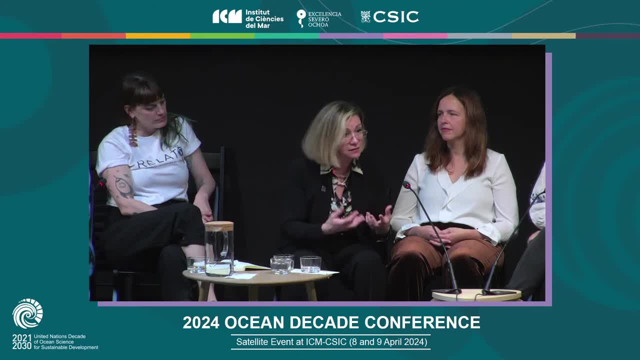 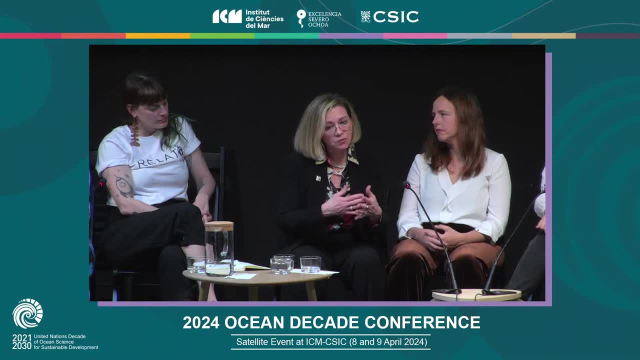 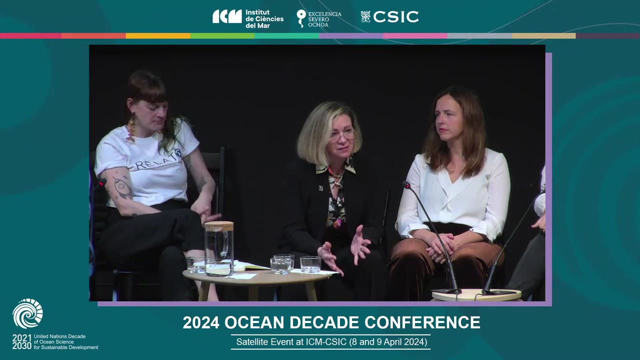 a lot of different people with different languages and really able to understand their communities, the knowledge they need and give it back. Barriers we noticed were language, which we have done our best to overcome, but also access. How easy is it for anyone? 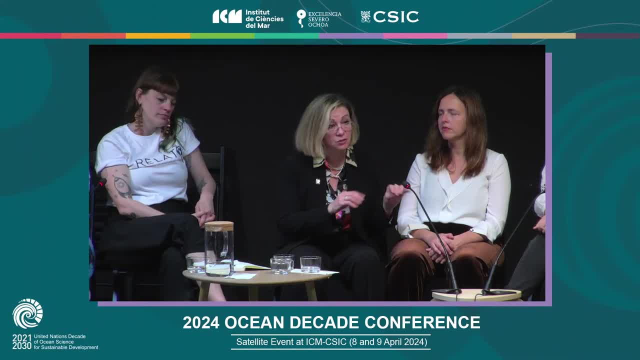 a citizen to be able to drop everything and go to a specialized course. Sometimes it's really hard, but if you're able to connect online to this and it costs you nothing except a bit of time and attention, then of course the uptake is much. 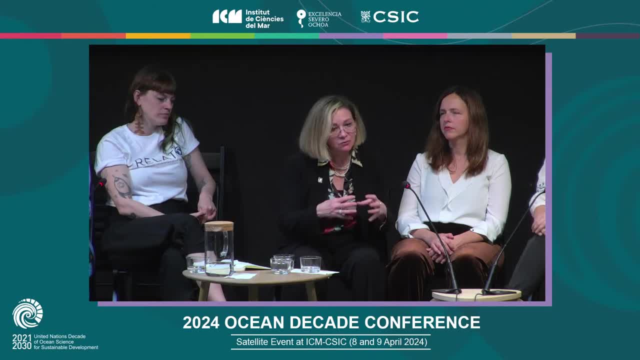 much easier, if you wish. The other thing we emphasize a lot in these projects is that the we strongly believe that, in order for us to achieve Agenda 2030 and the SDGs, people have to come on board and people truly, when they're interested, when they're invested. 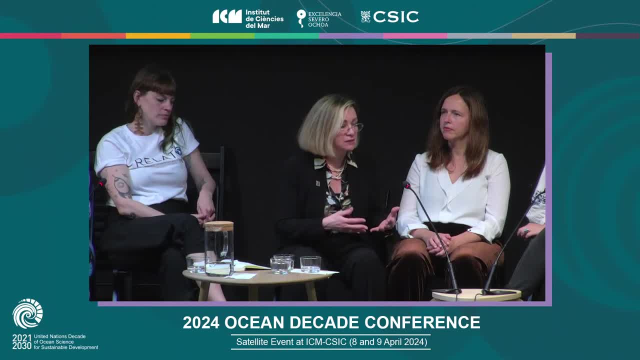 you know, in the jargon it's ownership and empowerment. but the reality is, if you know about something, you care about something. if you care about something, you're usually motivated to do something about it, and that is what underpins really the project. Bring information as easily. 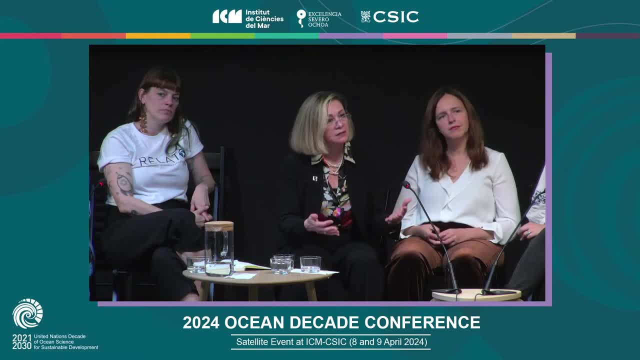 as possible to the target communities and slowly, slowly, drop by drop, and change will and does come. I'm glad to say it's been a very successful project. over the years, Thousands have joined. unfortunately, there's a lot more interest. we want to do more. we will do more. 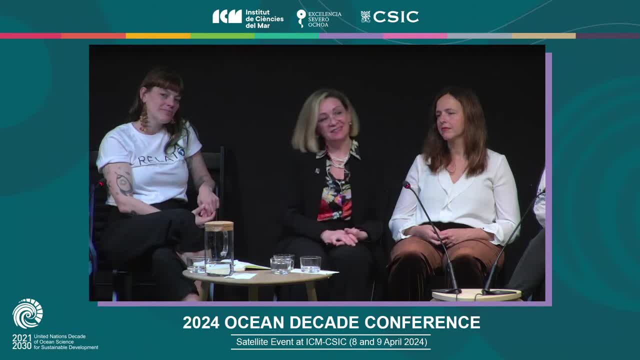 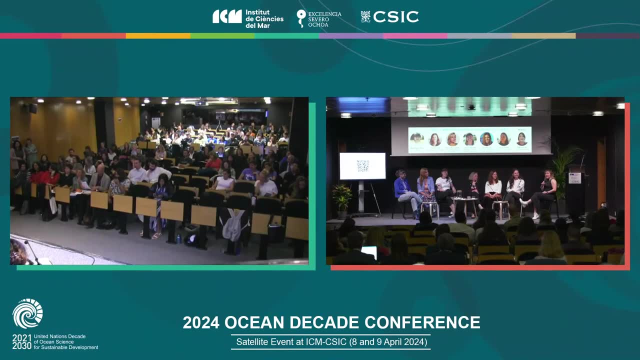 and in a summary, it's but happy to speak more about it with you later, Thank you. Thank you, So last chance, last question. Okay, Hello, I don't know if it's a question or a comment, but I think the the concept of turquoise. 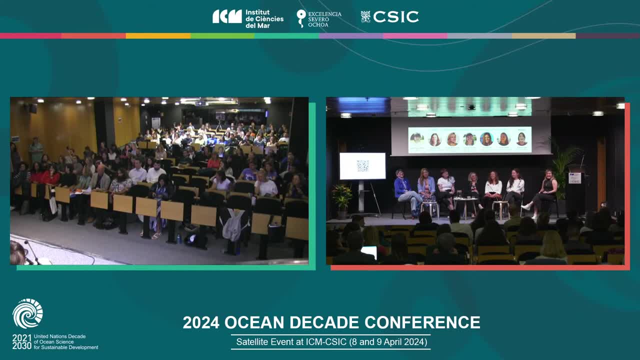 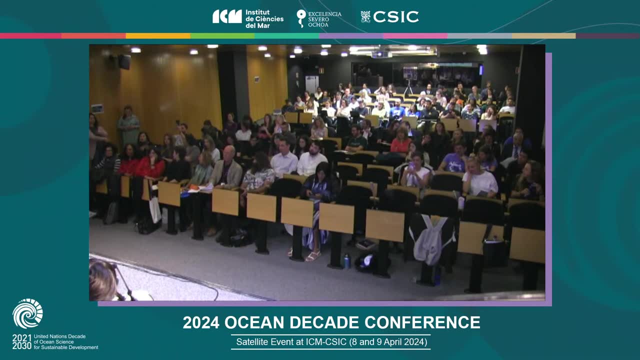 ecology is very powerful. So I was thinking, I was thinking it should be introduced into the educational sector, because I think it's a very good thing to talk about, especially in landlocked areas where they have special difficulties in treating the ocean, because I say, okay, we live. 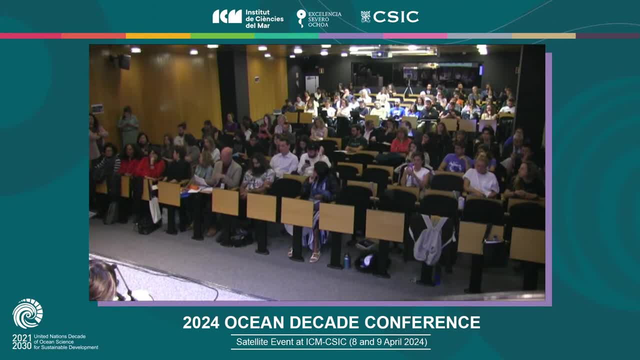 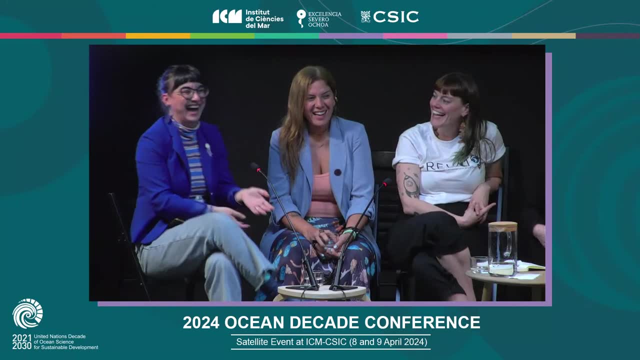 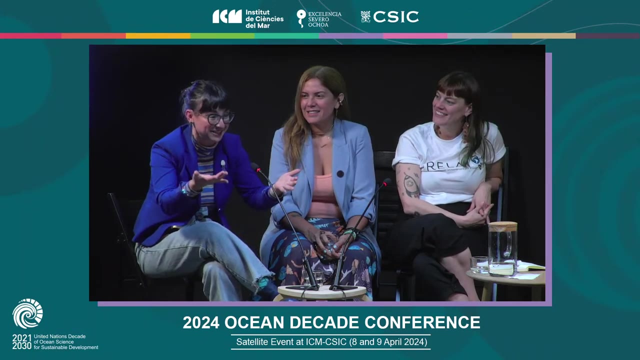 thousands of miles from the ocean. no, But we have a lot of problems in the educational sector, in the formal and informal educational sectors. Yes, What do you think? I cannot agree more: No, And also you know like I, I always think about my kids. 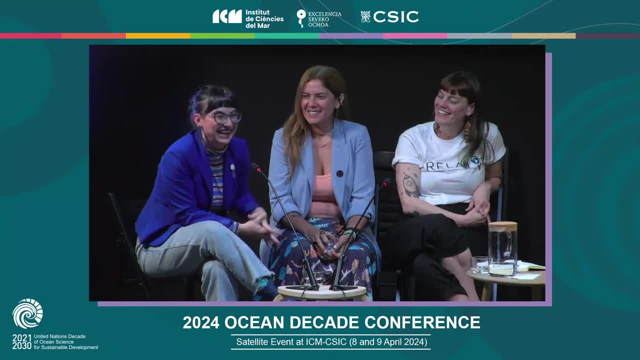 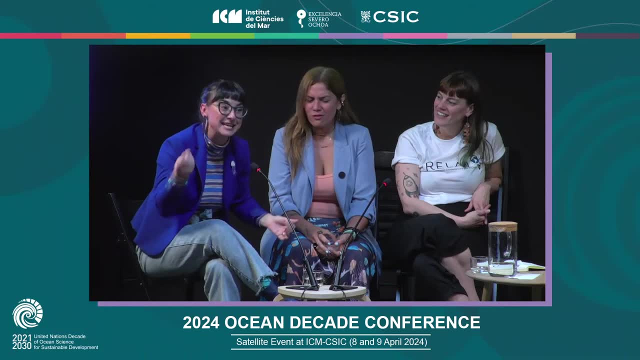 about that, because sometimes we're in the forest and my kids are obsessed with the ocean- I have nothing to do with that- and like and they and they pick up the trash and they say: what do you do? there has an effect, so I think that it can also be. 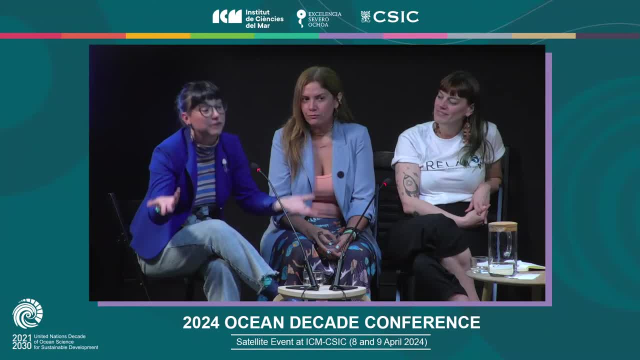 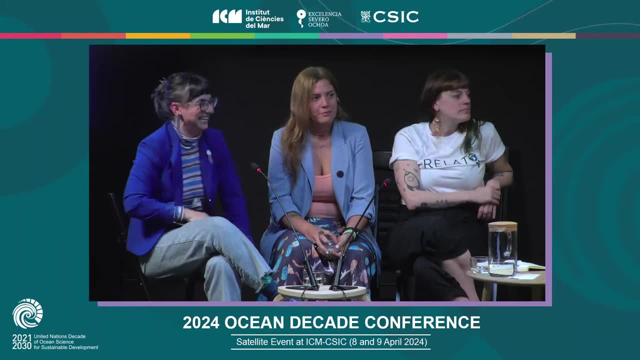 you know, a way to connect kids that are really far away from the ocean with the ocean, and because this is what we want, right? So, yeah, If I can say a small comment about this, because this actually reminds me, some years ago I did my Erasmus. 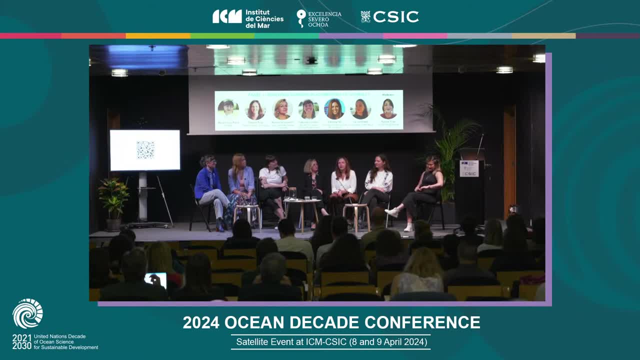 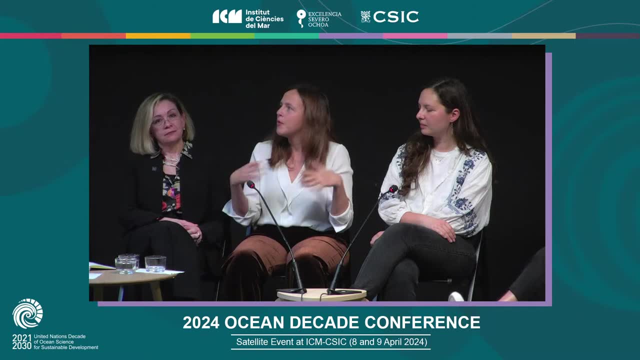 in Trieste and I had the best lesson ever. it was a lesson about about algae actually, but we were where there were trees and he was explaining. the teacher was explaining ecology, comparing the ecology of the trees, of the you know for the forest, and the ecology you know. 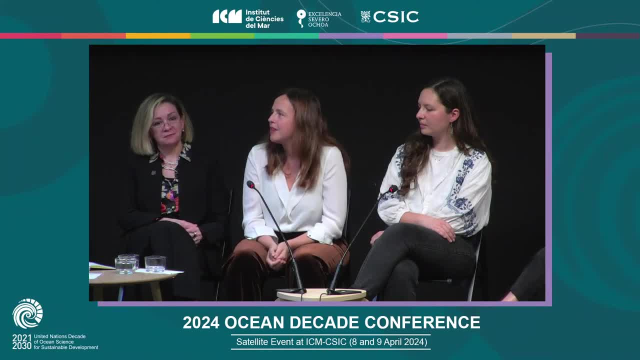 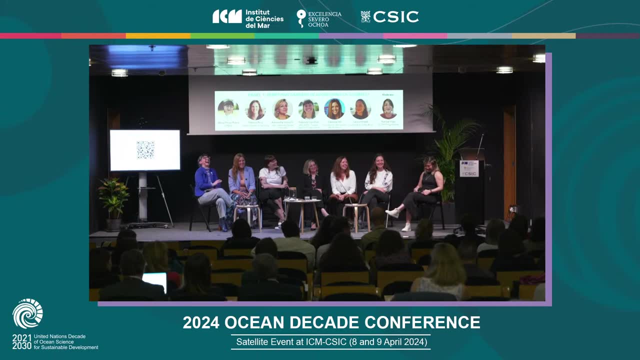 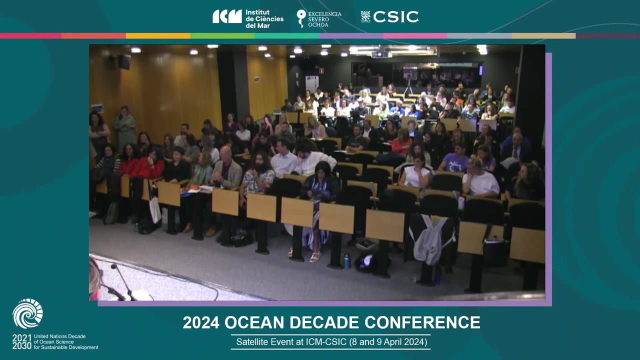 of the algae. so I think this is something that you can do, yeah, everywhere, even if you are not in the sea and you are not close to the sea. I can add something, because here in this house, at the website of the ECM, you can find a very nice game. 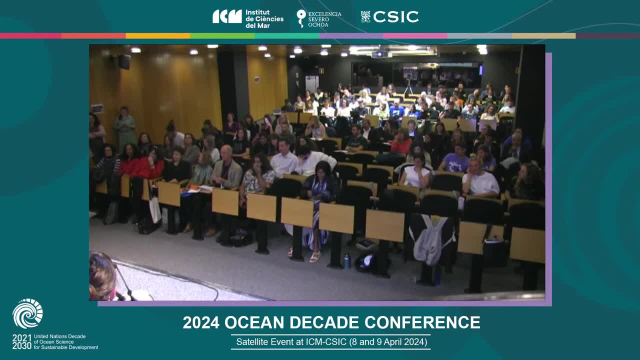 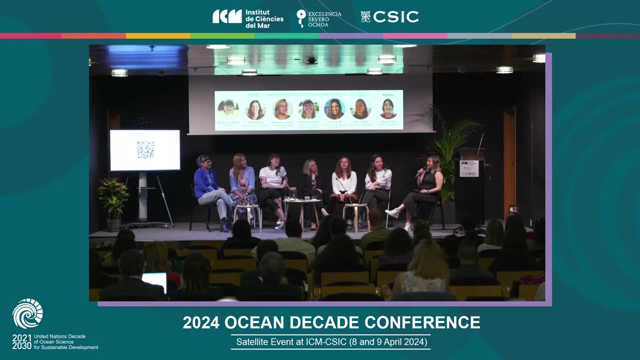 board game, which I think we are talking about, Patricia. so exactly, yeah, I know that book. it's in the entrance. I know everybody can take it. actually, yeah, it's a comic. it's really good, you can have a look at it. so ok, I will challenge my panelists. 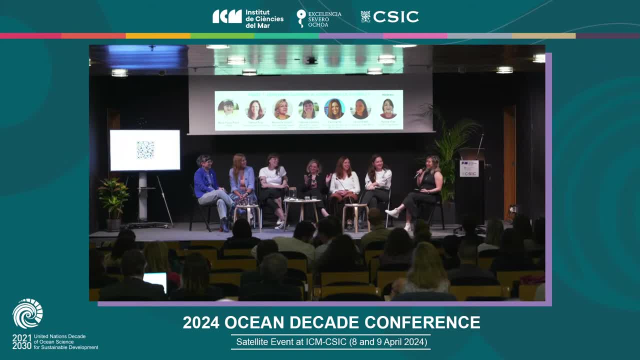 today. ok, with one question: are you prepared? no, it's really it wasn't. so we identified some, some common barriers on ocean literacy, and one of them is the generational barriers. okay, So we have seen many initiatives targeting youth, but there is a need to engage other generations as well. 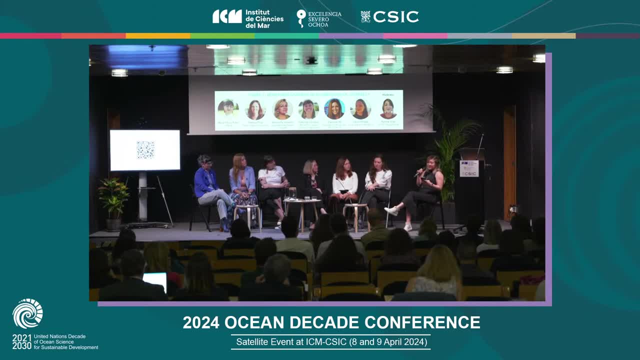 So how can educational institutions, community organizations and government collaborate to promote intergenerational dialogue and participation in ocean literacy activities? Yeah, that's a trick. a trick question. Shall we anyone? Okay, I always think that everyone here, everyone, everyone here. 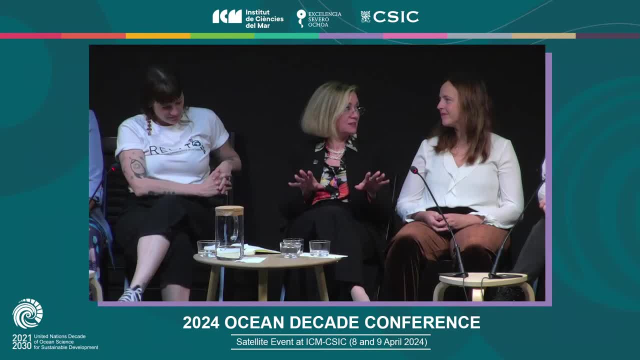 who makes any decision of any sort throughout the day has some deciding power on what happens with our world, with our ocean and with our climate. With that in mind, then, I think it's excellent, it's a good move to target all generations. 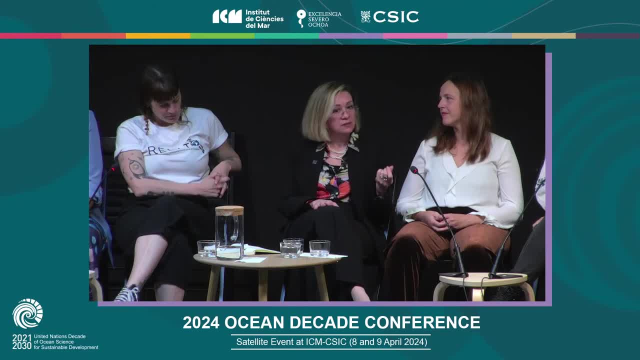 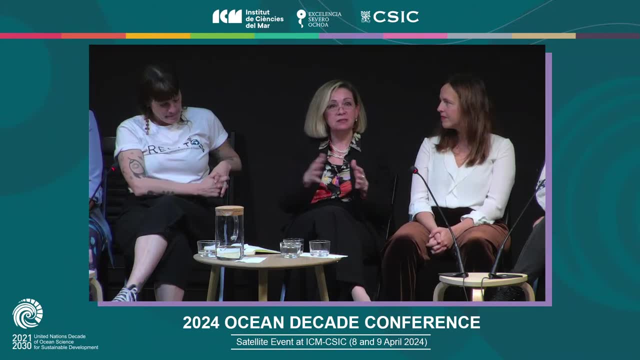 Whether it's the parents who hold the shopping power of the family, whether it's the children who are going to be tomorrow's leaders, whether it's the people maybe towards the end of their- maybe- careers and things like We all have. I think we- all of us- have a say in how things are going to be from this. 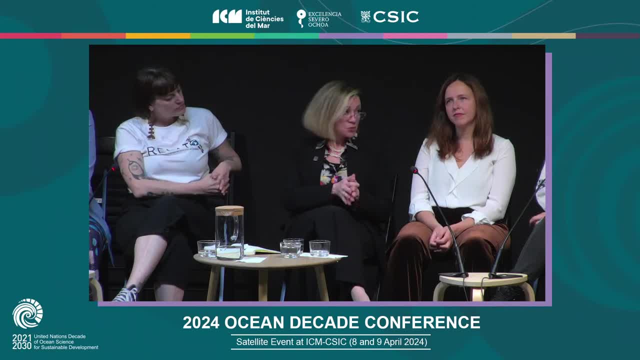 point forward every single day, And I think that's what ocean literacy is learning about: the impact of the ocean on you, but also your impact on the ocean. So anything that can give more information around that should be done. Each generation, policy makers, forestry people- it's all part of it. we can't leave anyone. 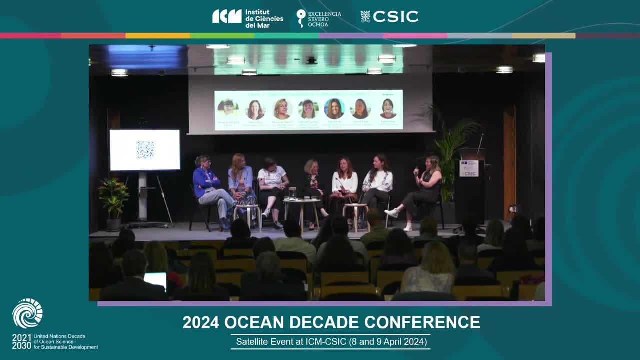 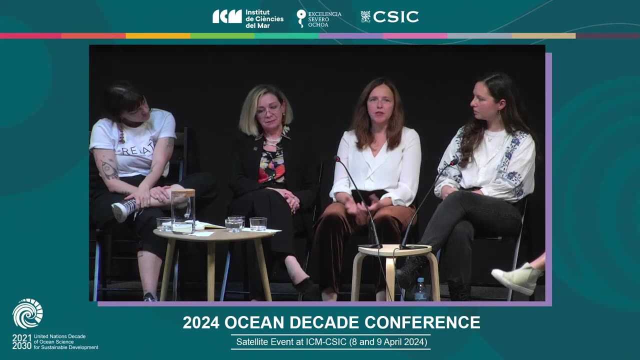 out right? Yeah, yeah, If I can come in. yeah, I totally agree with you, actually, and yeah, it's important to engage all the different stakeholders for the marine conservation and also find a common ground because of the interest of everyone for the ocean, for example, the tourism sector. 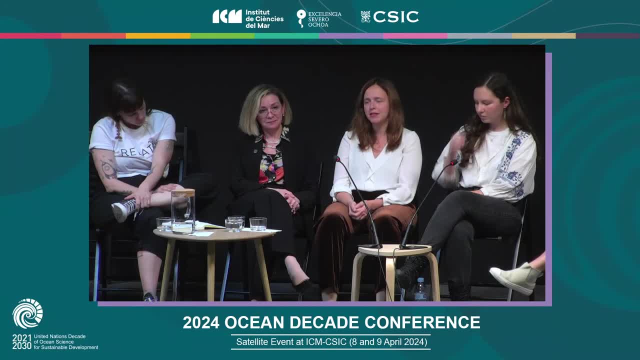 they have a lot of interest. They have the interest for doing activities in the ocean, but they also want to have it protected so they can keep doing their activities. So everyone you know I have to find a common ground. that maybe is not the pure conservation. 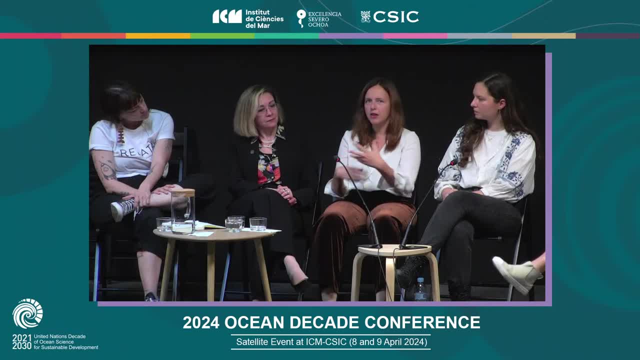 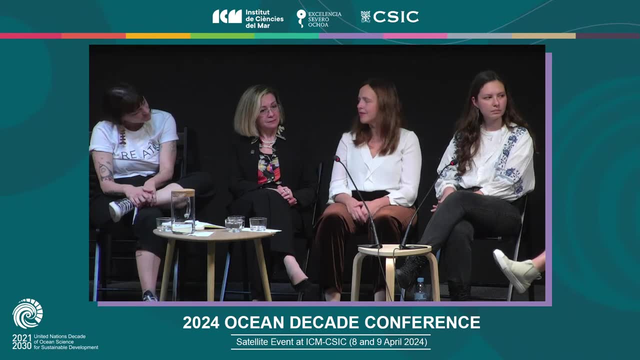 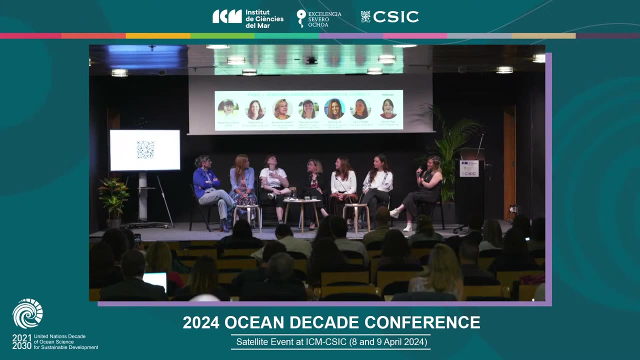 of the place, but is a good, proper management with the different stakeholders. So I think this is important to consider when we are talking about marine conservation and ocean literacy. Okay, I would love to add a couple of things. So I think that one of the, for me, the most important new ideas that I try to promote. 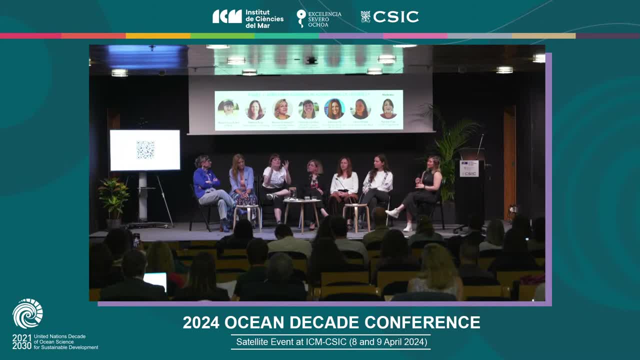 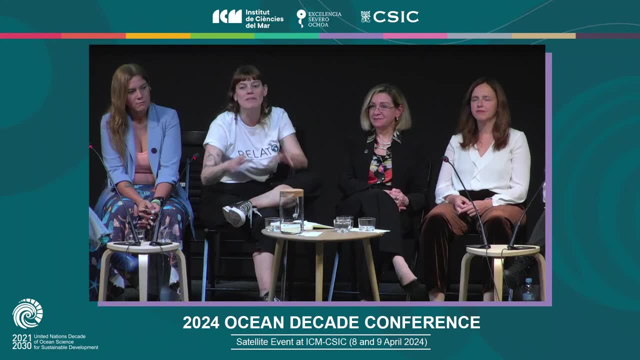 all the time and I will ask all the people here to try to implement. it's like starting to talk about the future generations, like, yeah, giving them all this responsibility about that we need to teach them because they are going to save the planet like we have. 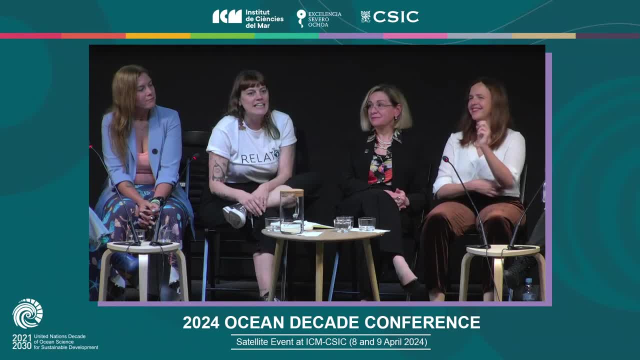 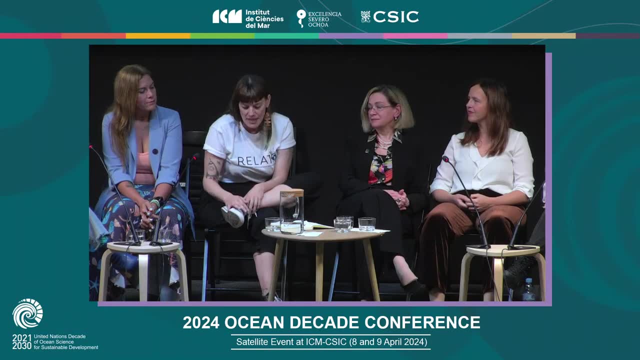 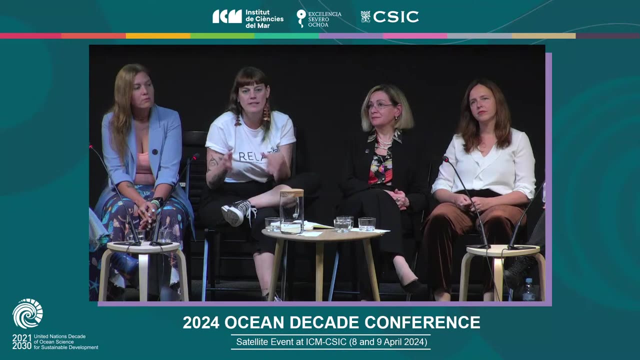 to stop with this speech and because of all the eco-ancity we are generating and all the ideas that they have, But also thinking about methodologies, like: first of all, we need to understand really well what is the context that we are going to work with, and it doesn't matter if it's 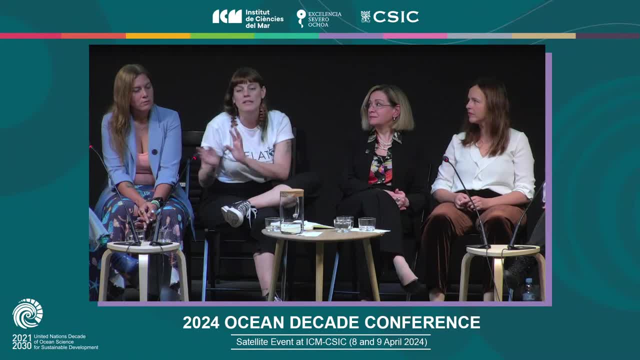 a fisherman or a fisherwoman or a policy-maker. but we need to really understand what is the public and then really understand their interest, because sometimes the ocean is not part of the interest. So how can we connect our interests and theirs and how can we design something? how we design? 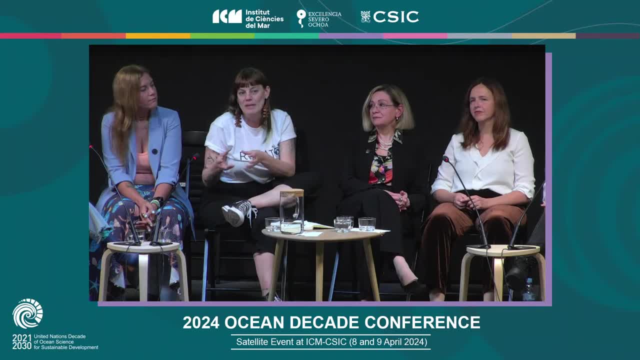 a methodology that could be useful, And thinking about that game is always a good thing to do, Okay, Even if they are adult people, because sometimes we think that, okay, they are a fisherwoman, we have to give a talk. 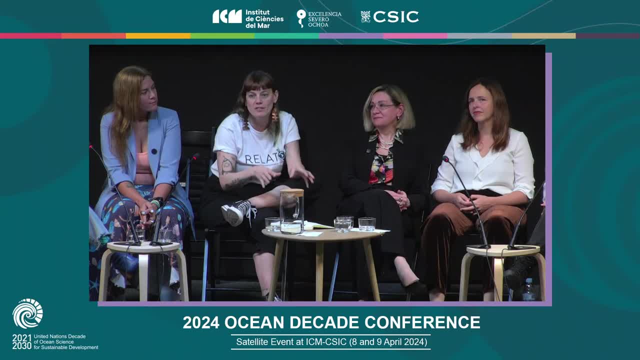 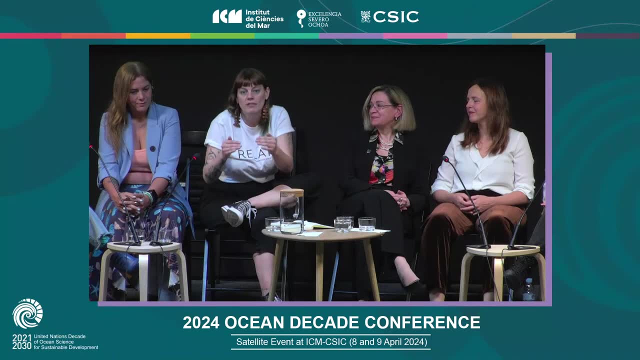 It's not a game, But we can use the same methodology for five-year-old kids and for 65 people in the community. exactly same methodology, different, deep in the knowledge. But we all want to participate in things that are interactive and give us the opportunity. 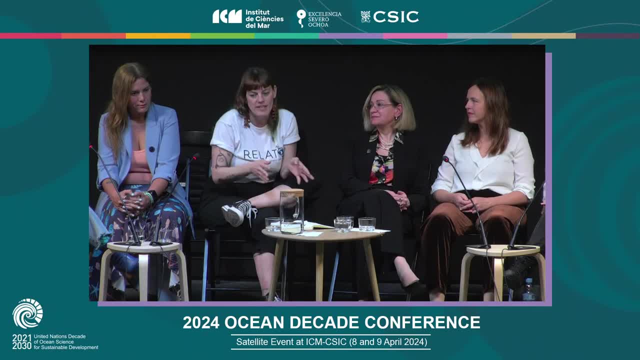 to think, to exchange ideas. So let's think about the context. Let's be very well-themed about this, Okay, Let's think about the methodologies we use and let's try to measure the impact, as Daniela does. Thank you, 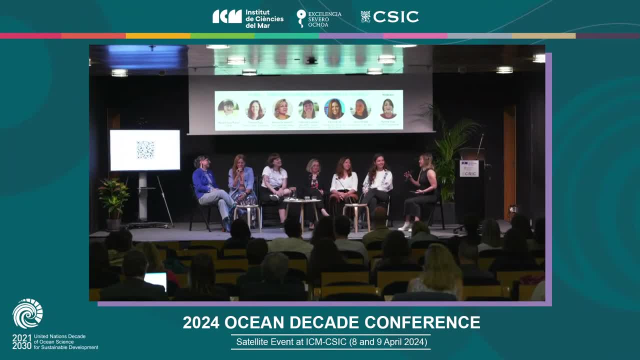 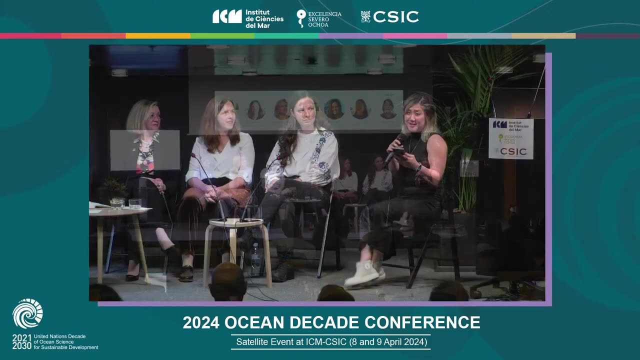 I'm sorry We don't have time. I'm so sorry, Sorry, No worries, But thank you all for your experience and ideas and hope that the ideas shared today will inspire for the actions towards a more ocean-literate society. Thank you very much for your attention. 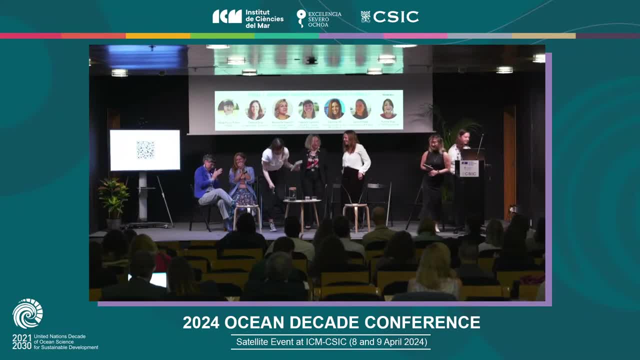 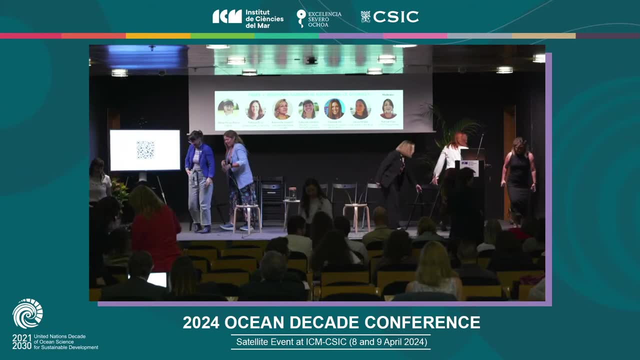 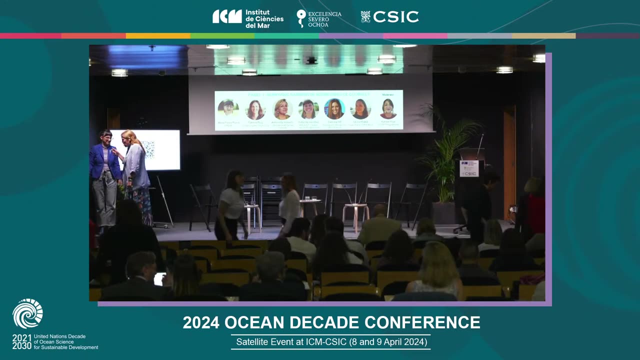 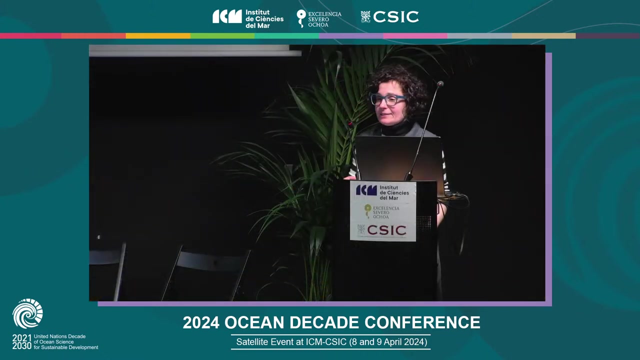 Thank you all so much. Thank you for these fantastic stories of examples of how overcoming barriers in ocean-literacy- barriers in ocean literacy. Now we'll have a slight change. We go to panel three that is about ocean literacy. 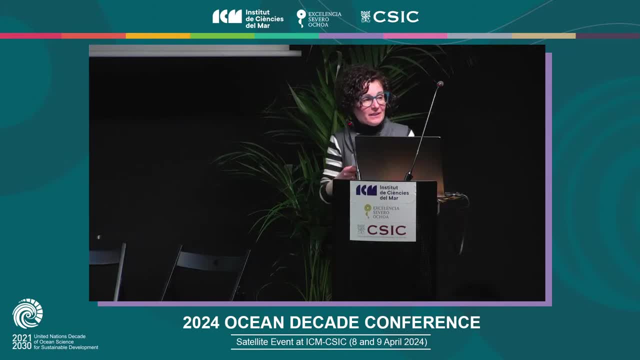 and ocean science. So I want to invite the panel moderator, that is, Giuseppe Luis Pellegrini, from here, from ICM, CIC, And then we have four panelists that are: Silvia Gomez-Mestres from the Autonomous University of Barcelona, Dine Parchina from UroGus, Donata Canu. 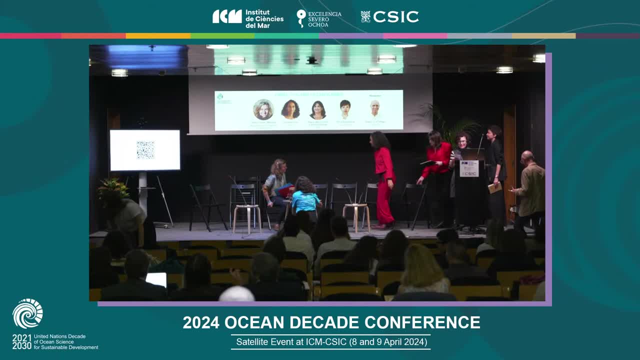 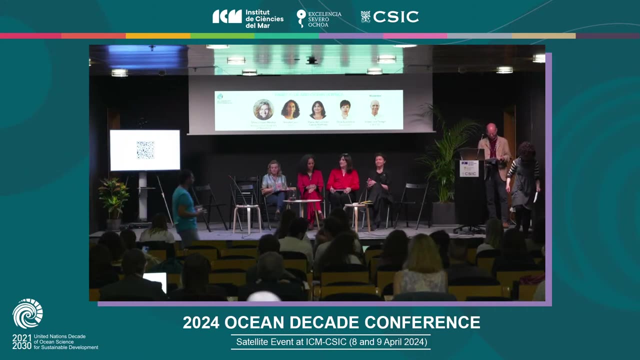 from the Italian Institute of Oceanography and Applied Geophysics and Maria del Carmen Garcia Martinez of the Spanish Institute of Oceanography. And please don't forget to check the QR code on the TV screen. OK, good day, I'll use these micros. 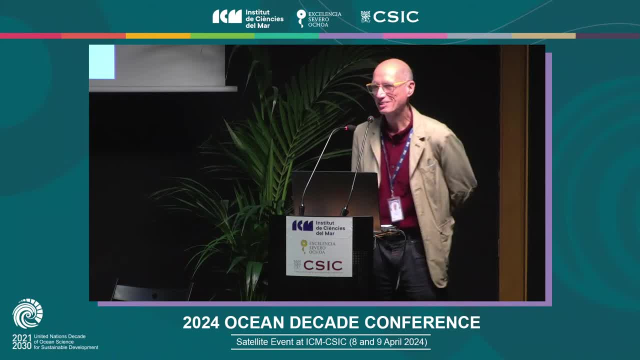 I think they sound fine. Well, it's a pleasure being here, this opportunity of moderating this second panel. I realize that I'm the first male that has appeared on a scene. This endorses our feminine side, which is what we all have to promote. 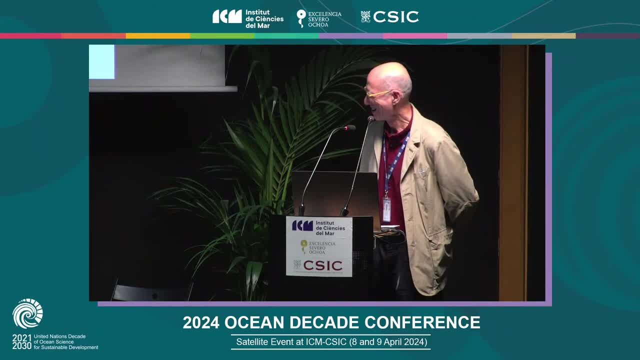 This is not exclusive Women, But also men. we can have this feminine and curator side, which is important. It's a real pleasure being here and trying to moderate this panel with these four wonderful scientists. They come from all fields, from social to natural sciences. 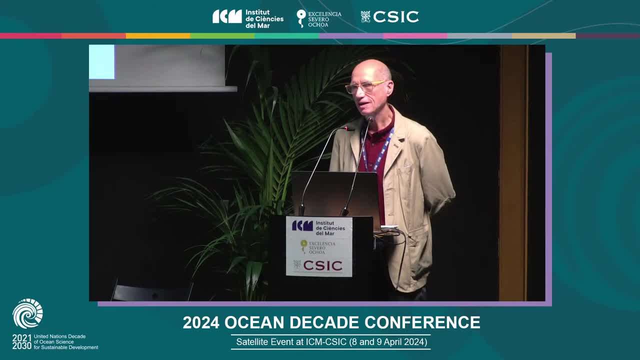 And they'll tell us a little bit about their experience related on how to promote ocean literacy from the scientific perspective. You know that in science we probably don't have a preparation on communicating ocean literacy. We don't have typically these backgrounds. 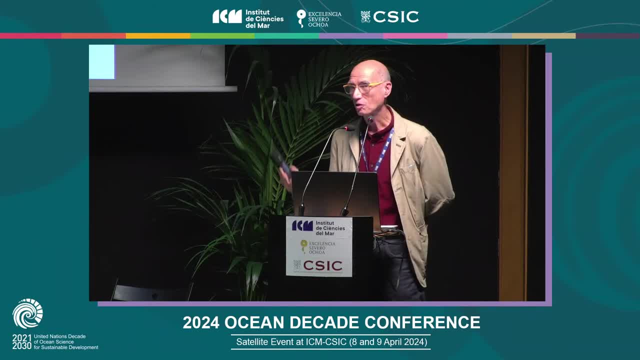 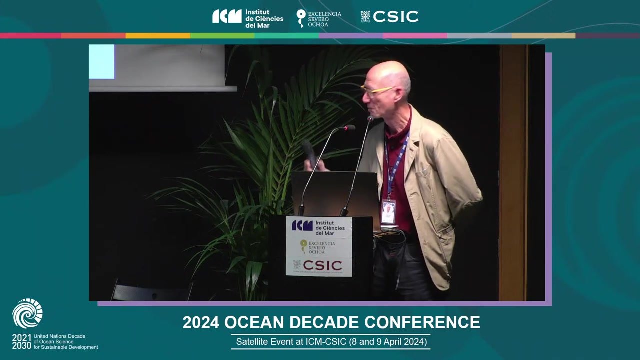 Our background is in natural sciences. We also don't have typically the resources- Projects that we handle are of limited extent in time And we don't have the structural resources that agencies- especially the agency levels- And further, usually these type of tasks. 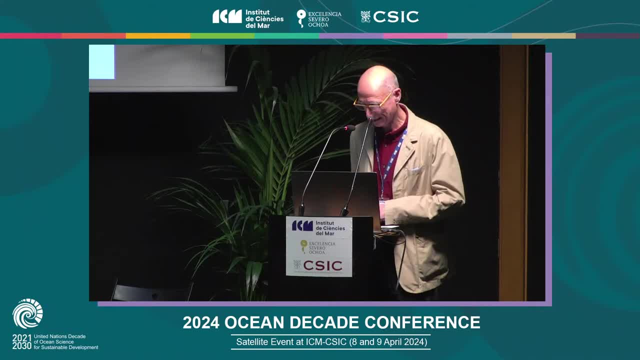 are not positively evaluated in the evaluations that represent our promotion. So it's great having them here and seeing their experiences on how to promote ocean literacy from the scientific point of view to the general public And scientists as well. We also have to get into that direction. 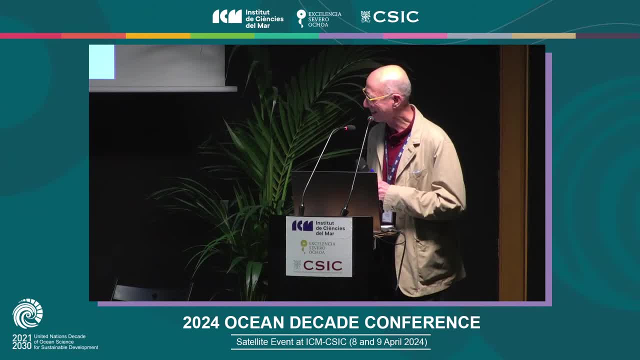 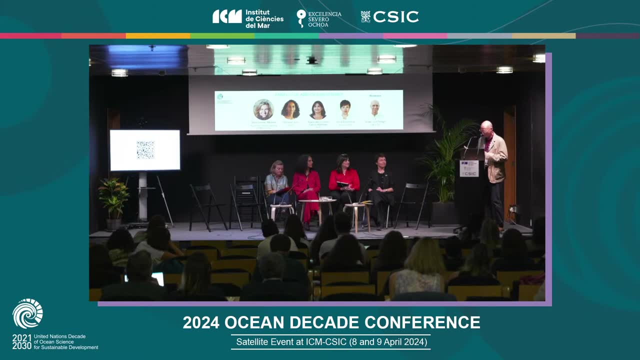 So our four speakers are: Dina Eparquina: She's a specialist on science policy stakeholder mediations. Mari Carmen Garcia, marine biologist and currently director of the Institut Espanyol de la Serrafia, the largest Spanish marine institute, and very much engaged in ocean literacy and communication. 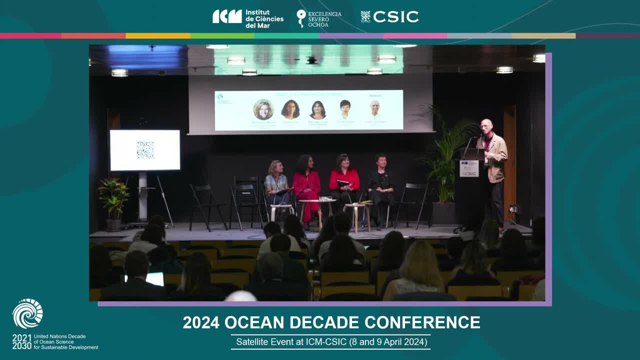 And Donata Cano. she's a marine ecologist with an emphasis on anthropology, the connections between the, the land and sea. and far, far far from me is Silvia Gómez-Mestre. She's a social anthropologist specializing in coastal communities. 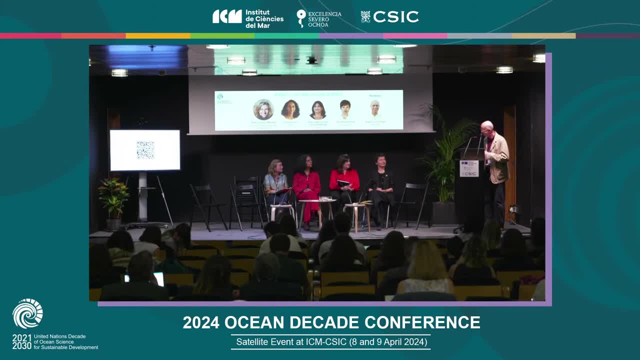 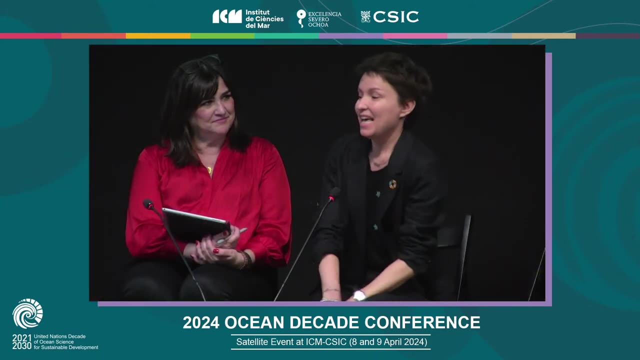 So I'll start with Dina. please, if you can explain what is your success story, how you transmit your this ocean literacy from the scientific point of view, Thank you, Thanks very much. I'm a marine ecologist. I'm really delighted to be here and representing URUGUS. 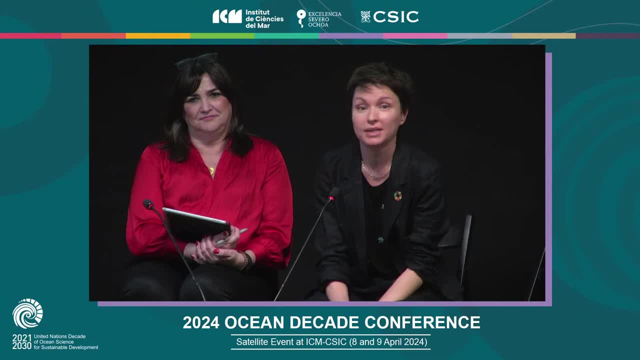 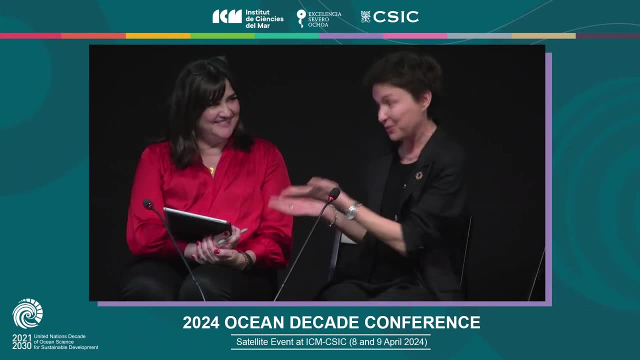 European Global Ocean Observing System and we have a working group and a decade project which is called Scientists for Ocean Literacy and Working Group on Ocean Literacy, And I'm happy here to share the stage with three- two other members of our working group. 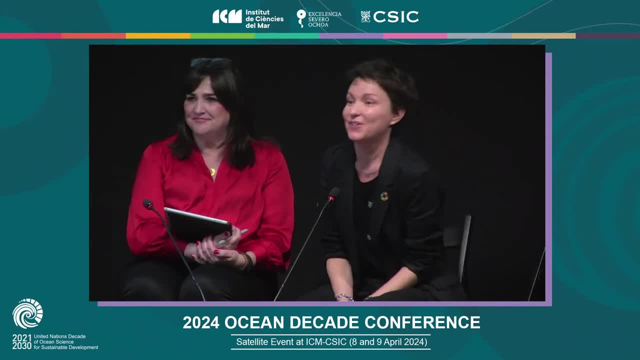 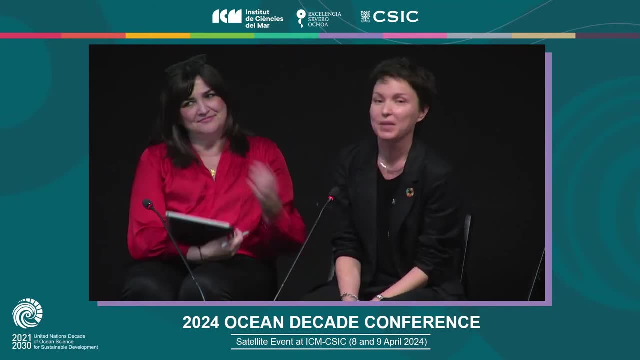 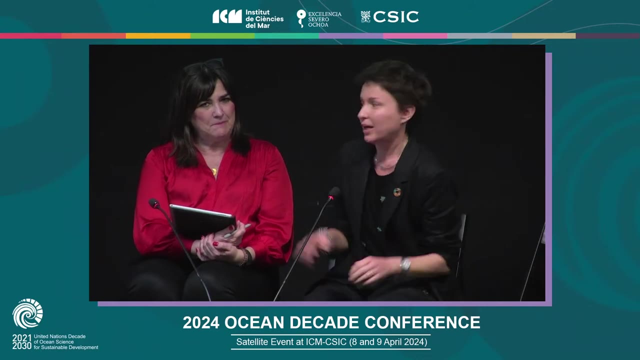 Mari Carmen and Donata, and kudos to Norin as well, who is in the room, who is another member of the working group. Overall, we bring together 25 organizations in Europe and what do we do together? We actually try to promote exactly that: that ocean literacy is not where only women are involved. 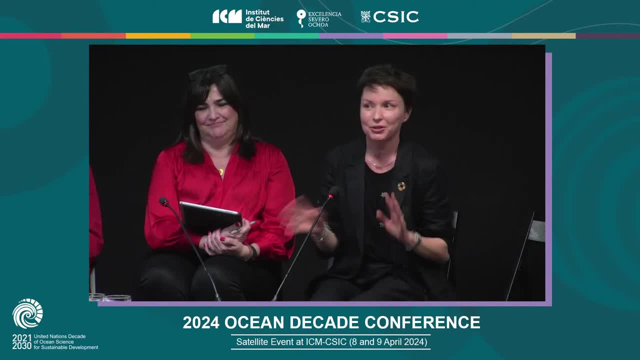 because they are caring for everything and they can make choices against their careers sometime. that ocean literacy is really accessible, really accessible in general sense, And I was really inspired by some of the examples in the previous panel that we reach out not only to people. 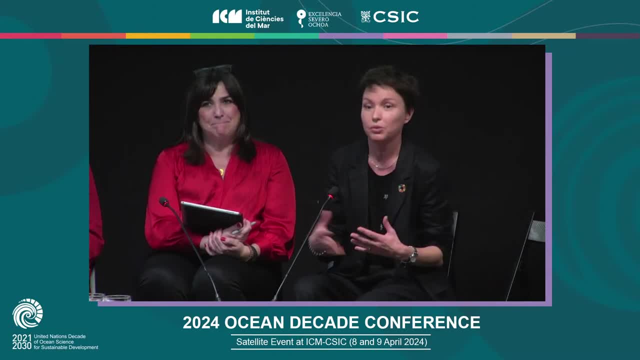 in their family time when they don't know what to do with their children. but we really work with professional environments, with guards, With governments, with local authorities, with businesses. that we also train scientists and involve scientists, encourage scientists to become ocean literacy advocates and champions. 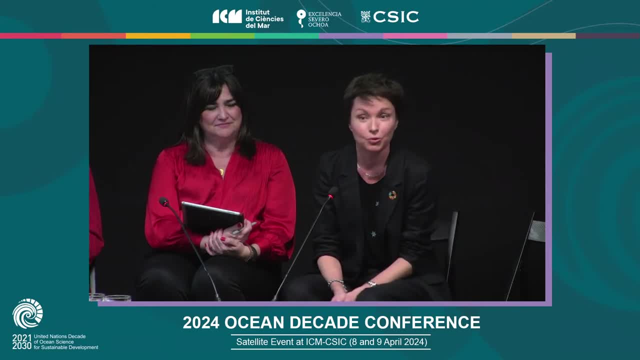 that we are not, you know, shoemakers whose children are without shoes. As scientists, we also feel ourselves empowered and recognized as ocean literacy actors And, of course, the career element is very important. It comes also with lack of funding, lack of recognition of ocean literacy as a strategic activity. 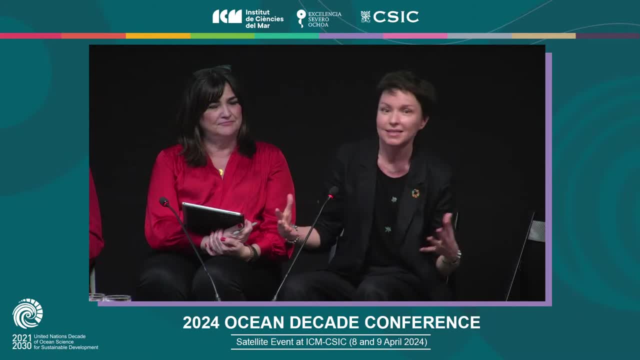 even though it is so sexy and attractive- and we hear it a lot now in scientific context- In reality things are: people are not so easily involved because it is not helping them to build their career, to have influential articles and papers published, et cetera. 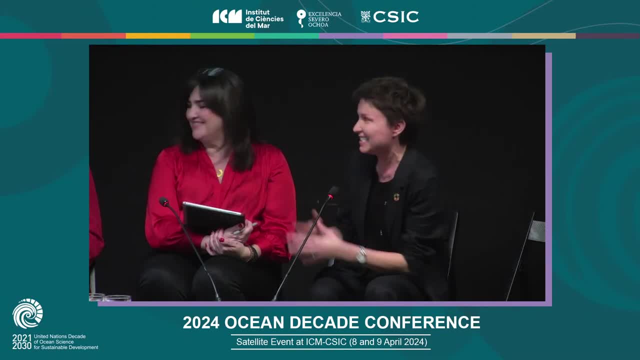 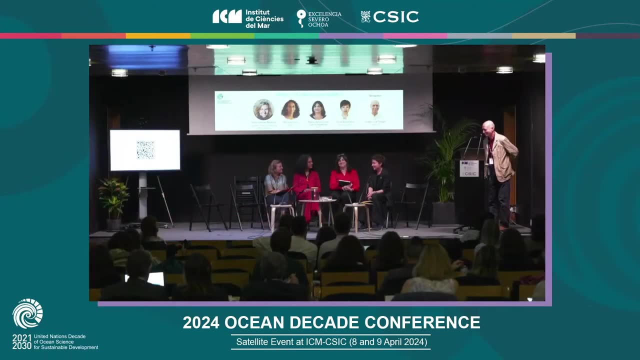 So here we are, and I'm really happy to have this discussion with Joseph And all the panelists, so looking forward to see what the others say. Let's make this flexible. That sounds wonderful, Maricarmen, go ahead, please. 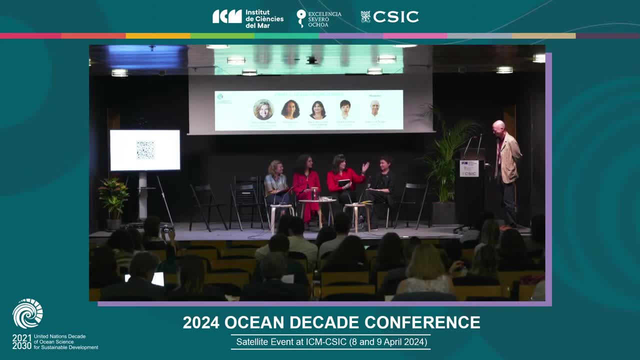 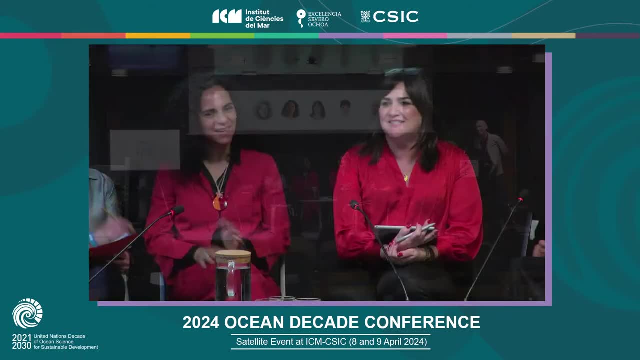 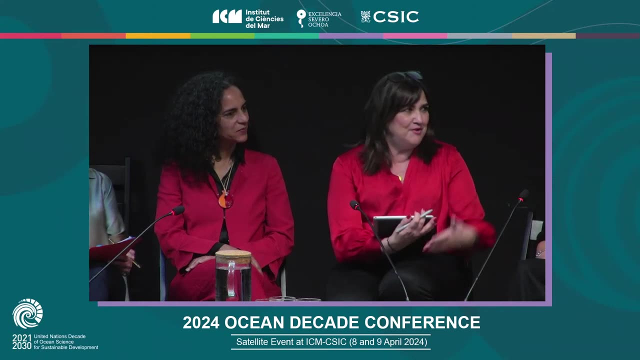 Hi, Thank you everyone, and thank you for having me And congratulations, Joseph, because you are the only man at the moment, so I don't know why There are many, many, many in the audience. There are a lot in the audience, but somehow I don't know why women are really more involved. 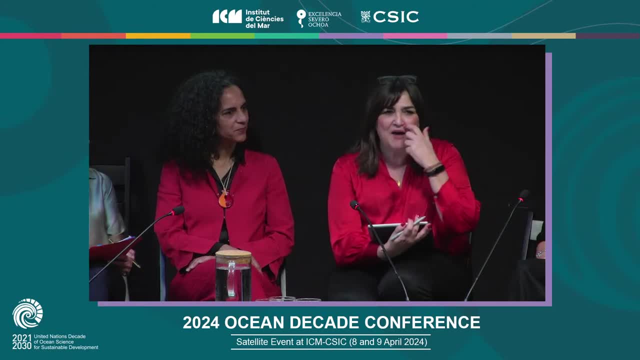 in this, so maybe we can change this Somehow. we have to work on this. I want to talk about one special project, that there are a lot of them in the Spanish Institute of Oceanography. We are around 850 people. Probably you know many of our projects. 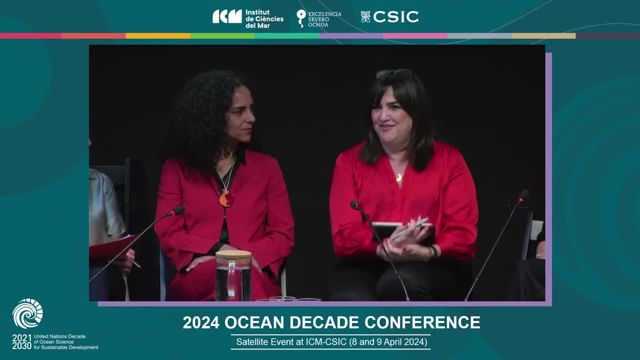 One of them is that is really famous because we try to talk about women in marine sciences, But today I would like to talk about another. one is called Mariona. It's a specific project that is held in the north of Spain, in Gijón. 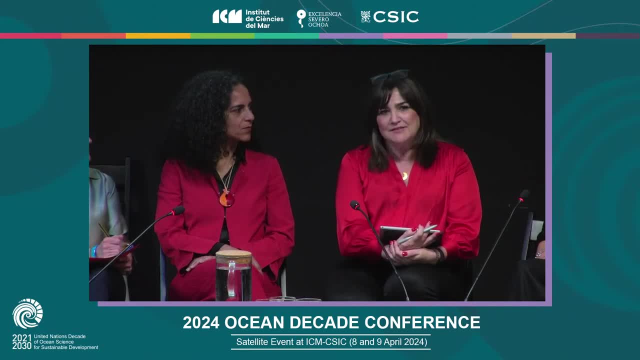 It's, And we noticed that we had some problems because if we have some open days in our institutes, they're always the same schools, because there are some specific teachers that are really interested in marine sciences, for example, And we decided to do something different and to bring or to take our institutions to the 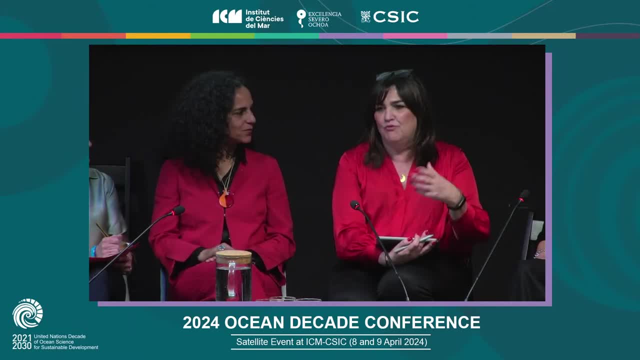 streets, to the neighborhoods, but not only to schools. We work with schools. We have some scientific projects with the schools, with children 12 to 14 years old. We have some specific activities with them, with the smallest one, But we also, during the same time, at the same time, we are doing some activities at the school. 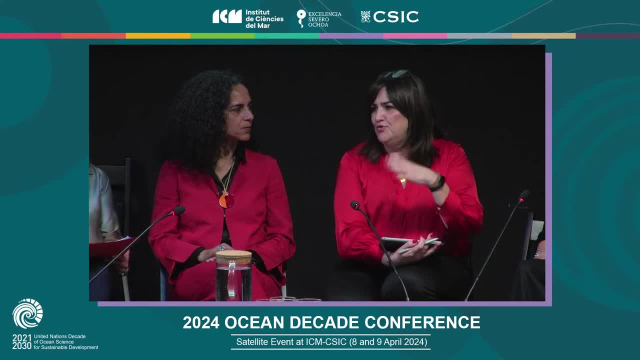 we are doing some activities in the neighborhood. For example, we use the shops. You can use the screens, the windows in the shops to send some tricky messages, interesting images, just to say the ocean is here. You can learn a lot about that. 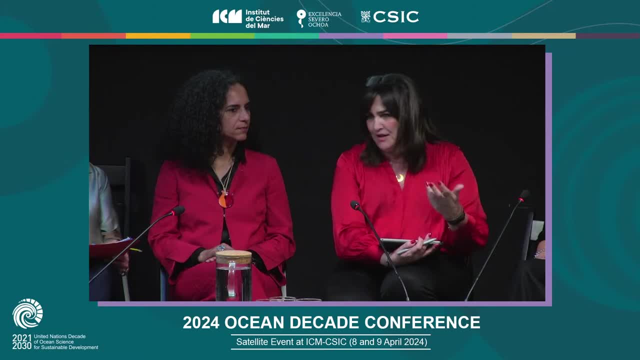 You can learn about marine pollution, biodiversity, climate change, anything. It's very interesting, Thank you. And at the same time we also give some talks in some specific places with the children that they are doing some specific projects in the school. 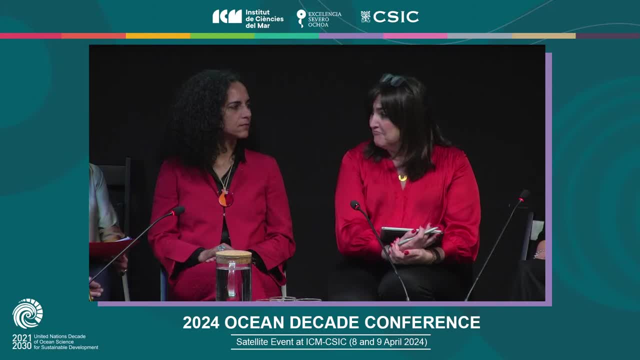 So I think it's a really nice project. We are really happy about that and we are searching just to see what is going to happen in the future, But I'm sure we will have perfect and really really nice results. Thank you. 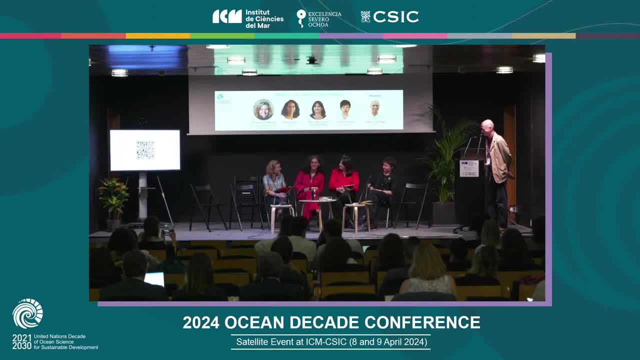 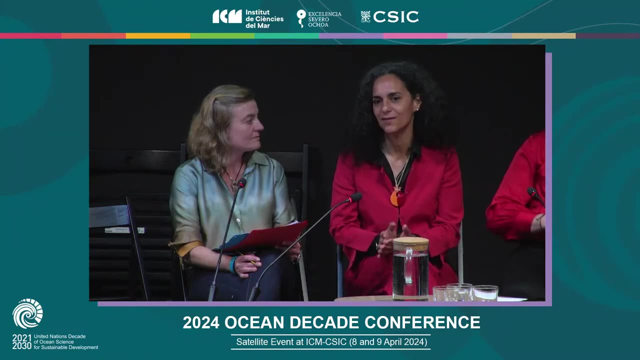 Yes, Go ahead, please, Donata, It's your talk, Sorry, Okay. So first of all, thanks for the invitation. It's a really pleasure to be here and to hear all these examples and stories about what we are doing for the ocean and for transferring the information and getting the information. 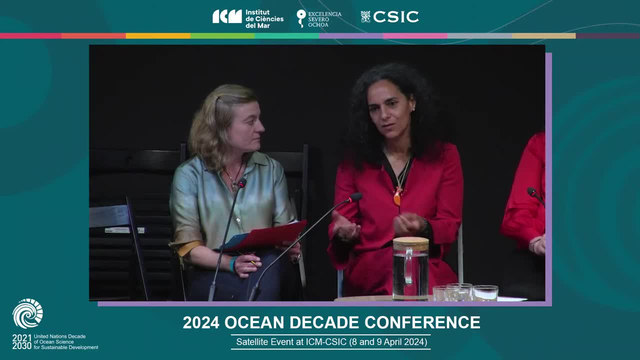 also from the people that are in the ocean and so creating this link between us and the ocean. And I'm from Italy, from the National Institute of Oceanography and Applied Geophysics. Our institute has a specific department that devotes to the research in the ocean and the 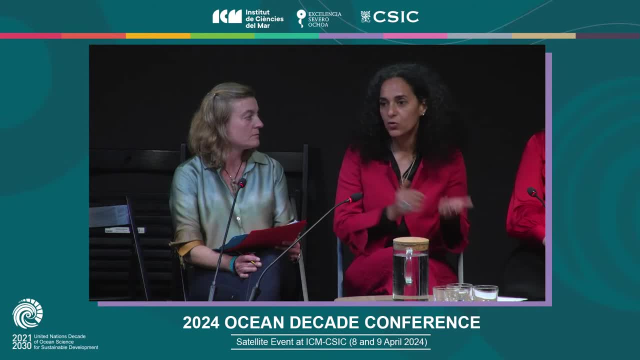 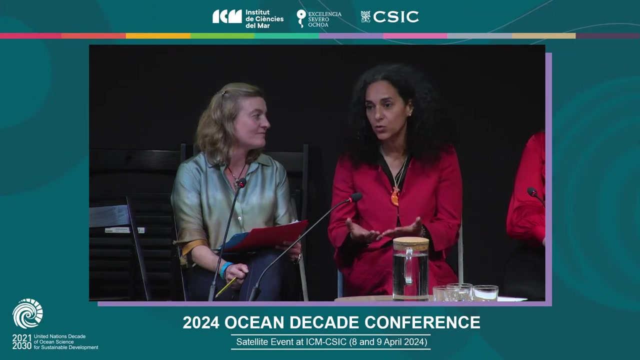 sea from the different perspectives, so biology, biogeochemistry, physics, with observations, modeling, so hard science. In recent years, we were more and more engaged in ocean literacy, not only because somehow it is also requested by the projects to engage with the stakeholders and with the institutions. 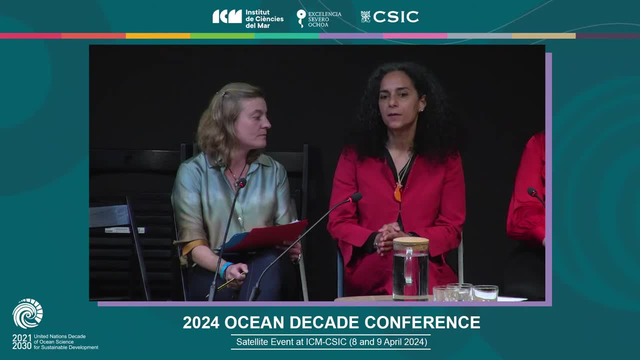 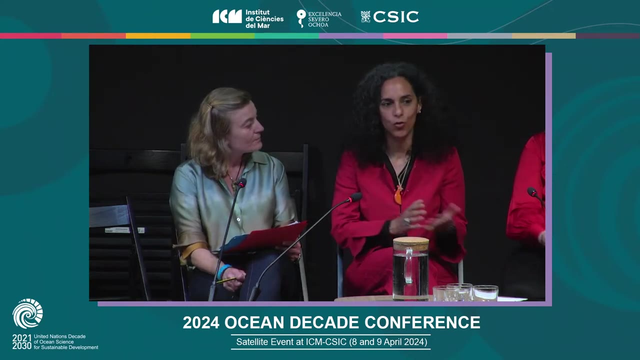 with the enterprises, but also because we really believe that it's a key to improve the conditions of the sea. We did a lot of traditional talks and seminars in meetings with schools- often the same schools, because those that have teachers that are more willing to participate. 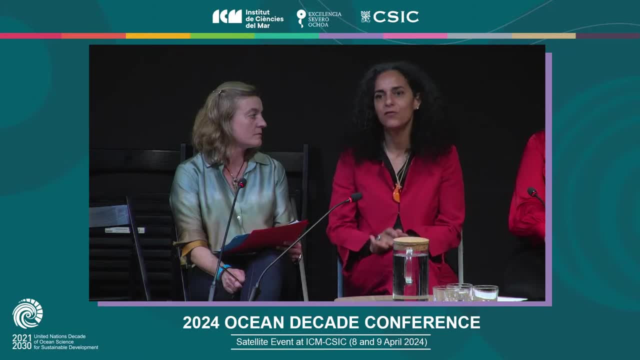 But what I want to present here briefly is a festival that is now at the fourth year that is done in Trieste and in the wider region. This is a city located by the sea, but the festival was done also inside inland meaning. 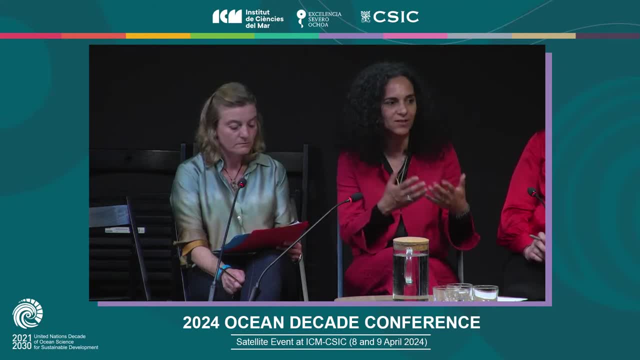 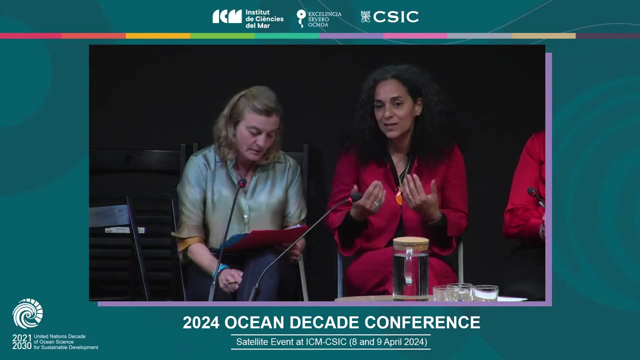 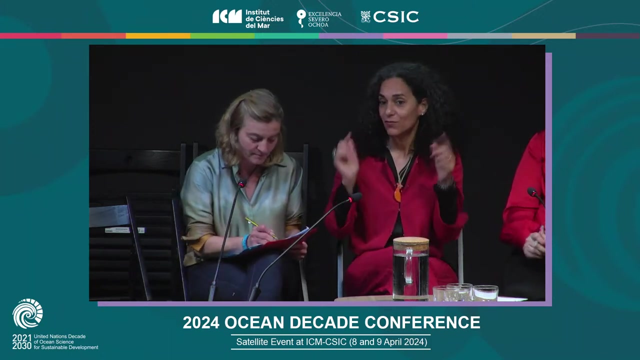 to connect the land and the sea toward this turquoise ecology. So the festival is called Mare di Refare. that recalls a very silly game that we did as a child. in Italy People learned the game when they were children. it shape their wife into little animals because 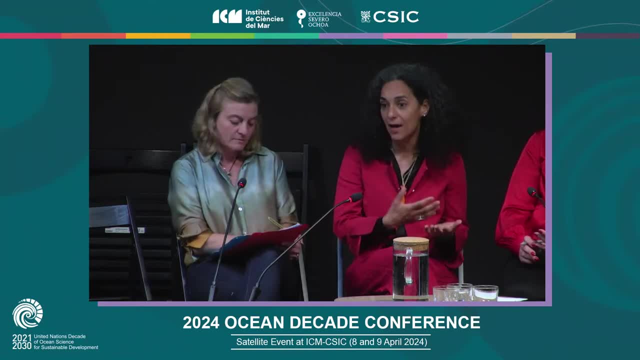 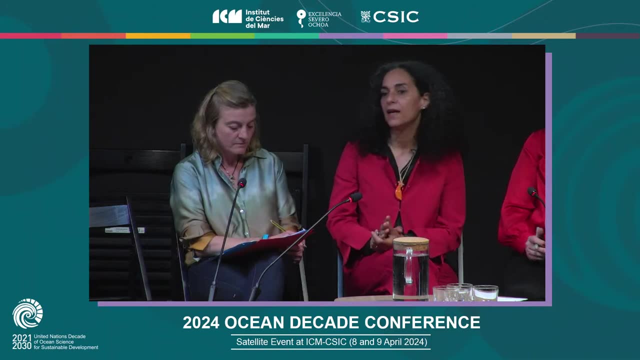 they love this game. There were also art, about art and the disabled. you can easily get the words pretty cool for helping the disabled and the late 40s. You can refer to SCHS Venedicti in the objective, in which things in the game by one side ceλ. 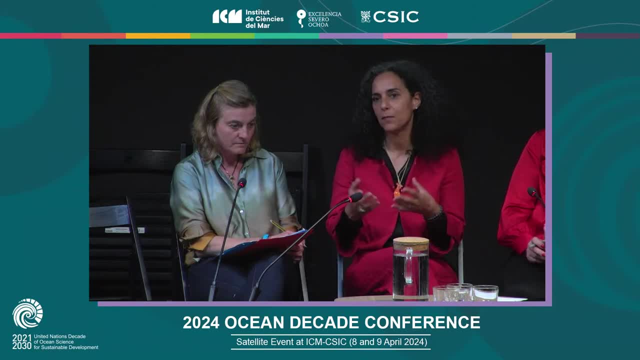 aE. aE- So just starting from the name- is something that has to do with the game and with art, Because these festivals, in the different four years, engaged with artists to promote, for example, exhibitions, Art- Warm Dawns, exhibition's that were then moved around in the libraries. 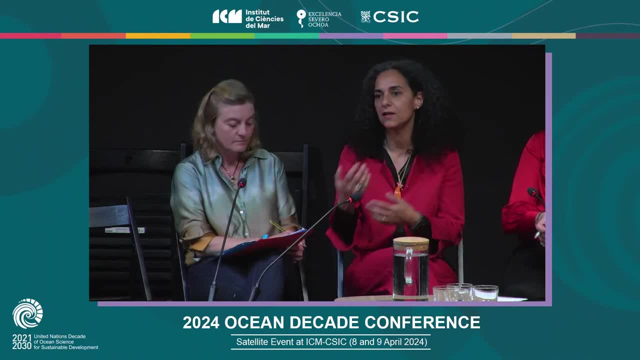 in capabilities, in so that asamen Blues or Des IRSRA's 걸�ies are considered to be fun in cafeterias and so on, to go inside to do to improve the connection with the city. and, of course, we had also traditional talks focusing on different topics, topics, topics that are less 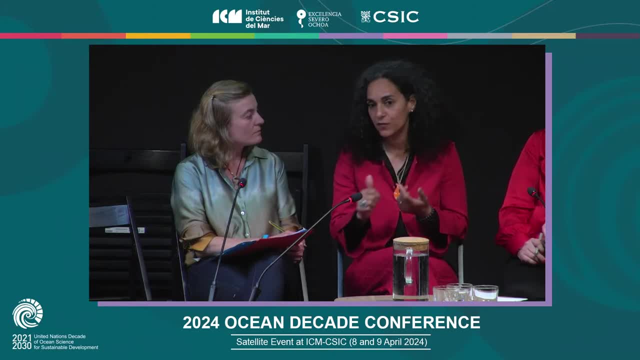 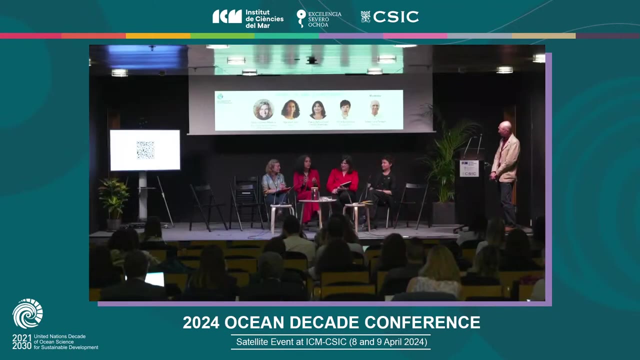 recognized, like, for example, the microbial life in the sea, the deep sea, and the topic that means that the the sea starts in the cities. so these were the topics and these were the ways that we in place to try to improve this ability to communicate, because it's not very often easy. 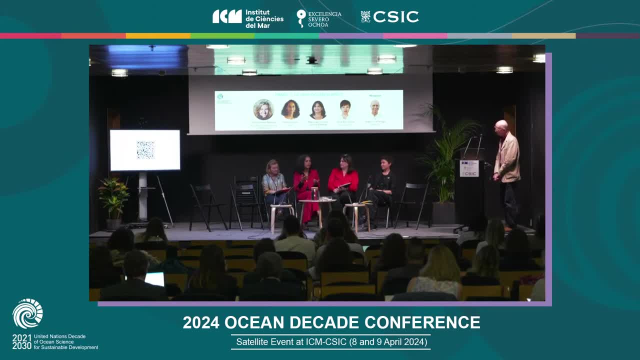 to engage people, especially in town that are very exposed to events related to the sea, as Trieste. so we really need to to engage also with people that are are able to engage with the emotions of the people and to improve the connection. sorry, I get, I was wrong, thank you. well, so we moved a little bit from the stakeholders and 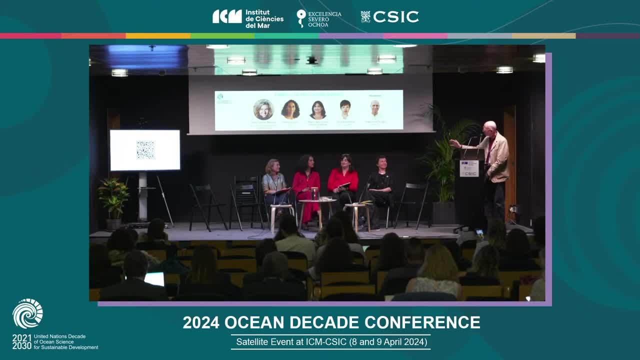 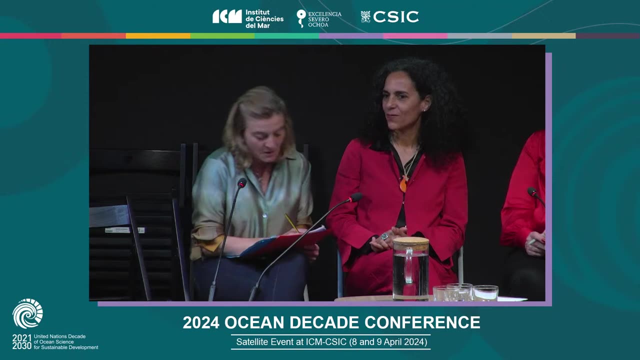 the national agencies to these public spaces and this communion with people through festivals and actions. and then, I think, Syriza now tell us a little bit about her experience using new technologies like the digital platforms. digital platforms- yes, well, I'm gonna talk about the digital platform that we have. 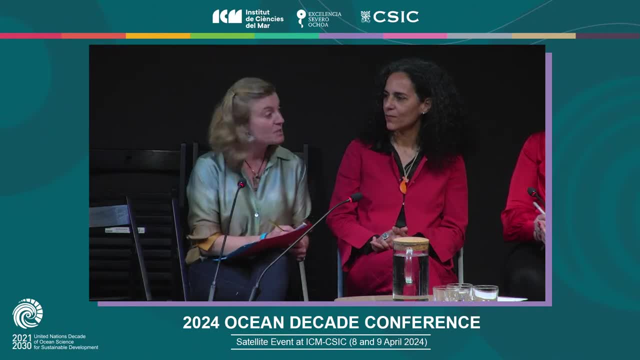 designed in the frame of a European project, empower us. and well, it's called a natural cup and it's for learning about the marine protected area of Cap de Creus. and we use this digital platform platform as a tool for ocean literacy and knowledge sharing, but to foster action oriented. 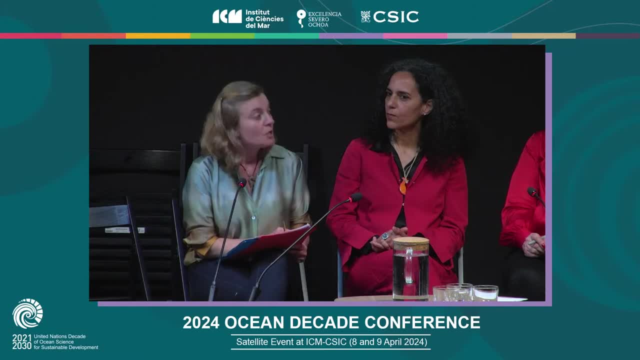 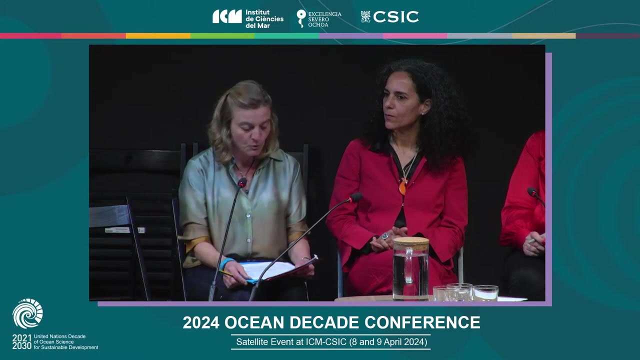 knowledge, that we think that is paramount to be effective in ocean literacy. digital platforms make it possible to reconcile scales of knowledge at the crossroads between social and natural science and to make society an agent of change. because I think that we think that ocean literacy has to be this purpose: to make society an agent of change, for changing um, the our, our. 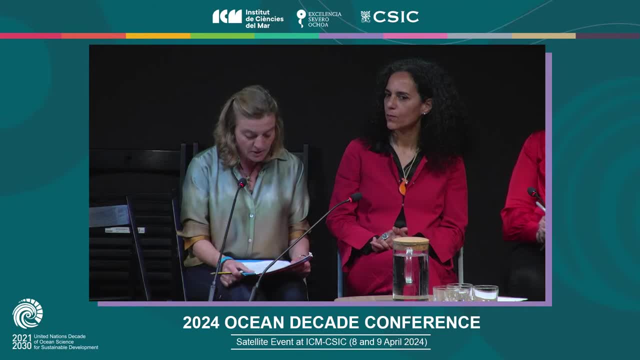 to relate with the ocean, uh. so uh digital platform is uh effective because uh can go beyond geographical or physical, cultural and social boundaries, and uh then allow us also to incorporate a new idea of science, more or less uh we produced previously to the design of this digital platform: knowledge. 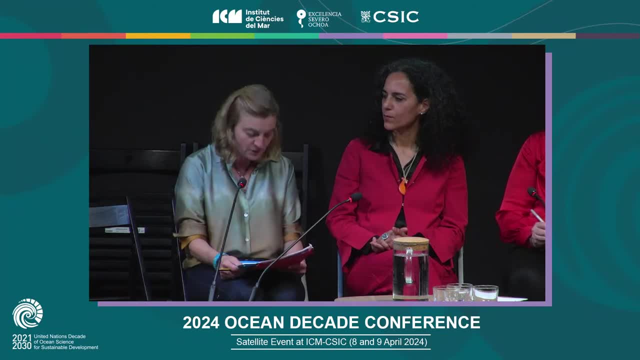 assessments in the marine protected area of Cap de Creus. uh this knowledge assessments showed that, regardless of age, income and level of knowledge, it was the conservationist ideas and the value of cultural uh embedded in natural heritage that was paramount to foster pro-environmental behaviors. that may change the 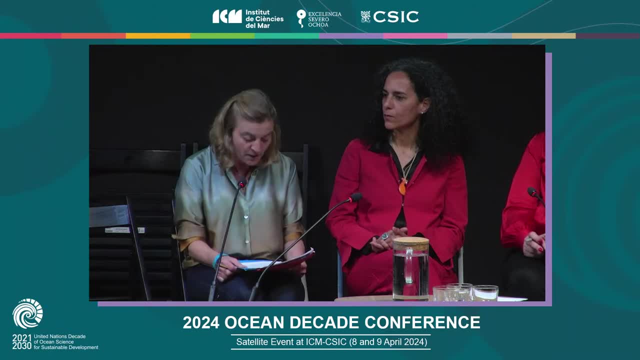 way we relate to the ocean. so, uh, this is the the idea of action oriented knowledge that claims for this holistic integration of social science and natural science, considering science as one marine science embracing different forms of expression, either art, late knowledge, technology or assessments in a laboratory or modeling. so science, we realize that that should be understood as forms of knowledge. 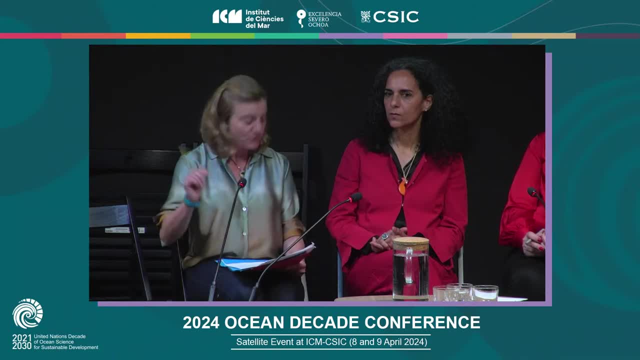 in plural. that necessarily refers to different scales, from the local to the global understanding. the local, well, this subjective, uh um, expression of the, the nature of the environment, of the ocean, that is qualitative, this is the tangible dimension that has to be articulated with this understanding of the global effects of human beings on the environment. that refers to the objective, the. 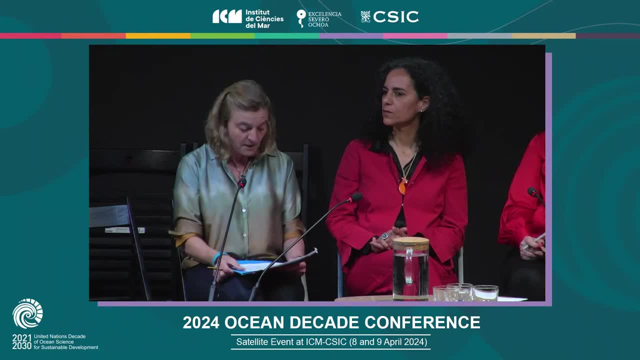 quantitative, that well, is the intangible dimension, both dimensions, uh, we realize that that is uh 보다. well, we realize that that is. you know, we are all related. but so i just want to jump back a bit and to bring this back to the point that i think, uh, you realized that there is a question, that, uh, 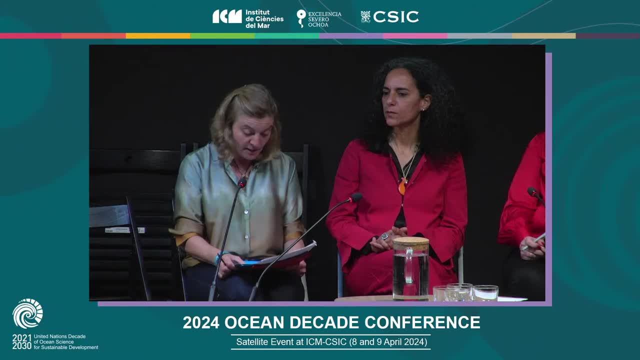 is another point that we wanted to transmit- is that being literate, uh, does not necessarily mean being respectful of the ocean. it is also necessary to change our conception of nature. to change- this is another point that we wanted to transmit- is that being literate, uh, does not necessarily mean. 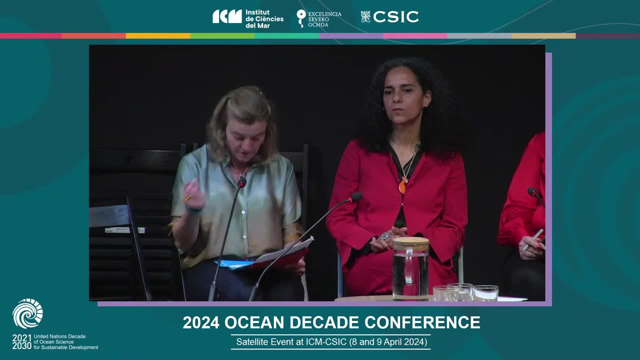 our reception of nature to change this way. we relate to the ocean often. uh, western societies have an idea too much anthropocentric of the nature. and you will say, wow, as social scientists are not left alone, as we are connected with our cultures or even ourwritting villages or tribes. 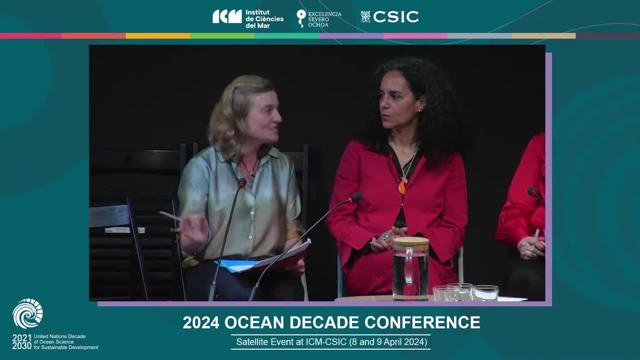 because we have the connection of our social and cultural people to each other. so we can have a iad, for example, like a certain social connection because we have a mother and we have a law that is equal to a. a social anthropologist saying this: Yes, because indigenous people are not so anthropocentric. 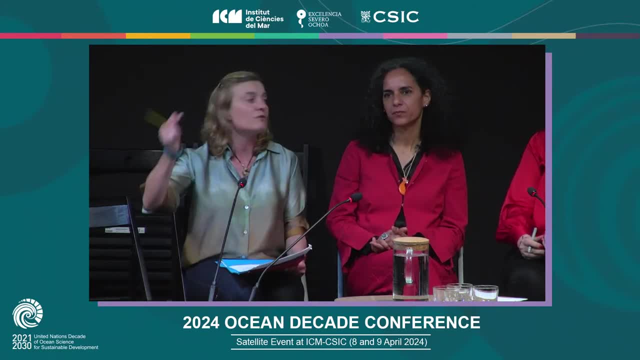 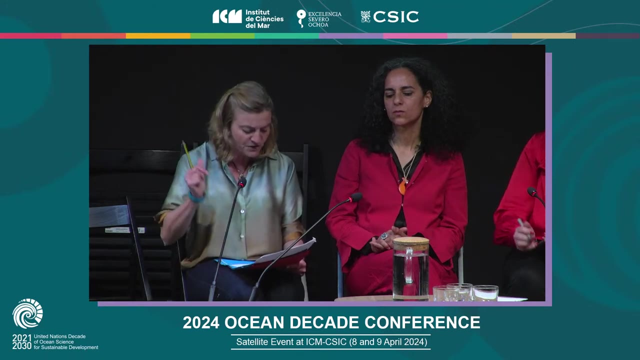 because they have another way to relate, according to their cosmologies, that is more reciprocal with the environment, with the ocean. So in our societies we have our society, in Western society we have the idea of the ocean as provider of well-being. 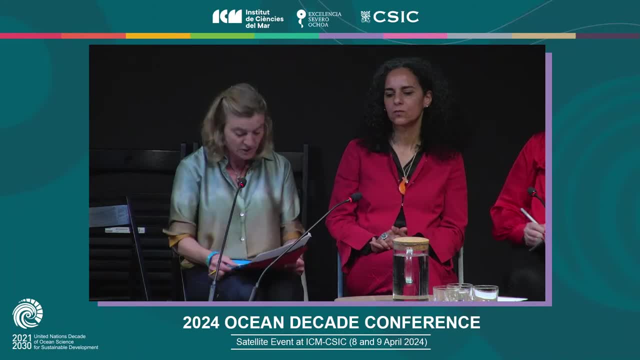 But what's well-being? So we need to change also this conception of well-being, rooted in the comfort leisure values typical of Western society that is partly linked to the idea of nature consumption and dependent on the consumption of our planetary resources. We need to produce this ecocentric turn. 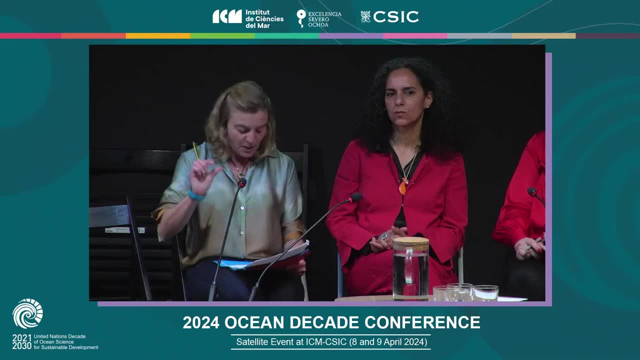 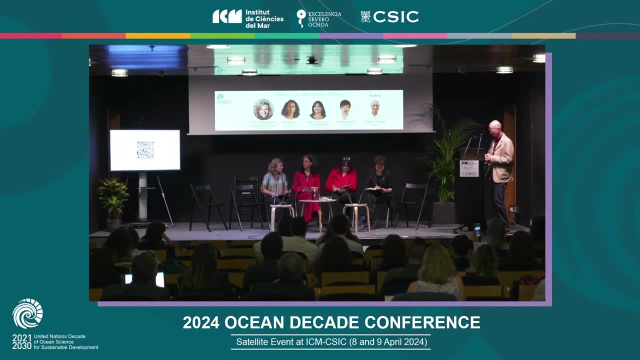 to become more indigenous in the finitive, to blur this human nature divide together with its hierarchies, because the human nature divide implies hierarchies. So this is what we try to produce with this digital platform. Mariprotected area is not for fun, it's for protecting. 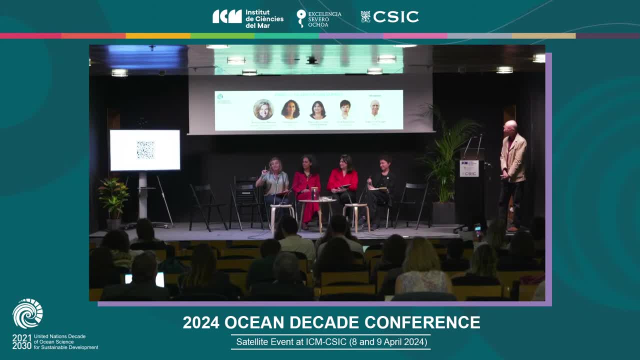 So we have to bear in mind this. So this implies, as I said, to change this conception of well-being and of having fun. So we have to have this change in the environment, in the ocean. So, to conclude, I think that the moral and ethical angles 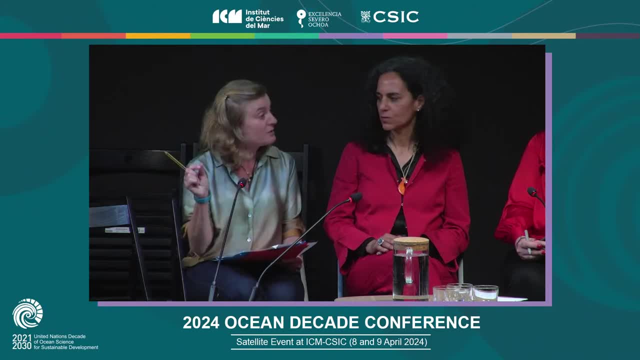 of our relationship with the nature are those principles that can unite social science and natural science, despite differences, despite different approaches, despite different ways of understanding the science. I mean, that is, these principles, moral and ethical principles- that unite both the social science and the natural science. 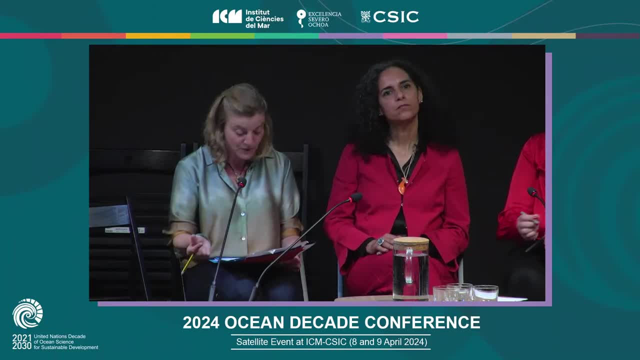 And we need to work together in defining these ethical and moral principles. Also to rethink science from a transdisciplinary approach, And this has to be integrated in this idea of ocean literacy, overcoming the old dilemma between science and lay knowledge- subjective, objective, quantitative, qualitative. 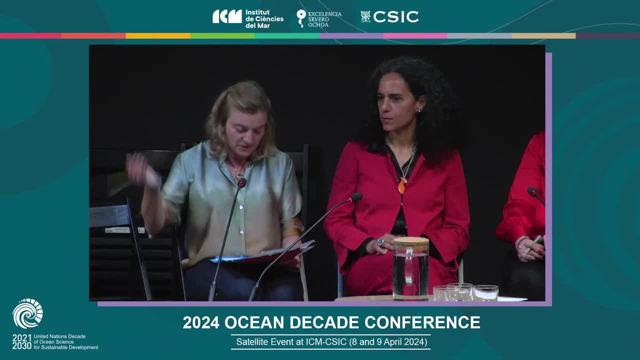 indigenous or local community knowledge or science? It is not a question of which is the true science, but which is the science that can produce action-oriented knowledge towards sustainability. That is our purpose in ocean literacy. With knowledge alone, it's not enough. 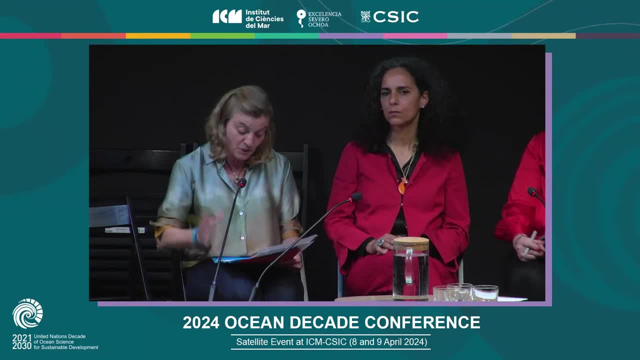 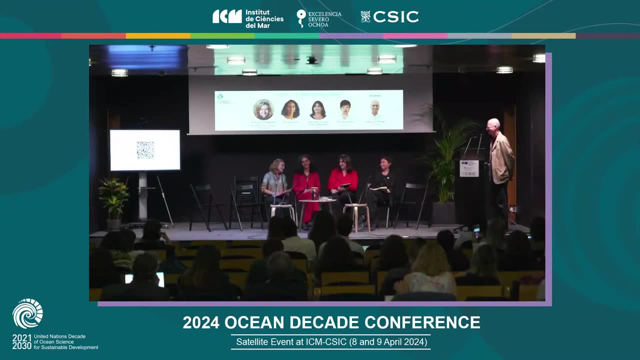 So we must produce this changing. Yes, so well. this is what we try to produce with our digital platform, NatureCap, that you can already download, And in the poster exhibit there's the QR to download and to start learning about the Caldecreus marine protected area. 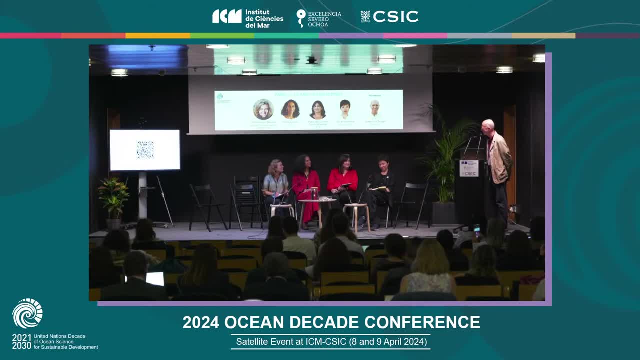 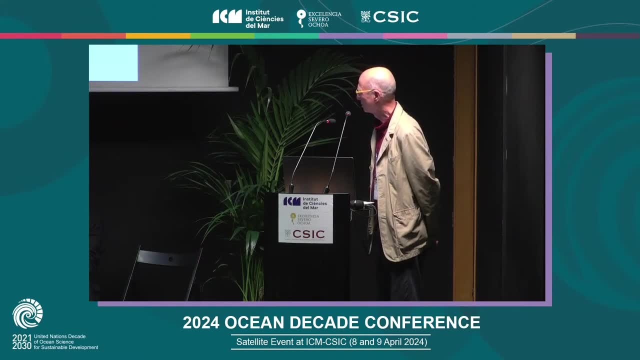 Thank you, Silvia. I think you raised a very good point for the other three speakers to discuss. What is really science? What is really intelligence? Can we talk about natural, ocean, earth intelligence that is much beyond our mental cognitive part, the way we interconnect. 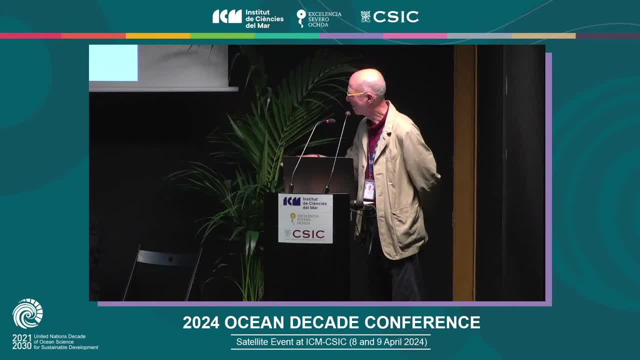 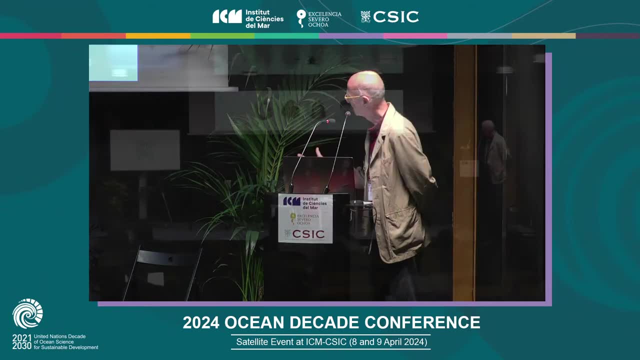 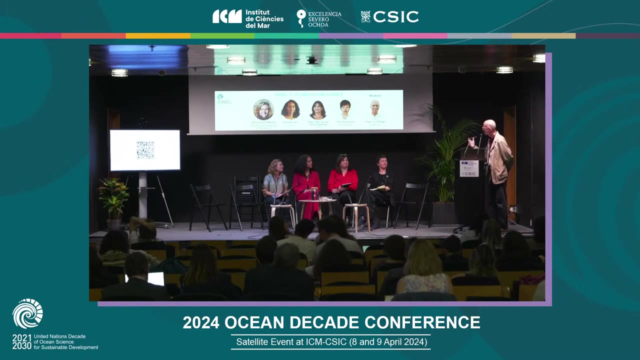 And I think this event is really an example of how we interconnect, So how you could explain to children that engage them and encourage them to become a scientist. What is the essential element of science, of intelligence, of natural intelligence. How do you think we can? 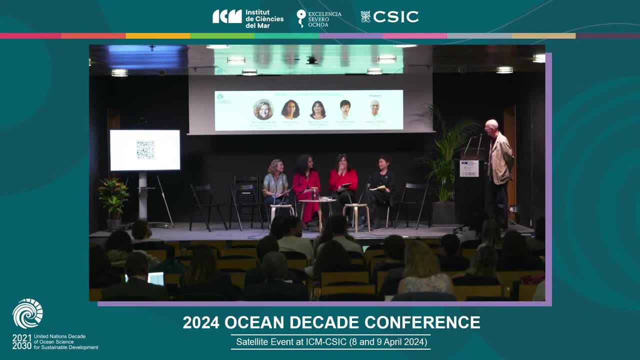 for sure this question that, in a way, Silvia posed. Well, this is something. it's a tricky question and you've said many, many different and interesting things that I think I can mix with the people behind. I think we are talking about turquoise again. 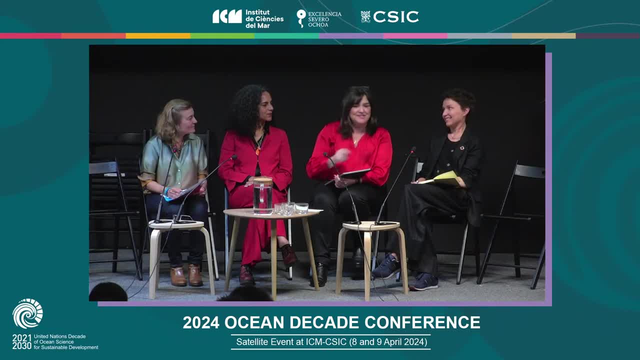 We are going back to that because you mentioned it. We have been mentioning that. I'm grabbing that word from you And you said something that was really interesting. I'm guessing that what you do in the brown impacts in the blue, But maybe from our point of view as researchers, 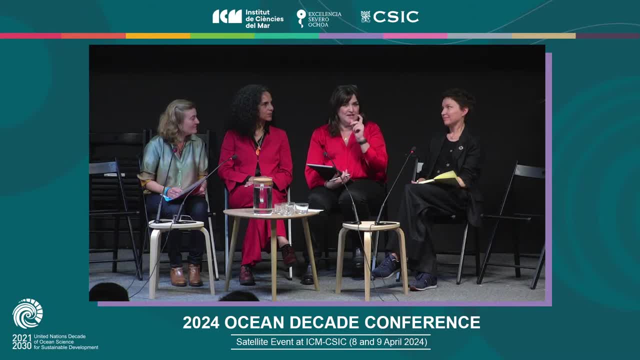 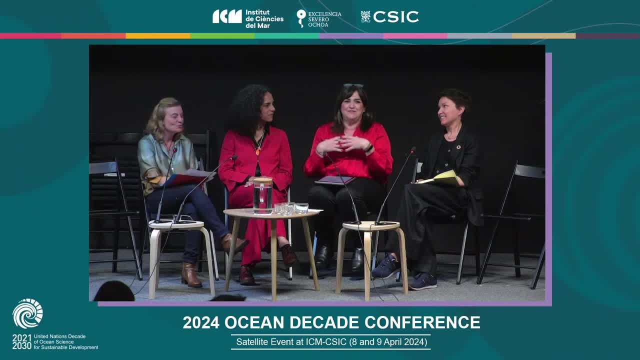 I'm tonic, Yeah, So I think our main job is to introduce the people that the ocean is a part of my house, It's my ecosystem, It's what we need. It's not only from our point of view as researchers. the terrible message of we are gonna die. 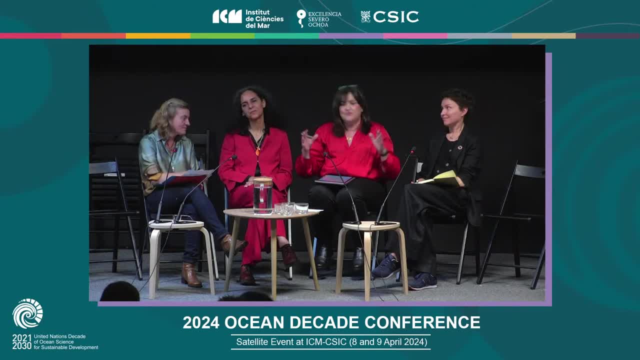 Everything is terrible, climate change dream- no. So we have to change the relation with the people. So we have to say: well, the sea is there. We have to face many, many, many things, many different, a lot of problems. 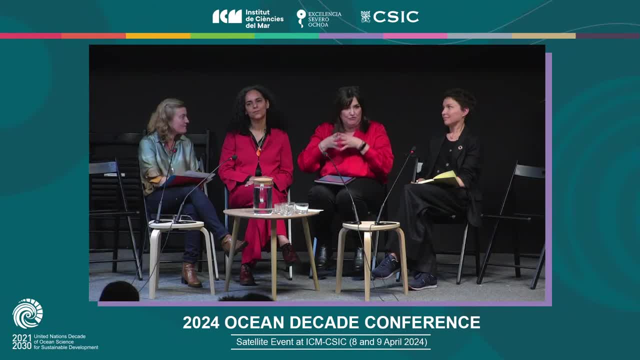 There are huge problems that they are really impacting on us And we have to change this relationship, And the only way, in my opinion, is to say, yes, this is my house And the ocean is part of my house. I want a clean. 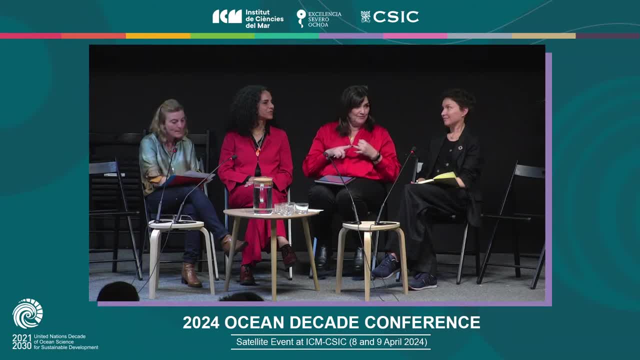 house. I want a resilient home. I want a predictable home. I want my family to be predictable. Exactly the same things we want for the ocean. It's exactly the same things I want for my house, for my home. So the only way to have a 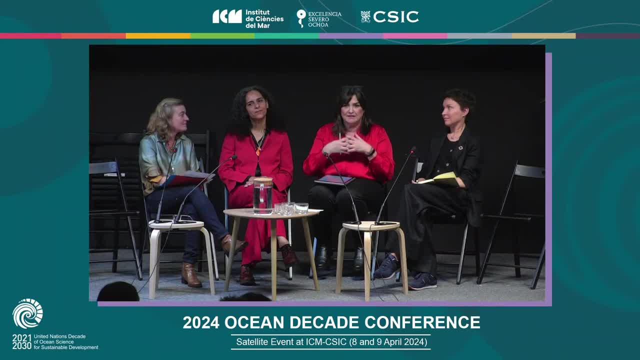 really good relation to the sea is to say, yes, the ocean is your ecosystem. You are an atmospheric animal, We are atmospheric animals, So that's the reason why it's easier for us to understand what's happening on Earth. But we need the sea because our climate. 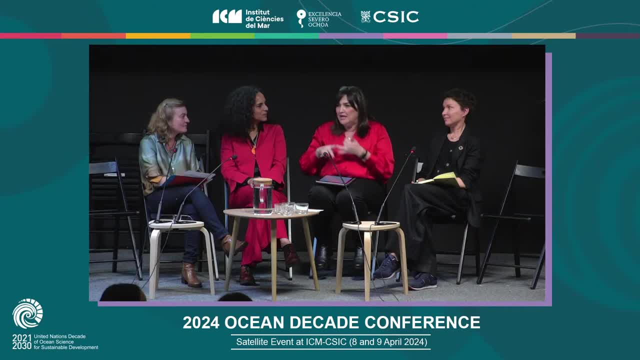 is the climate we have because we have the sea. We can eat some food because it comes from the sea. We can work because we have the sea. So the only way to change this is to make us understand the society understand the importance of 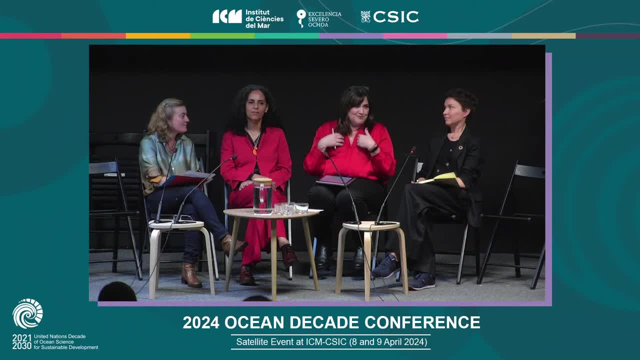 being also aquatic animals, Because I think I am an aquatic animal. Thank you, Okay, we have just a few minutes left. so Donata and Dina, No, no, that's wonderful If you want to wrap up a little bit. Thanks. 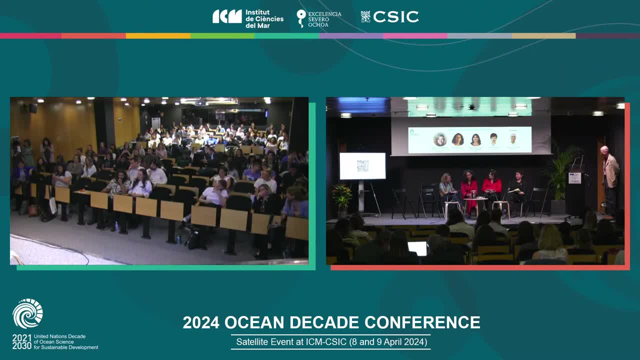 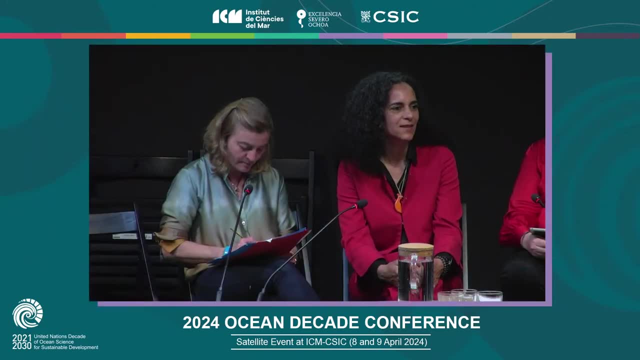 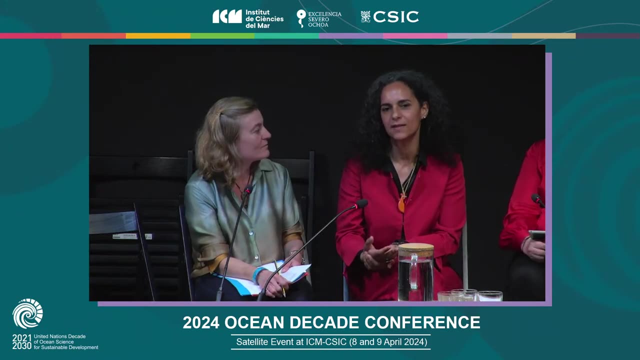 What comes to my mind is that we should never stop kids' curiosity, because kids are curious by nature. So what we can do to stimulate their engagement with the sea is to respond to their curiosity and to show the linkages of the ecosystems, of what happens in. 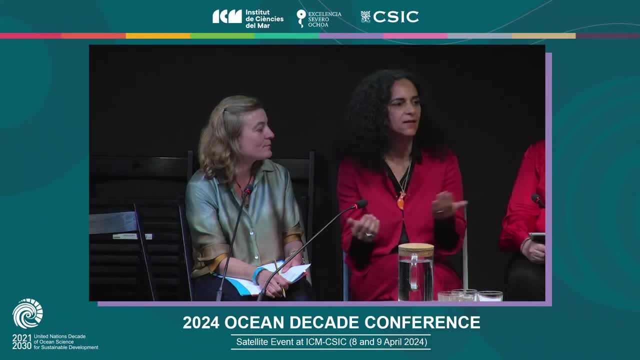 the sea and happens in the water, in the land. All these interconnections are fascinating to the kids because they are a kind of adventure into the nature, And I think that being able to dive with them into these interconnections can be a key to stimulate and to 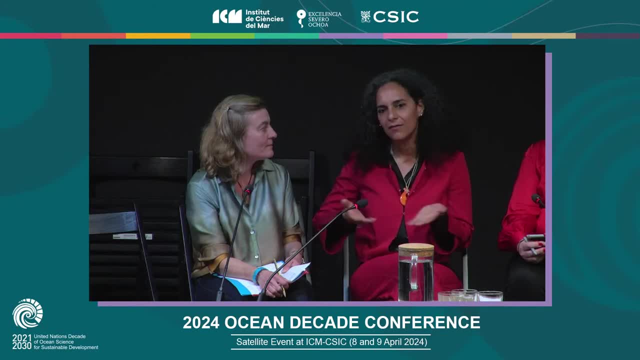 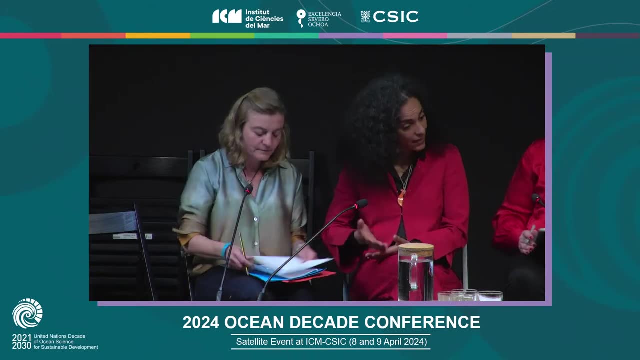 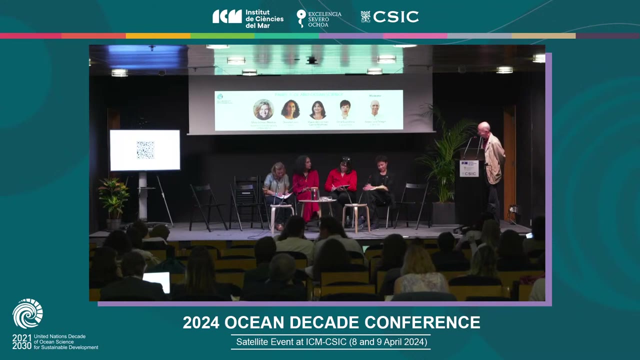 answer to their curiosity And keeping alive this curiosity, I think, is really, really important to improve their engagement. And to answer to your question regarding how to improve- and I don't remember the question, but it was related to how to make kids interested in ocean science- 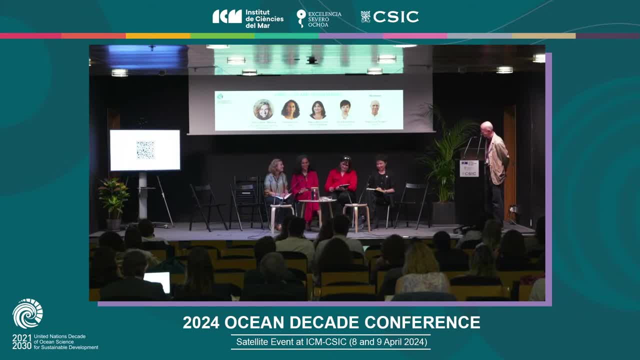 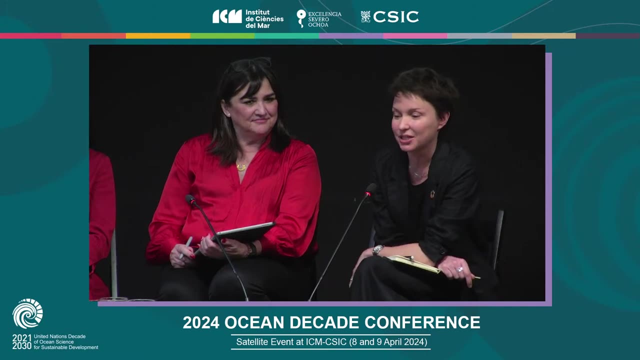 Thank you, Tina. please, I just have a few words in our turquoise house. If we look at the house as a marine institute, oceanographic agency or meteorological agency, which are the organizations I work with, and we imagine that marine science is not just one part, for example, the kitchen. 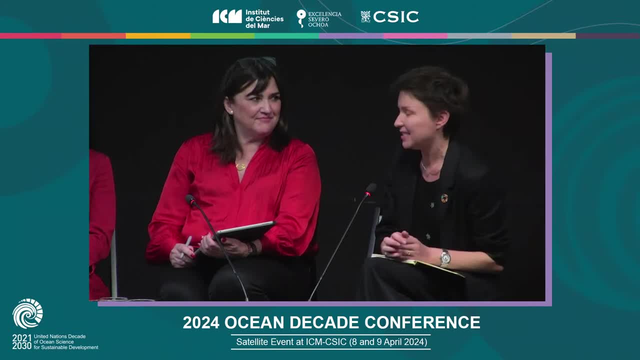 We have all different parts in these agencies and I think what we try to do in URUGO's ocean literacy work is really promote multi and cross connections between different disciplines and sectors which actually all make our house, which is the turquoise marine institute. 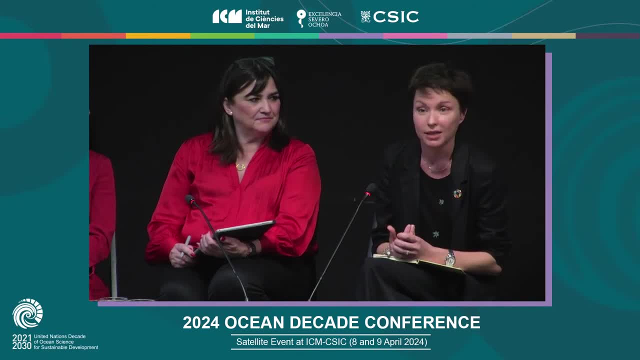 It's much more impactful, much more open to new talents, to blue careers, to other disciplines. It makes science better and richer And this is what makes social literacy so really strategic for marine research And I think clearly we are on the right track. but 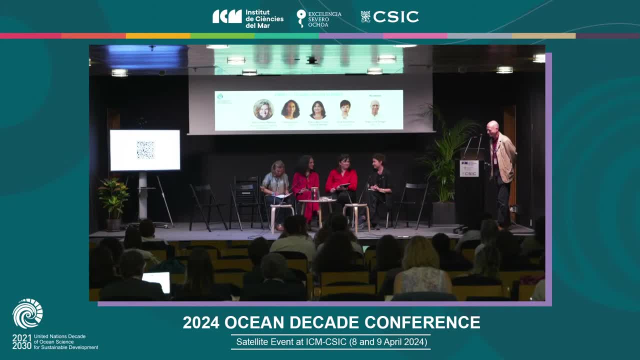 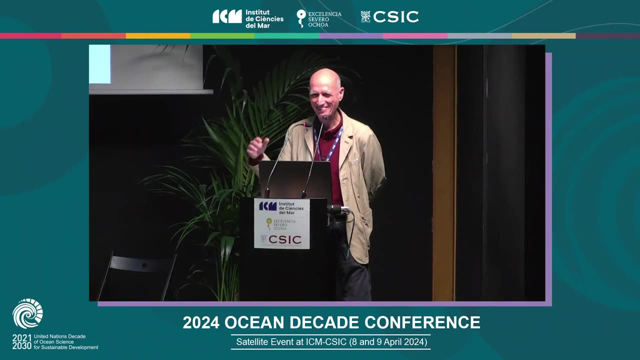 still much, much more to do. Well, I think, I must say, because I'm I'm 66 already and I've been in many, many meetings and many events, and this has been in over 40 years of experience. 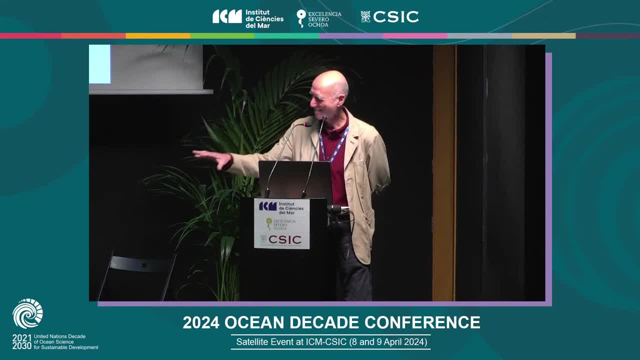 the most, most, most collaborative event I've been ever. At some point I thought it was not going to come out, but magically at the end, this collaborative natural intelligence that in a way reflects that we are part of a collaborative living Earth. 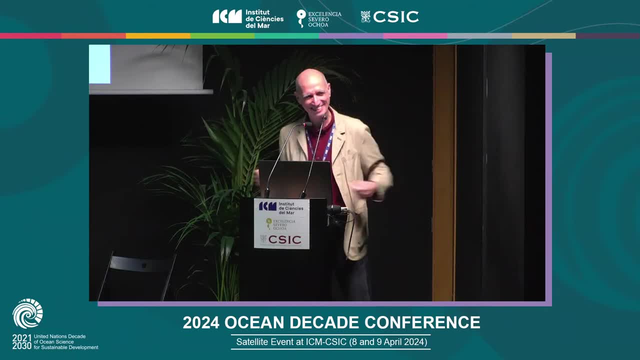 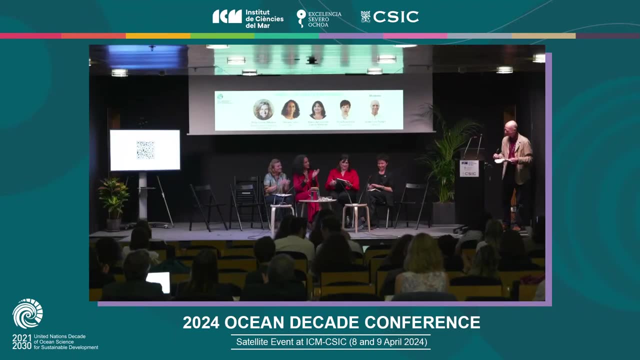 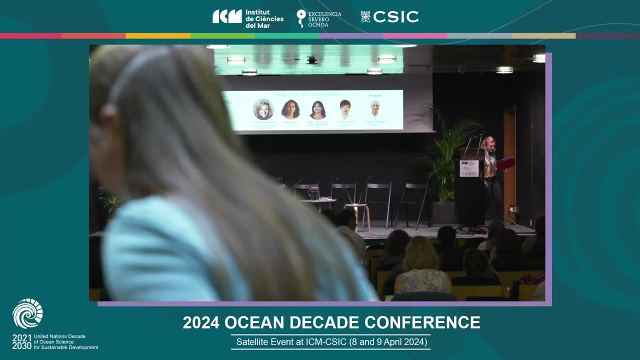 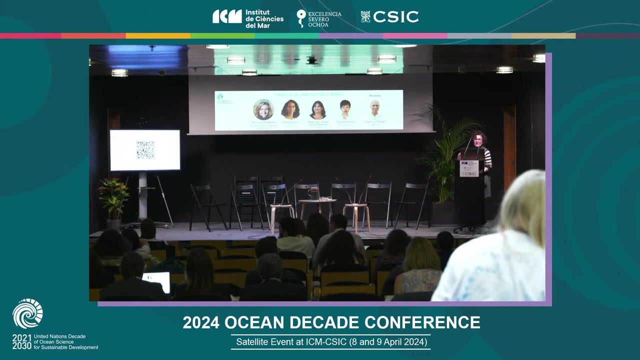 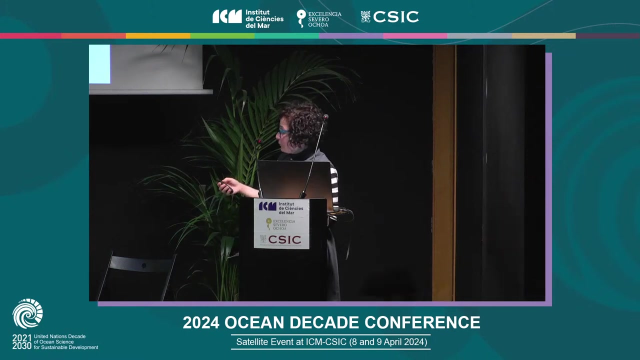 has come out in this wonderful session, and I must congratulate the organizers. Thank you, Thank you all very much, and I want now to invite on stage panel two, that is about communicating ocean literacy in local communities. So it's another great panel that is going to be moderated by Emilio Beladies Martinez of Plastic Oceans. 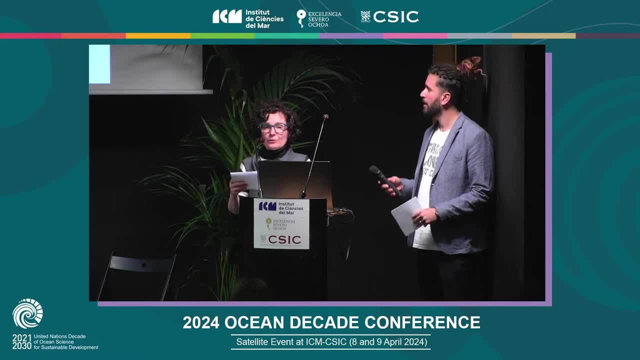 and the panel is going to be on the stage. Thank you. Our panelists are Noemi Fuster from ICM-XIC, Joseph Mendoza from the Sustainable Ocean Alliance, Beatriz Patraca-Dibildot from the Autonomous University of Barcelona. 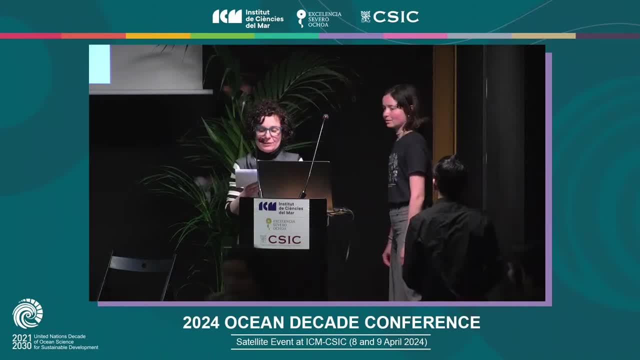 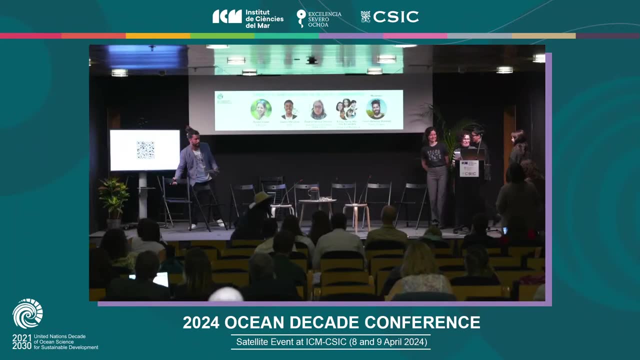 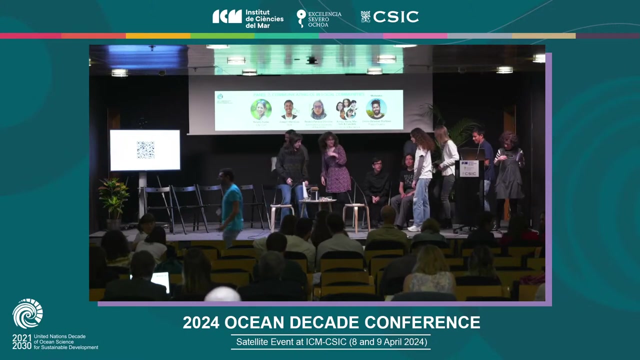 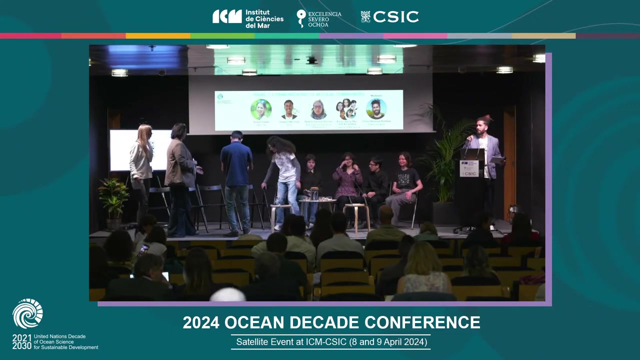 and a group of five students from the University of Barcelona: Arnau, Berta, Mar, Ada and Candela. Welcome all. We are looking forward to hear your stories. Hello everyone, Can you hear me with these microphones? 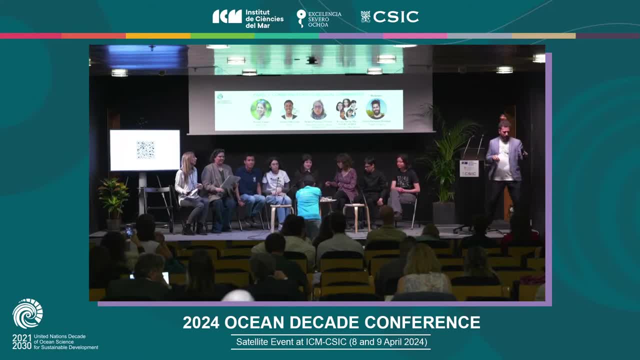 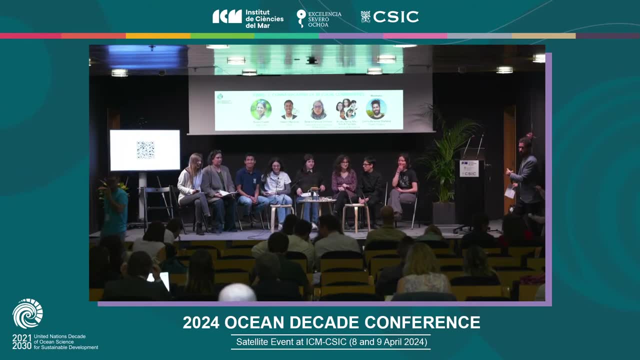 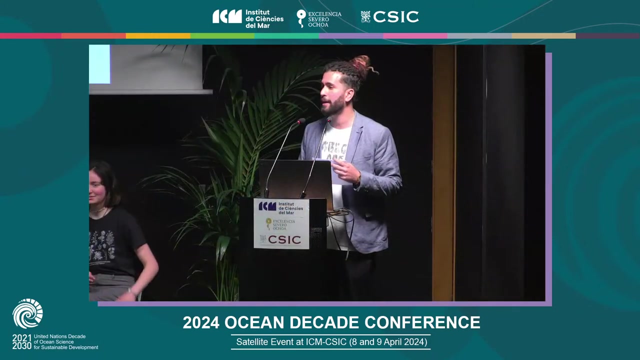 It's okay, the sound Okay, So we just This one. Yeah, Okay, That's wonderful. So we are going to start with the next panel- Thank you for the bubbles, I love that. And today in this panel, we are going to talk about communication on ocean literacy in local communities. 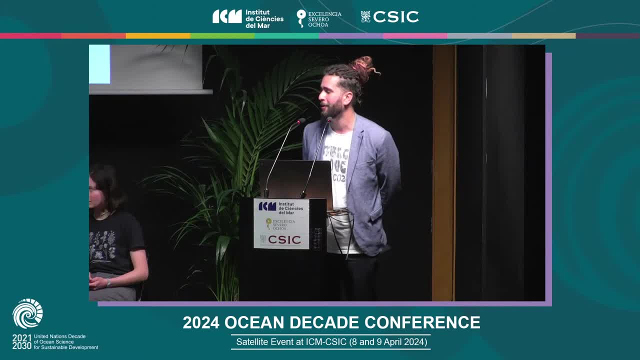 Today we are one of the biggest panel of all the sessions because of the amazing group of students that we have today here And, as I mentioned, as I was thinking like we all talk about the no blue, no green, that the mention of Dr Sylvia Ayer and no water, no life. 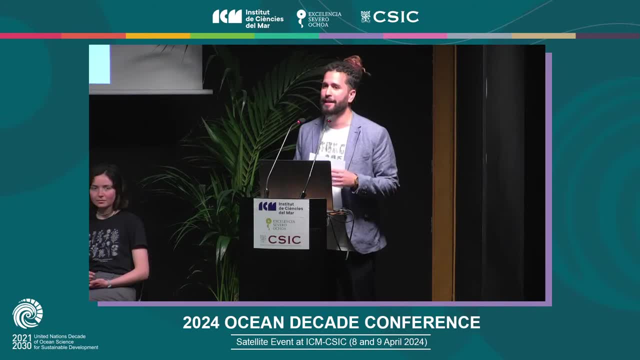 So it's so simple: right the problem and it's so hard to get to the solution, but it seems like today we are getting there. We are getting to know a lot of propositions, a lot of initiatives that are really based on success and on collaborative knowledge. 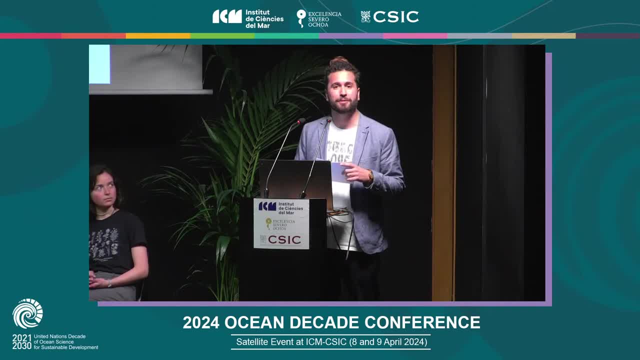 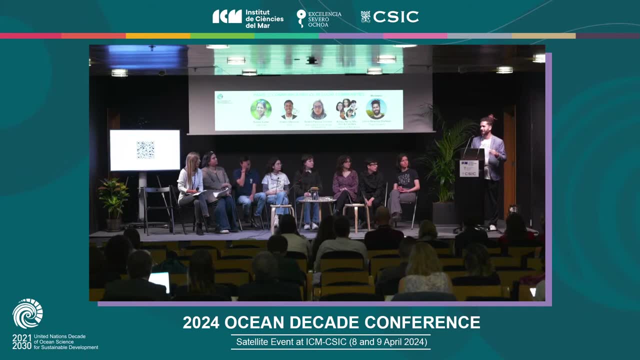 as we mentioned in the last panel. So, as As the time is ticking, I'm going to start just naming the panelists and starting with the presentations. okay, So, if you don't mind, the first groups, the first group, sorry, Candela Guerrero. 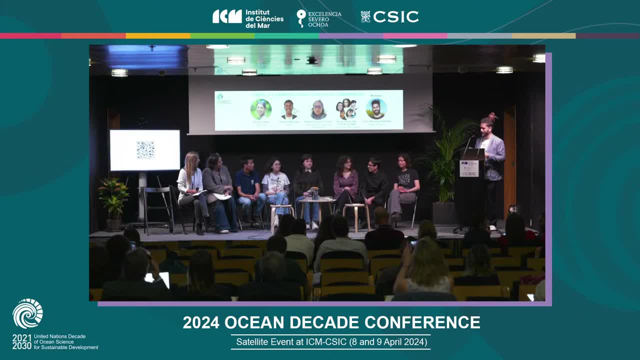 Arnaldo Cipres, Berta Jordan, Ada Ferrer and Mar Ainud all present. okay, So please introduce your project. Okay, Hello, Good morning. Our project is based to creating a survey to evaluate the Catalonian population knowledge. 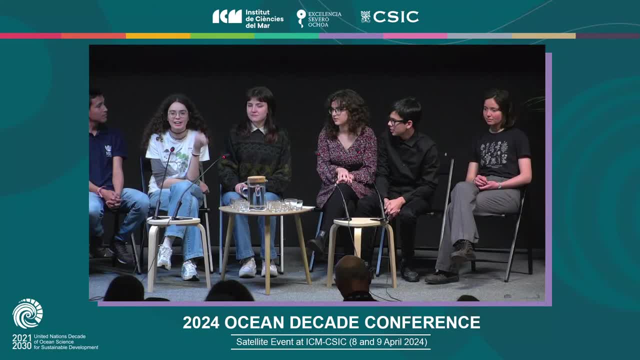 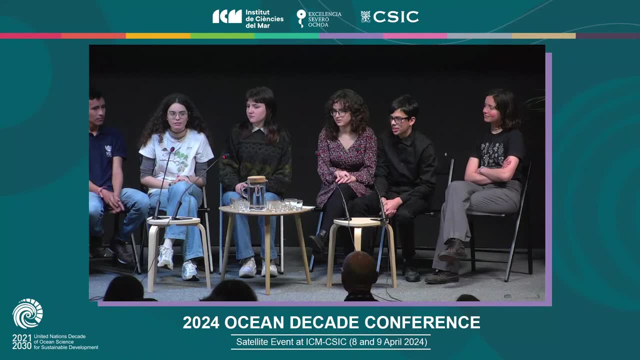 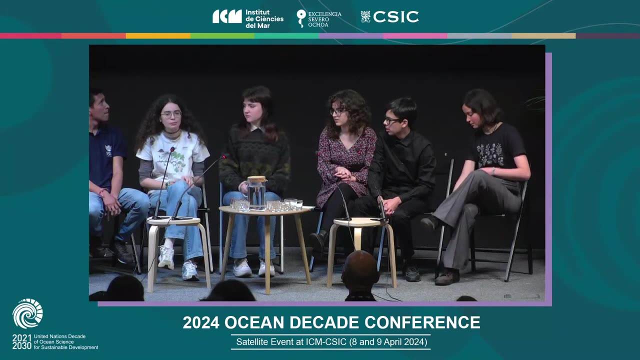 About the ocean, like certain issues and adversities that may occur in the ocean and in the beach. Based on the research and face-to-face interaction, we have found that the majority of participants didn't know about citizens' science, and we consider this important. 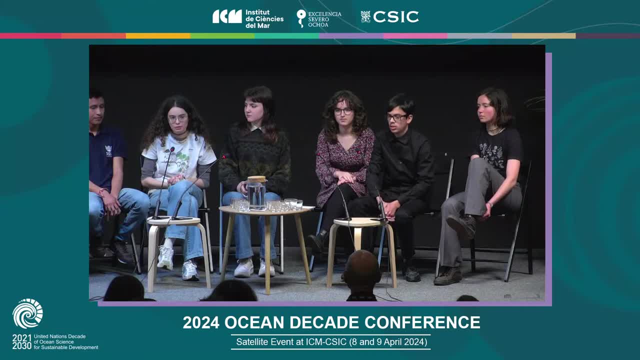 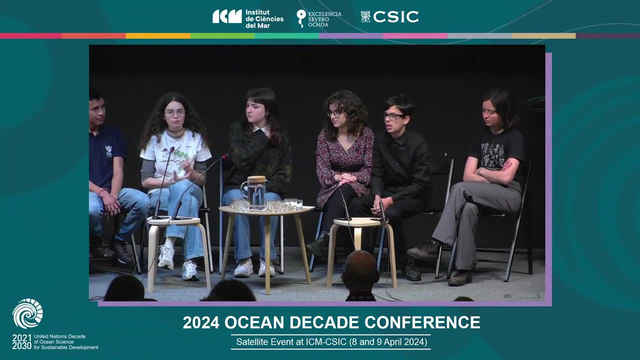 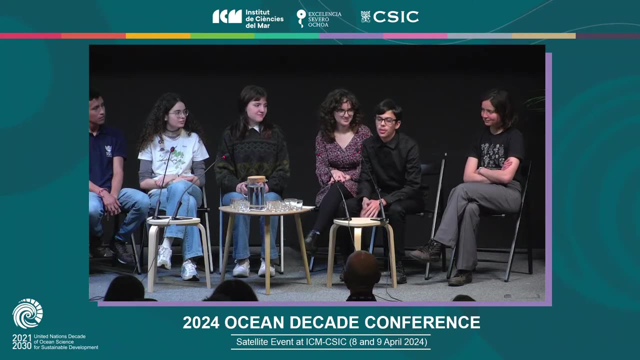 for all the environment studies to reach the pollution and, in this way, and promote the ocean mindfulness and improve the environment. Okay, This survey. this survey was open for 24 days with a participation of 549 people from different parts of Catalonia. 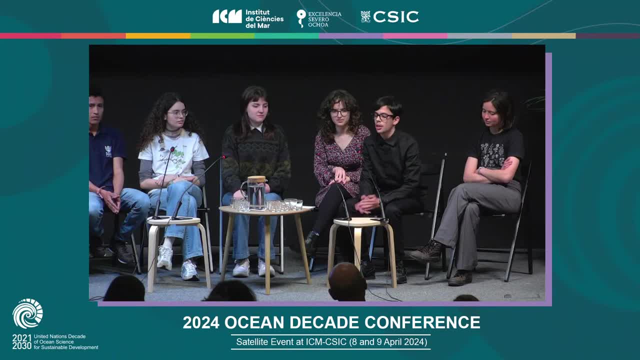 Furthermore, this survey is structured in various sections that are knowledge of ocean literacy, including global warming, and put people in various situations to see their reactions. Another section is fishing, where we ask people if they know the best fishing techniques and its consequence on the marine environment. 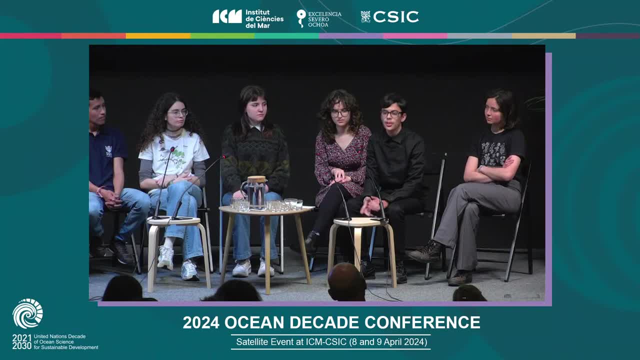 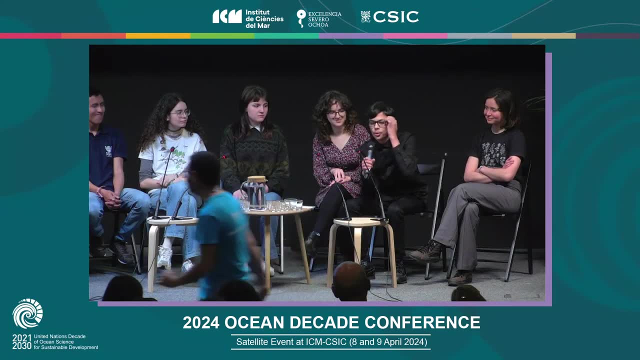 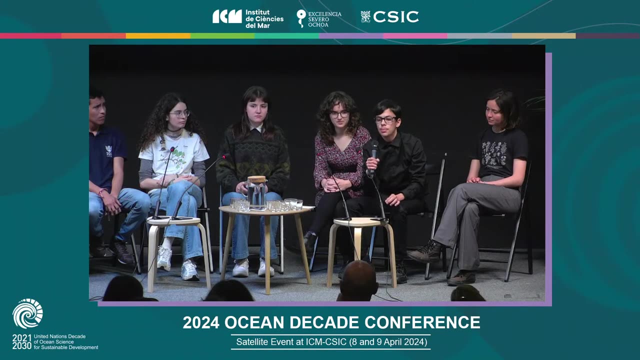 And the last section is related with this conference and with the decade, in that we are in Because we ask people if they know- sorry, thanks, okay- Because we ask people if they know that we are in the ocean. decades and the 90% of the people survived didn't know. 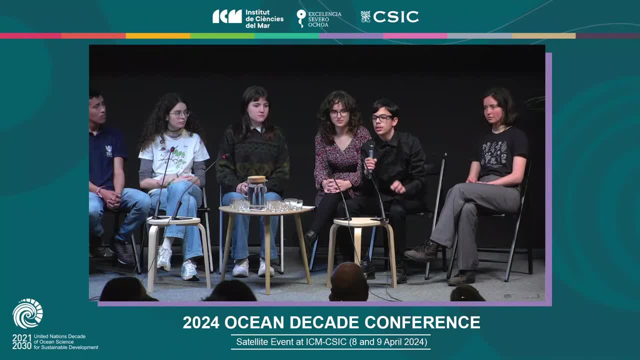 Also, we ask people if they know that the conference of the ocean decade is here in Barcelona, and the 87% of the people survived didn't know either. Okay, So this 87% represents more than 475 people that didn't know. 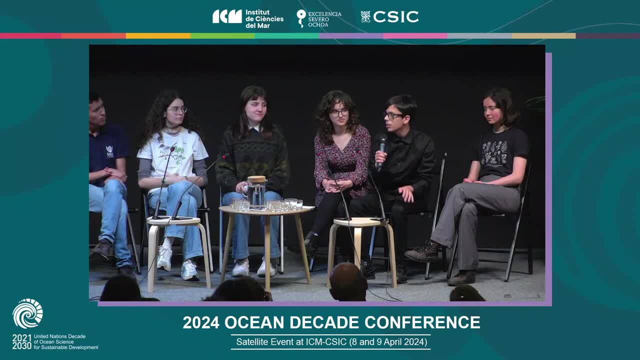 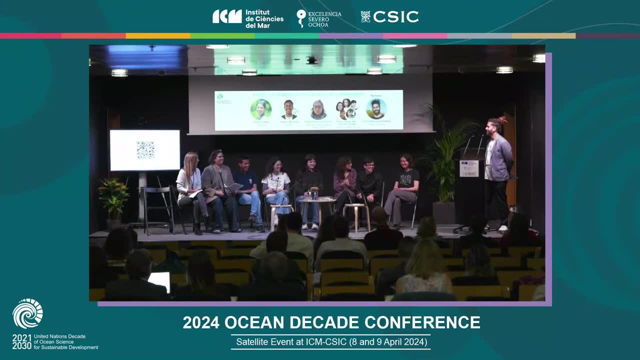 that this conference exists and that it is being held here in Barcelona. Okay, perfect, Thank you, for That's sad. that's sad. I know that's sad. I didn't expect that ending. So, Joseph, please introduce the joining staff. 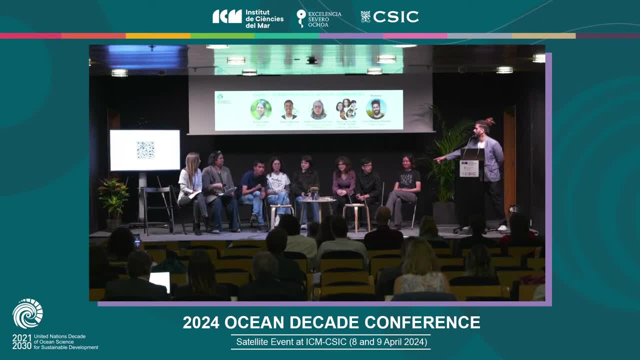 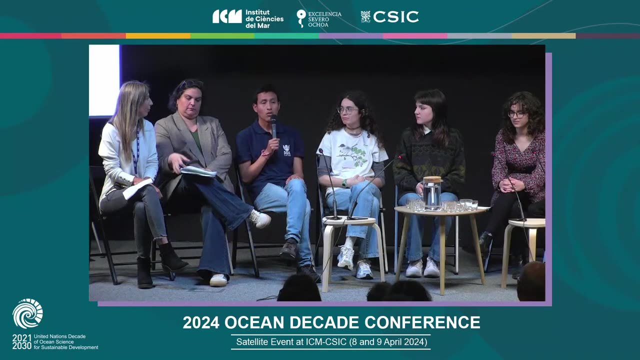 Okay, yeah, okay, perfect, Hi everyone. Thank you everyone. Okay, better, Hi everyone. Well, my name is Joseph and I am part of SOA. SOA is Sustainable Ocean Alliance. It's an international organization that activities young people around the world. 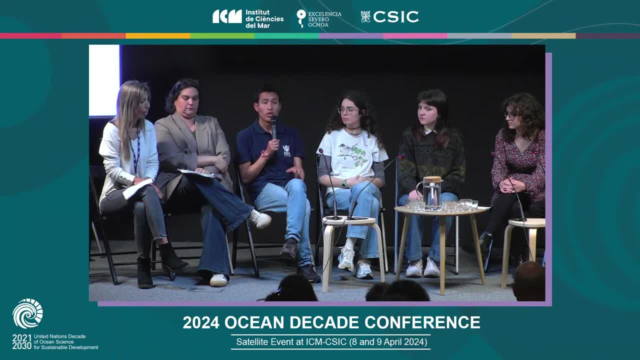 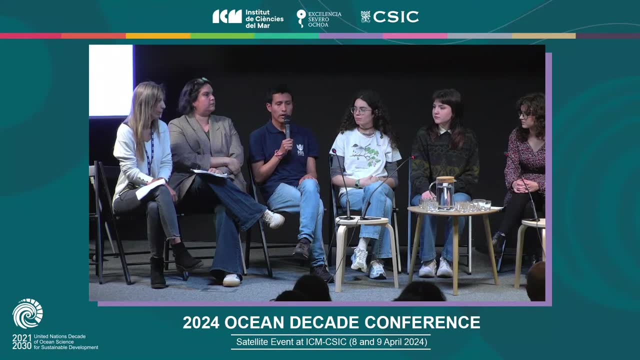 In fact, it's the world's largest community of young people working for restore the health of the ocean in our lifetime. So So we we have many programs and develop and implement innovative solutions. For us it's important that point because we consider: 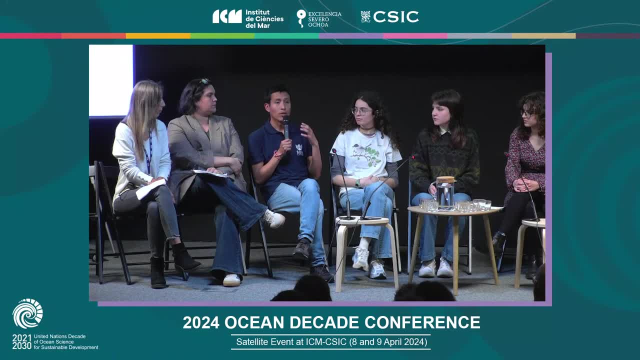 that the ocean literacy is one of that innovative solutions that we have the possibility to develop and implement in different initiatives or projects around the world, because we are working around the world with different hubs, different teams, from Latin America until Europe, Africa, Oceania, etc. 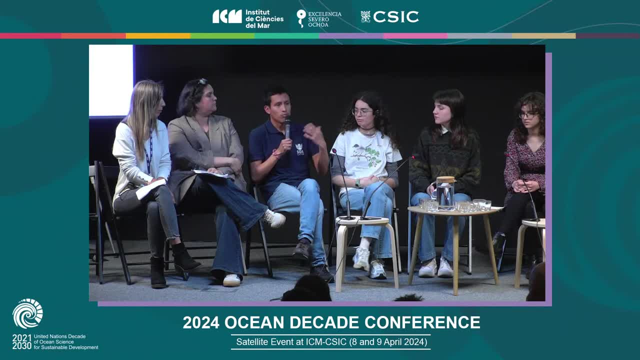 So that is more than a project for me and for the rest of the people here. that is part of SOAIS: A community, a community working based in many issues, but specifically today for talk about the ocean literacy. Thank you, Joseph. 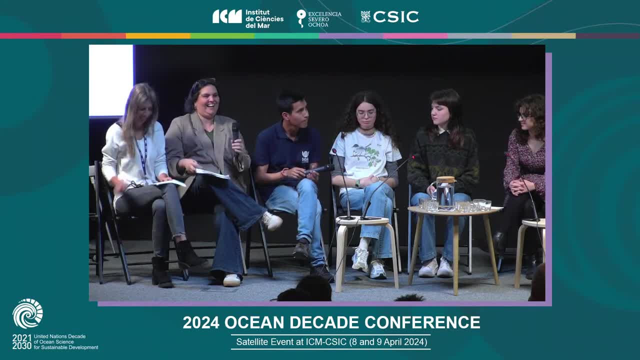 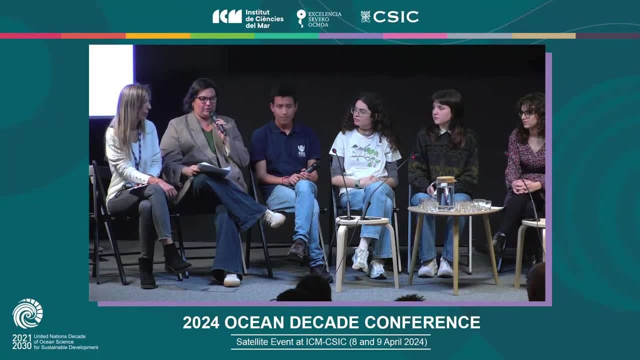 Pass the mic to Beatriz Patraica. Oh, don't need it. Okay, perfect. So, Beatriz, whatever you want. Good morning. We are working with Silvia Gomez-Mestres in the Empower Us project. Our pilot project is, as Silvia says: 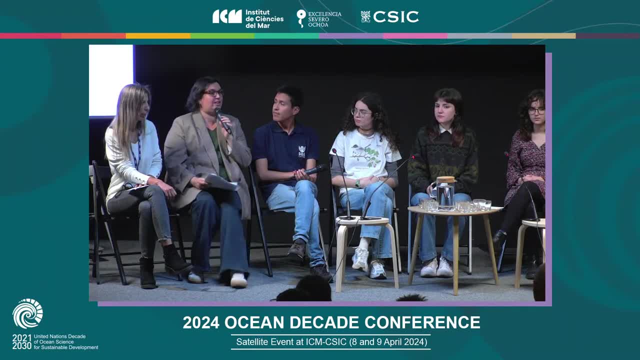 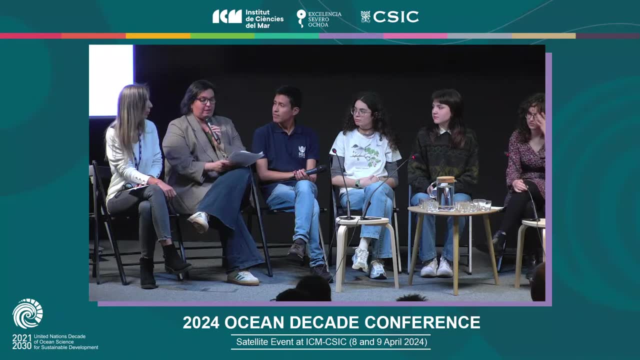 a natural cap. Silvia talked about the ocean, literacy and the science, and I want to talk about the social project, the participative and community project. And well, our main challenge is the need for creating alignment between the interest of low-economy stakeholders. 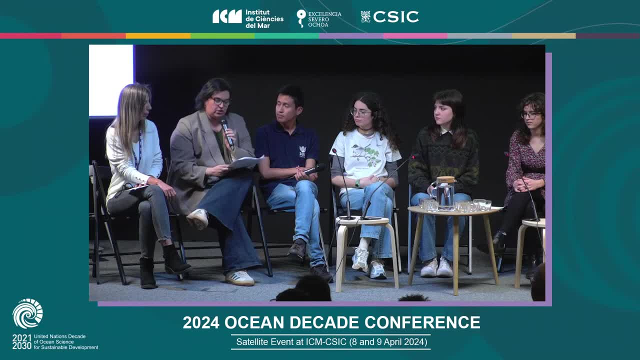 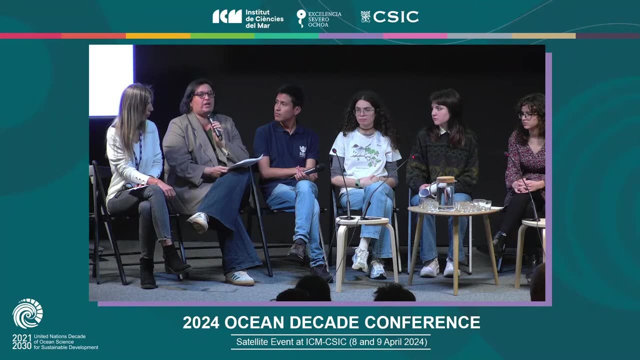 and our environmental conservation goals, Above all, in the way of carrying them out. We employ an approach of reaching online and offline spaces, because it's not about to get a majority project. if we want to get involved with all the voices- And the process was very 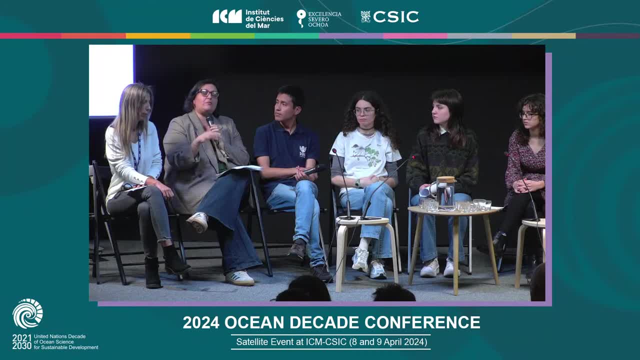 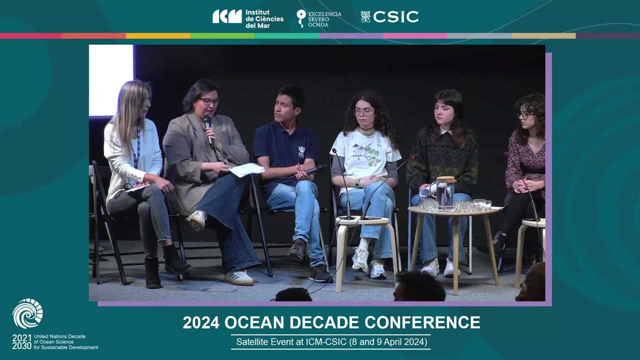 very specific. because we have very specific, because we have two workshops. We in the first workshop we try to get the challenges And in the second workshop we try to present to pilots for the stakeholders. But we need to do an hybrid solution. 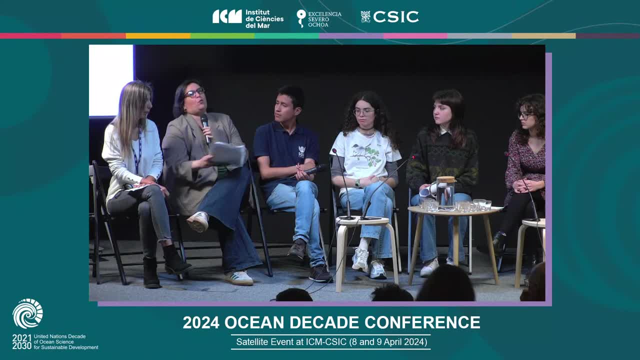 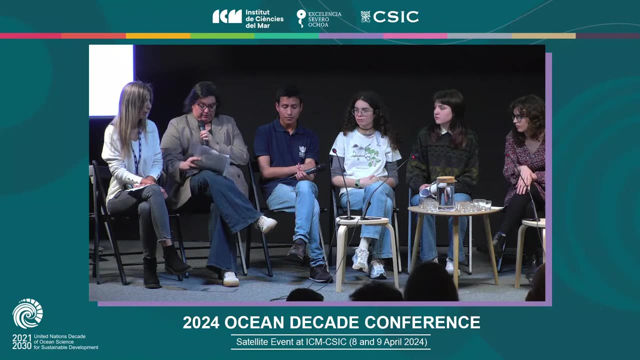 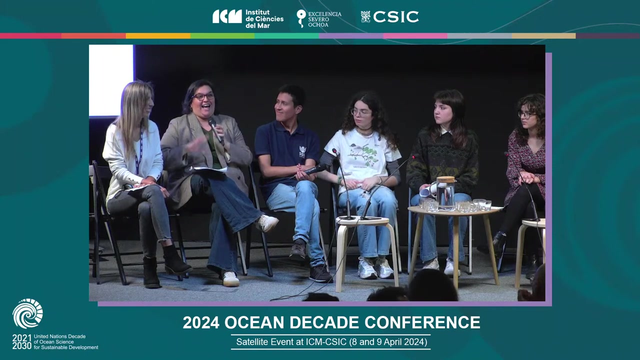 because someone, some people- prefer a digital tool, but the other, some others are, with some avoid of the digital tools. We try to create and continue online and offline. Well, today, talking about online and offline spaces is very old-fashioned, but we try to get one project. 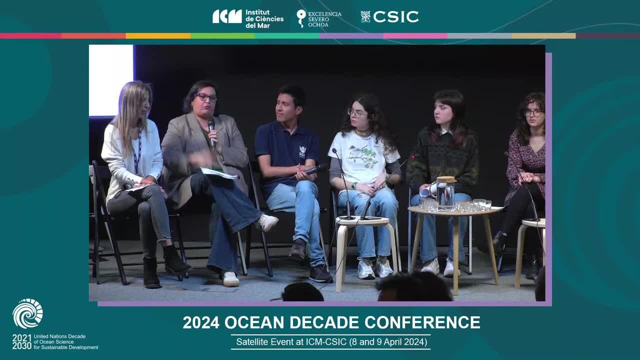 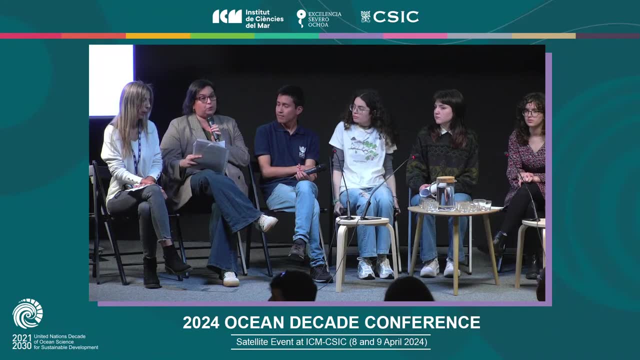 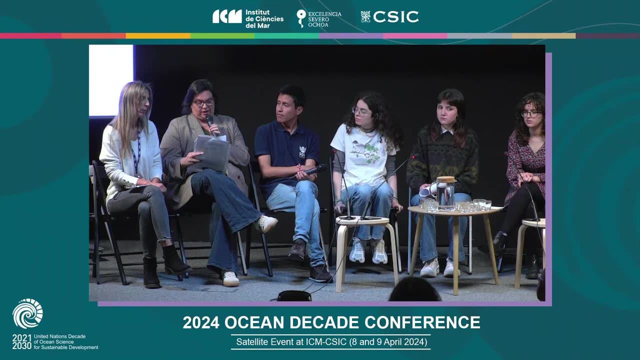 that we preserve the community face-to-face experience and the digital solution. And well, in conclusion, Natural Cap stands as a replicably pilot project where coastal communities are empowered, not just users of the sea, but activity guardians and ocean literacy agents. 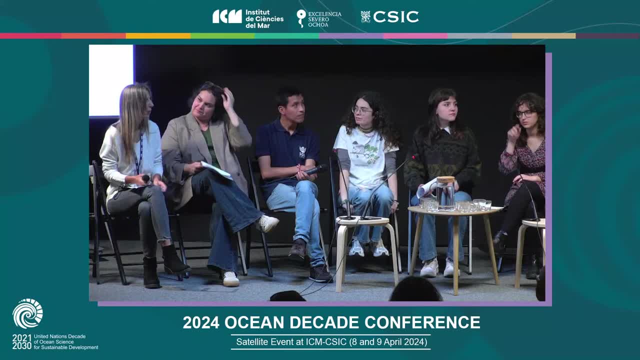 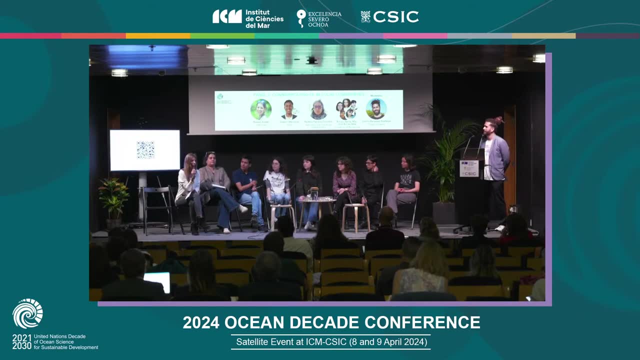 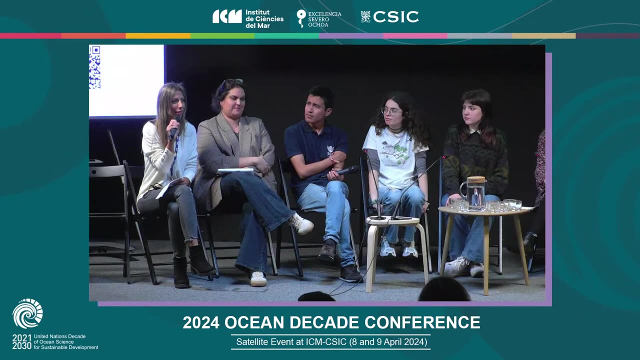 Thank you. Thank you, Beatriz. So, Noemi Fuster, tell me about your experience on the project. Good morning, My name is Noemi. I work in this amazing center, the Institute of Marine Science. Okay, I have been working here for about 30 years. 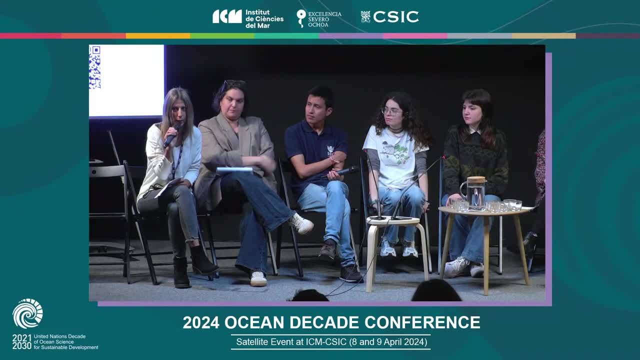 I think, like I said, we're the first to have an institution where citizens are engaged in citizen engagement. So what can I tell you? So I started out as a researcher. I am a science teacher, but from three years ago. 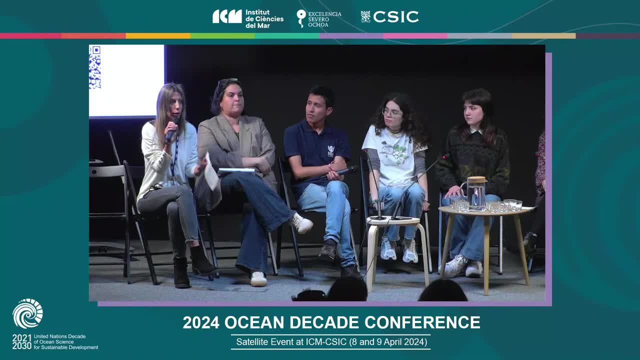 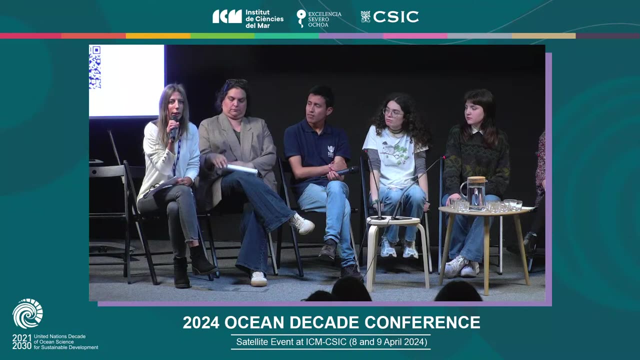 there is something that keep me awake at night: how to get real citizen engagement. It all started when the main goal of the Mission Ocean was published, By creating a network here in Barceloneta neighborhood. It's a it's a very small area. 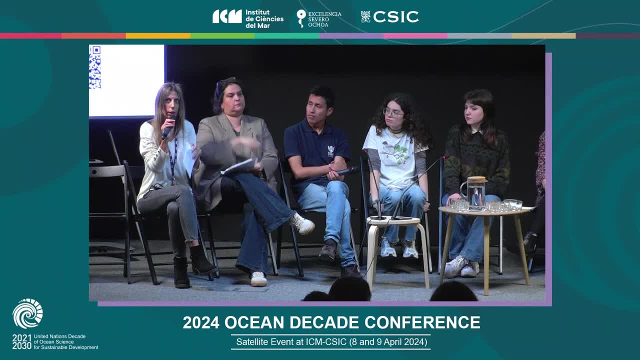 But with a broad target. we have The City Council, the port, the citizens, the fishermen. so once we made this network, we put it to the test and we proposed a morning of activities to 30 CEOs of the main companies of the port, activities such as Mindfulness at the beach, snorkeling by learn more about biodiversity. 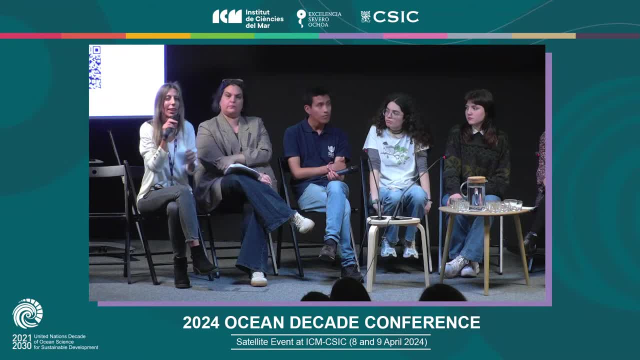 also Removing surface waste and we visit environmental and information center, the central, a plateau. in the beginning and at the end we did a profile of mood states test. This test identifies 34 different emotions and you have to Mark the ones that you feel connected to. the results show a decrease in negative emotions, such as 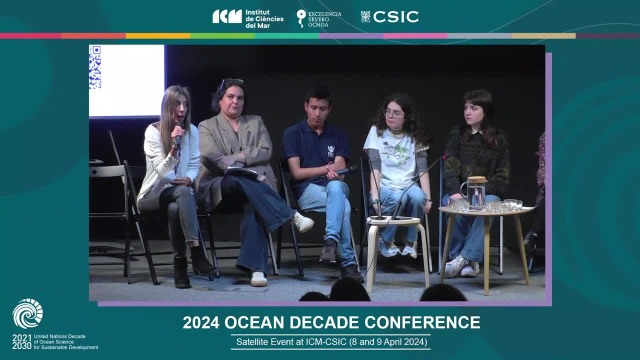 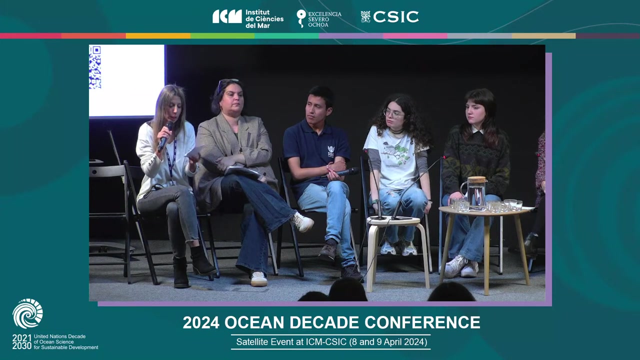 Hopeless, helpless or sadness, and an increase in positive emotions such as happiness, confidence and commitment, So indicating that when they finish the activities, people had a more proactive and committed attitude. So we got it. We got it. using a local network to do immersive activities In the ocean seems like a necessary step to get citizen engagement in ocean restoration. 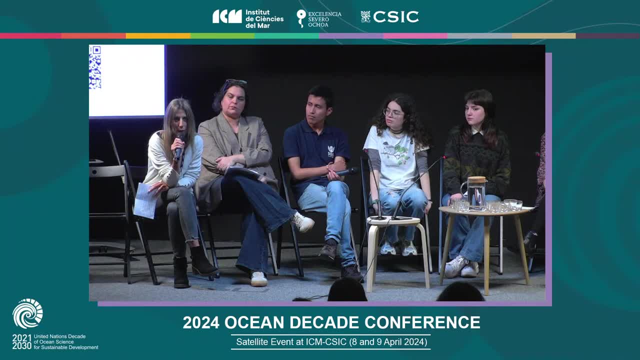 But then another question came up: What is ocean? Does the ocean represent the same thing to all the people on the planet? Then we did. we did a survey among citizens in Barcelona and in Sanya in Gambia. It showed us a difference when it came to defining the ocean. 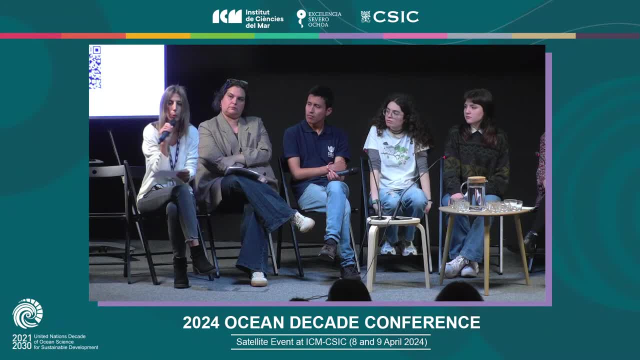 in Barceloneta, the more the words that represent the ocean were freedom, water and life. But in Sanya in Gambia, the most common words were income, fish and God. and this last word is really interesting because in some cultures The, the health of the ocean. 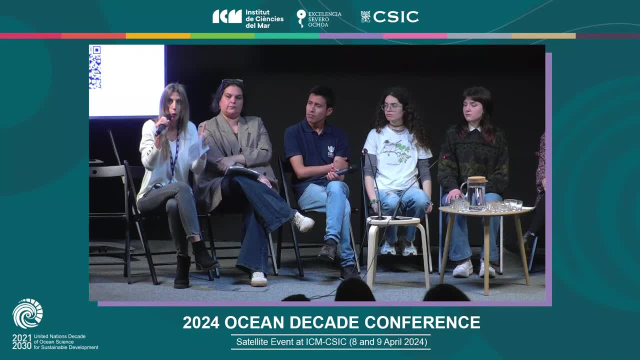 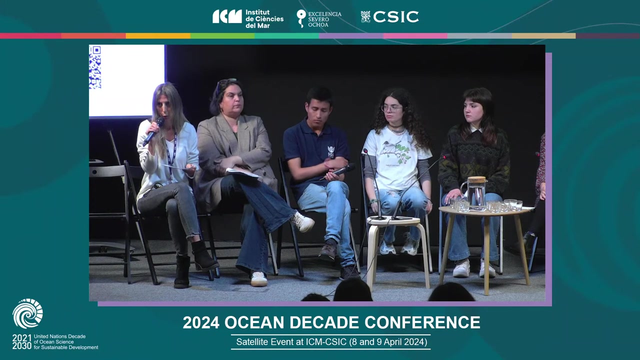 Is measured by science. but in other cultures the ocean is a gift from God and his belief that God will always provide fish. So if the concepts of the ocean are so different, we must look into the cultural background. It's necessary to consider this if we have to face such a big challenge and recover the ocean by 2030. a 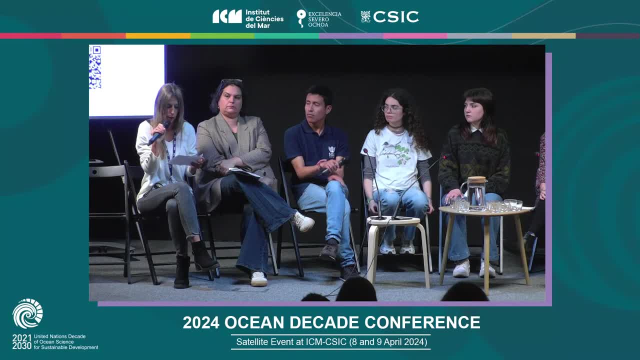 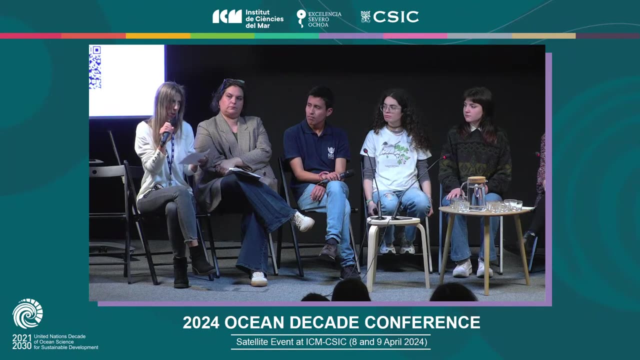 challenge of this magnitude requires a planetary commitment and In order to restore the ocean in record time. so, in conclusion, We believe that the first steps to get real citizen engagement are: Find the activity that makes the biggest impact in our emotions. You can use the the profile of water states test. 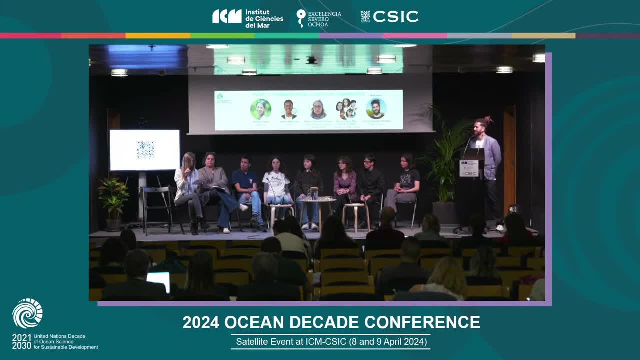 Please do a survey- the survey before- to find out what ocean means, in order to know what approach to take and what communication will be most effective and, Of course, involve local networks with the same cultural background. You have more information with better grammar or better vocabulary and on the poster outside. 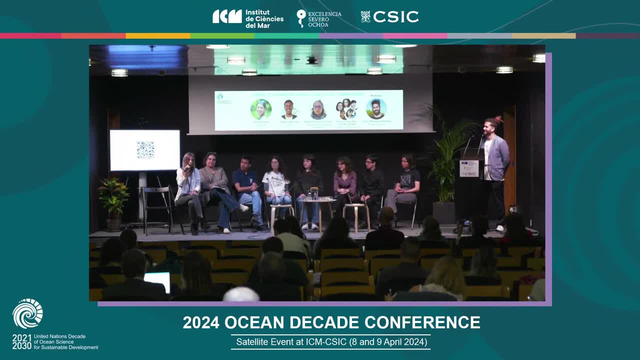 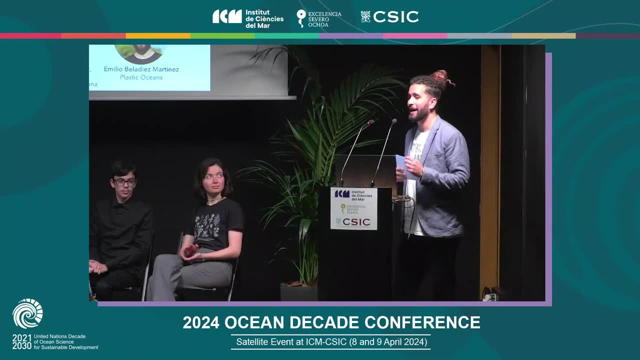 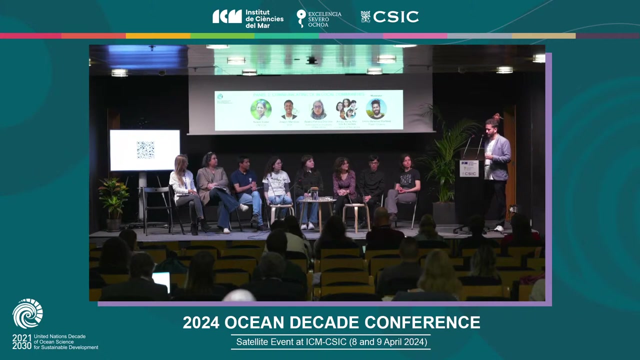 Thank you so much, and eight Mubarak to the all-muslim community. Thank you As we have. as we have some minutes left, I'm going to ask you one question to each group, so be ready. okay, Are you prepared? Yeah, So the university group. according to your results, what aspect of ocean knowledge, of ocean literacy, do you think should be enhanced? 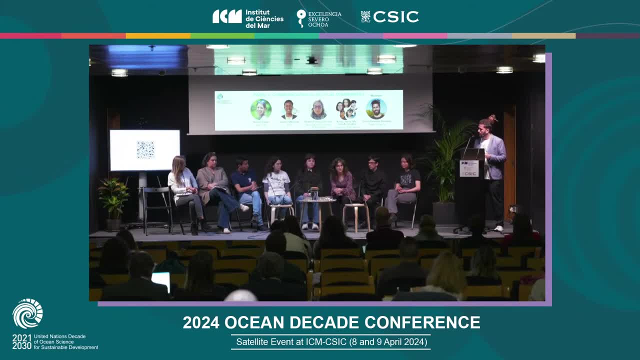 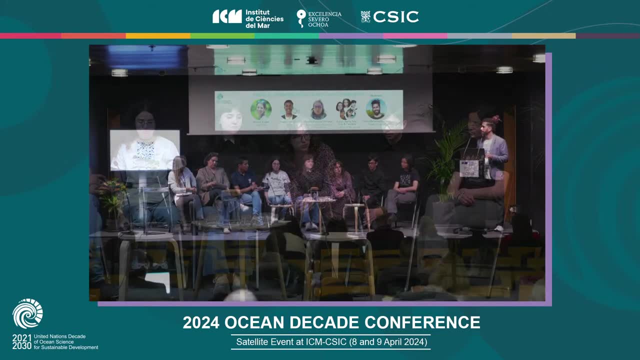 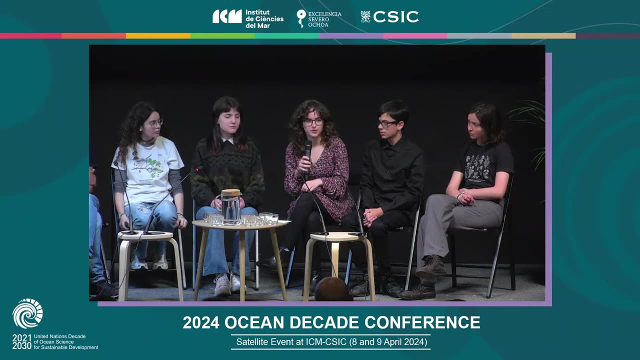 Well, we think that general knowledge about the oceans should be enhanced, specially things such as how to act in emergency situations like getting Sorry, like getting a jellyfish sting, because we found that about 60 percent of the people we interviewed didn't know how to properly treat such a. 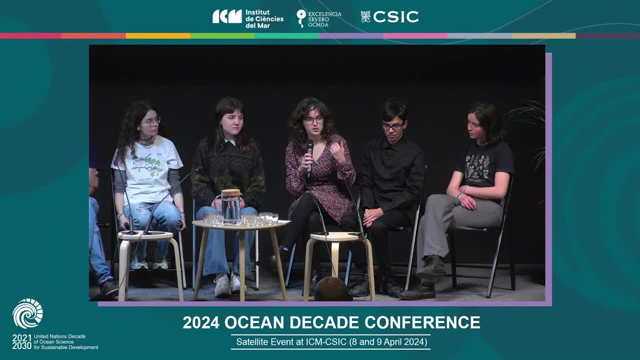 common Occurrence nowadays, and also to like enhance certain areas of knowledge, like blue carbon, which we found to be a area that was very much lacking in knowledge, because we asked our participants to like rank certain topics, like to say: Which topic do you know about the most, which less? and we found that blue carbon, which is a crucial 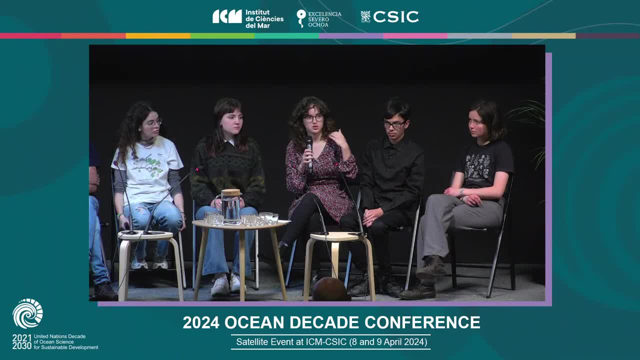 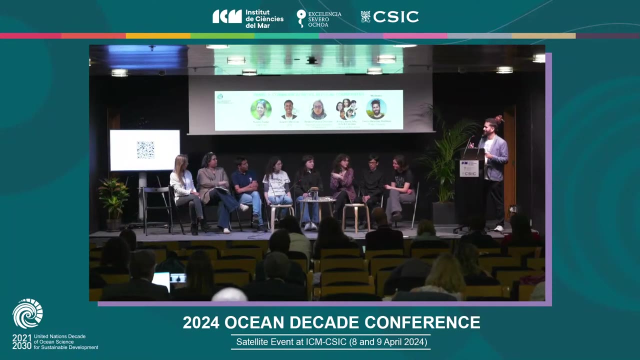 Thing to know nowadays, due to climate change and such, Was one of the topics that people, that less people knew about, so we should try to like enhance those areas In knowledge. you can find further information on the poster. Okay, okay, Thank you so much. Pass the mic to Soa. 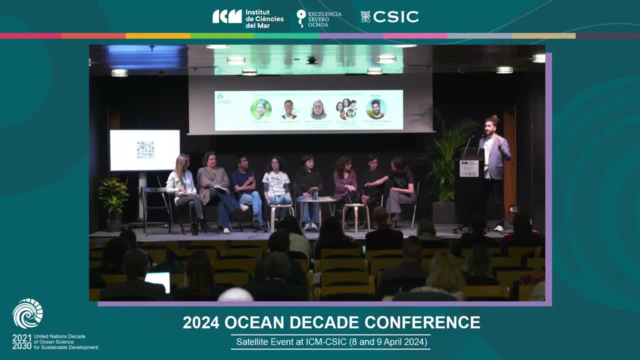 to Joseph And, as it has been said in the other panels about the generational topic, generational barriers, like the youth is not really engaged. But today we have this example- you are example of youth engaged on ocean literacy. So how does your organization so engage with the youth to encourage them to be like a speaker of the ocean? 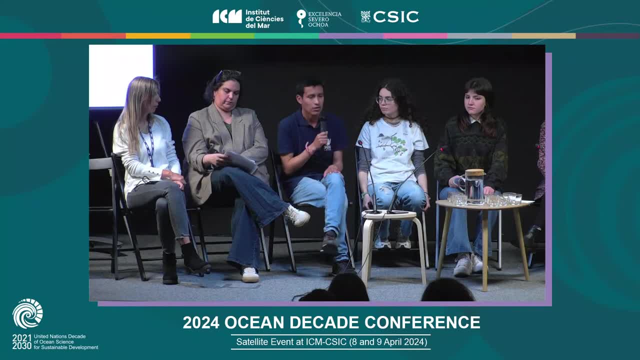 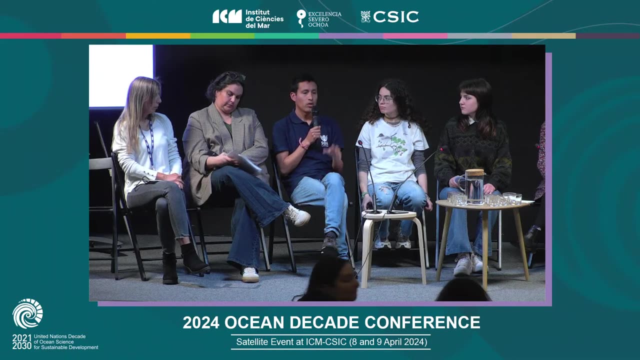 well in our case, well in my case also. So I have a Different programs. I was talking about it, But I kind of put the focus on one of the programs, a ocean leadership program, because with that program- or throw that program- the idea is a Facilitate tool, tools for the young people around the world. 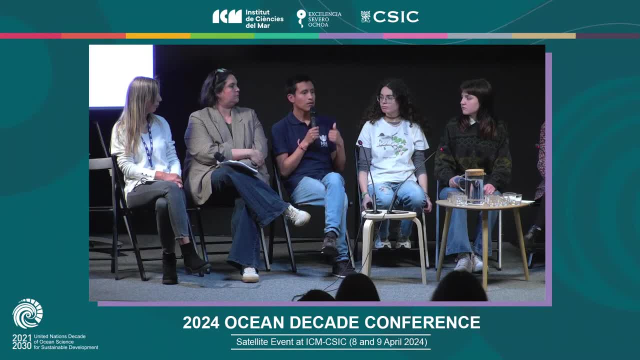 for example, offer a capacity building, a mentorship, a funding researchers that are very important and, yeah, true that a different researchers. we have the possibility to Develop and implement, for example, initiatives or projects around the world basic, for example, in ocean literacy and work near to the 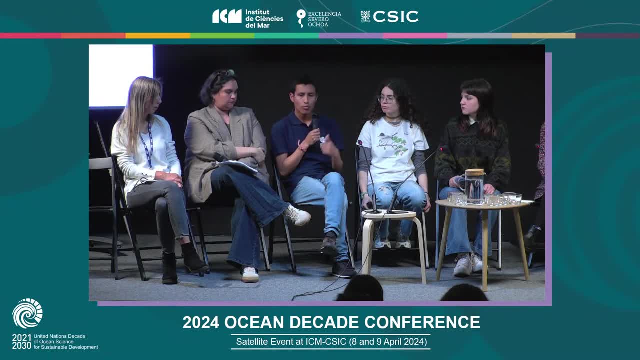 communities, communities from Chile, for example, from here in Spain. so that is the, the main point of a, of the, so a working through this, this program, Yeah, understanding that the most important thing when we are talking about ocean literacies: promote that the people understand how the ocean influence. 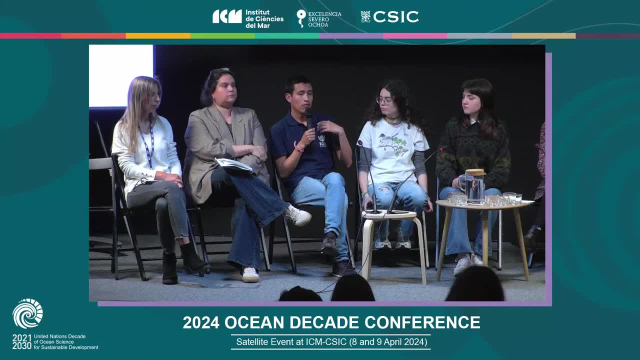 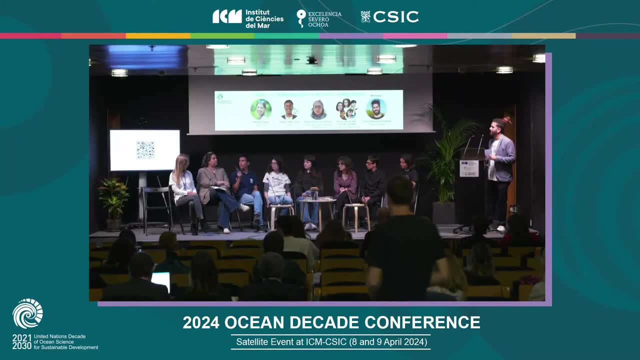 on us and how we influence on on the ocean. so that that is a the information, Thank you. thank you, Joseph. So that's it with your own mic. I have another question, because you were talking about the app that was mentioned in the last panel. 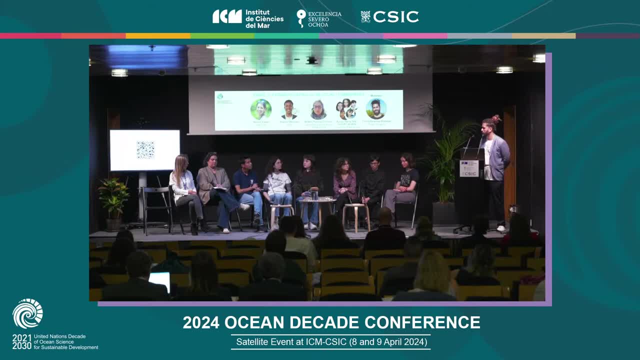 So I want to know: how was the experience of co-creation, How was the co-creation experience of building a communication tool with such a variety of partners, Because you talk about online, offline, I guess it's different profiles, So it sounds like a challenge. 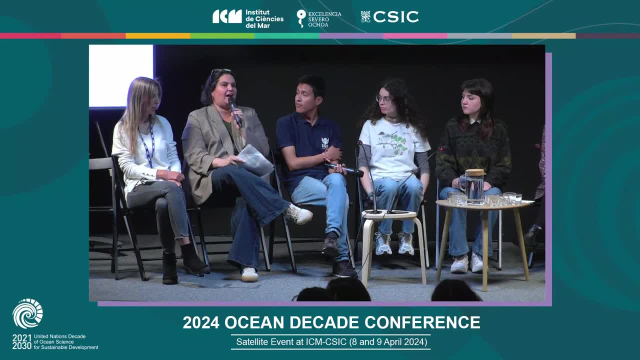 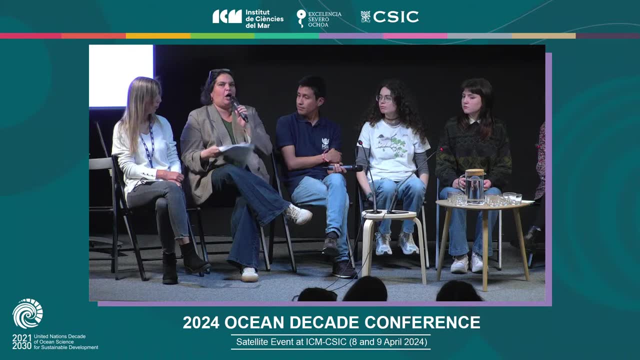 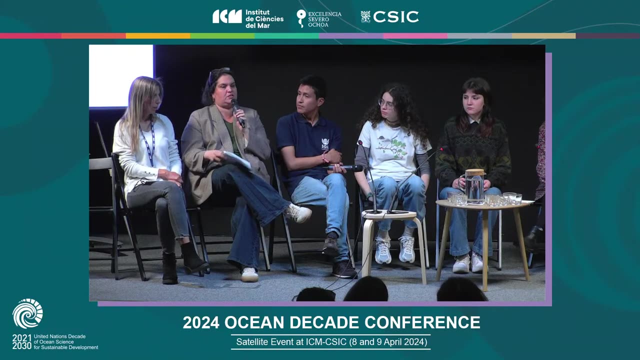 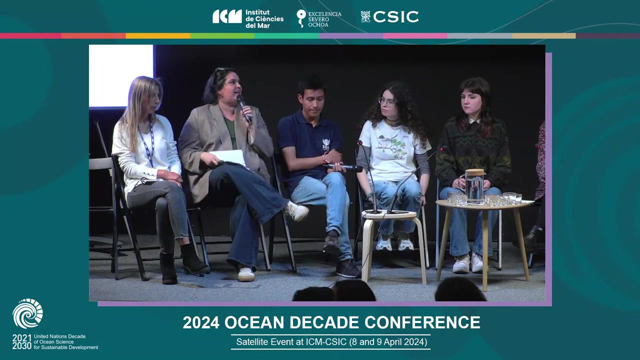 Yes, it was very challenging because the stakeholders of this area- Cab de Creus area- are very historical stakeholders and have a very heavy participation in all social processes And well we know, before the workshops, we know that being impossible to be according to one solution. 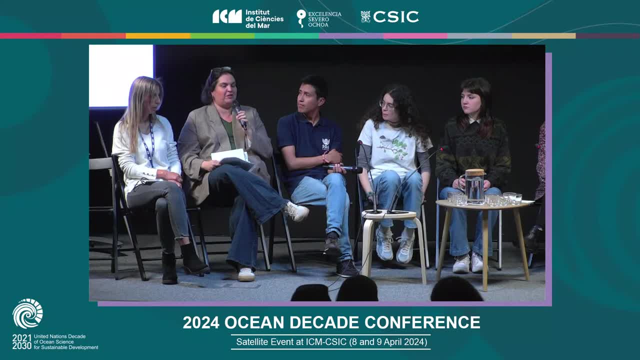 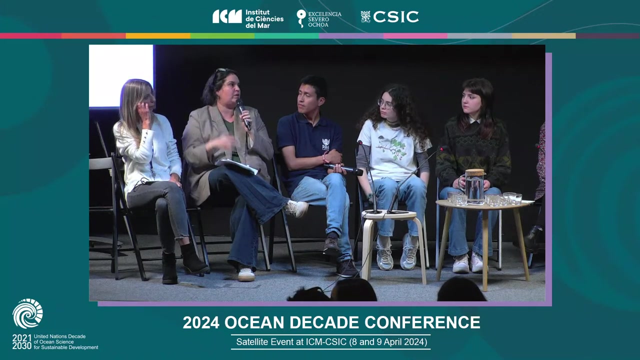 And we are. We are prepared for this situation, But at last we find a formula with an hybrid solution And, for example, for the app- we collected photographies, image, questions for all the community and tried to everyone was represented by the app, for example, 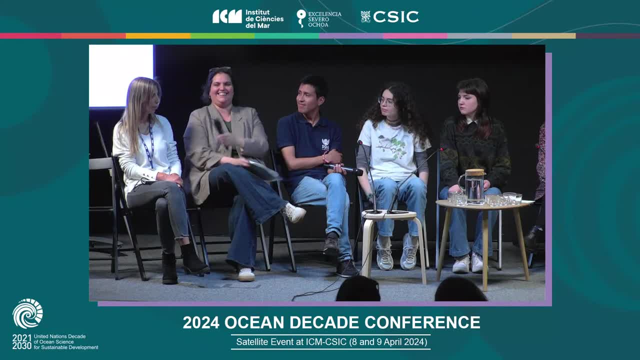 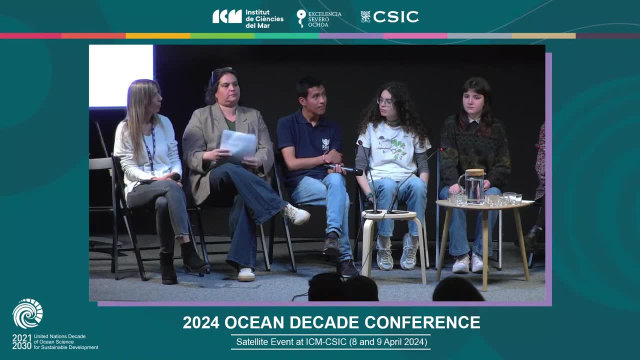 But it was very difficult, Difficult process. yes, Thank you. Thank you, Beatriz, And the last one, Noemi, With your experience, because you talk about the contrast of the survey, doing it in Barcelona, in Africa, in Ghana. you said: 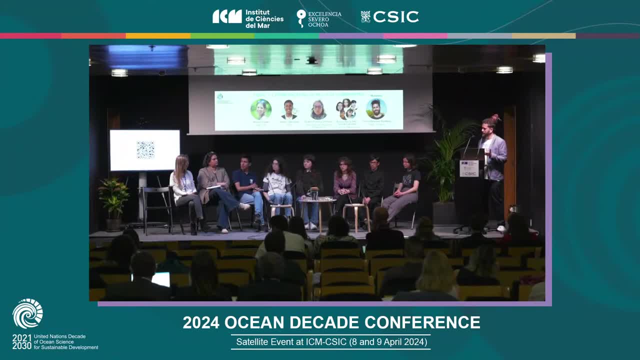 You mentioned Gambia. Gambia, okay, With your experience, do you think direct experiences with the ocean may change people's perception of the ocean, like from sad to happiness? Yes, definitely I think so, But also I think it's important to you know, for the community and for the you know, for the government and for the people who are here, and for the people who are here, and for the public and for the people who are here, and for the public and for the people who are here, and for the people who are here, and for the public. 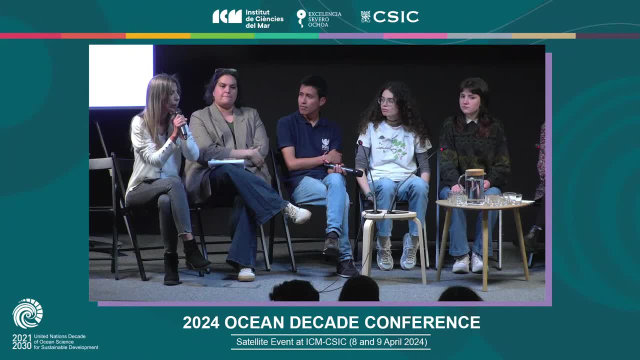 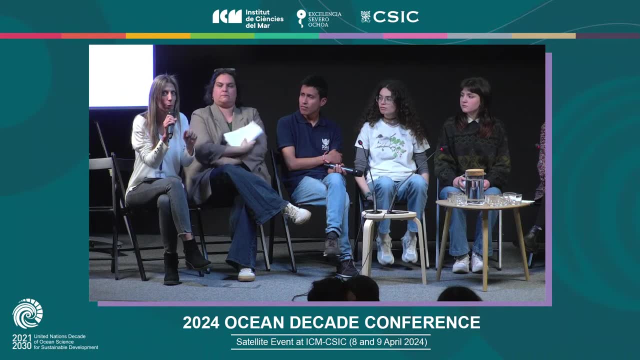 I think it's important to know the cultural background, as I said, And also I would like to add the personal experience with the ocean. We cannot propose the same activity to someone that has a yacht in Cap de Creus than to someone who crawls by boat from Tunisia to Lampedusa. 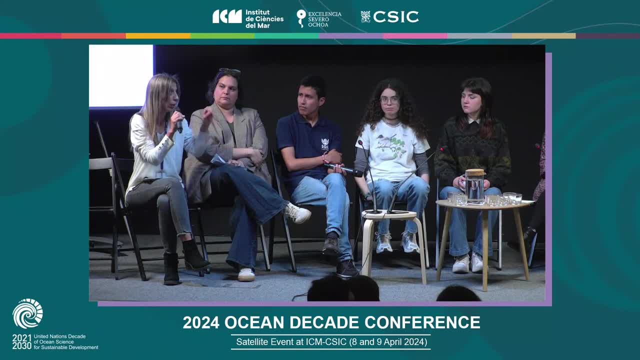 because the experience with the ocean will not be the same, So the starting point must be different. Does it mean that they should be excluded? No, because it's a global goal for all the humanity. So I have two things clear. 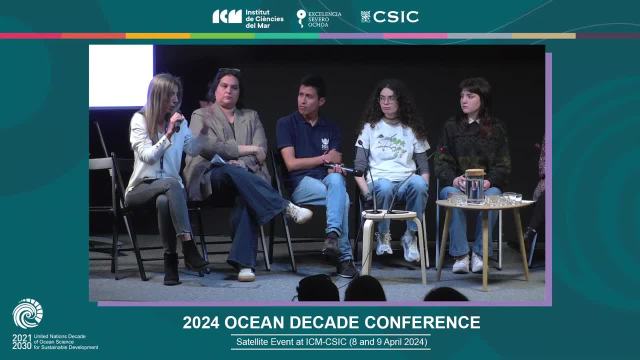 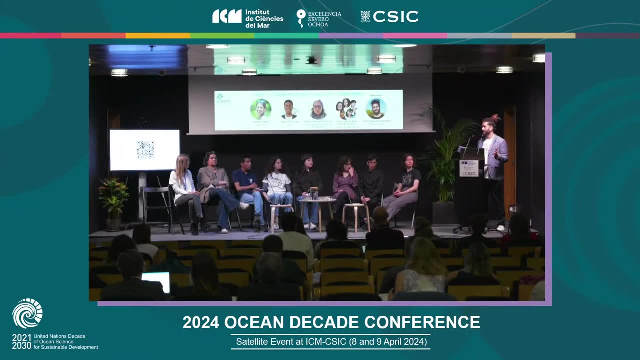 No one can be left behind, but one size doesn't fit all. That's true. that's true. So I think we are running out of time today in this panel, So thank you everyone for listening And, as you have seen, we have different initiatives. 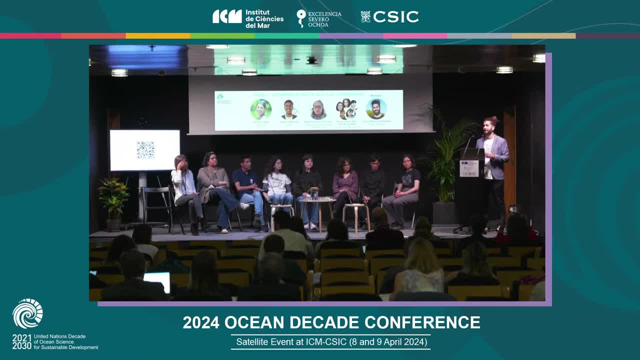 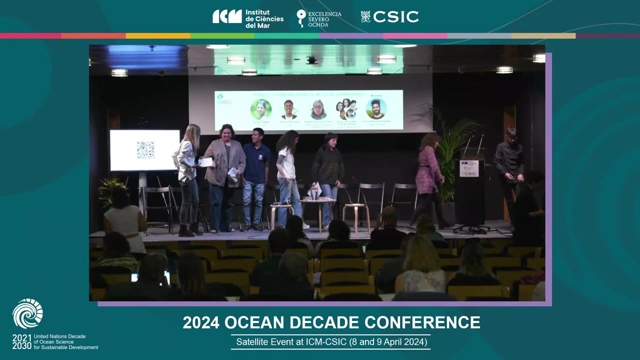 of trying to communicate this ocean literacy And I guess, to wrap up, we need to spend more time in the water. So let's do that. Thank you, Thank you, Thank you, Muchas gracias, Thank you for having us. 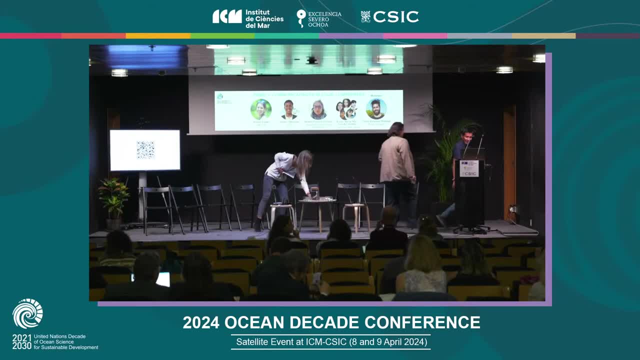 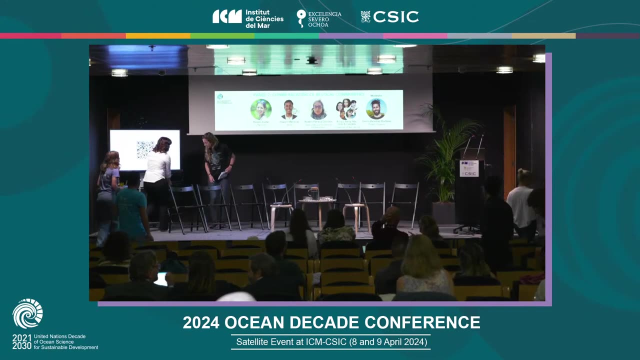 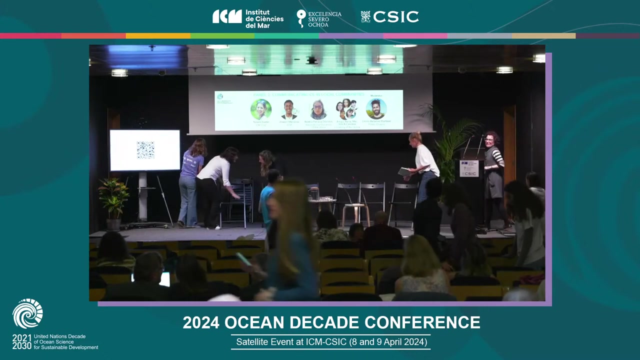 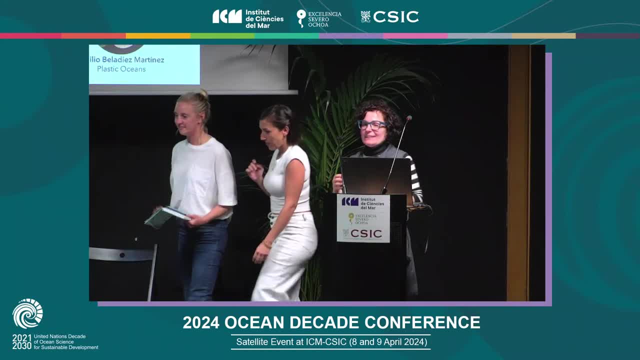 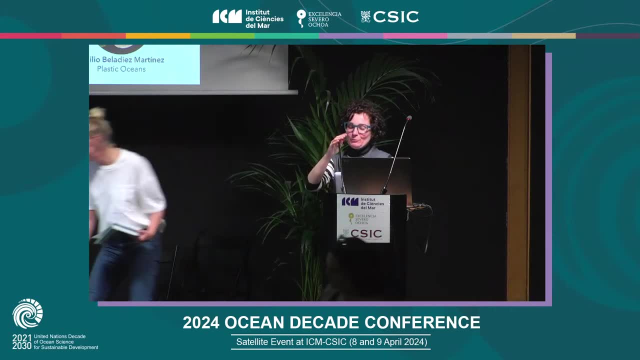 Muchas gracias, Muchas gracias. thank you once again to our panelists and thank you, Emilio, for the perfect synthesis for your panel. and now we are ready for another, another great discussion. that is the last of our event today, so our fourth panel is about ocean. 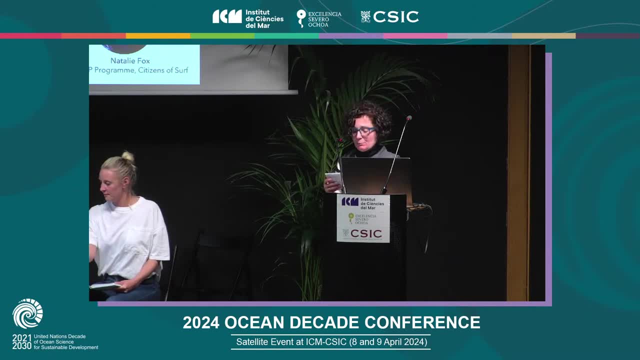 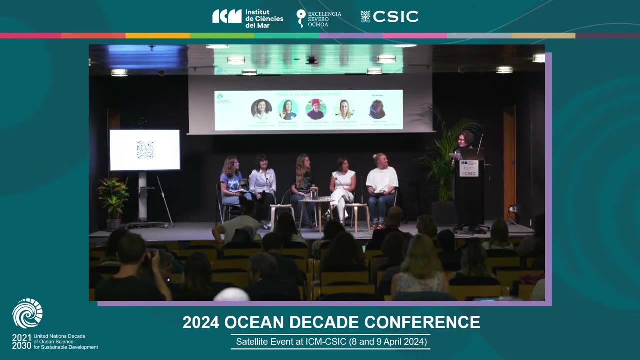 literacy and water sports. it will be moderated by Natalie Fox of the ECO program and citizens of surf, and our panelists are Lucy Hunt from the ocean race and the Irish social literacy Network, Maibe Hermoso from Buceo Consciencia, Giovanna Scagnolatto from Tata UGA and. 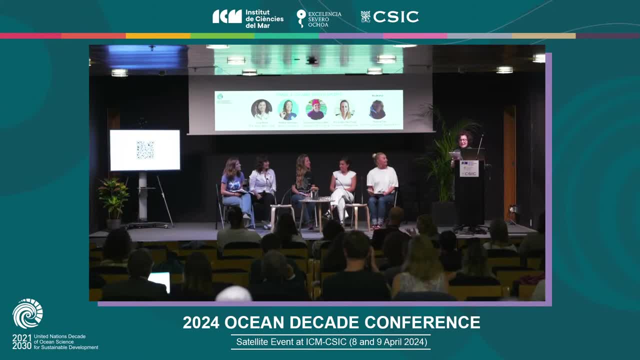 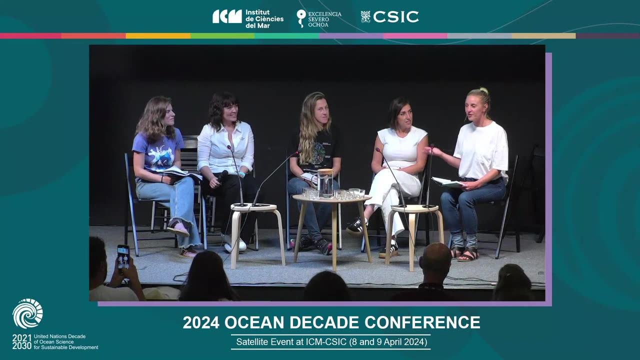 sustainable ocean, ocean alliance, Campinas and Anna Sanchez-Biddle from the University of Barcelona. thank you, thank you everyone, and so yes, on that note, we should spend more time in the water. we have amazing panelist that are all working in, on or under the water and have ocean literacy. 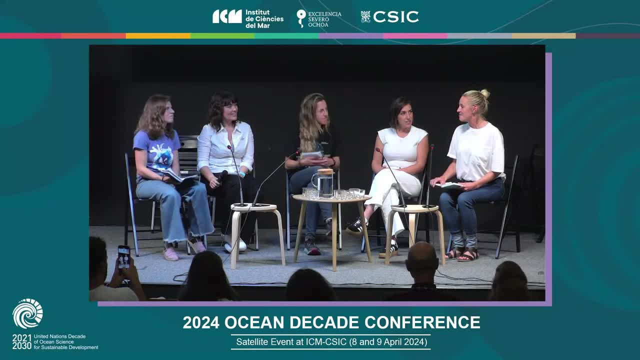 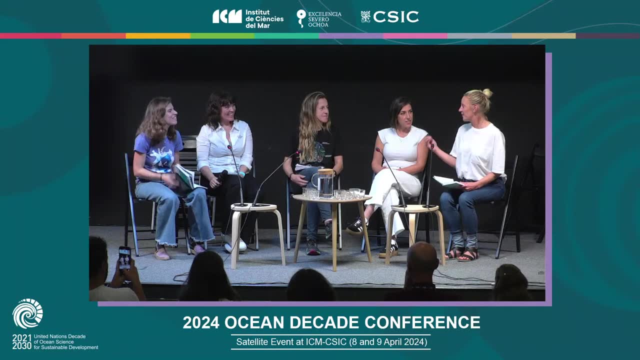 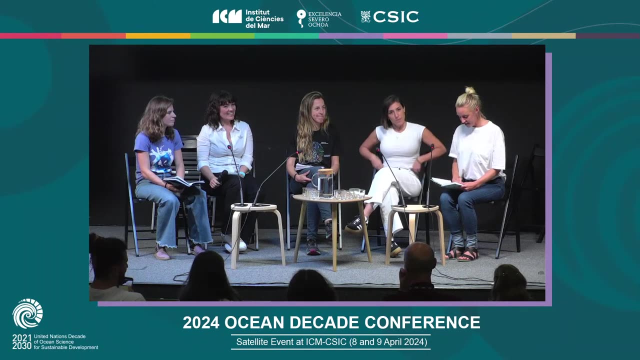 integrated into their activities and impact. so we don't have much time left. so we're gonna stick with one question and it will try to have a lot of information in that one question, and it just encouraged you to take the QR code so that you can have more information about each of the projects, and we're gonna 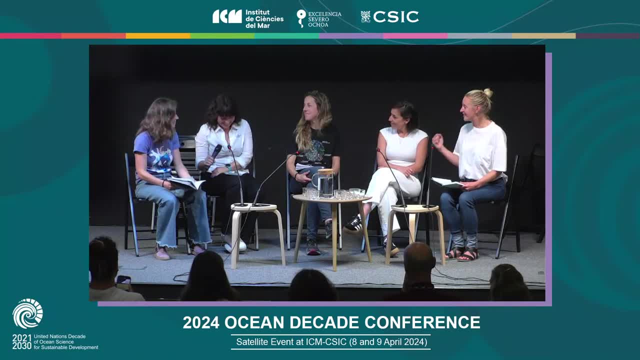 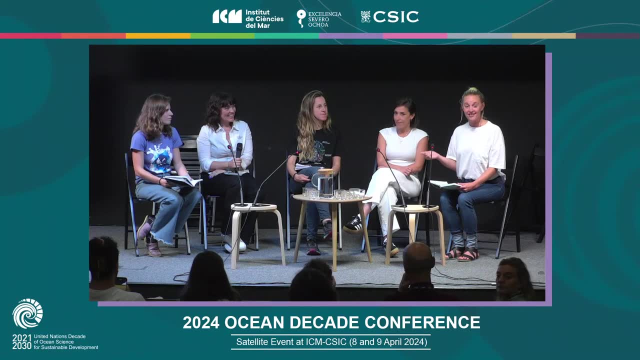 start with Lucy, who's managed to make it here across town in the Barcelona traffic, Thank you. So here we are, back at the ocean race, and the Strava N95 is fairly much a business model. there's running a preached objective and one of the 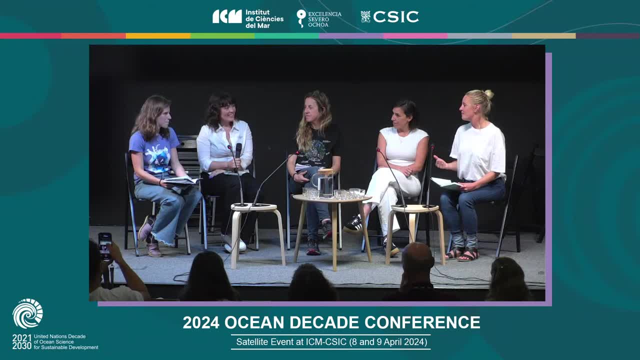 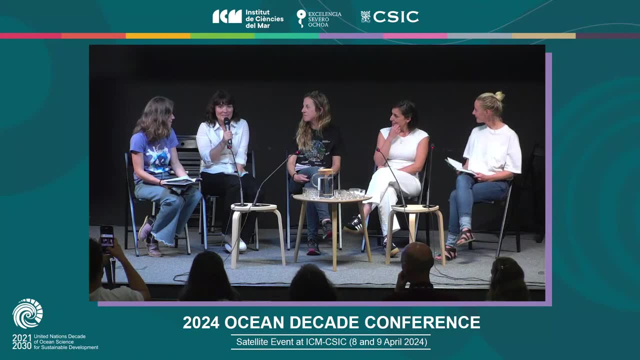 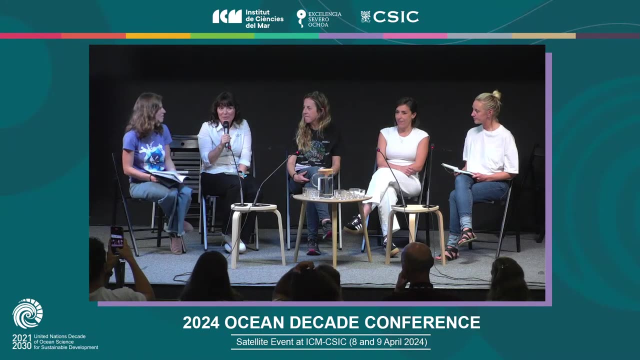 lessons learned from the ocean race is that sport as a team of professional sports is based on competition, and so tell us a bit about the ocean race, which is very exciting and engaging competition. how do you leverage that to encourage a more collaborative and, like, caring sense for the ocean? 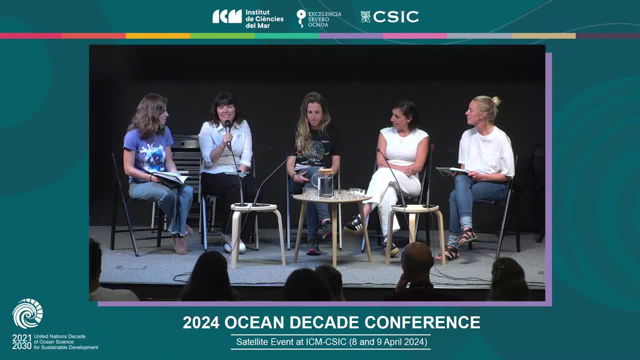 sailing race. it's pretty epic. it lasts for about six to nine months and it happens every four years and it's the pinnacle of sailors careers, like an ever the everest for them. so we actually have a whole sustainability program called racing with purpose, that the race itself is now known as. 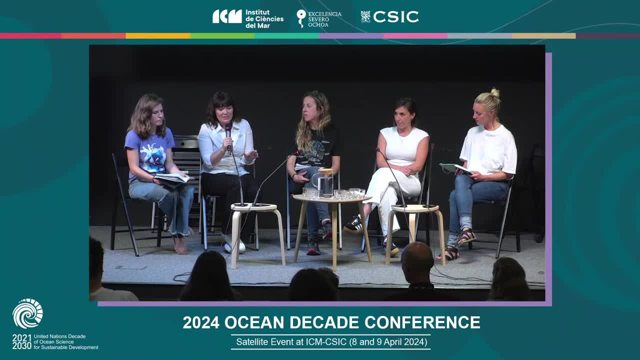 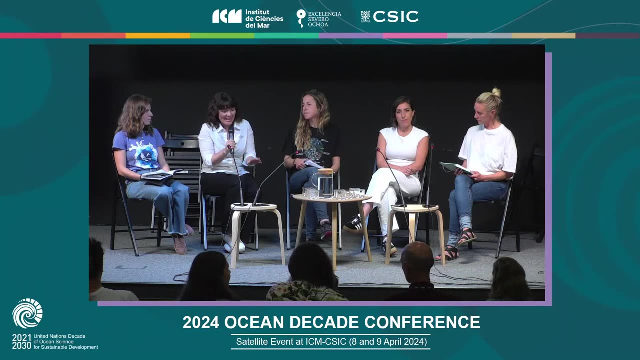 as the most having the most comprehensive scientific program. because we've science on board and I'd like to extend that to a sporting event with probably the most comprehensive ocean literacy program as well. because we have our resources for primary school and secondary schools, developed in 11 languages that are rolled out in 80 different countries with over 250,000 students. 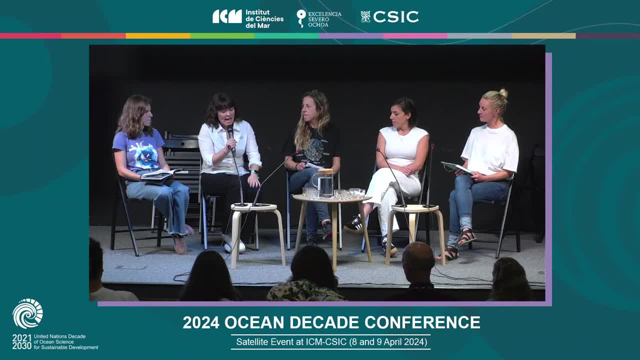 since it started in 2017, and so, yeah, it's a competition, it's grueling. the sailors are amazing to be out there and for the students it's really engaging. it's exciting because they get to see these amazing human beings, but they get inspired by them because they think one day maybe I can be out there too. 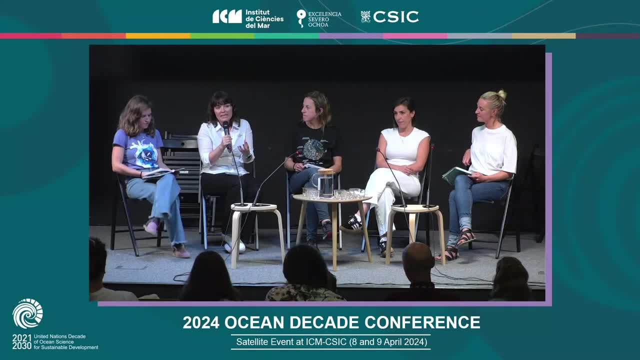 and then for the racers. it's really nice for them because they can engage with students and they can talk to them about what they're seeing out on the ocean. so some of the things that they're seeing is, you know, less wildlife over the years and more plastic pollution and some of the 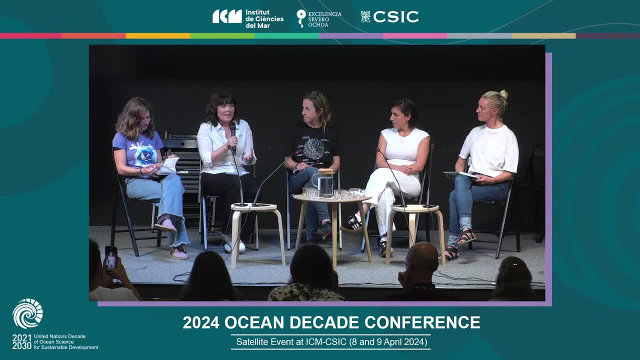 exercise is, then, that we ask, through our ocean literacy program, is to imagine that you're an ocean racer and imagine what you might be seeing out there and how would you communicate it. so it gets them into that thinking of being out there on the ocean, connecting with the ocean, and then part of our 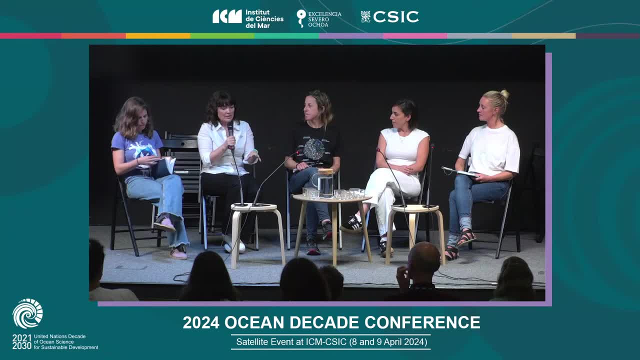 program is when we go to the different host cities around the world and there can be up to eight host cities. in that six months. we engage thousands of kids and invite them down to the race village. so we have a whole ocean literacy program which is like an exhibition, and they go to different workshops and have lots of 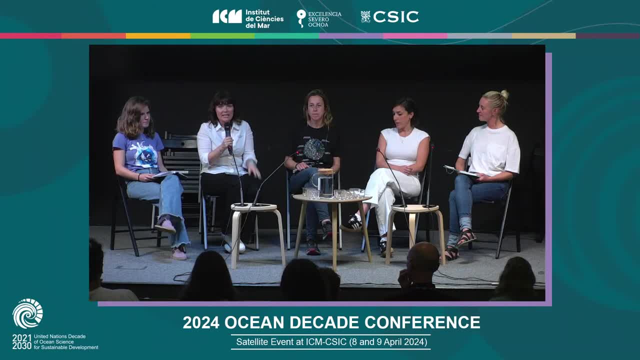 hands on experience and get to see the boats and some of the sailors as well. so it's really engaging and inspiring. and then, just to let you know, our generation ocean program, which is our secondary school learning program. it was the first ever ocean literacy resource that started to talk, or started 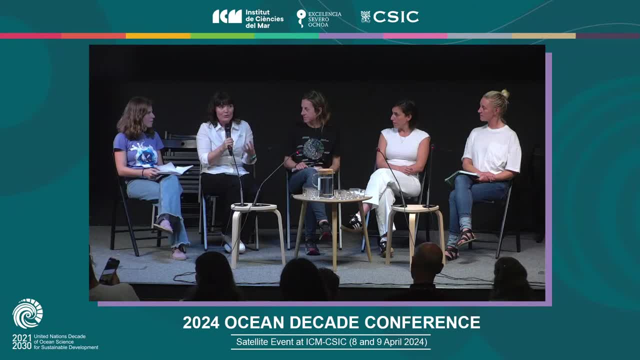 to have content on that eco centric Sort of viewpoint, so talking around ocean rights and and viewing the ocean as a person, that's in itself so a very different way to our anthropocentric sort of viewing, which Sylvia I think was speaking about when I came in earlier. so it's a there's some really great. 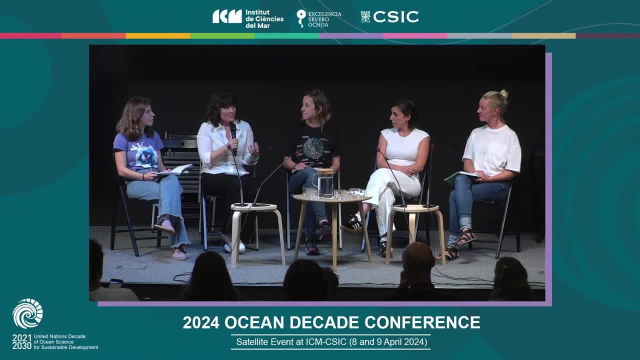 resources. it helps to inspire kids. it helps them to like, learn about the ocean, and then in an exciting way as well. so, yeah, if anyone wants to talk to a bit more- because there's a lot more to it- I'd love to speak to you after. 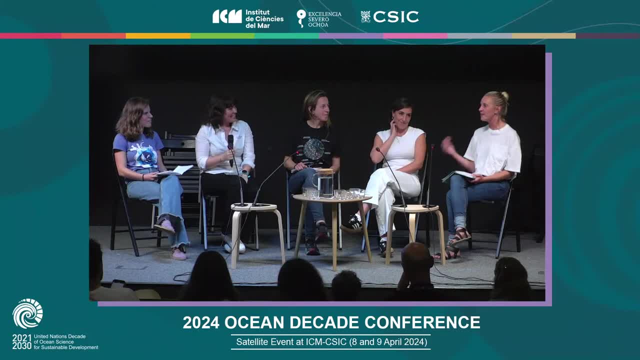 Thank you. Thank you, Lucy, And so talking about that observation of people being out at sea, diving, is a different way of observing the ocean, maybe a lot slower and a lot less rough. so talk to us, maybe about your work and how you're transforming the consciousness of divers. 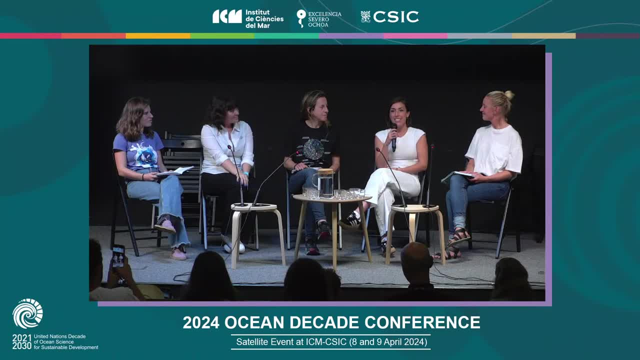 Okay, thank you. In my case, my project was born from the result of my thesis, of my doctoral thesis. I was trying to understand the how divers wanted to participate in citizen science project. We found that they they wanted to participate a lot, but they their main barrier was the knowledge about marine biology. and they really what they really wanted to learn about marine biology, but they didn't know how to do that. 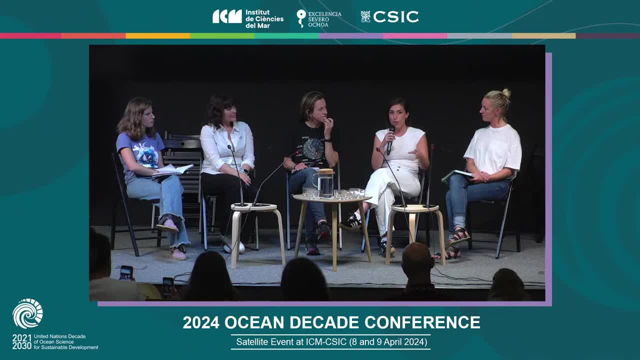 No, they don't have like a recourse to do that, So I So I found that both their content here that it is- and We are creating like innovative experience in education in marine biology, specifically for scuba diving industry. We have marine online courses, very like dynamic visuals fans know, because we are teaching for people who do that. 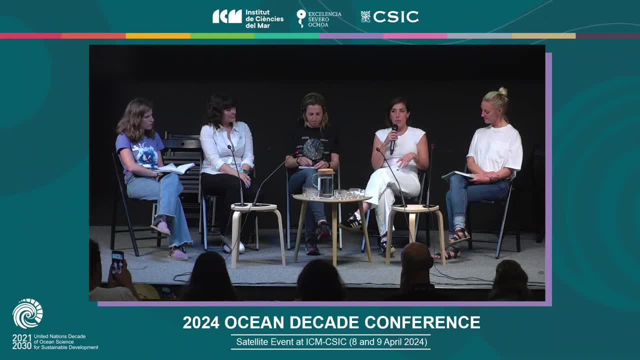 By recreation Right. We also have, like the typical diving trip to Maldives, with sea or something like that, But with the main objective to learn about the marine biodiversity in these places. We have leader also the world record, So the The number of scuba diver participating in citizen science in one day. 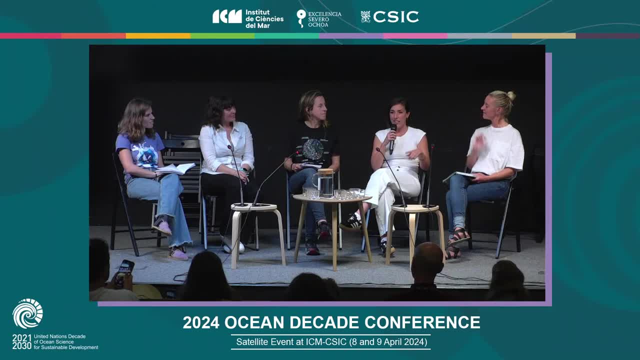 No, With here, with observadores del mar In the same, And that kind of things is what we do, What our main objective is: to teach diver about marine biology to, for empower them to leader marine conservation initiative- Because we think they are very important- or strategic group of marine user. 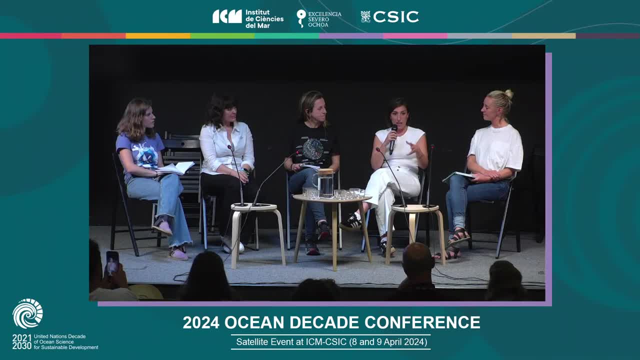 Because they are who. they are the witness of what is happening under the sea. They can detect pollution points. They can. They are the first who can see an invasive species. They are who feel the chain in the under the sea, No, in the marine ecosystem. 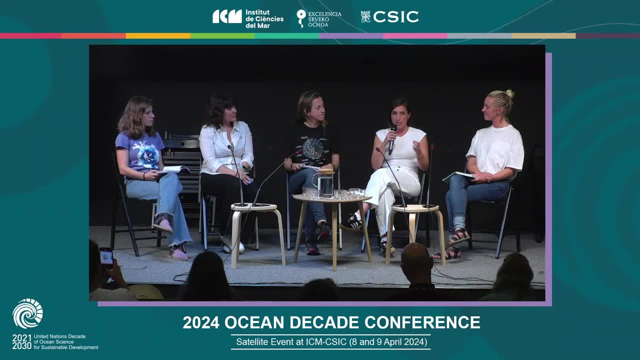 So They are very strategic, They. But To get this We need them to know about marine biology, to have all these Things from there, No, So We're trying to empower them to ocean literacy And From the knowledge. 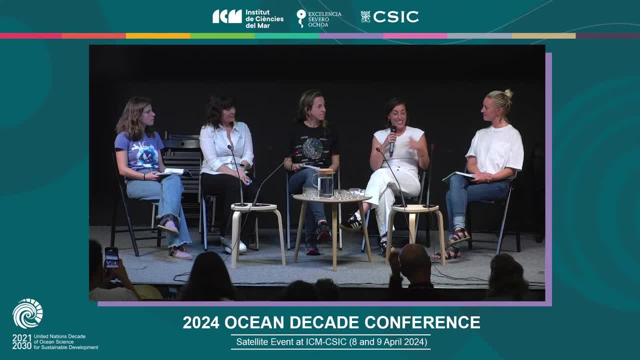 No. And We have Say a lot of time like the, no green, no blue. And From the content, Yeah, We say No black, No blue, Because we really think we need the divers empower To marine conservation and 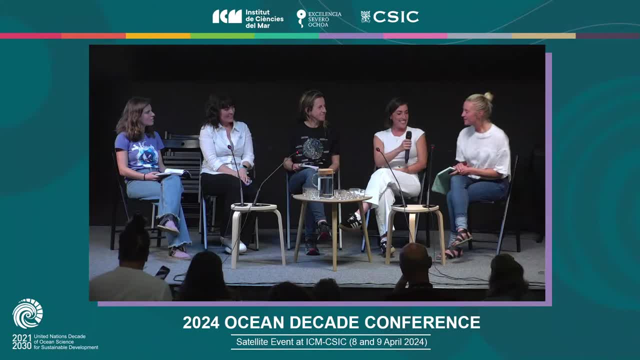 Protection of the sea. So there's like a A jump there from ocean literacy to then Being marine Citizen scientists. So, Anna, This is your work. You have Been using different tools to engage Ocean users, So introduce us to your project. 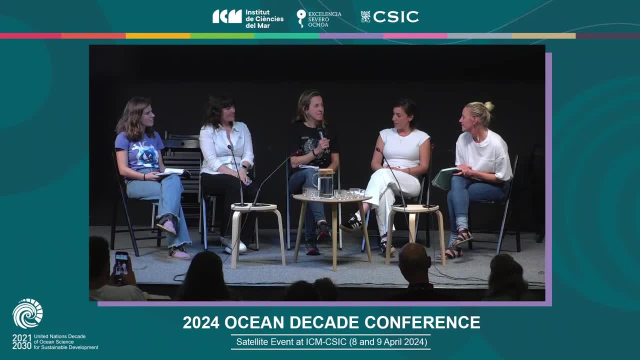 I had a go at it this morning, Actually Thanks to you, Yeah, Thanks to you- and Ari. So Thank you, Natalie. So, Yes, In In Like, Six years ago We designed it, We invented the. 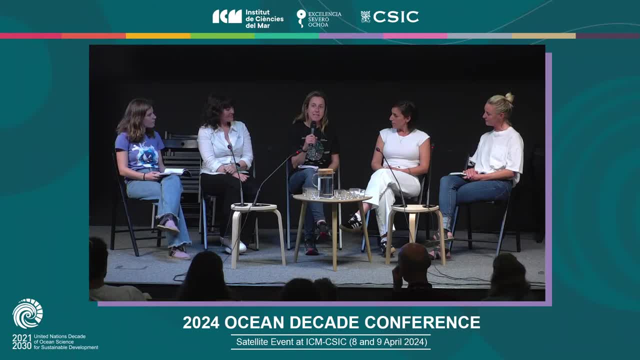 To collect Floating plastics From the very near shore. In fact, Is that Because I use it this morning. Really, If you want to Just show a little bit, This is a very Easy to use And cheap, Affordable. 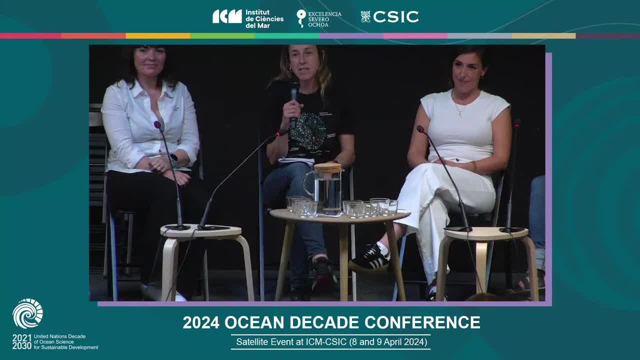 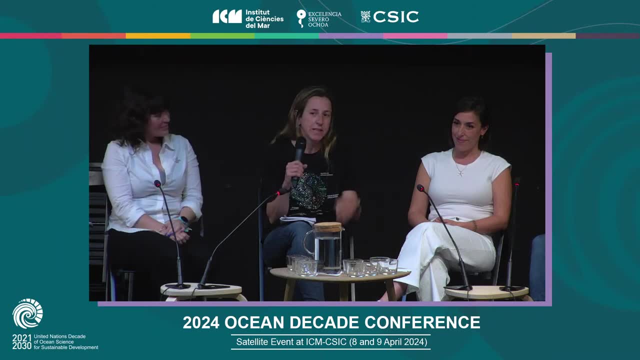 Troll That can be towed From Surfboards, Rowing Boats, Kayaks And whatever Floating Device. So With this Troll We Built Citizen Science Initiative. We have Around 15.. 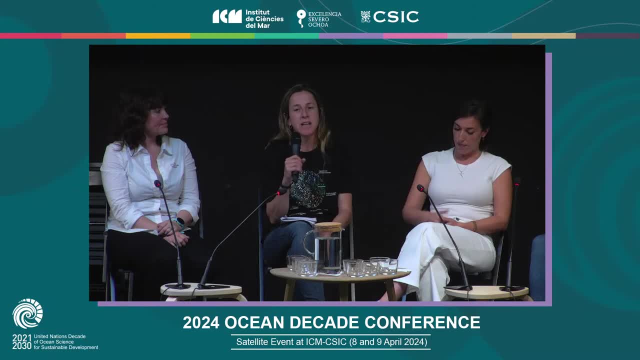 Of these Trolls, Collect samples For us. Together, With the help Of Survivor Foundation, We have this project That's called Surfing For science. And Well, We have been able To Collect. 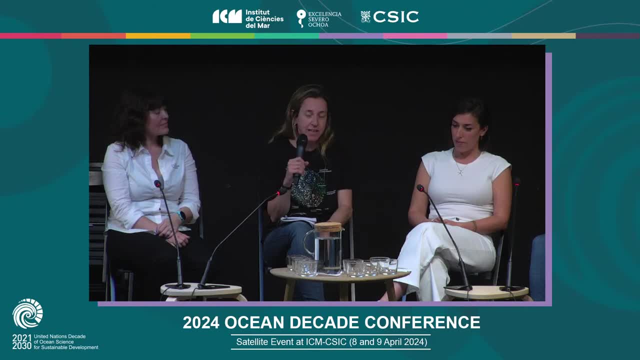 And Characterize. So We know The size, The area, The color, The shape, The region And the polymer Of more than 100,000. Microplastics. So We Have A lot. 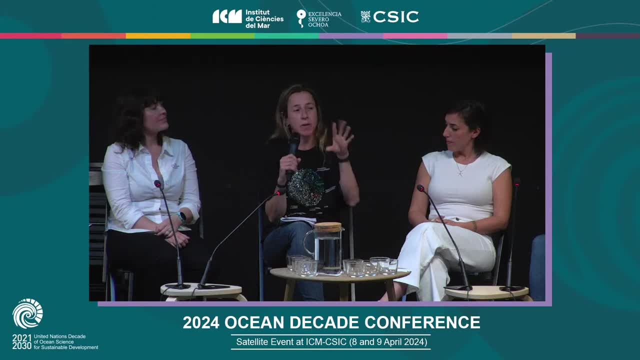 Of Disseminators. So We Have An Instagram Account That's Called Surfing For science Lab, Where We Put All The Scientific Samples There And We 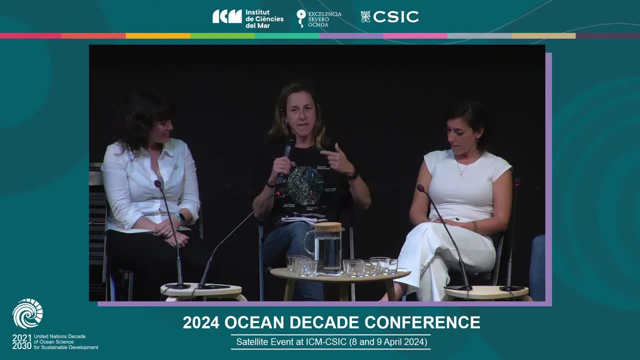 Also Made Some People Do The Same, That As I'm Doing Now That Look, This Is Artificial Turf. These Are Microbeads, These Are Pellets. 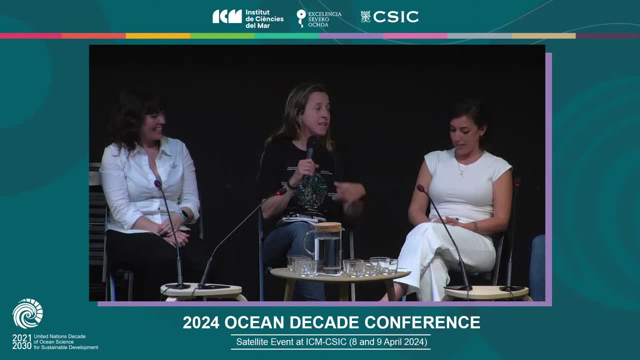 These Are Fragments, These Are Films, So We Have There A Lot Of The Participants Of The Project That We Have Like Four Pilot Interventions. 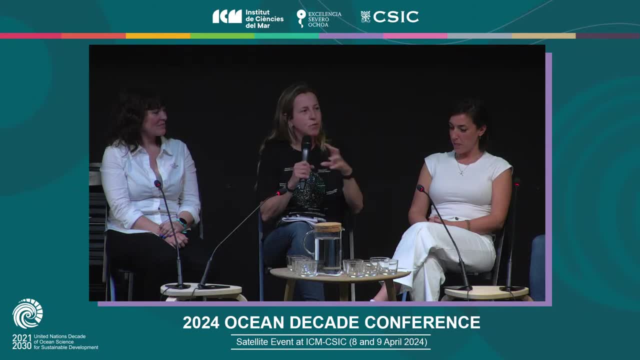 With Different Sports- Surf, Diving, Sailing And Kayaking- In Different Countries- And We Have A Lot Of Artificial Turf And We Have A Lot. 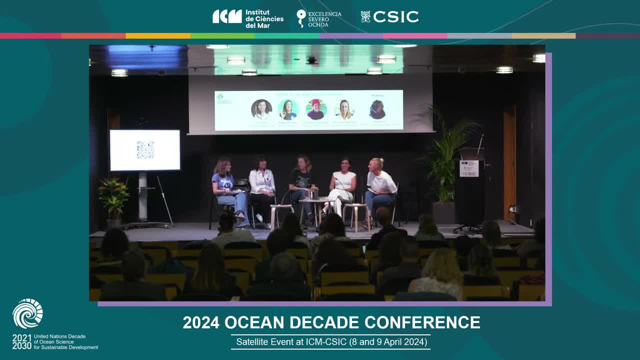 Of Artificial Sports Diving, And We Have A Lot Of Artificial Diving And We Have A Lot Of Artificial Turf And We Have A 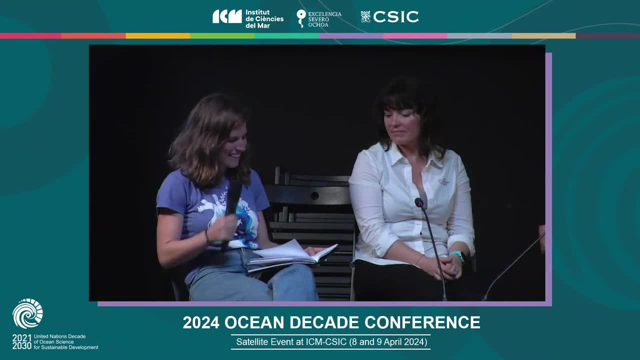 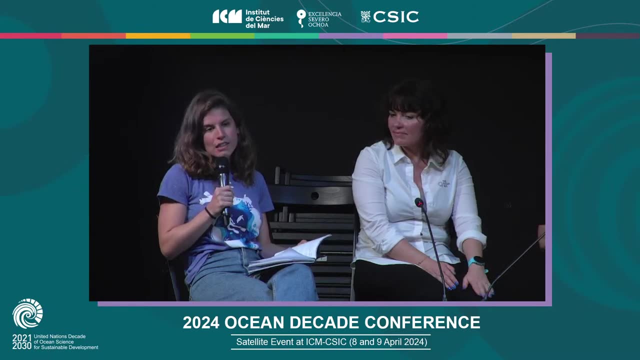 Lot Of Spieler's Space And We Have A There For More Substance And Diving Like A Diving. And So My ары situation and these young. they study in public schools in Brazil and they live in. 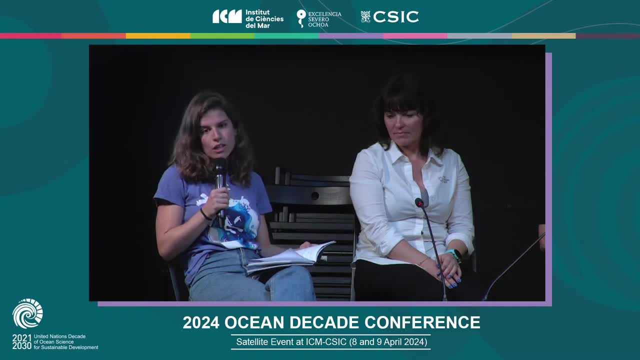 coastal areas, We offer our ocean literacy course and after we take them to explore the underwater world with scuba diving. We use scuba diving as a tool and we believe this unique and wonderful experience can turn transform them. I don't know the reality in other countries, but in Brazil we have a huge difference between 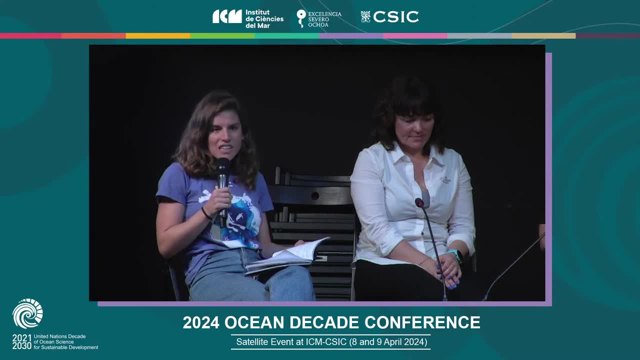 public schools and private schools, and topics such as environmental education, ocean literacy usually is not addressed for them in public schools. So we try to stop this gap And change this because these young, they face daily with humans' impacts like climate. 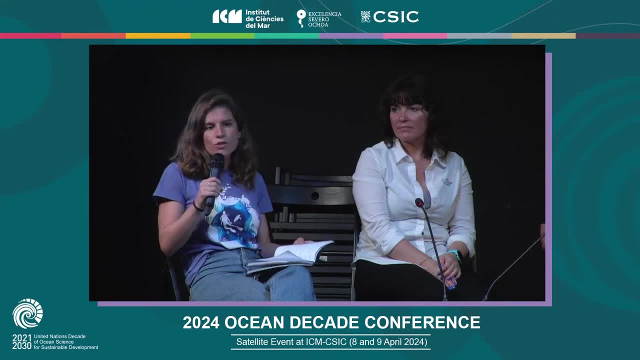 change, overfishing, ocean pollution. Of course this affects all the people, but then they live in coastal areas and their sustenance came from ocean or coastal environments. And uh How the access is limited for them about these topics. they don't know, they often 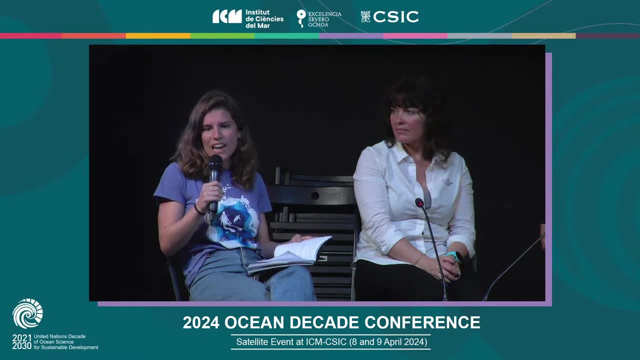 they usually don't know how to advocate for their rights, So we try to pass the knowledge for them and encourage them to advocate for their space, their lives, their environment, their ocean. We truly believe We only take care of what we love. 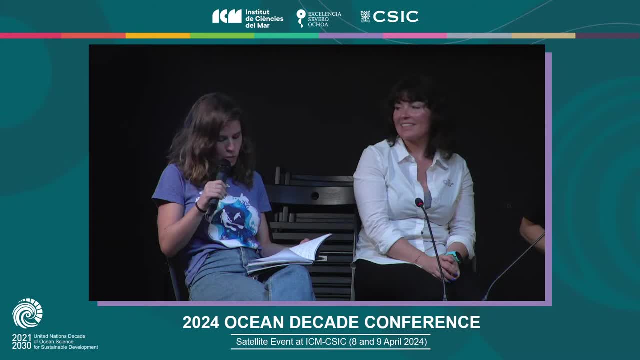 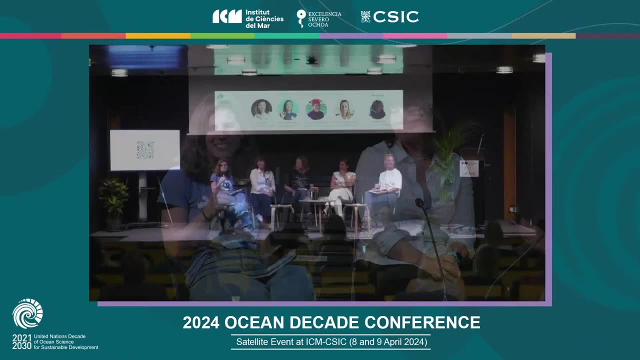 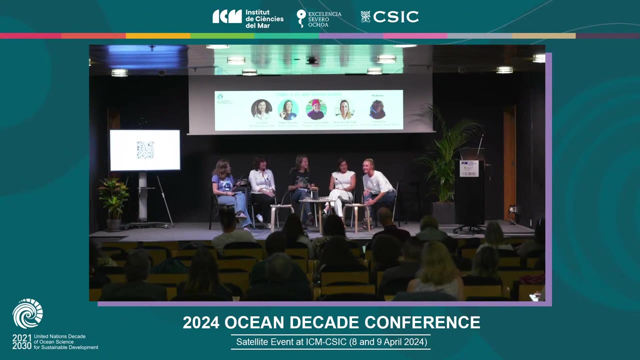 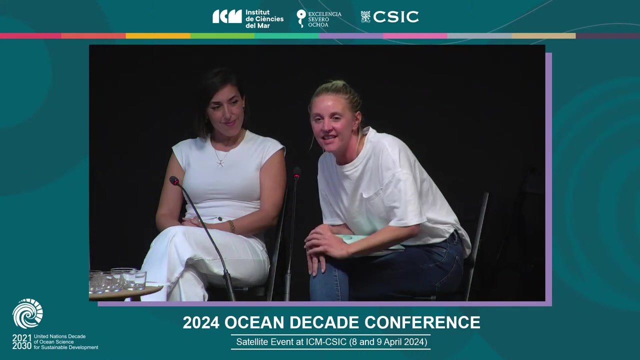 And we just love what we know and understand. So we try to do this for them and for all the people, I think, because this is the point where we're supposed to end the event, maybe I'll open the floor just to see if anyone has a question. 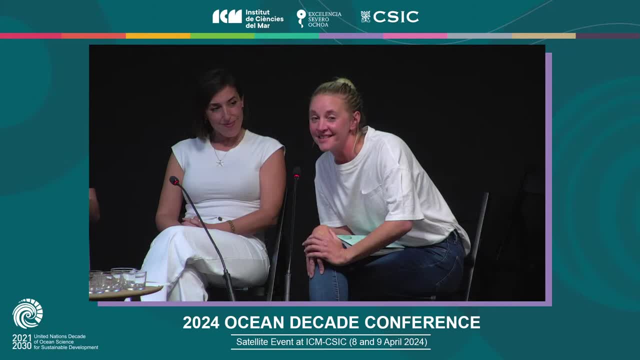 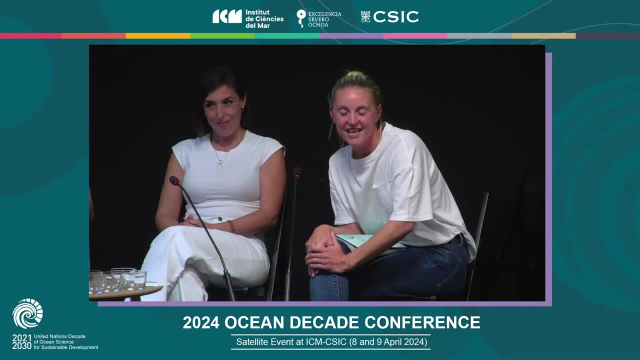 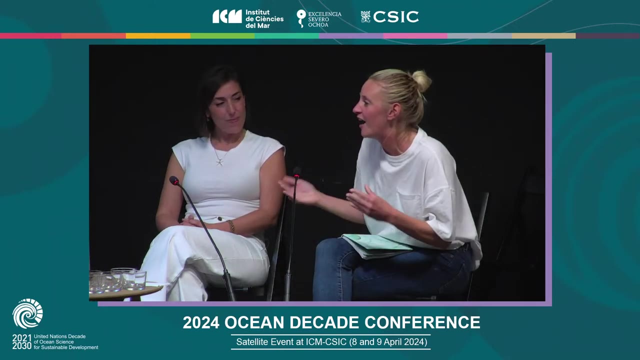 And if not, we can maybe wrap up and then we will be finishing on time, because I'm sure everyone has got a very busy day. So if there are any questions, then go for it. I have a question actually. My question is: so it's easy to see how water sports and ocean literacy go together, and 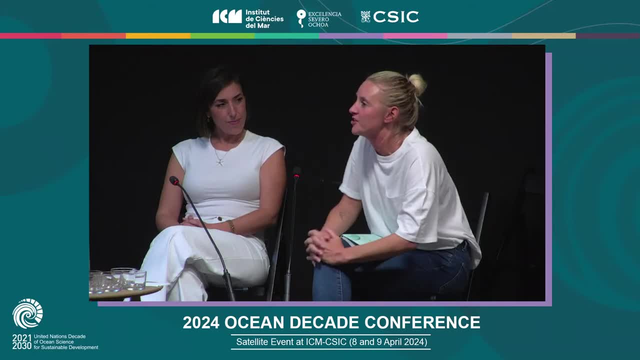 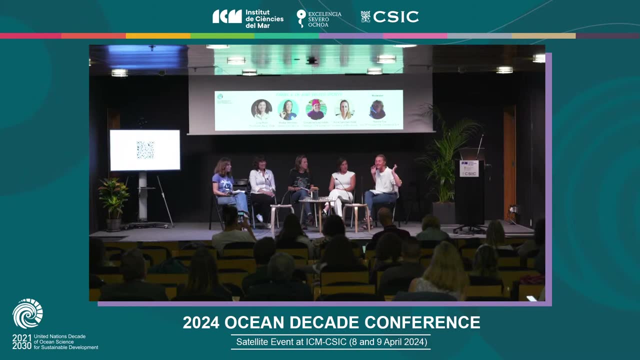 can help us as humans and also help the ocean. But what about other sports where water is not involved? How can we get ocean literacy out beyond these kind of blue spaces? Yeah, any ideas, maybe to the audience as well? I think you, water sports can, can be a. 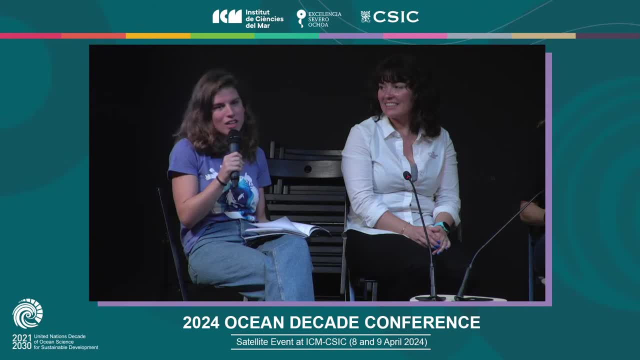 great tool to ocean literacy, especially scuba diving. when you can see the marine life with her own eyes, reef in the water, it's, it's amazing, it's indescribable. so I think it's a good, good tool, but it's difficult because in Brazil scuba diving it's a elite sport, it's a. it's very expensive, it's not. 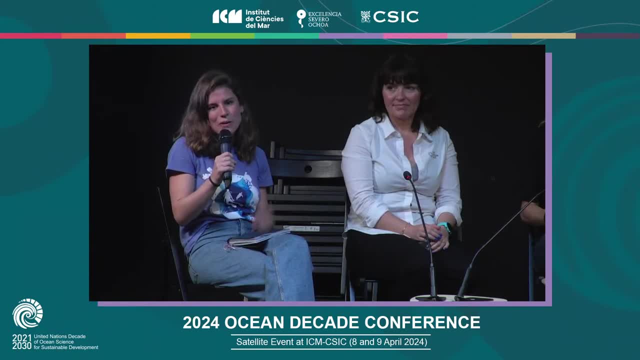 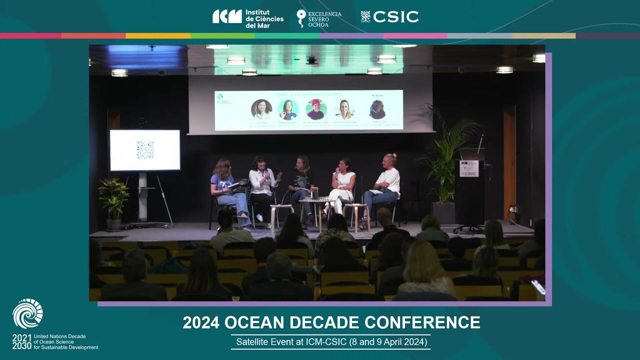 accessible for many. so we need to, to, to be partnerships, fundings, to to provide this for social vulnerability, community units and this, yeah, just quickly I suppose as well. the ocean race lends itself to ocean literacy, but I think there are innovative ways that we can engage other communities. we are all ocean citizens. we all breathe the same. 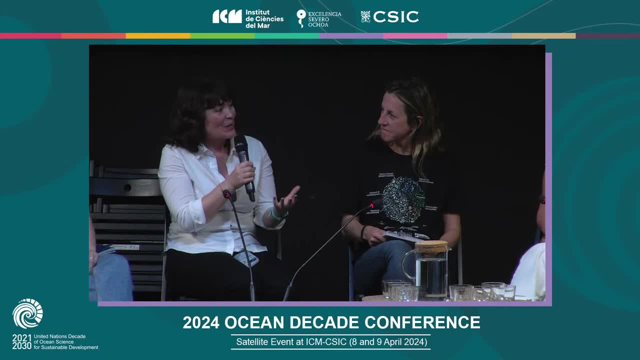 air that is created by mother ocean, so in there's definitely creative people out there that can help you with that. so I think it's a great tool to be able to help in campaigns. you know, if it's a football game, there could be some cool billboards or things like that. you know, there's definitely ways that we can be. 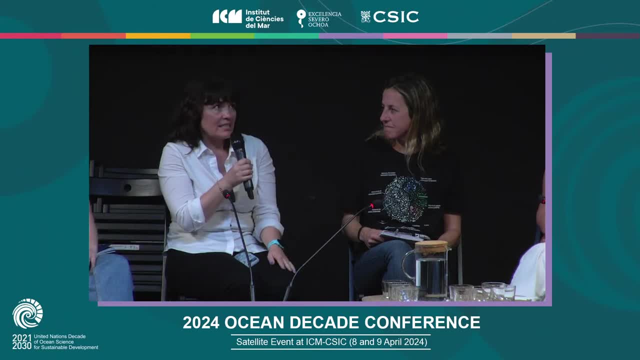 innovative when it comes to communicating about the ocean, because that, this, that it's that whole thing of communicating. we're all part of the one system. we're all in this universe together, all breathing the same air, all all of us working towards the same things. but there's many other people. 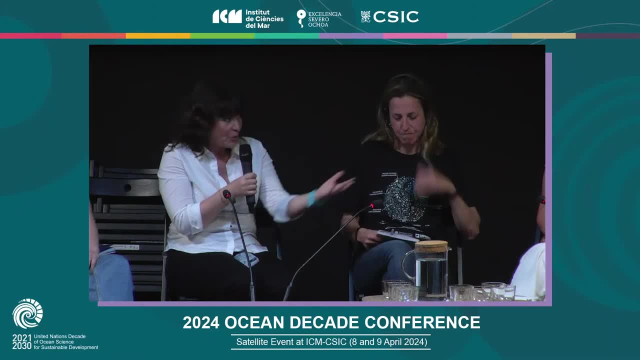 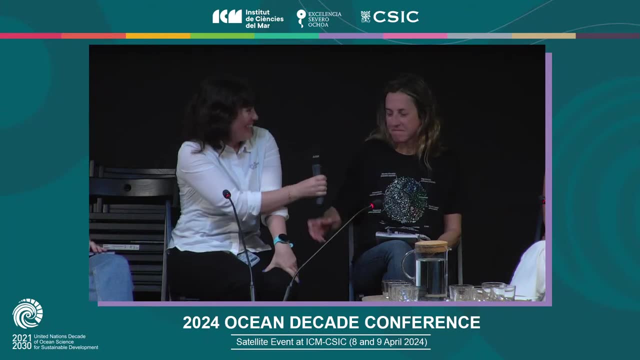 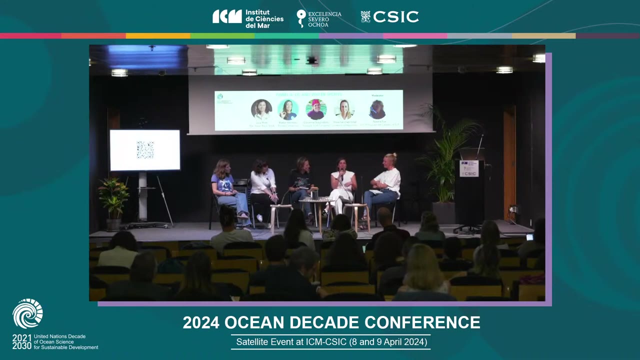 that aren't even aware of. so if we can engage those people- true, these different sports that you're saying, you know it gives you so much hope. Yeah, there we go In my case. I just want to say that when I was in my studies about the participation, 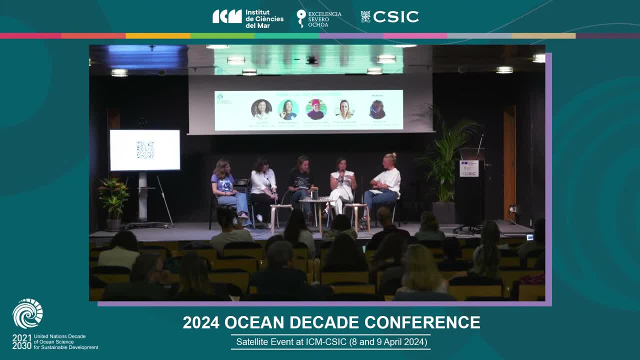 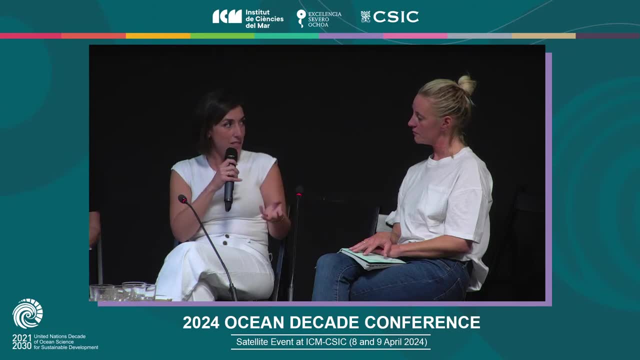 in Citizen Science. what I feel is that when you are working with a community that is previous, that previously exists, it's like easier to make them to participate in science. So in this case, just like if they are in a sport community, 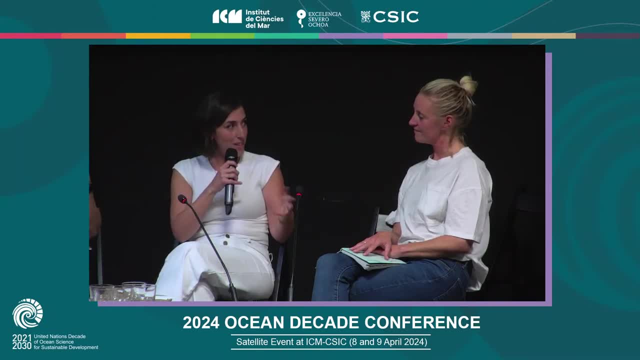 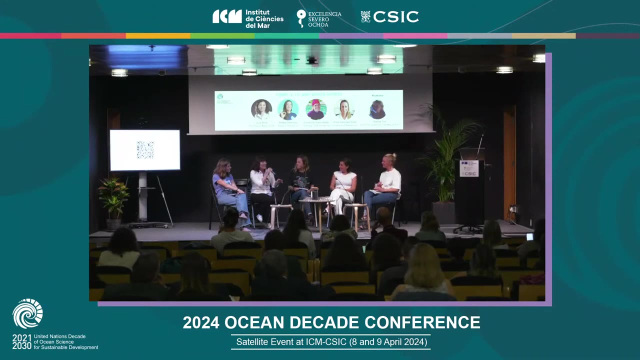 you can like, invite them, talk to them in their idiom, with their interest to try to get closer to the ocean or that kind of thing. And just one thing to add: if we engage, the sporting heroes like so, our sailors are advocates for the ocean. 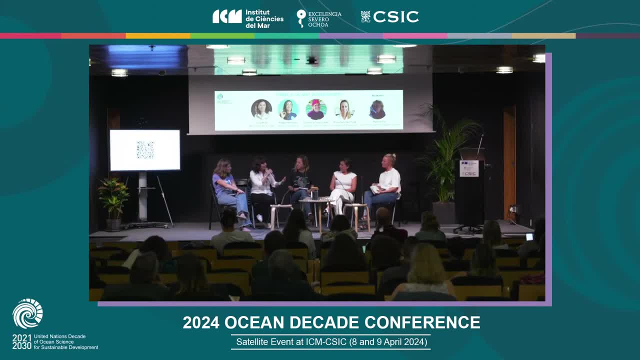 but if you have the Messi's of football or whoever it is getting engaged, they bring their fans with them. So it is about like connecting with people so that and offering them those ocean experiences, so that they know how important the ocean is. 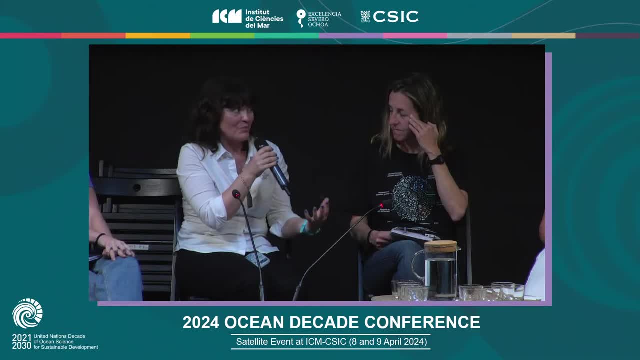 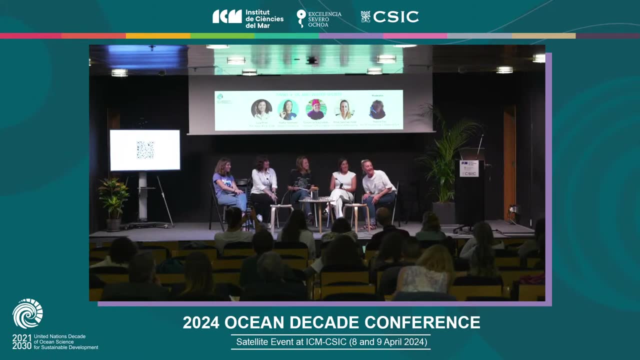 And then they can also bring thousands of people with them once they start talking about it. Okay, Yeah, amazing. Thank you to all of my panelists and thank you, Maria. I think we're wrapping up, So, Yeah, I'm going to. 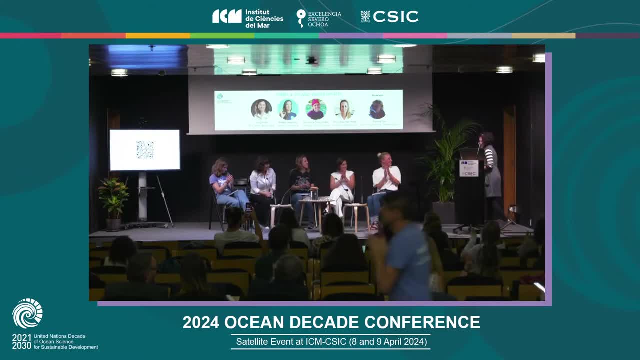 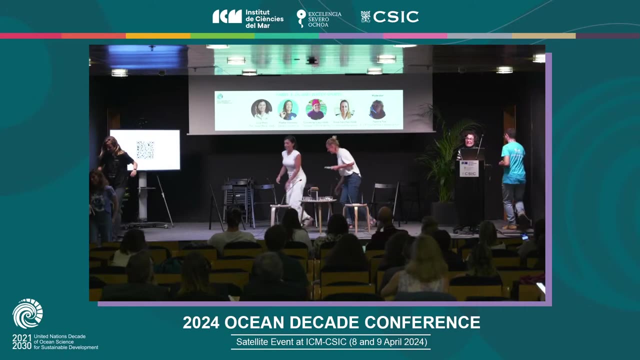 should we stay? We had, well, it's not even. we had just the last slide. Goodbye, but no, thank you very much all. I hope you all enjoyed as much as I did these wonderful stories from all over the world actually. 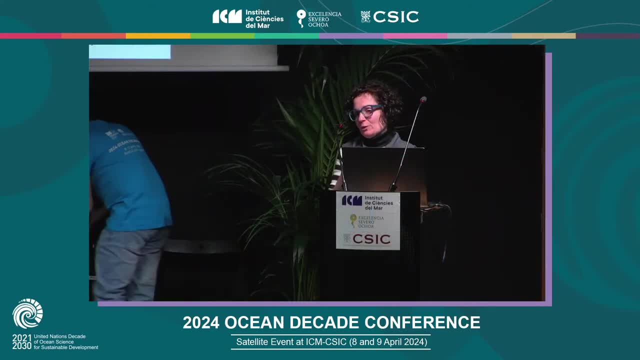 And with this journey, so today, we have discovered so many ways to bring ocean literacy out there. So, as I said at the beginning of the event, to connect ourselves with the ocean. but we don't want this journey to finish today. 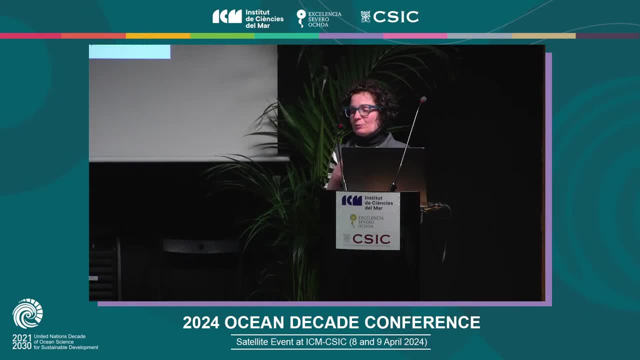 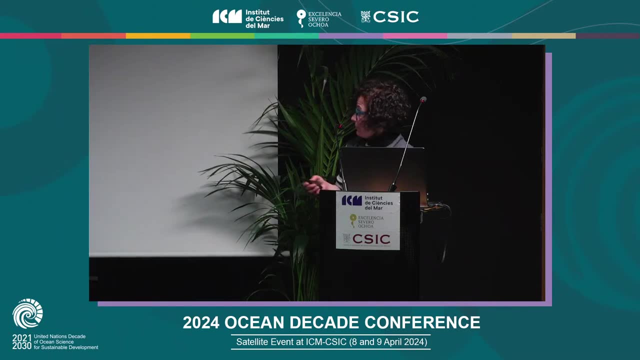 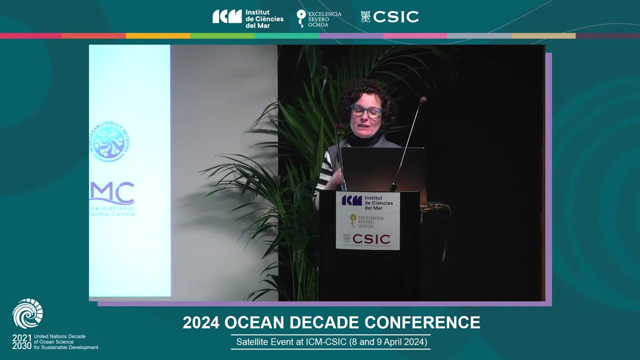 Our intention after this event is to continue bringing more the knowledge of all the different ways we can create this connection, change these relationships between us and the ocean through a white paper. So we want to bring together all the results of this conversation today.